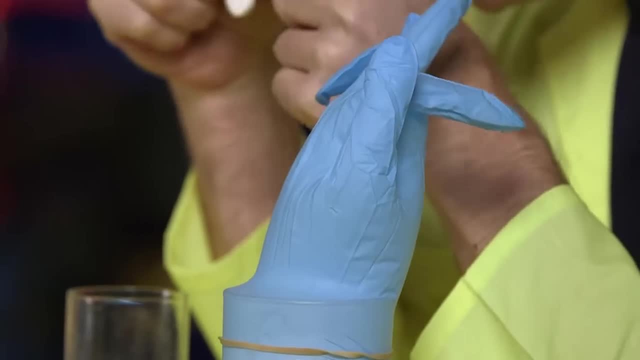 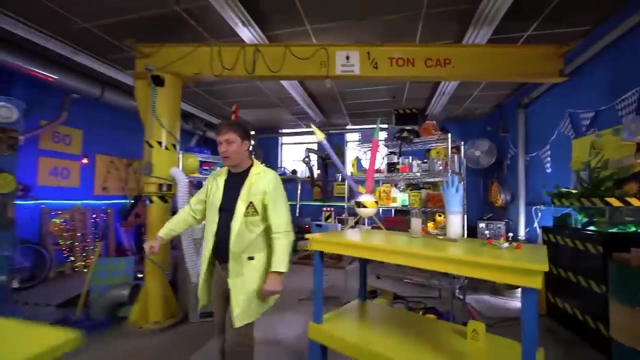 If we contain the reaction, the carbon dioxide gas builds up and creates pressure. High five for science. Alright, so let's look at our chemical powered rocket. What you need is one of these. This is a. This is a film canister. 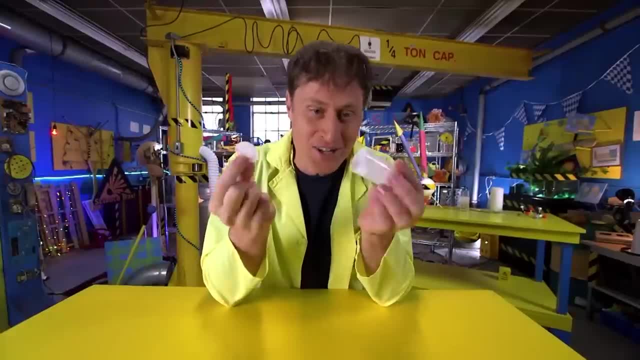 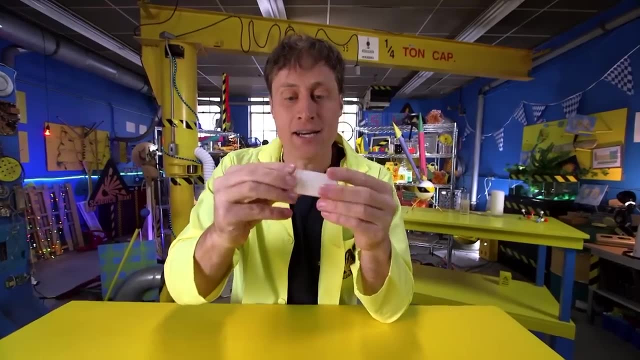 And ask your parents what that actually means, Because they're not used for holding film anymore. You can get these at craft stores, though, to hold paint or little things, But really all you need is a plastic container with a good lid that snaps on nice and tight and keeps the air in. 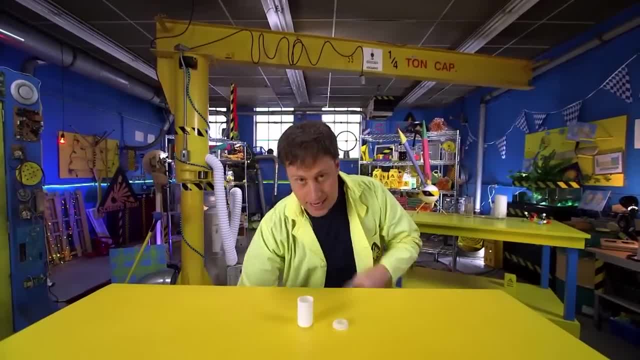 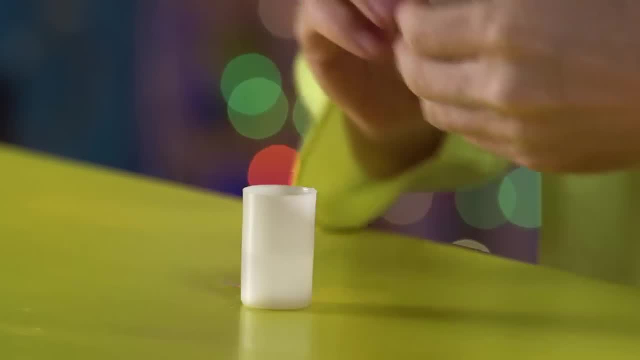 And then, of course, what you need are your antacid tablets and a little bit of water. So pour in some water and then put in your antacid tablet And snap the lid on, Flip it over and wait for the carbon dioxide gas to build up. 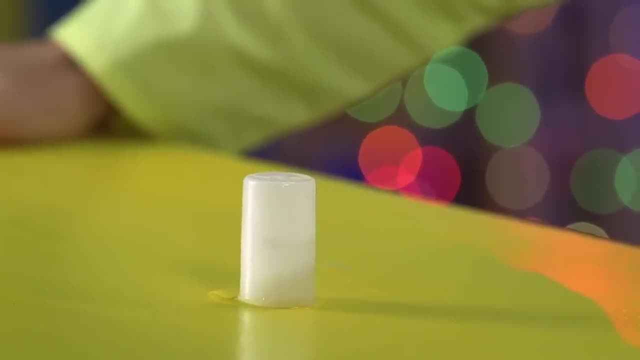 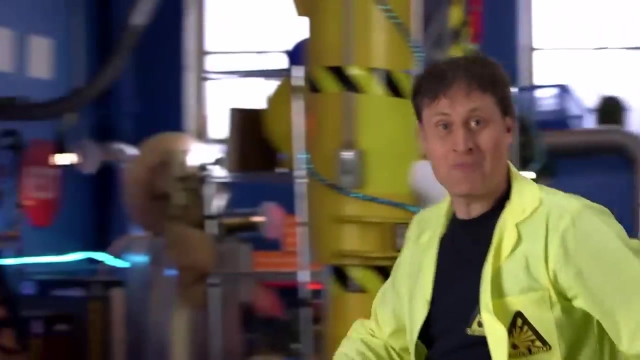 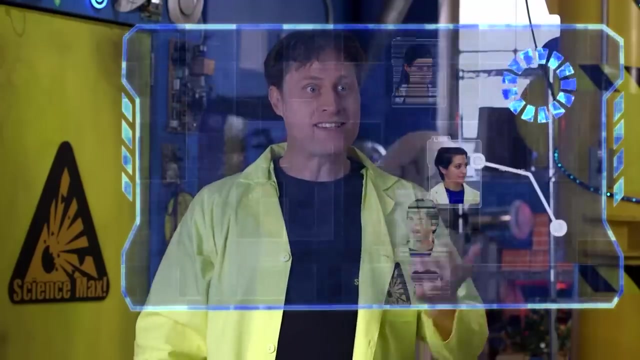 Which will build up pressure, Which will Launch your rocket. Ha ha. So there you go, A chemical powered rocket. Come on, Let's max it out. So first I need an expert to help me. Oh, Lisa from Logix Academy. 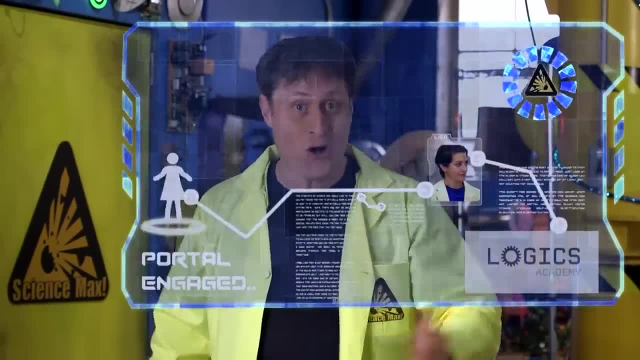 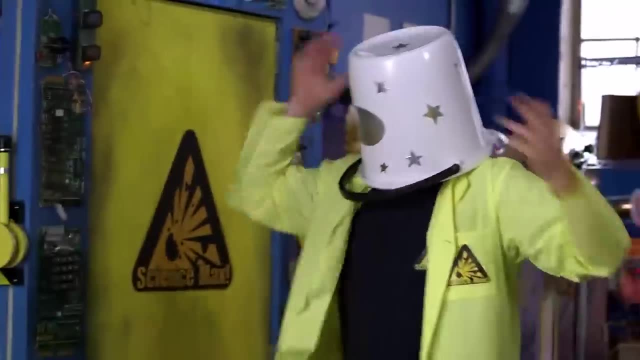 Of course, Logix Academy people have helped me launch all the rockets on Science Max. This is going to be great. Oh, I'm going to get my helmet first. Okay, let's launch. Let's launch some rockets, Let's go. 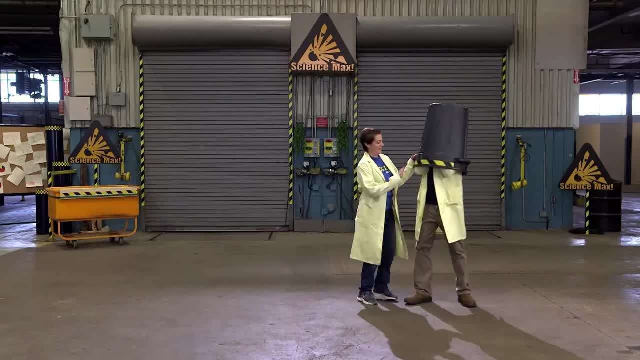 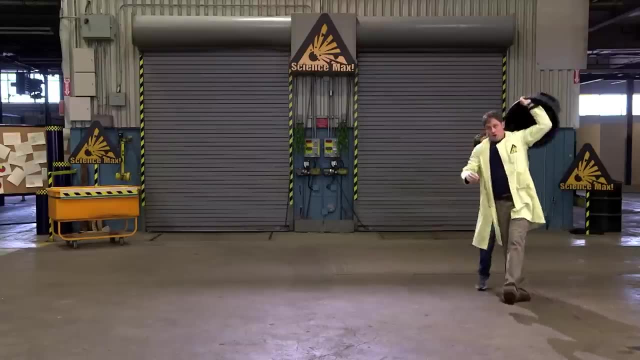 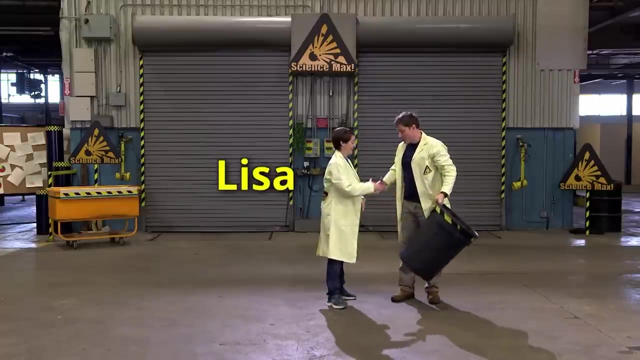 Whoa, Wow, it's really dark in this room. I can't see anything. Bill, Lisa, Bill, Lisa. What Bill? Where did this come from? I guess the portal's malfunctioning. Hey, Lisa, Hi. 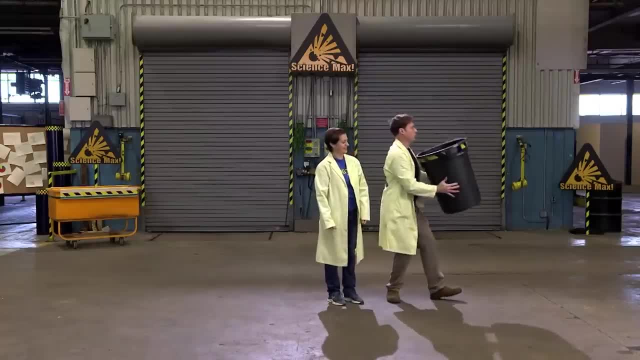 From Logix Academy. Great to have you here. Great to be here. Over there, We are here to max out the chemistry. rocket. Ooh, What is that? It's just a small plastic container, But when we put an antacid tablet in there and some water? 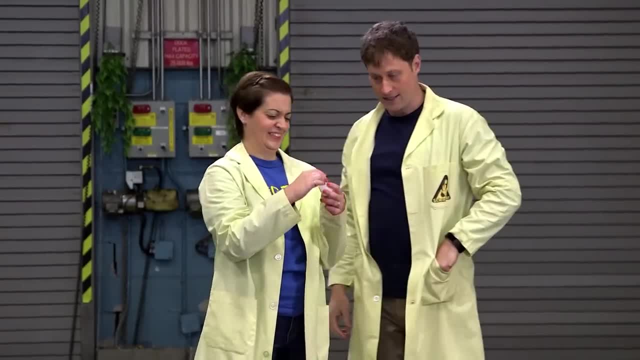 Ah, we get a chemical reaction. We get a chemical reaction, And so that's what creates the pressure, And then that pops the lid off and we get a little rocket Kaboom. But now we're going to max it out: Get a bigger container and more. 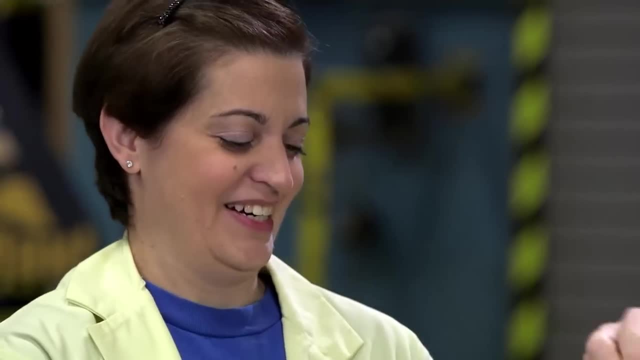 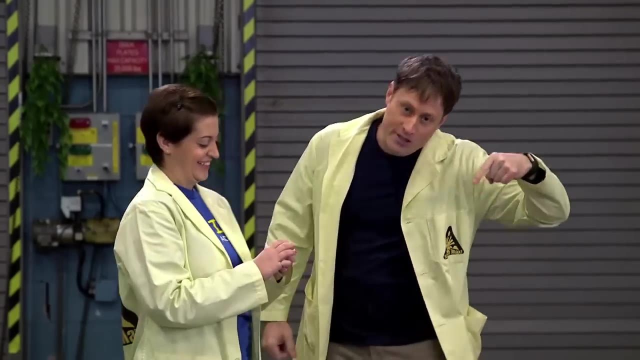 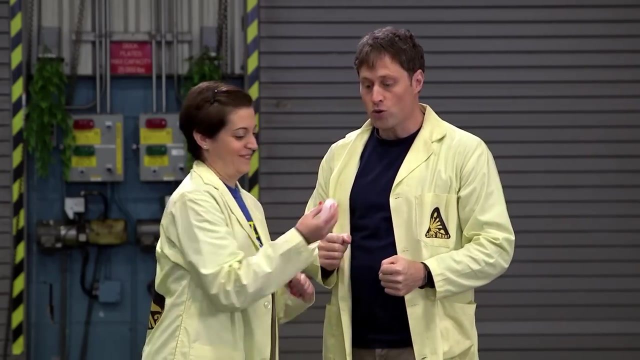 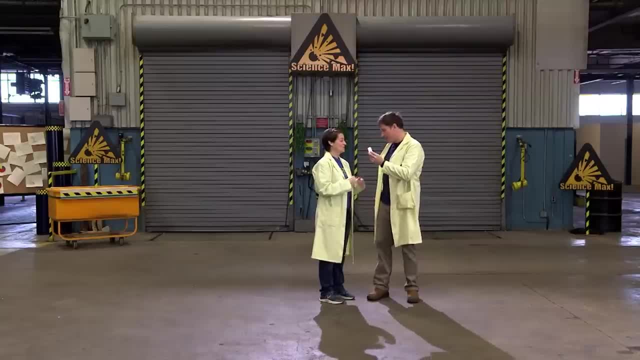 Exactly, Okay, great. So we just need a whole bunch of these And a whole bunch of, And a whole bunch of science antacid. Yeah Well, that's okay, I get them both in bulk. Come on, let's go put it together. 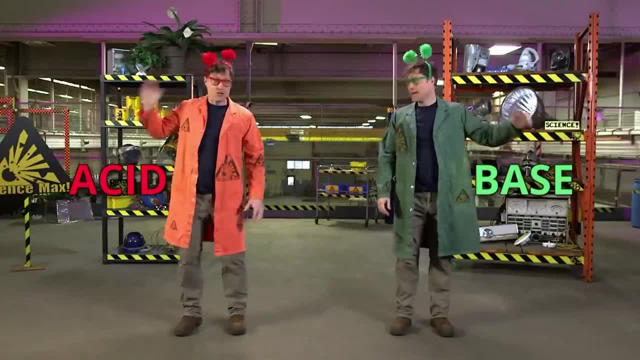 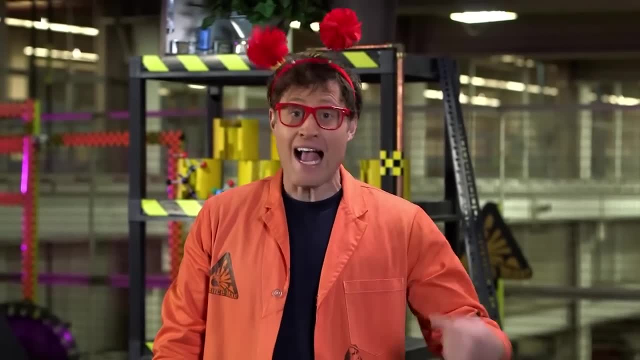 I'm an acid And I'm a base And we are enemies. Oh Well, we're not really enemies. Yes, Yeah, that's true. It's all about how we react chemically. You see, as an acid, I really want to give protons away. 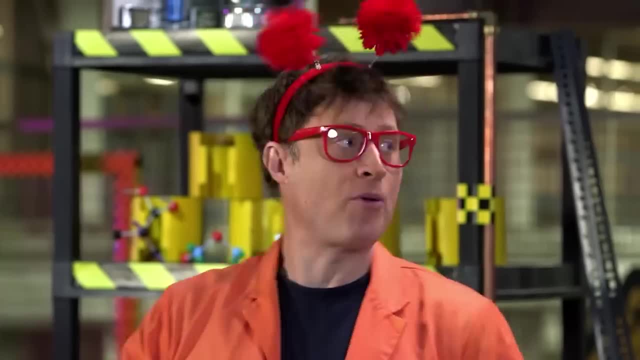 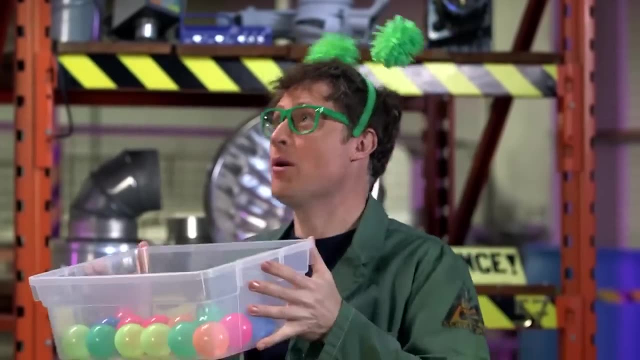 Protons: Who needs your protons? Get your protons here. Protons: I got more than I want, I don't need them anymore. And bases: we need protons. We'll do anything to get them. Protons: are you giving protons away? I'll take some. I'll take some protons. 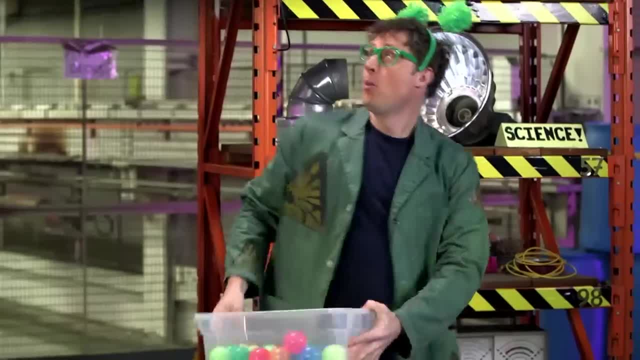 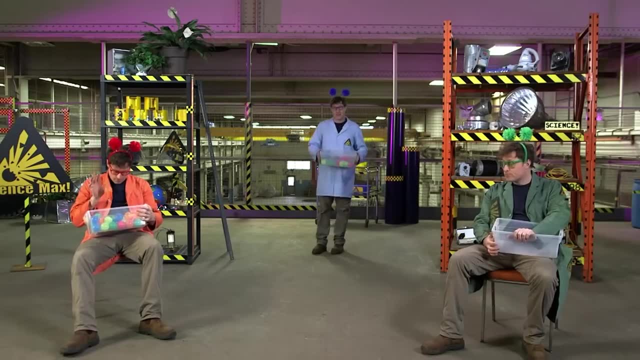 You'd think that when you get these two together you'd have some pretty great chemistry, But the truth is, when they're together, they often don't react. That is until water gets involved. Once you have water, acids and bases react. 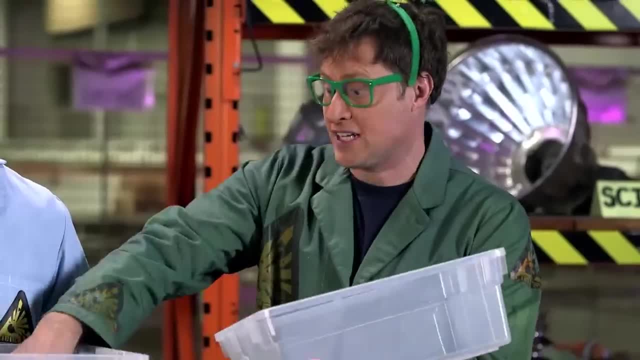 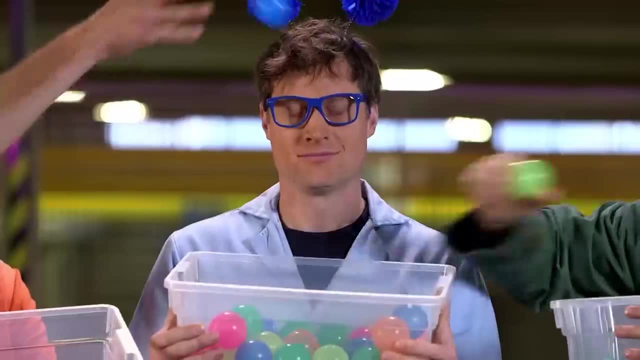 Here, take some protons. All your bases belong to us. Here you go, Take some protons. I don't need them anymore, I want more. I want more protons. Water is a solvent allowing the chemical reactions to take place. 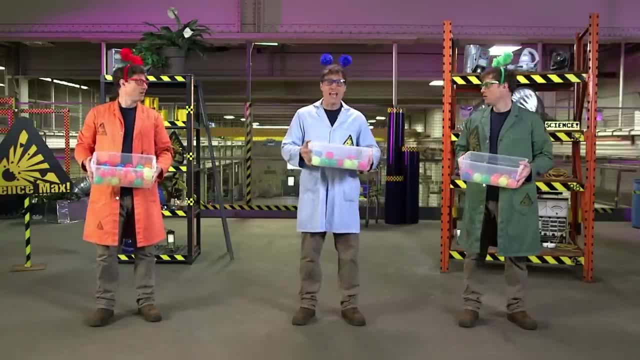 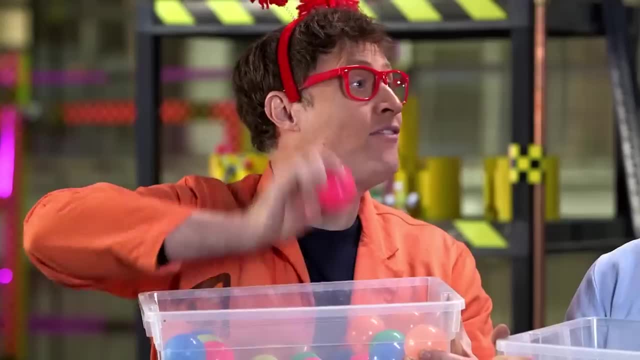 Depending on the strength of the acids and bases, that reaction can be mild. Would you like a proton? Oh, no, really, I couldn't Please. please take it. Oh well, thank you, That's very generous. Have another? Oh, perhaps, Maybe I will. 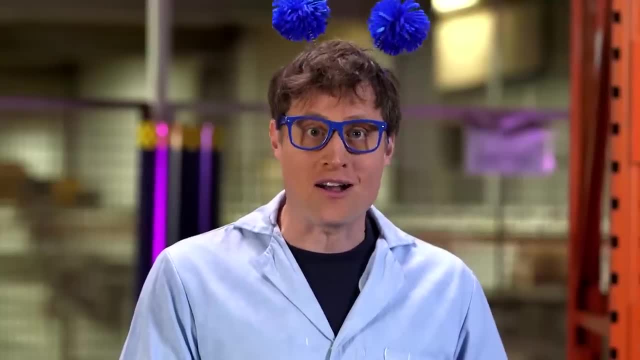 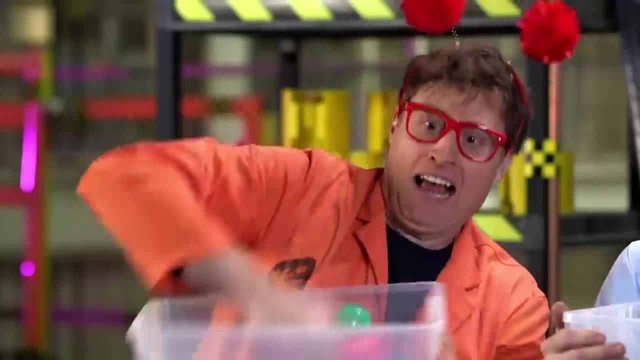 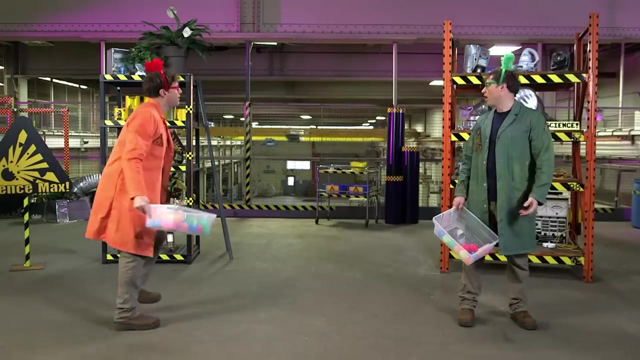 Here's one, Maybe just one. But if the acids and bases are strong, the chemical reaction can be really extreme. This is what's going on in the antacid tablet And why, without water, nothing happens. Oh, water, Water. 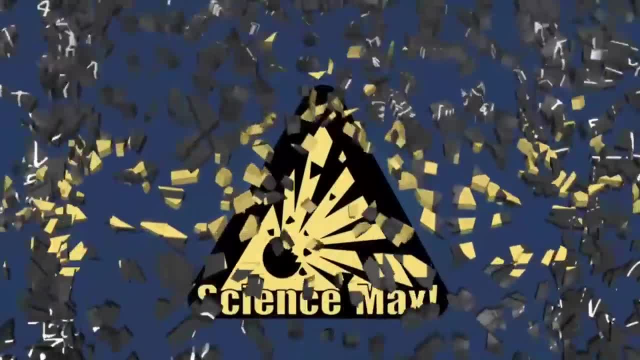 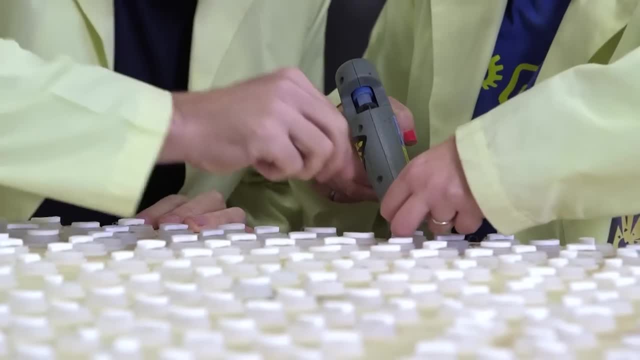 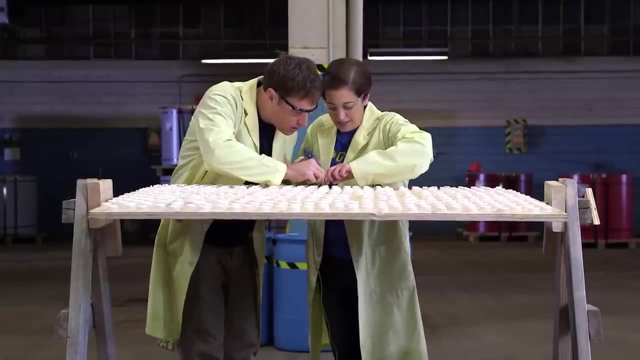 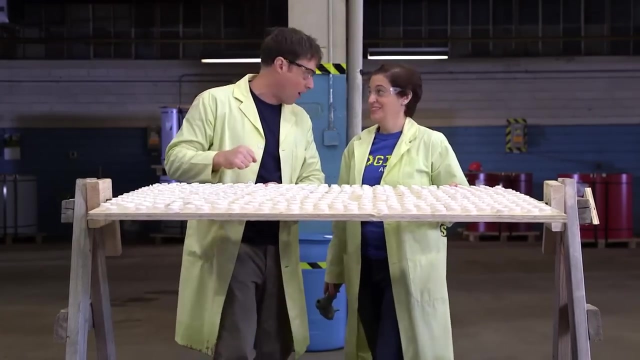 Come on, What'd you do? That's the last one. Lisa and I are maxing out our chemical-powered rocket, not by making it bigger, but by making more of them. How many more? Four hundred caps, all glued down. Four hundred antacid tablets, or part of all glued down? 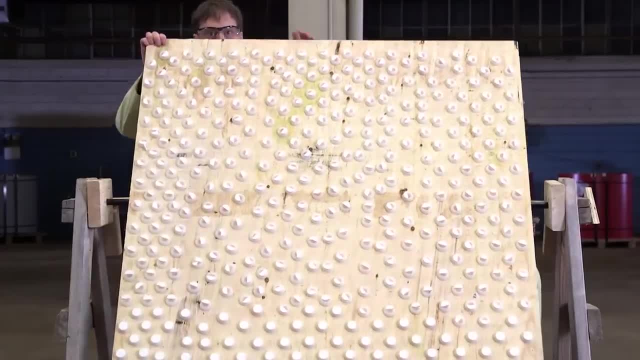 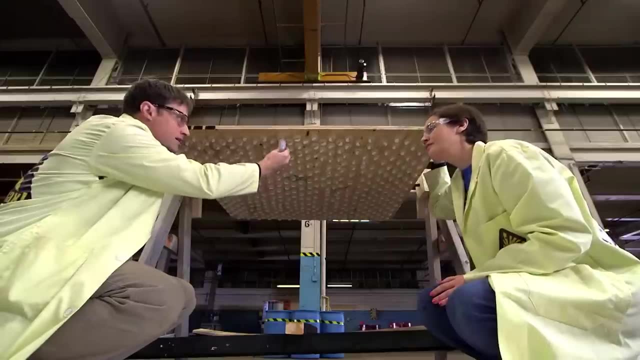 And they're glued on this fancy-pantsy spinning surface. So we rotate this part upside down, We fill each container with a little water and snap it on underneath. This way the antacid tablets will not get stuck. The tablet and the water don't mix until we flip it back over. 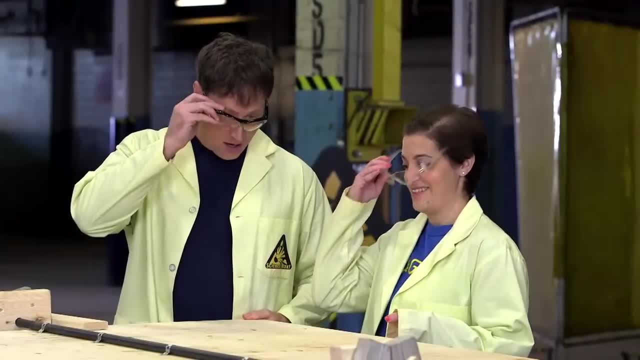 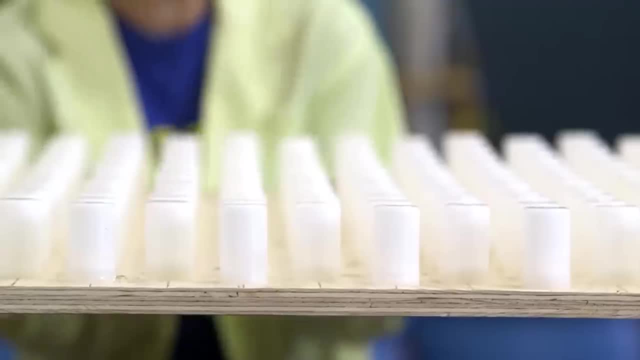 It also allows us time to snap them all on. Okay, ready, Ready, All right, Four hundred containers, Here we go, Let's do it. Once we flip the board back over, the reaction started taking place, building up carbon dioxide gas and increasing the pressure, until 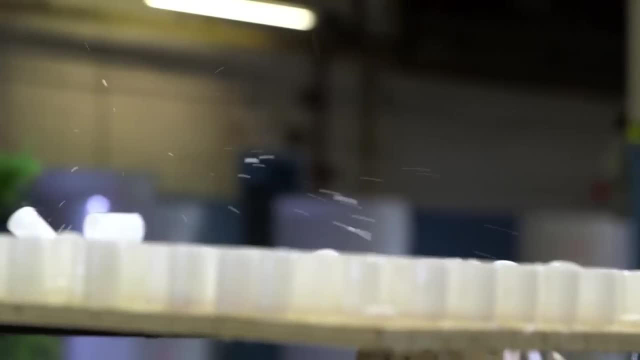 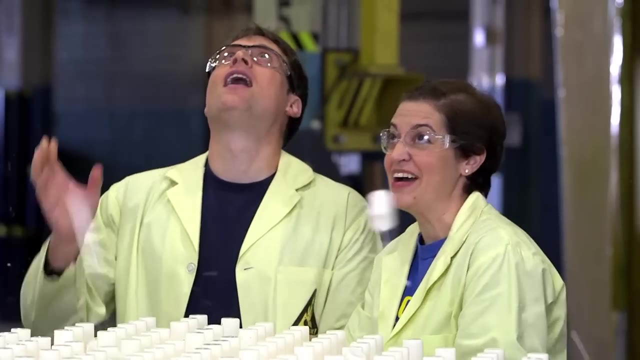 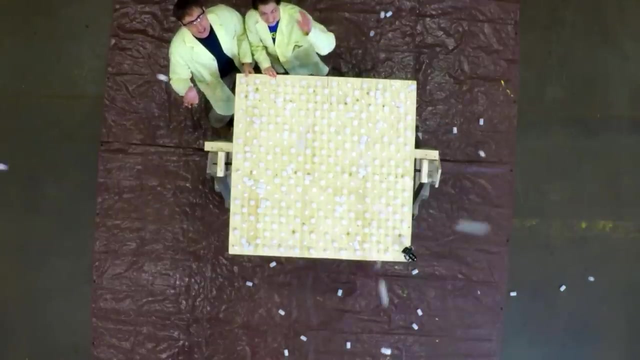 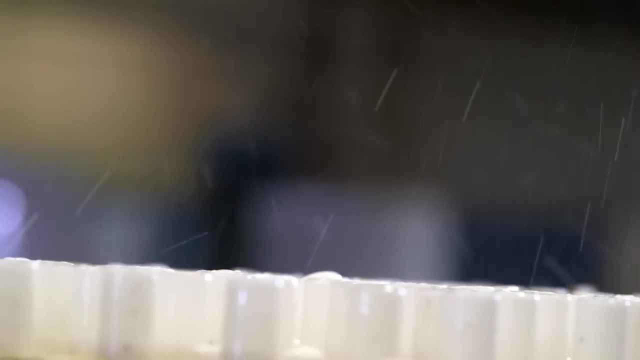 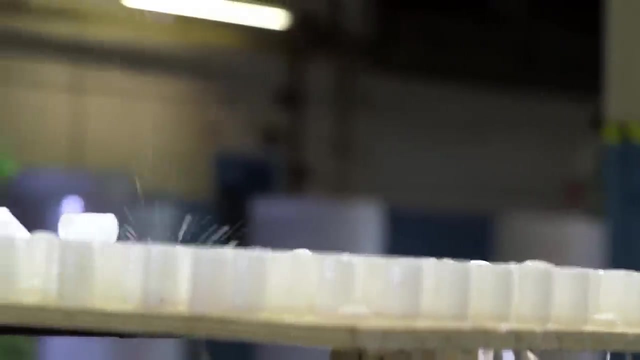 Whoa, Whoa Twenty seconds. Oh yeah, Oh yeah, It's a good life if you catch one. Wow, that one was really tight. Awesome, That totally was great. Okay, so high fives on that. 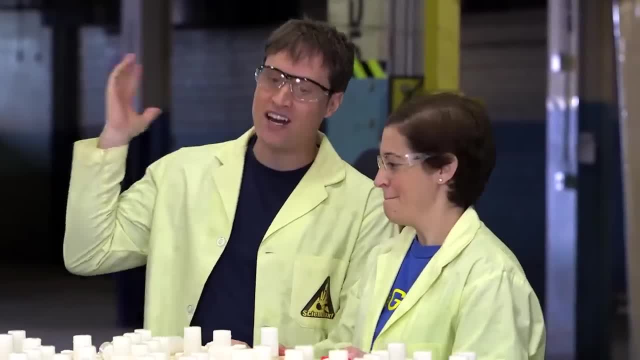 That worked spectacularly. That was awesome. So we've done this. Let's go bigger. Let's go bigger. Okay, so let's go and we'll clean this up afterwards. Okay, let it go. Whoa, whoa. 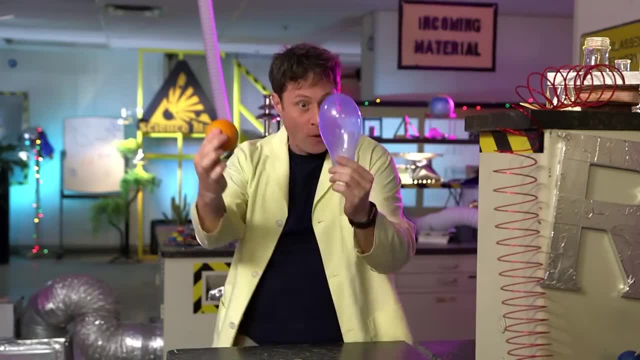 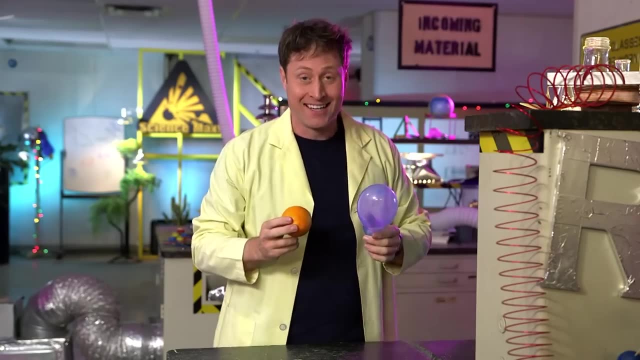 This is a balloon and this is an orange. When you put them together, a chemical reaction happens. Ah, how'd you go in there for a minute, didn't I Hit? no, no, all right, Well, you can actually do a chemical reaction. 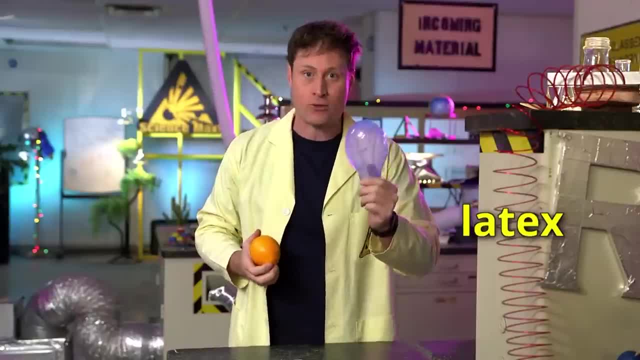 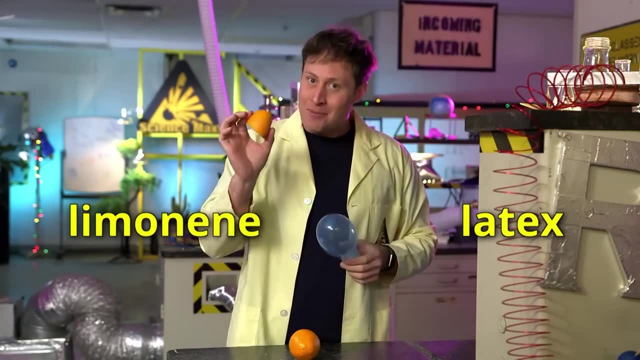 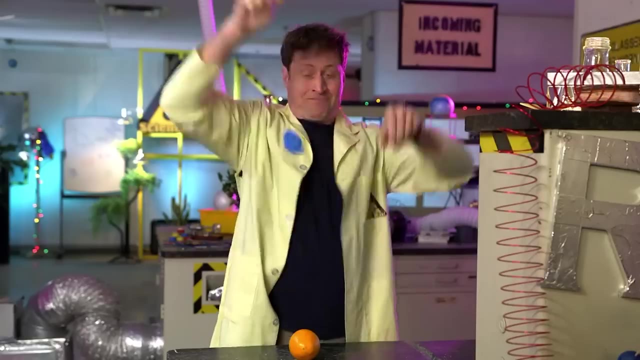 between a balloon and an orange. You see, balloons are made of latex, which is a kind of polymer that's very, very stretchy, and orange peels contain a chemical called limonene. Limonene breaks down latex. So we have three questions. 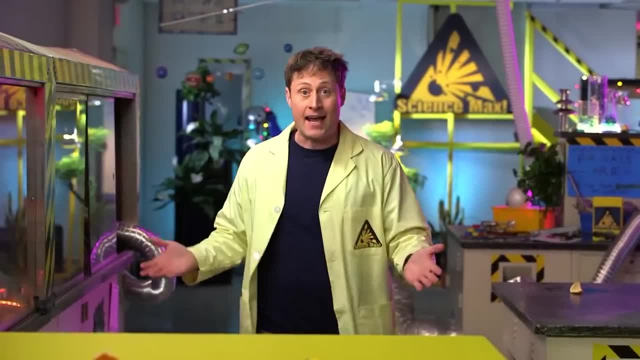 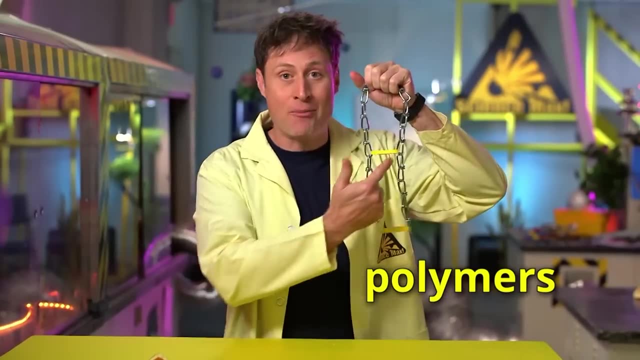 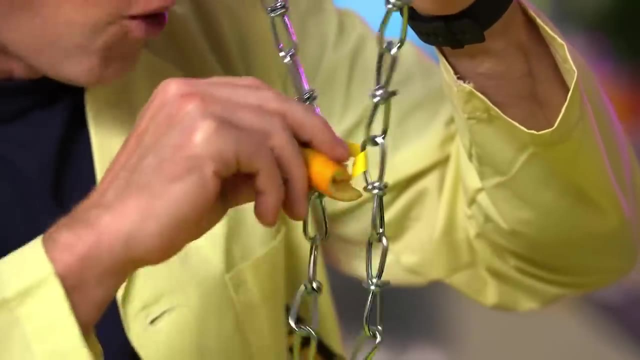 The first is: why does this happen? Well, like I said, it's all chemistry. You see, balloons are made of polymers, chains of molecules held together by chemical bonds. A limonene molecule attacks those bonds. Om nom, nom, nom, om, nom, nom, om, nom nom nom. 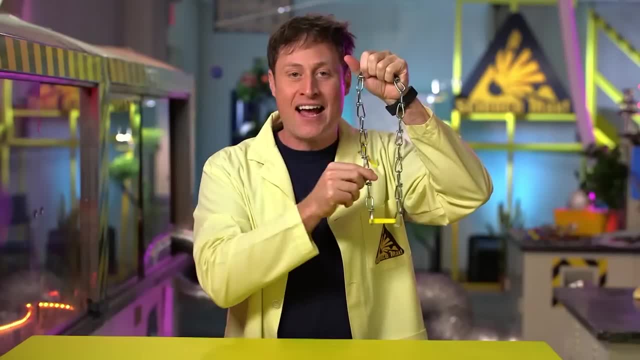 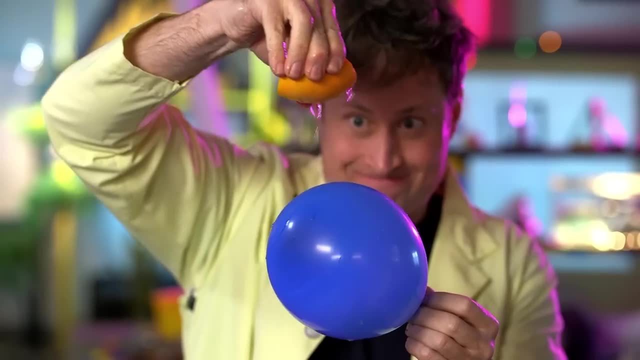 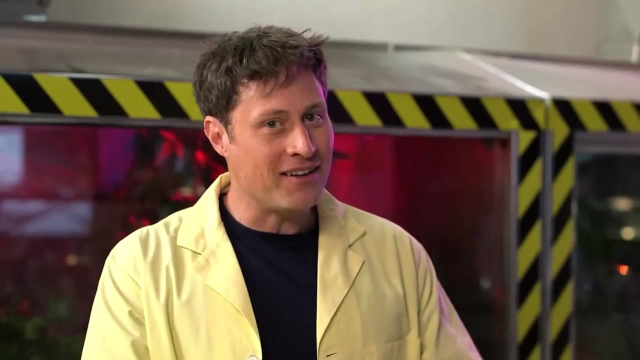 om nom nom. delicious- and breaks it. That separates the polymers and that pops the balloon. But remember it only works with natural latex, So maybe let's make sure you're using natural latex balloons. Second question: why do they call it limonene? 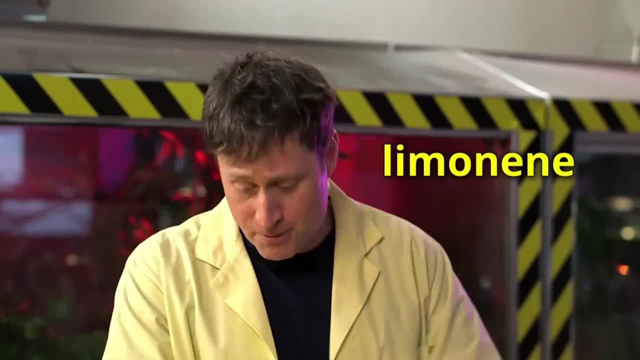 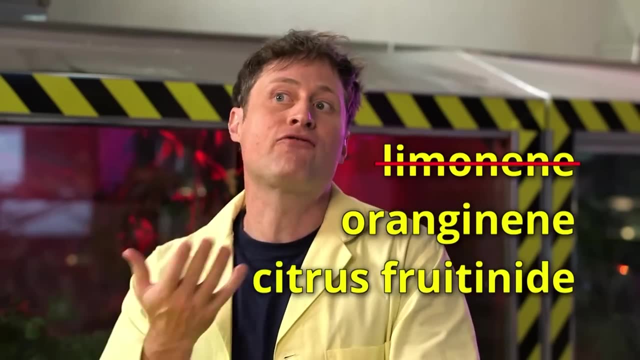 when it's in orange peels. I mean, yes, it's in lime peels and lemon peels, but the chemical itself smells like oranges. They should call it orangenine or citrus frutenide or anyway. Third question: should we max it out? 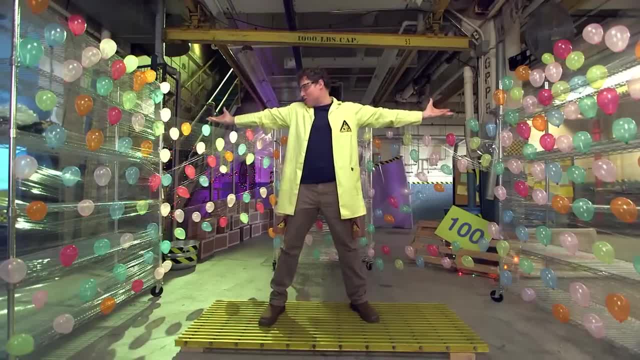 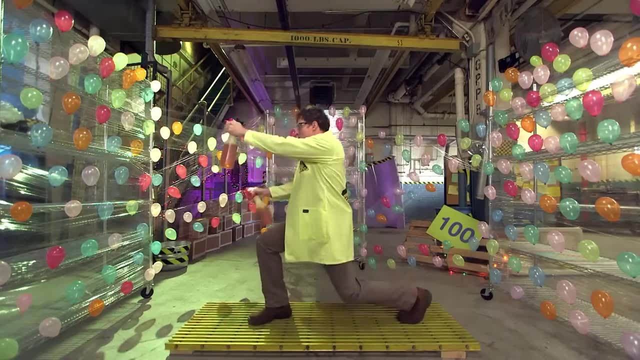 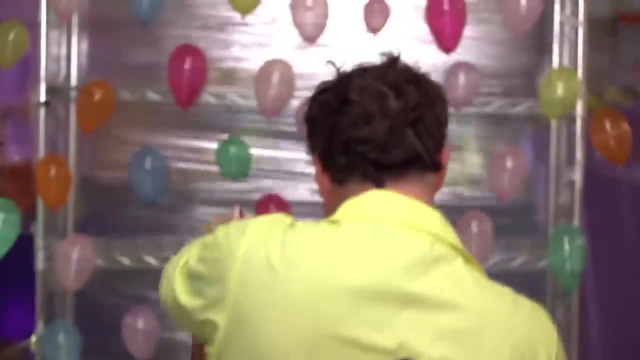 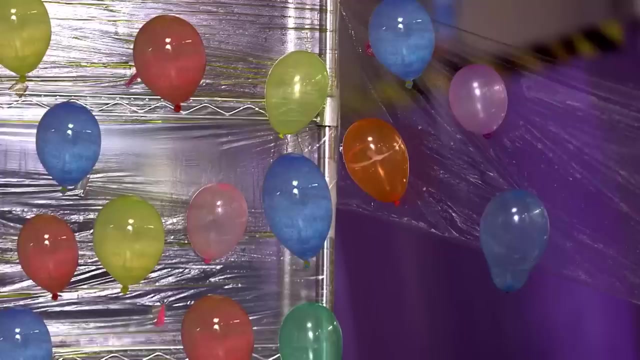 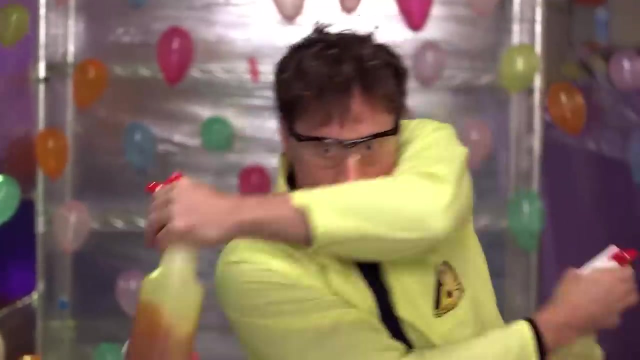 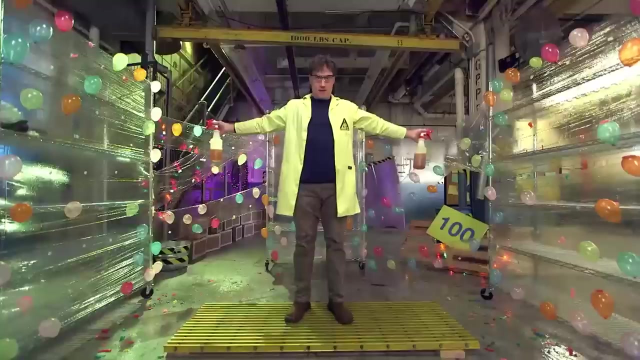 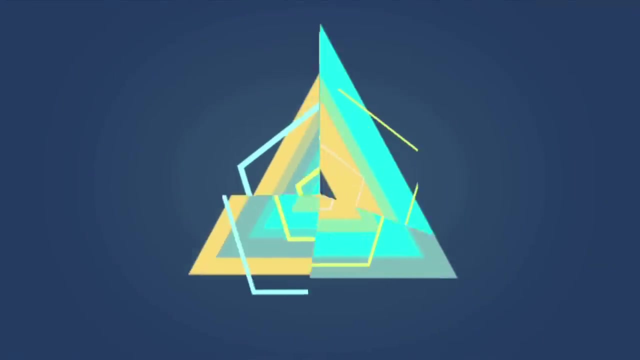 Of course we should come on. 200 balloons versus two bottles of lime, Two bottles of limonene- Ready Go. the first attempt to max out our chemical rocket was 400 plastic containers. Oh yeah, That worked well, but now it's time to make the container larger. 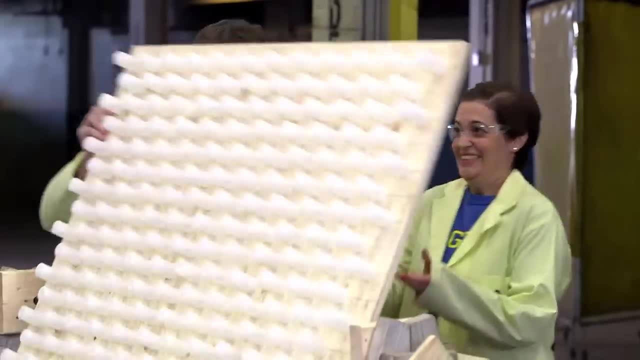 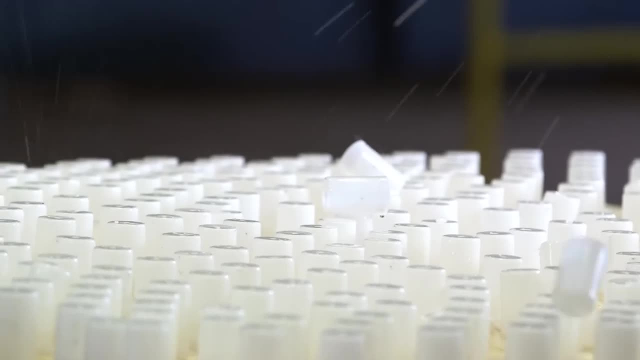 Whoa Giant maxed out chemistry rocket canister- Oh yeah. That worked well, but now it's time to make the container larger. Whoa Giant maxed out chemistry rocket canister- Oh yeah. 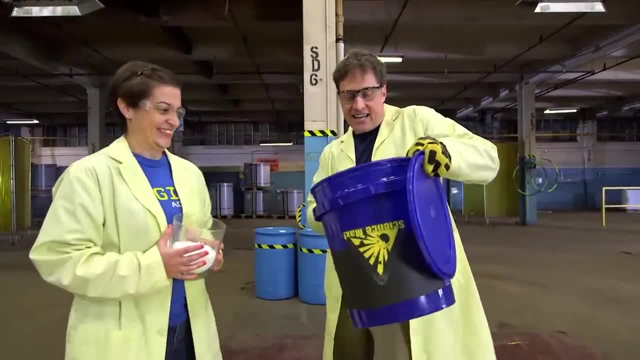 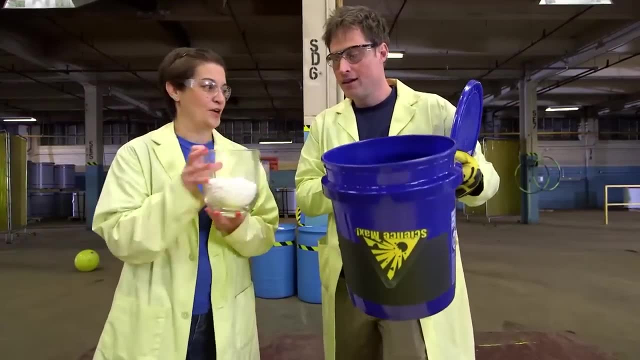 Oh yeah, Oh yeah. I have a big plastic container with a groovy lid that sits there on airtight, which is great, And I have a giant jar of antacid- How many? It was like 60 antacid tablets or something. 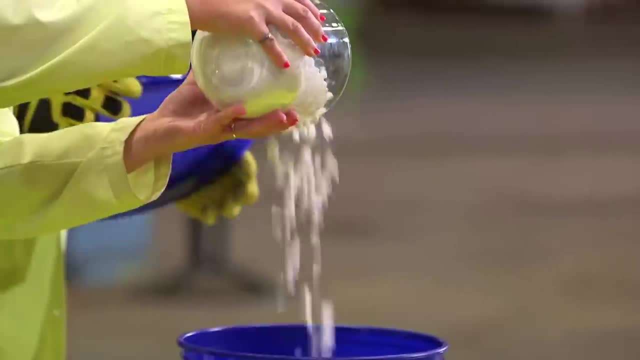 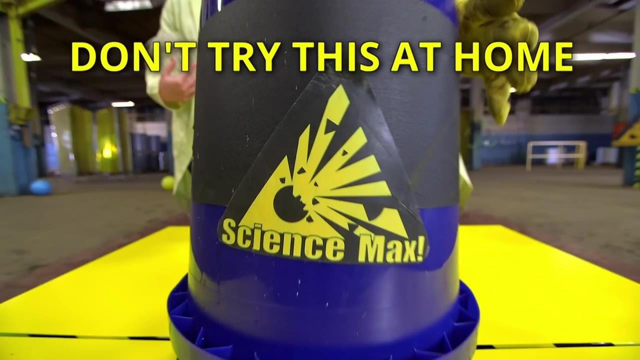 At least This works exactly the same as our smaller containers. We dump the antacid in, seal the lid airtight, then flip it over. And now would be a good time to mention not to try this at home. Whoa. 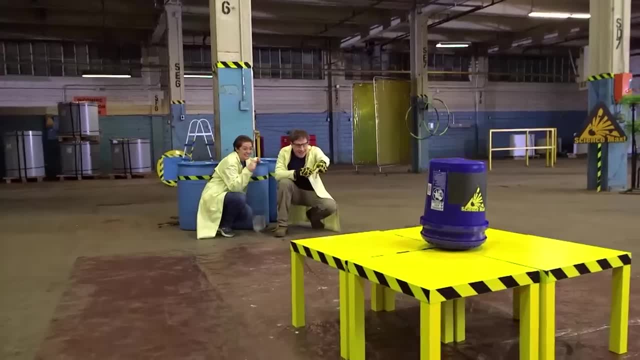 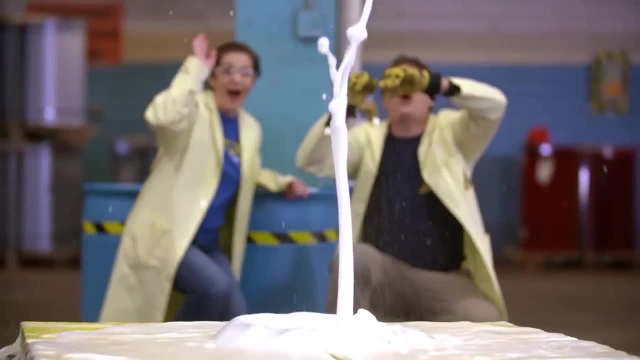 Okay, Oh, it's not gonna take long. Oh my God, Oh my God, Okay, here we go Splash. Hey, Look at that. Oh, Oh, Alright. So that was the canister version. Now we need to be pot bottle version, the rocket version. 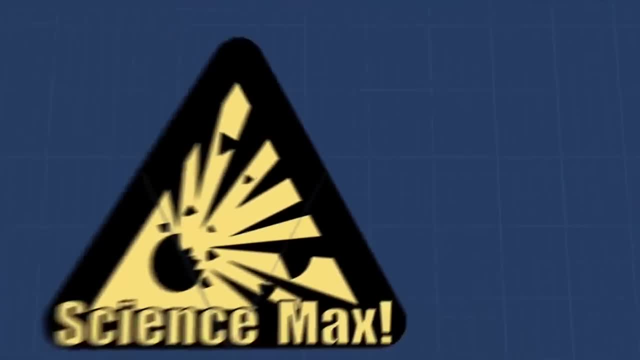 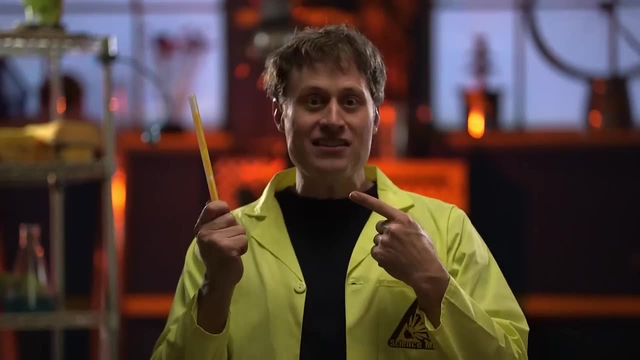 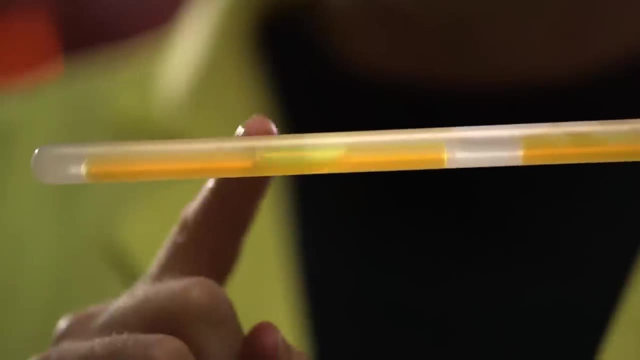 Yes, yes, Okay, let's go make that. Let's do it, Okay. Mitty Maxx, This is a light stick. It creates light using a chemical reaction. There is a liquid chemical inside and also a glass container that holds another chemical. 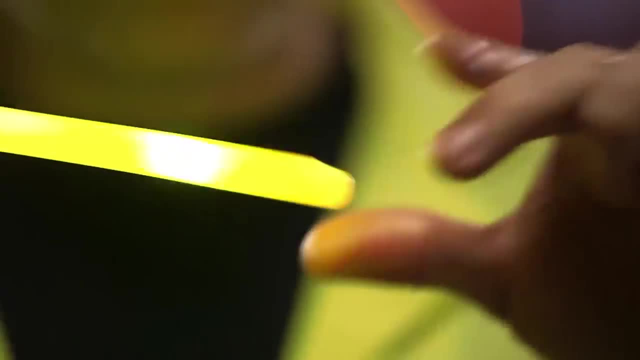 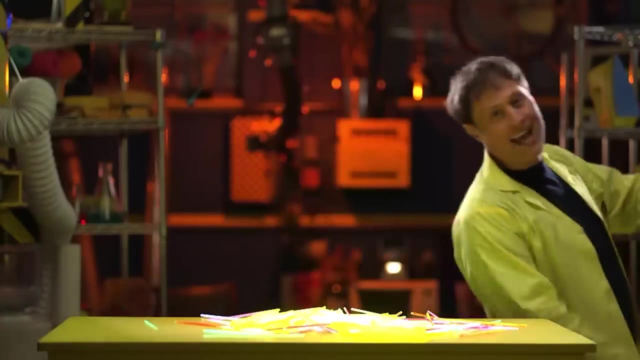 When you bend a light stick, you break open the container and the two chemicals mix, creating light. There you go: Light sticks, Chemical reaction And yes, of course we're gonna max it out. This is a whole bunch of the two chemicals. 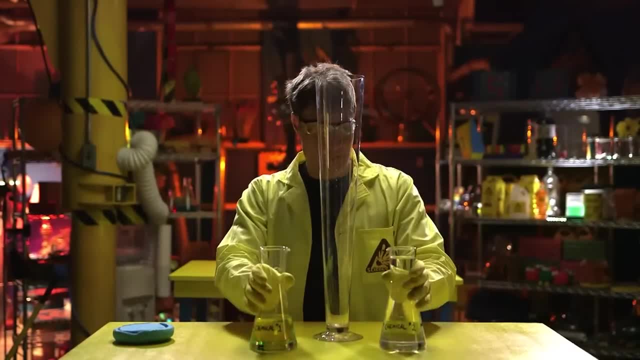 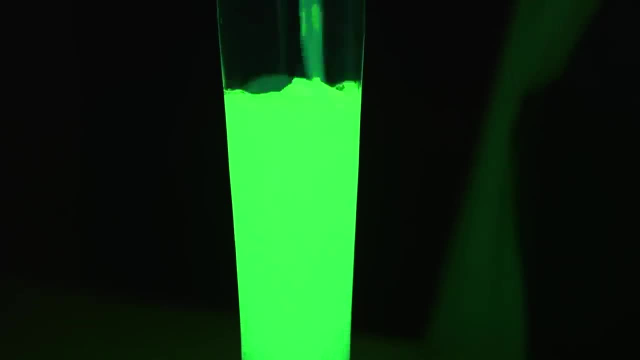 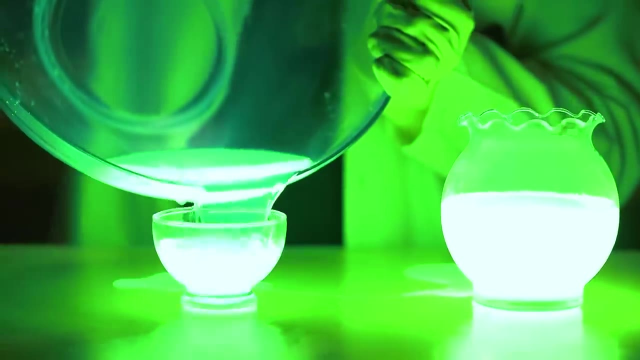 in a light stick. Let's max it out. So how does a chemical reaction produce light? Well, a lot of chemical reactions produce energy. You might think of a chemical reaction producing heat. Well, heat is a kind of energy. This chemical reaction also produces energy. 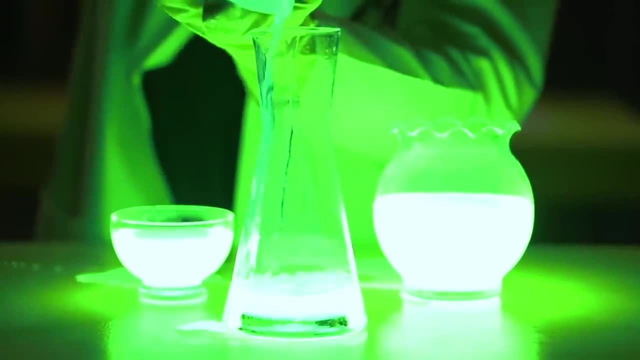 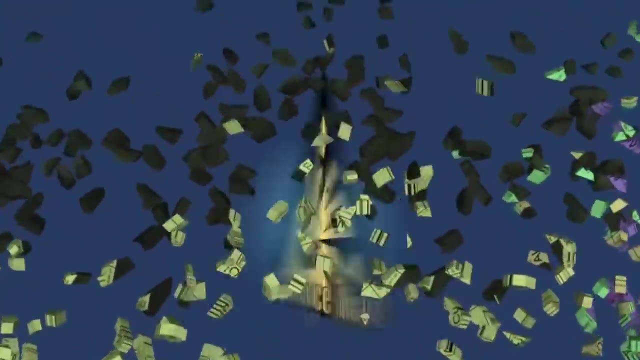 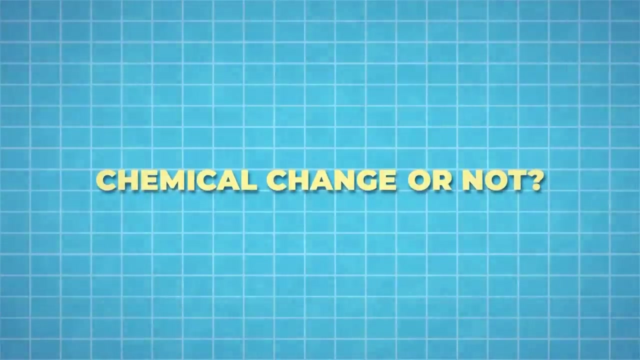 just energy in the form of light. It's just a different kind of energy. Whoa Maxed out light stick And now for a Science Max quiz: Chemical change or not? What's a chemical change? Well, let's demonstrate. 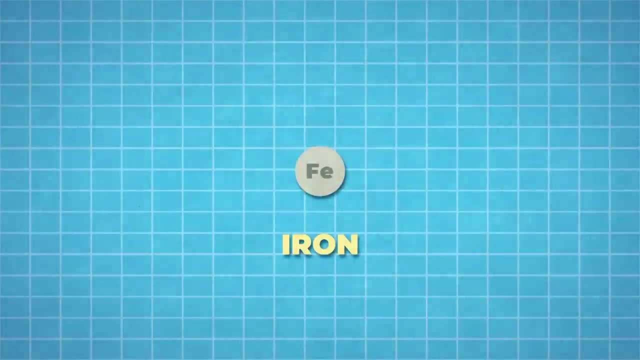 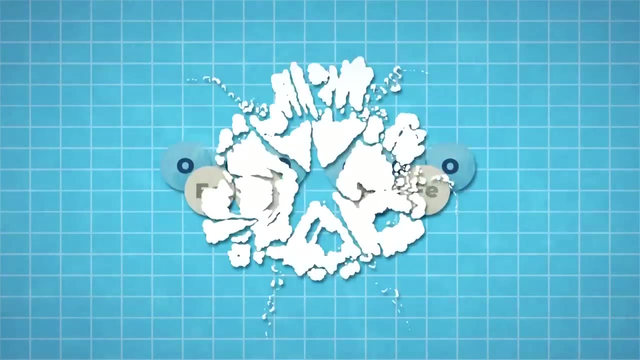 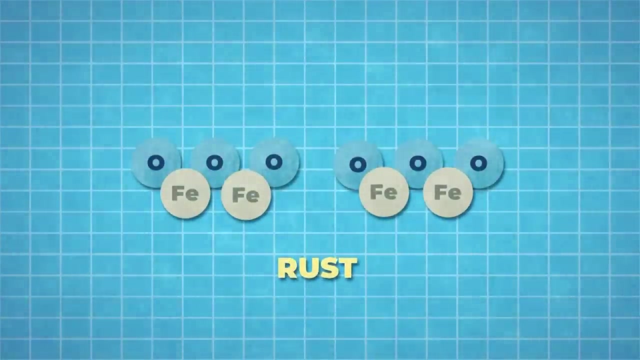 Look at this: It's a happy little molecule of iron. And here's another molecule of oxygen. If they were to have a chemical change, they would react and form different molecules. Look, it's a molecule of rust. Rust is a different chemical than either iron or oxygen. 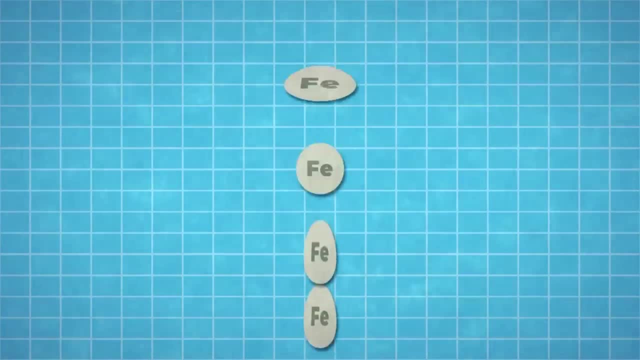 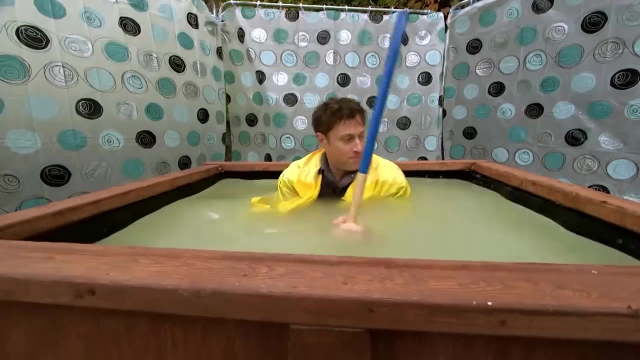 It's a chemical change. Now, if these molecules mixed and did not change, then it's not a chemical change, It's a physical change. Sometimes it's hard to tell if it's a chemical change just by looking, But asking what kind of change it is leads to good science. 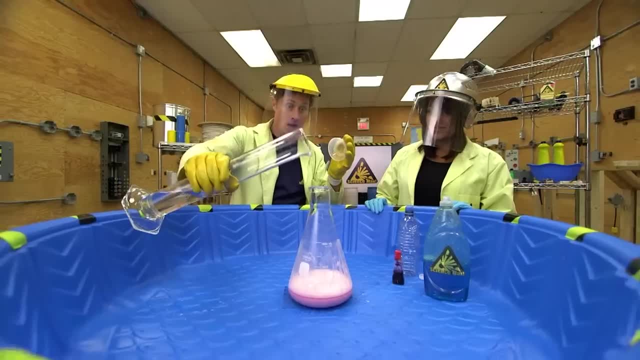 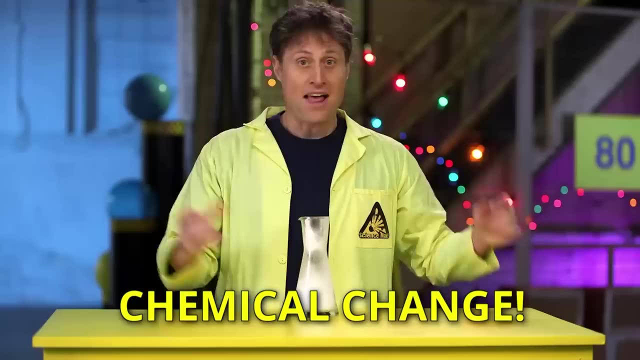 So let's look at some examples: Vinegar and baking soda. Is it a chemical change? Yes, Vinegar and baking soda react to form different chemicals: Sodium acetate, that's the white stuff that's left over, and carbon dioxide, which makes the bubbles. 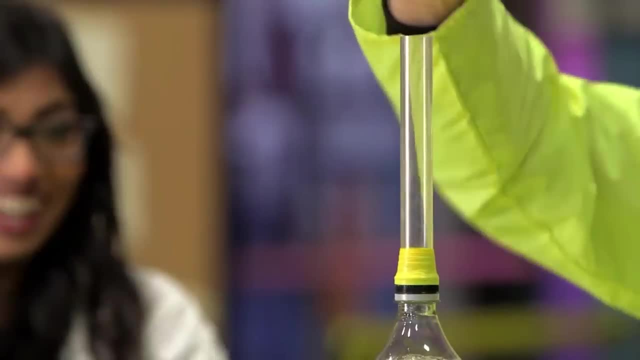 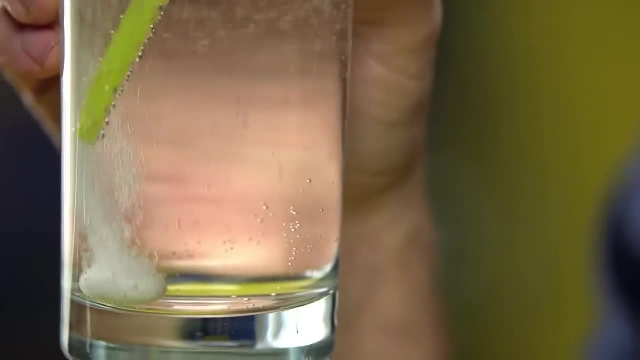 How about a nucleation fountain with diet cola and mints? Ha ha, A lot of people think that's a chemical change, but it's not. The mints cause carbonation, the bubbles to escape faster. But it's not. 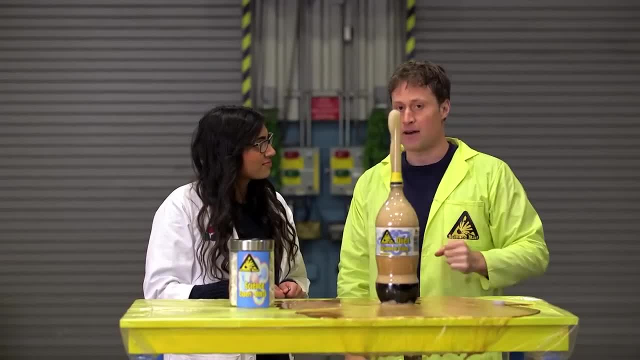 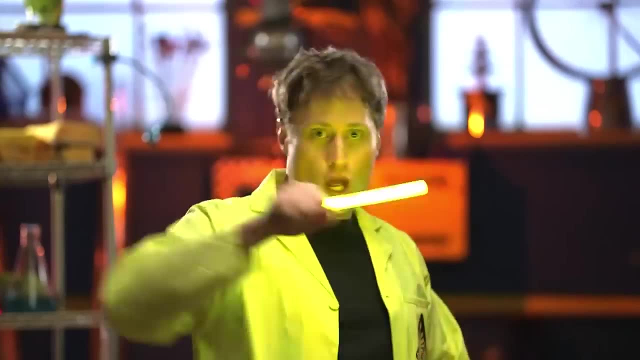 But in the end you still have cola and mints, No new chemicals And without the carbonation nothing happens. So it's a physical change. Take a guess at this one: Glow stick chemicals. Well, producing light or heat is usually a sign of. 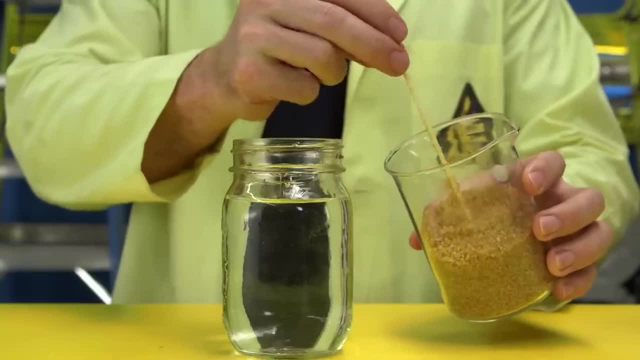 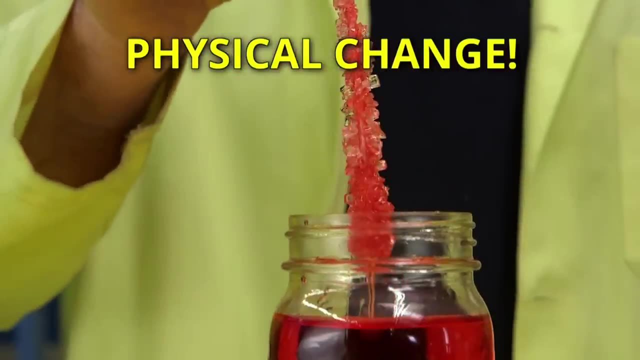 a chemical change. How about mixing sugar and water to make a sugar pop? That's a physical change. You start with sugar and water, you mix them and when you have a sugar pop, what chemicals are you left with? Well, sugar and water. 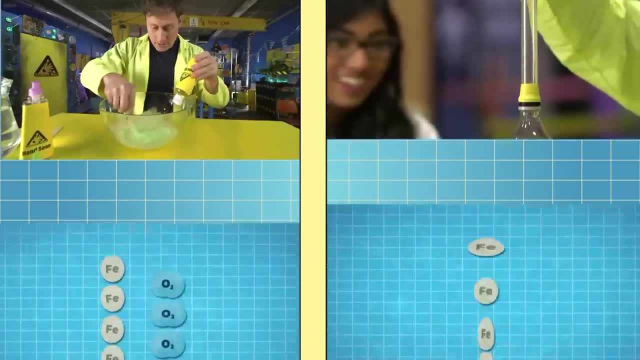 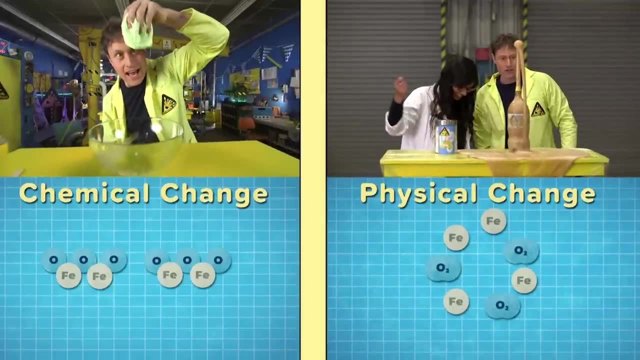 So no chemical change. It can be hard to tell sometimes, But whenever two things mix, think to yourself if it's a chemical change or a physical change. And now you know it's either one or the other, And that's the first step to good science. 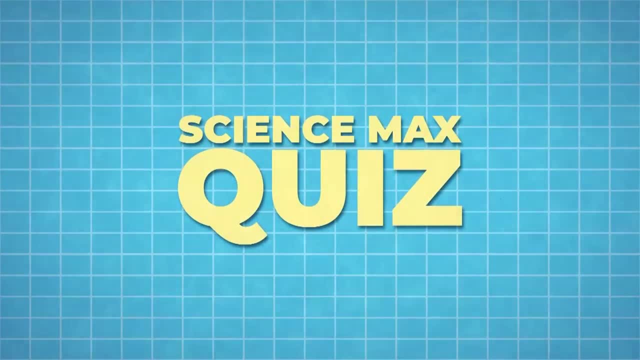 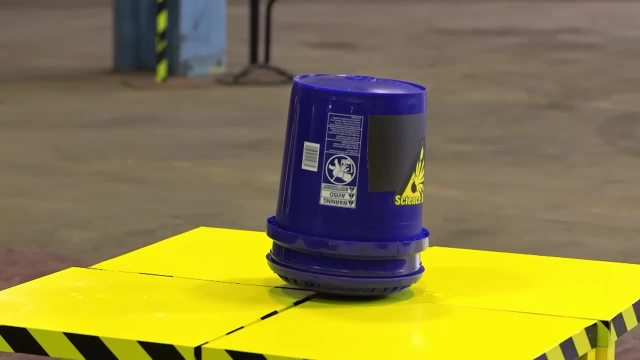 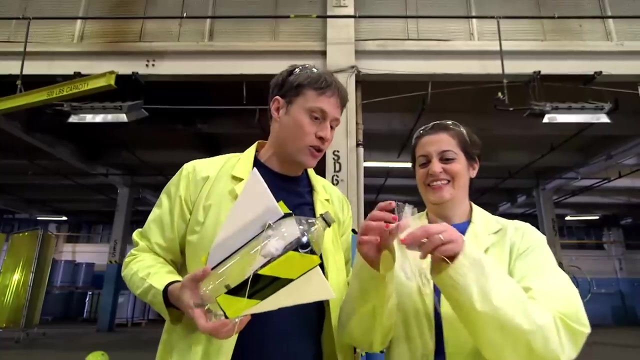 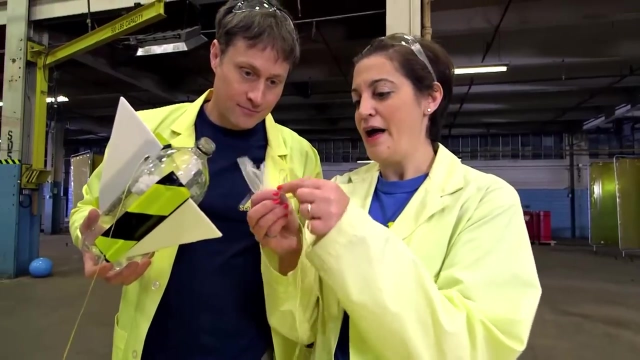 Thanks for playing our Science Max quiz. Our maxed-out rocket worked great. Whoa Ha ha ha. Now to make it look more like a rocket. so we have a mesh bag here to put the antacid in Right, And we have some paper clips attached to it. 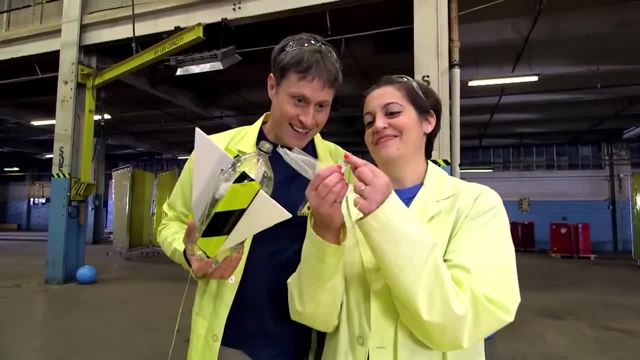 And what are the paper clips for? Well, Phil, we have a magnet, Ah, And so the magnet sticks to the paper clip, And so that's what we have here. You see, the bag is full of the antacid tablets. 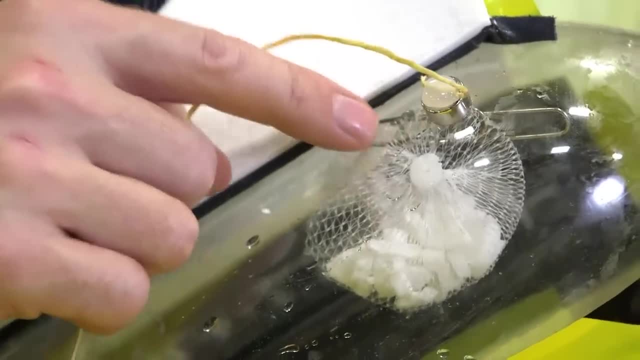 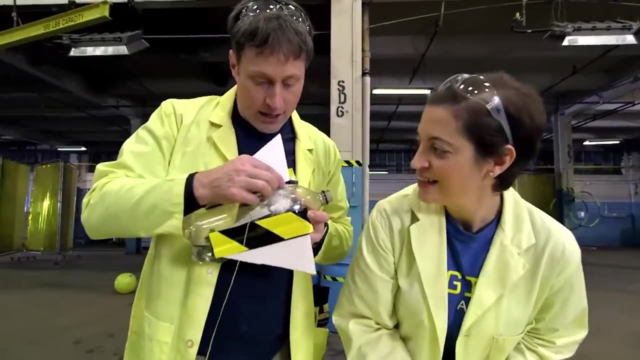 which we put through the mouth of the bottle, And the magnet is holding the paper clips on the other side of the plastic so we can sort of move it along, So we can start with the bag over here where the water's down there. 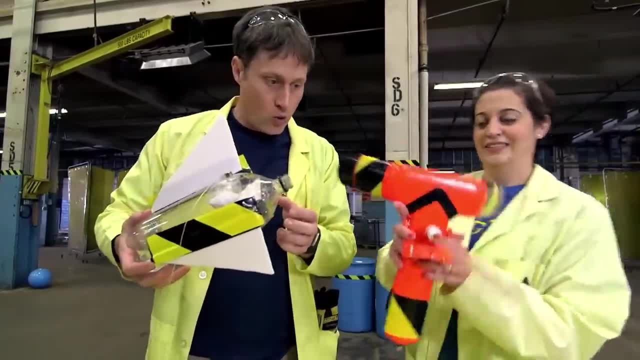 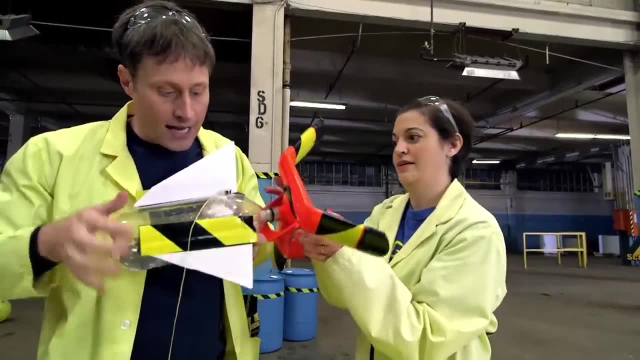 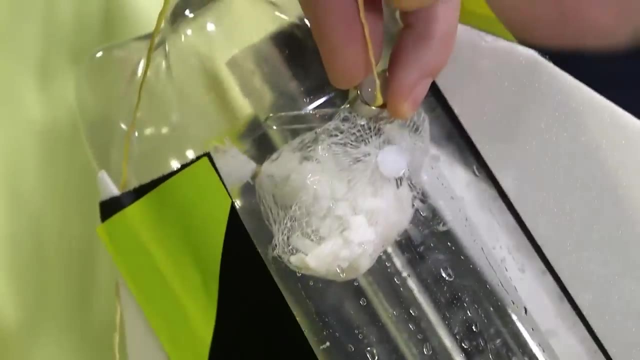 But now we attach the launcher, like. so. All this effort is to keep the reaction from happening until the bottle's on the launcher and we're ready to go. And then, as we pull the bottle over, we bring the bag up this side, And there the water and the antacid have never touched. 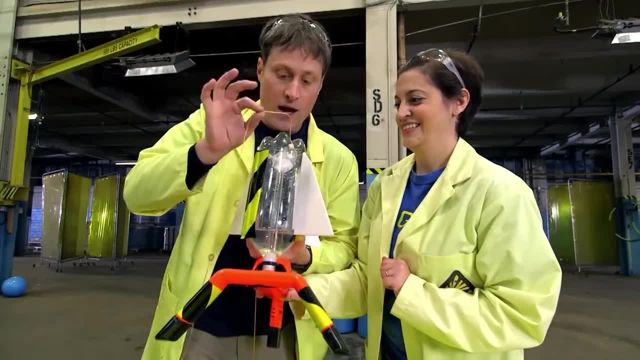 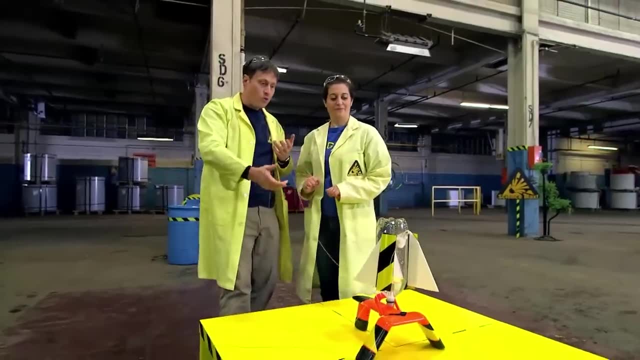 No reaction. All you need to do now is just we pull this magnet away and the bag will fall into the water, And then we will have the launcher down here And we pull the release and the rocket will go. We add some weight to the launcher. 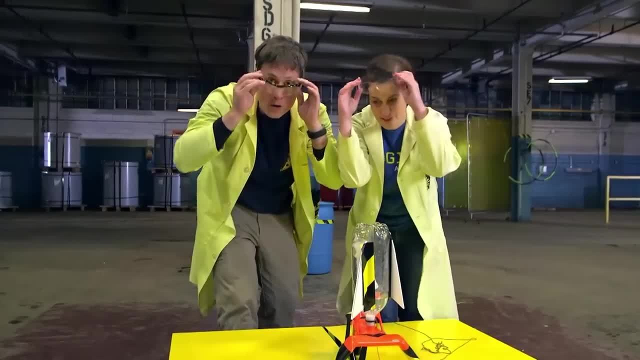 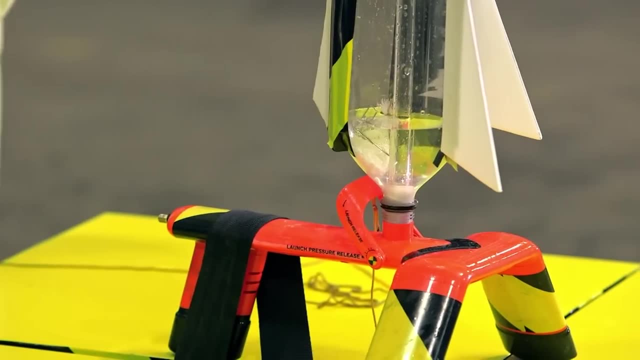 to help keep it in place. OK, right, wait, Glasses, Safety first. OK, ready. And then we pull the string with the magnet That drops the bag of antacid tablets in the water and starts the chemical reaction, Because we have a latch holding the bottle down. 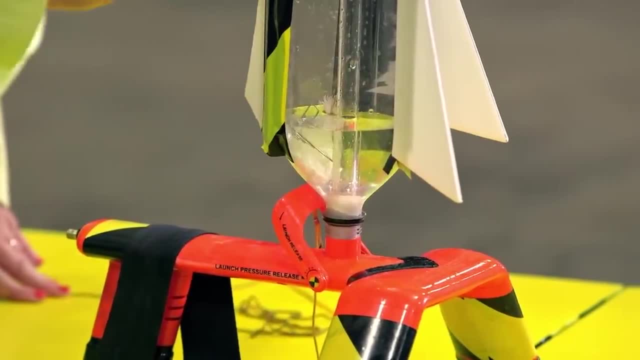 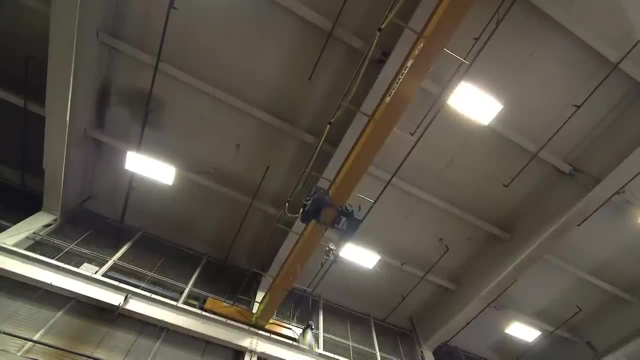 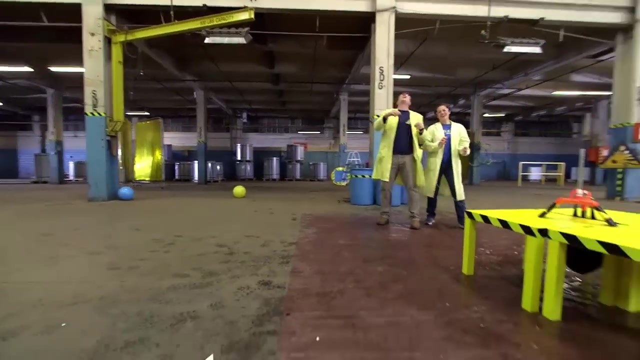 we can wait until the chemical reaction happens fully And there's a lot of gas pressure in the rocket before Three, two, one run Woo, Oh, That worked. Yeah, I hit the ceiling. I think we need to do this outside. 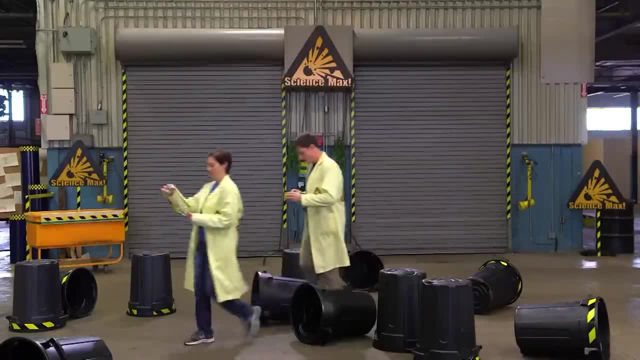 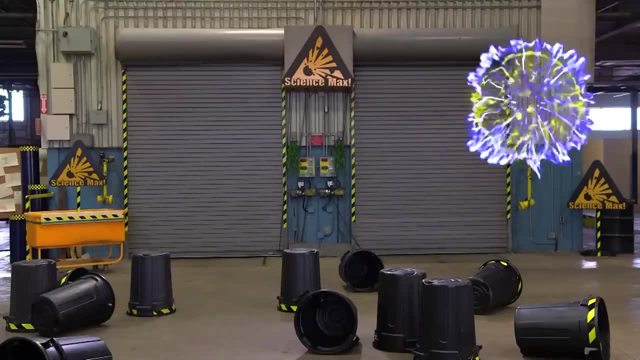 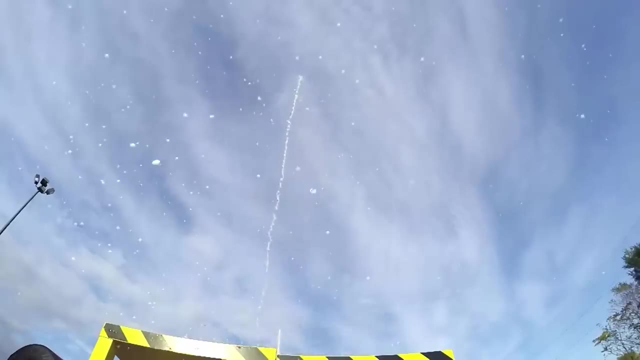 Yeah, I think we definitely have to do it outside. All right, totally great, Weird. Anyway, I was saying we should put three or four of these Three, two, one, go Woo, Let's go. There it is. 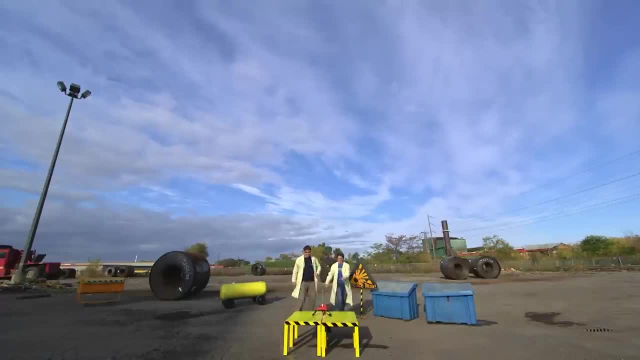 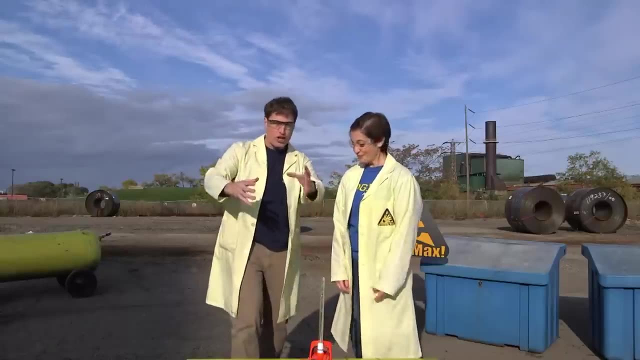 Oh my gosh. Yeah, We tried it outside and it worked great. The only thing left was to max it out even more. So larger chamber, Yep, more antacid, More antacid, more air, more water, Absolutely. 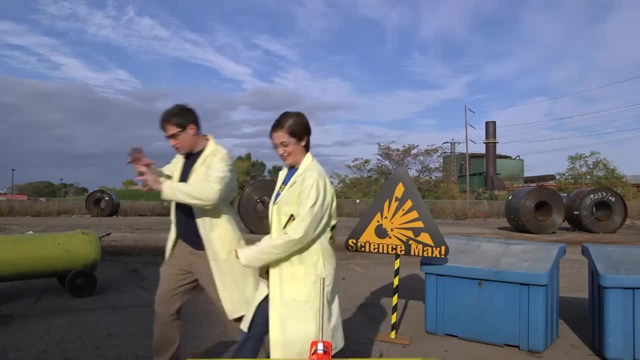 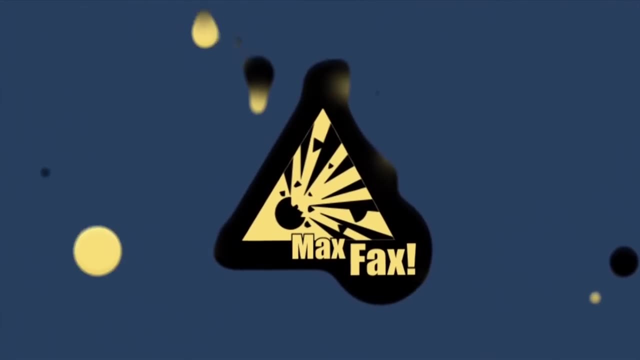 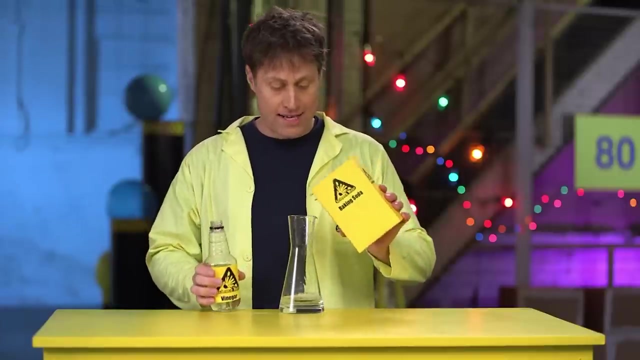 Bigger rocket. OK, so you know what. I know how to splice two bottles together. We can increase the size of the chamber. All right, This is sodium acetate. How do you get sodium acetate? Well, when you do a visit, you're. 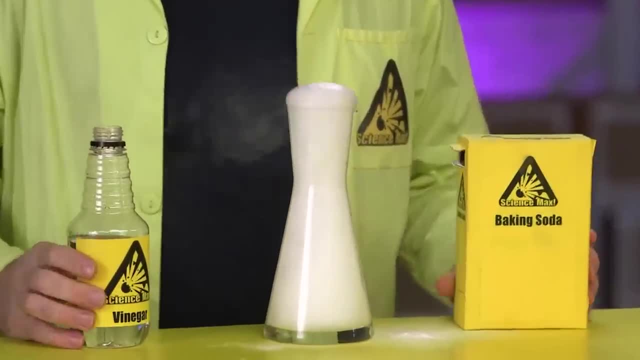 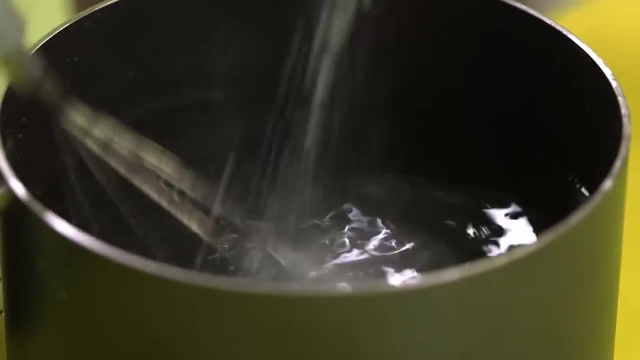 going to have a vinegar and baking soda reaction. What you have left once the reaction is finished is sodium acetate. It's a crystal and you can do something fun with it. that may seem familiar. You make a supersaturated solution of sodium acetate. 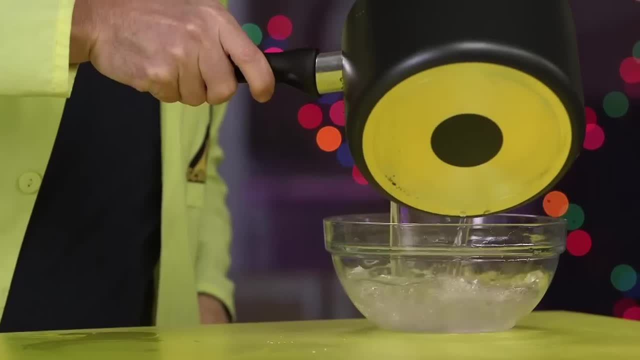 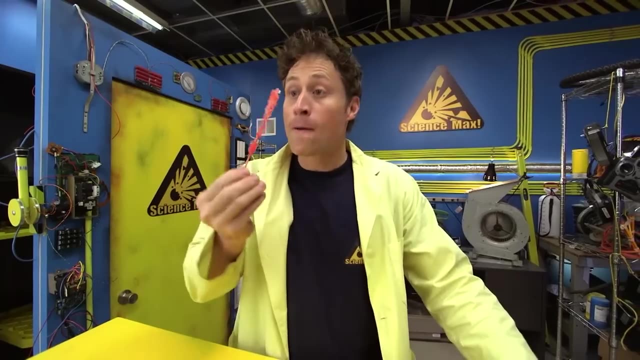 by heating water and dissolving as much as you can, And then, when it cools, you can get the crystals to reform. Now, if you did this with sugar, you could make a sugar pop, which we've done before. If you do it with salt, you could make a salt pop. 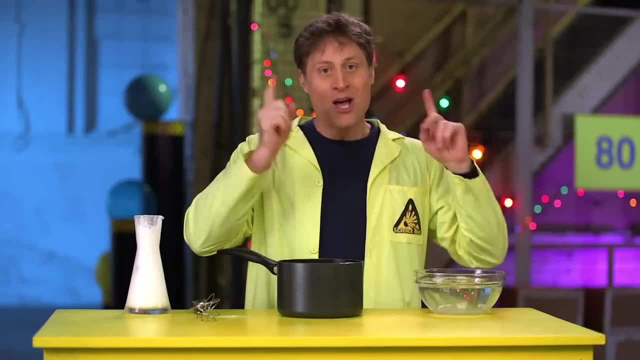 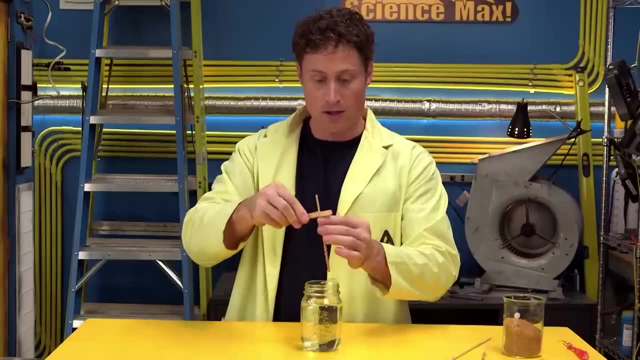 which is less appealing. And if you do it with sodium acetate, you can do this Just like with the sugar pop. all it needs is a seed crystal to get the crystals to reform, But unlike sugar, which takes a few days. 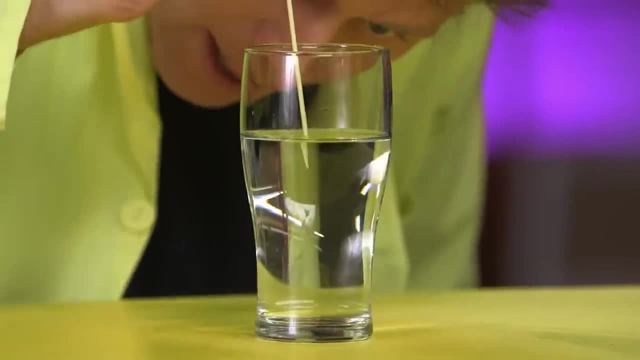 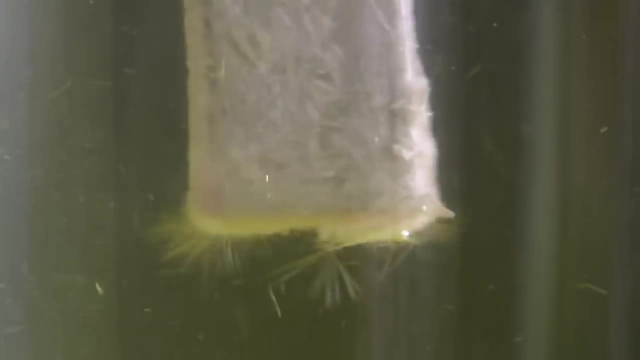 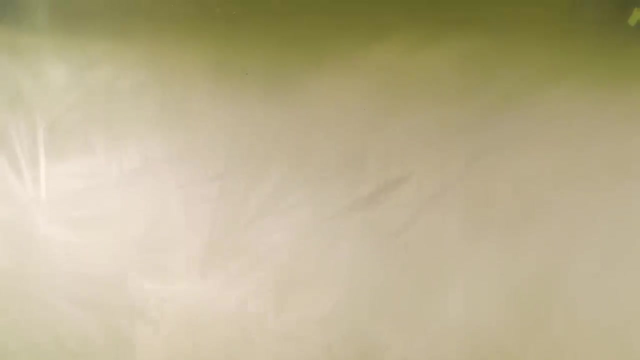 sodium acetate recrystallizes right before your eyes. Because we heated the water, it allowed more crystals to dissolve in it, Ooh- But then it cooled down afterward. There's more crystals sitting around in this water than there should be at this temperature. 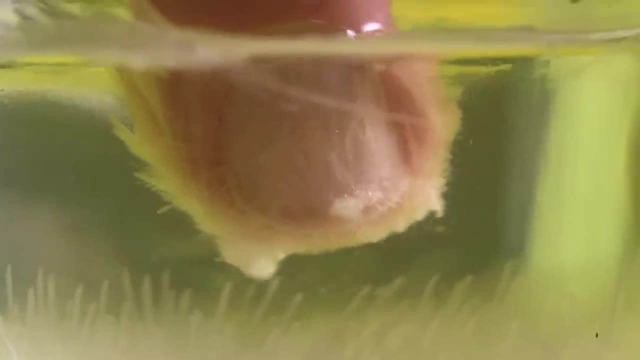 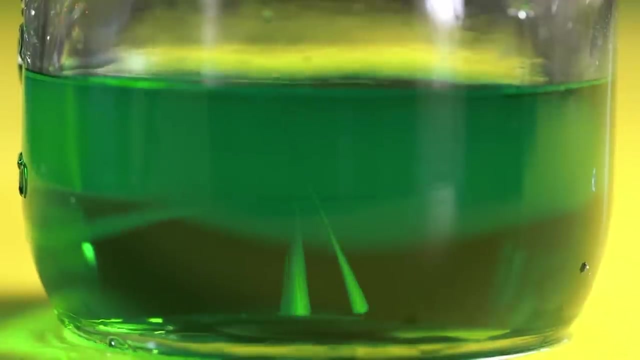 They want to turn blue, So we put them back into crystals And all they need is something to start them going. I've colored this one green because I don't know science. Maybe it'll look cool- A tiny crystal on the end of the stick. 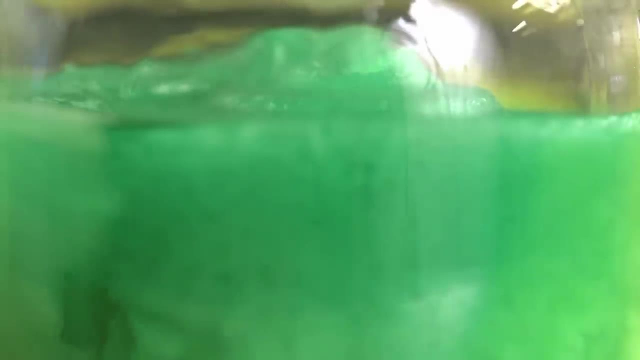 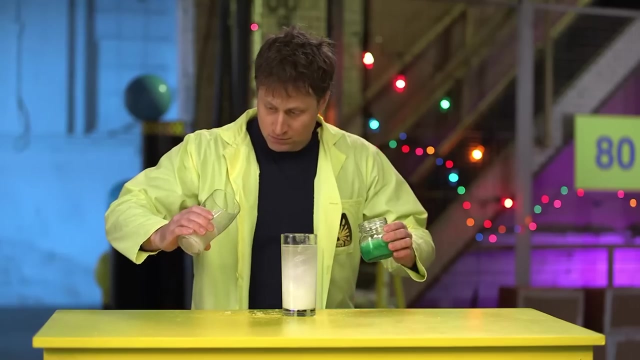 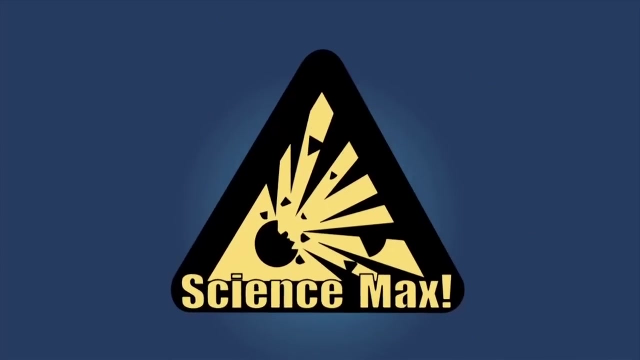 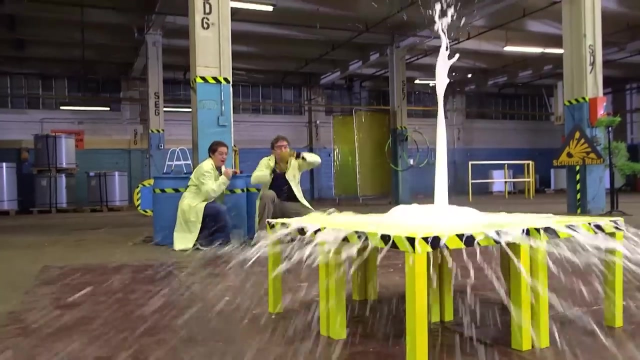 is all we need to start the reaction happening. Whoa, Wow. And there you go, Sodium acetate. Hmm, That one wasn't done yet We've gone from small containers, Oh yeah, To a large container- Whoa. 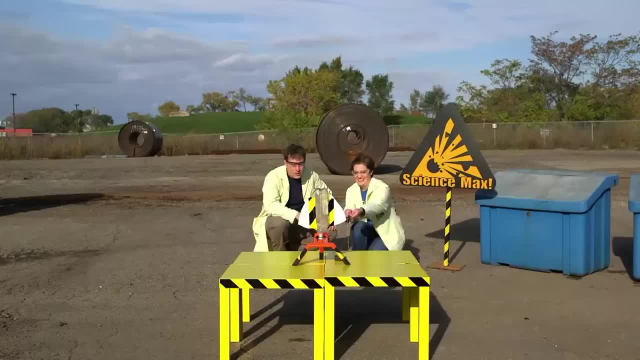 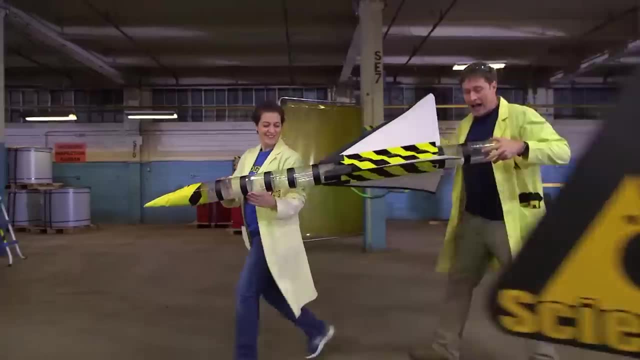 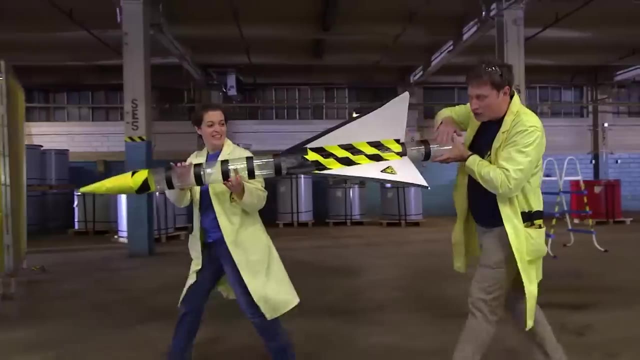 Whoa To a rocket, Yeah. So what's next? Super maxed out rocket, 12 two-liter bottles all spliced together to give us a very large chamber to build up pressure with. So the chamber is all the same. So it's all one big hollow tube. 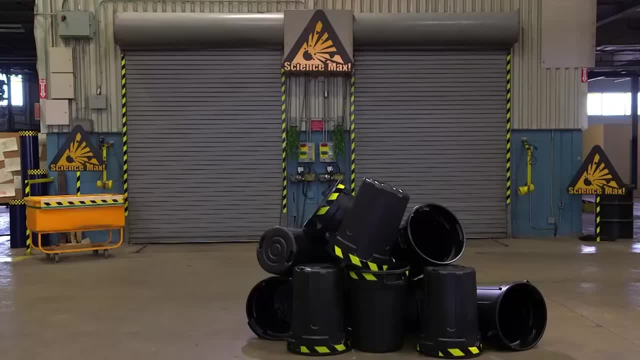 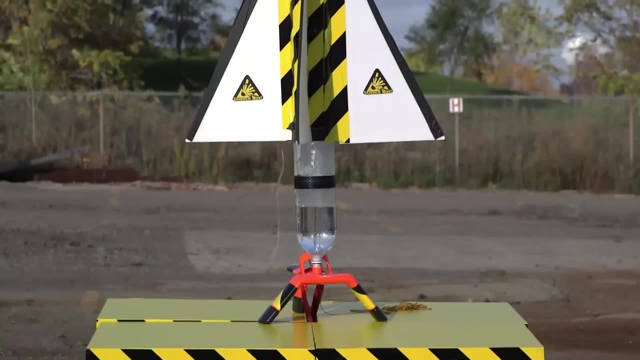 And now we're going to fire it off. Let's go, Let's do it. Awesome rocket. Yeah, Lisa and I follow the same procedure as before. We use a bag of antacid tablets held up inside the rocket with a magnet. 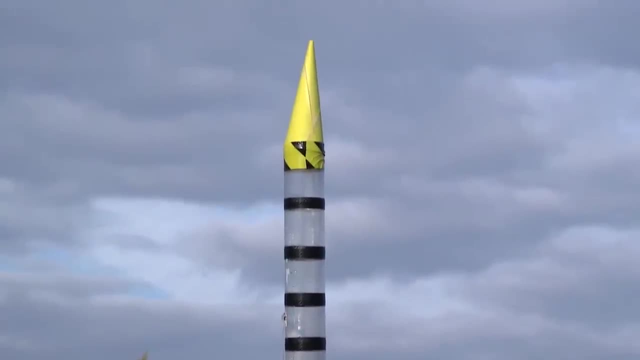 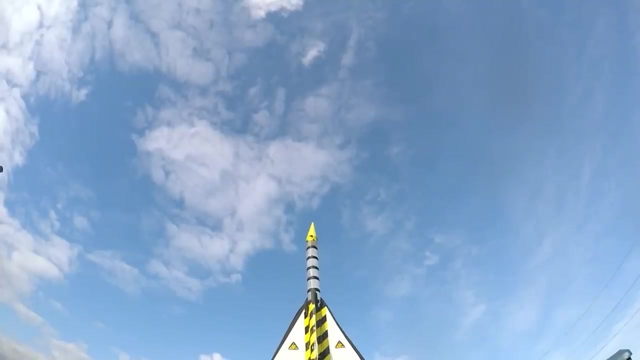 And once it's sealed on the launcher, we pull it off, let the antacid mix with the water, let the chemical reaction happen for a while to produce enough gas pressure, and then we fire it. OK, here we go. Three, two, one go. 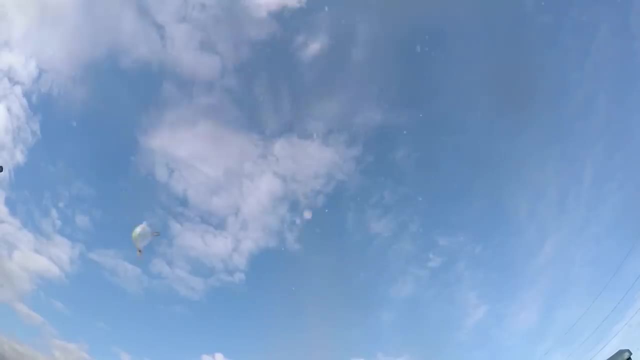 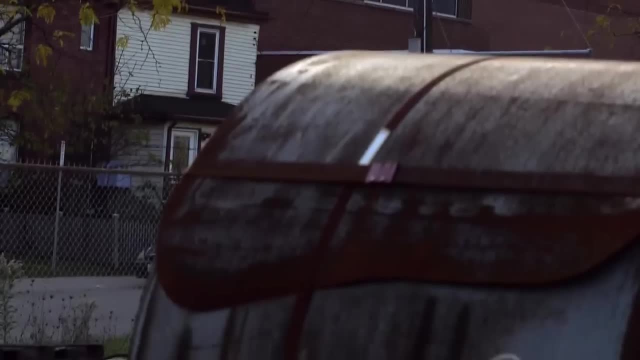 Oh my god, Oh no, Oh no, Oh no, Oh my god, Oh my god, Oh my god. That is the highest I think we've ever shot a rocket on Science Max. That's amazing. 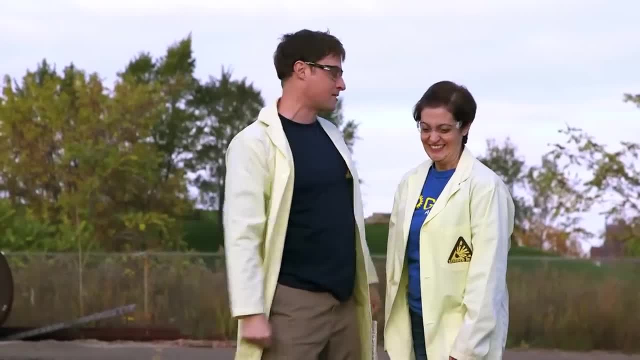 Well done. Chemical reaction rocket. thank you very much for joining us on Science. Max Experiments At Large, We should build another rocket. I think so, Because that one is probably broken. That's done. OK, let's go. Let's do it. 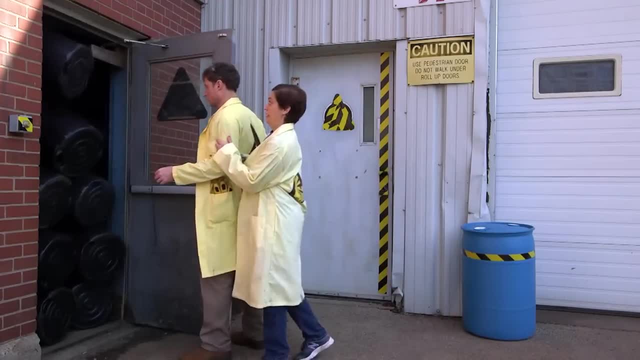 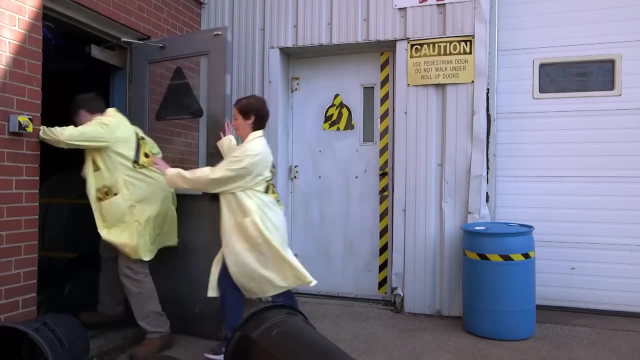 All right. so this time, I think what we need to do is: Ah, Oh no, It's nothing but garbage cans in there. We've got to turn the portal off. Come on, We've got to get Greetings. Science Maximites. 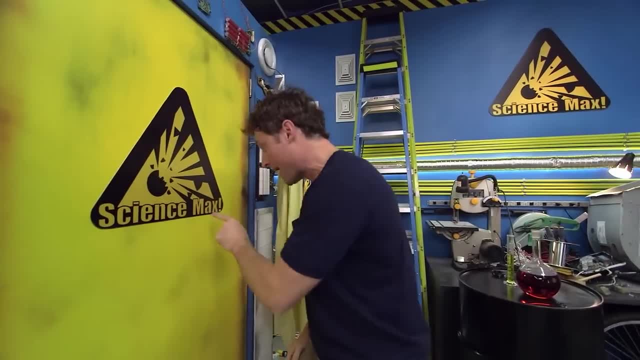 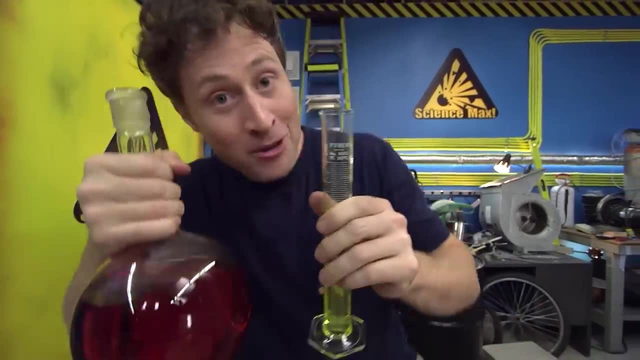 My name is Phil McCordick and the name of the show is Science Max: Experiments At Large. Today we're taking a closer look at chemistry. Ooh, Chemistry is the science of atoms and molecules, that things that make up all matter. 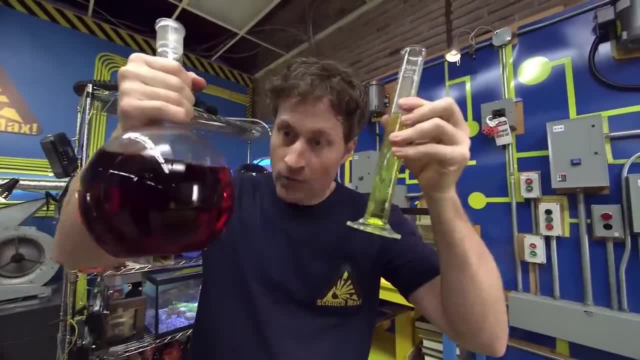 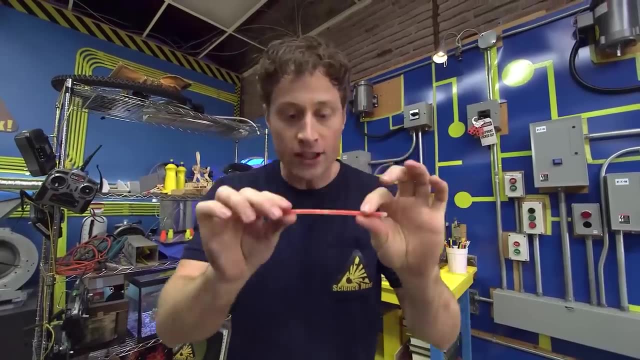 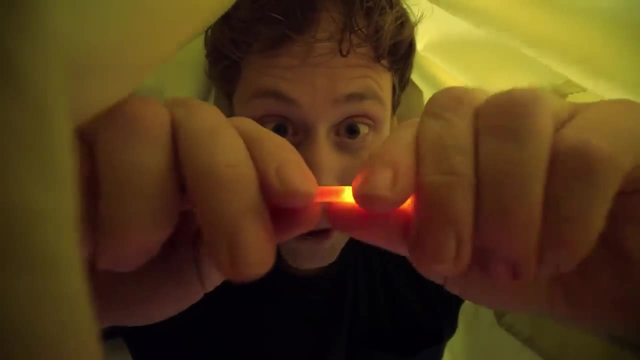 and how they interact with each other. Take, for example, this glow stick. Actually, don't take it, because I kind of need it. The glow stick doesn't glow until you- um, the glow stick doesn't glow until you break the barrier. 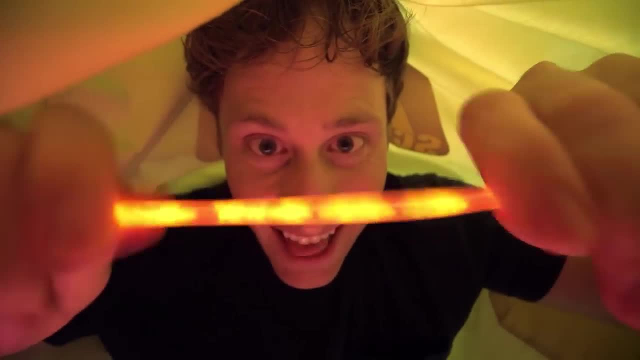 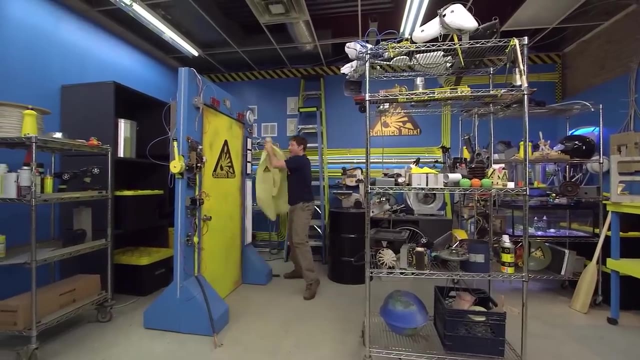 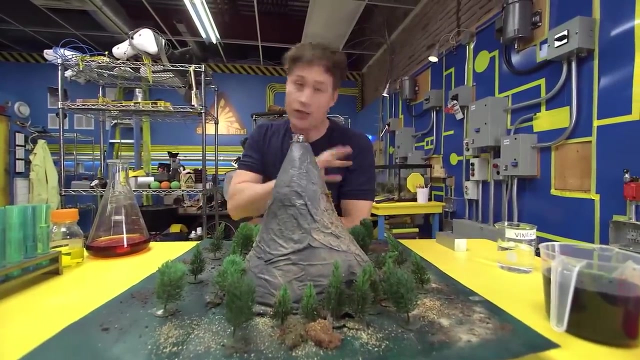 and mix the two chemicals and they start to glow. Huh, Pretty cool, huh Chemistry. Now, the chemical reaction we're looking at today is the old vinegar and baking soda volcano, But this reaction doesn't have anything to do with volcanoes. 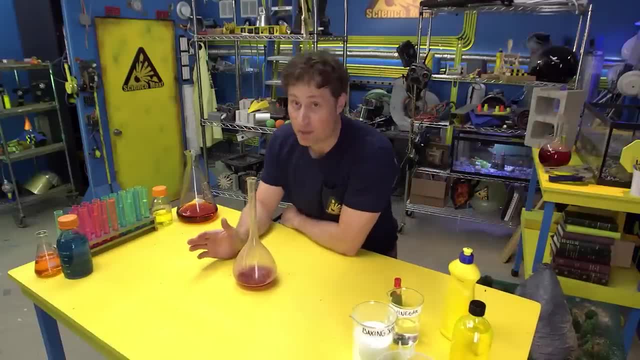 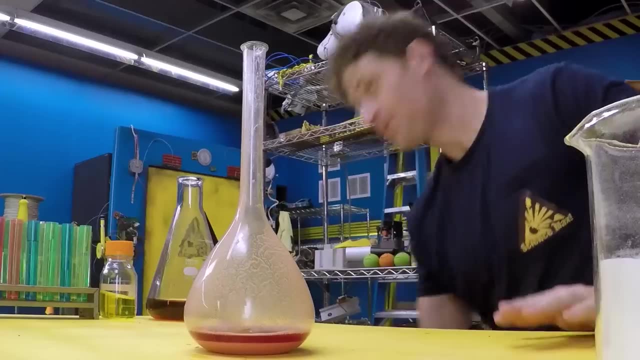 It's chemistry. Now, this experiment is totally safe, but I do recommend you get an adult's permission before you do it, because it's very messy. Uh, Uh, Yeah, Ha ha. First you're going to want baking soda and vinegar. 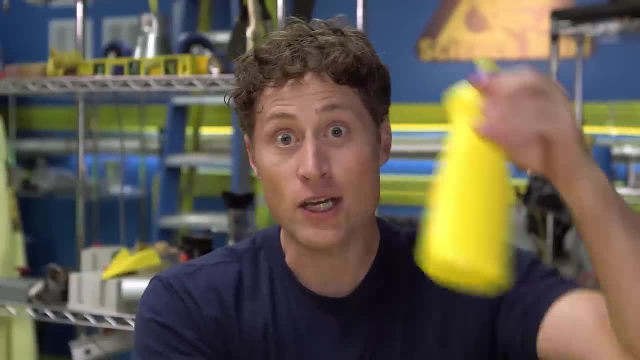 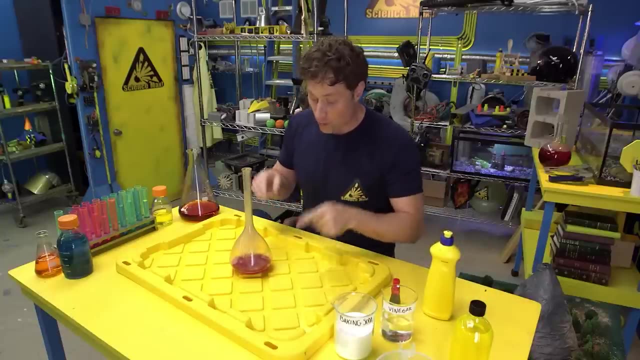 These are your two main ingredients, but you'll also need a little bit of vinegar, And you'll also want dish soap and red food coloring if you want it to look a little bit more like lava. Now I like to mix the baking soda: red food coloring. 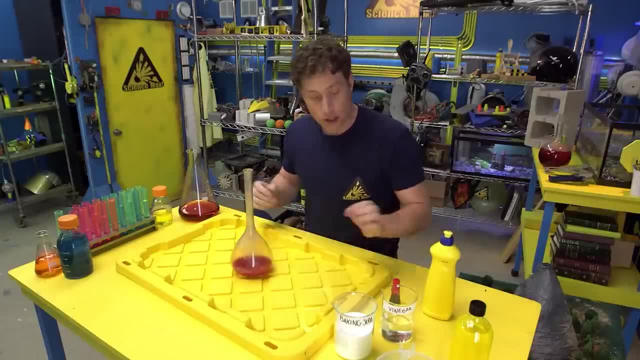 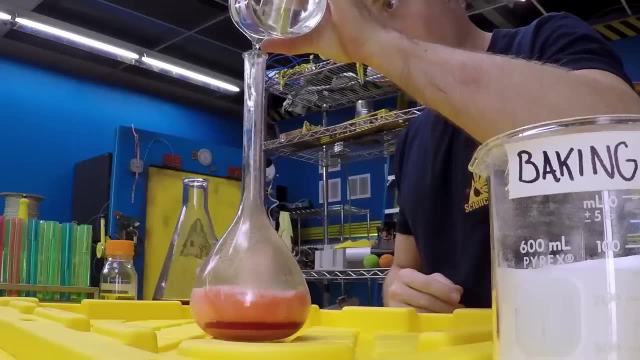 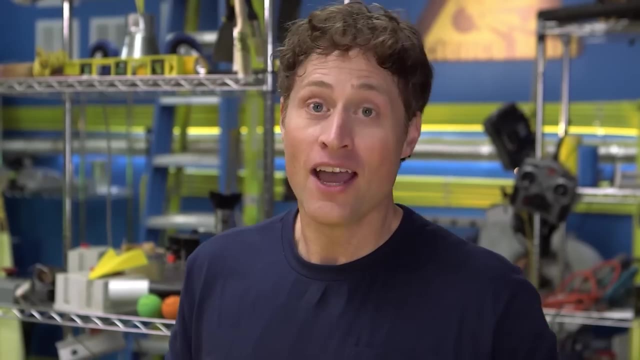 and dish soap together with a little warm water. So all you have to do is add the vinegar, And when you do this is what happens, And there you go: Chemical reaction. Now I know what you're thinking. You're thinking, Phil, how much vinegar? 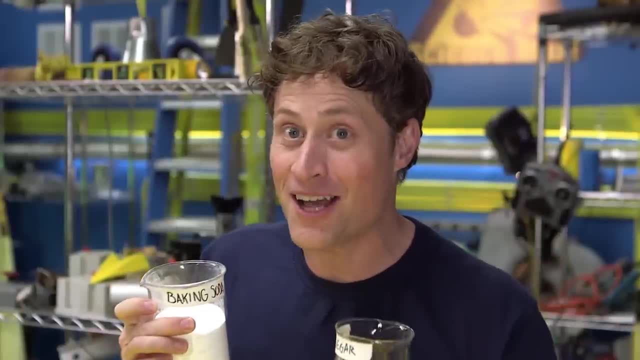 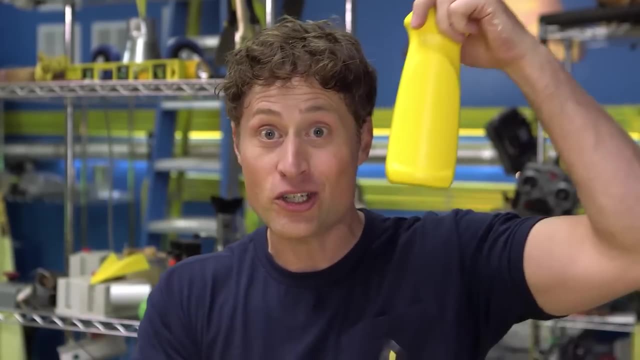 or baking soda do I use? Well, I'm not going to tell you. This is where you can be science maximites. Try different amounts: More vinegar, more baking soda, more dish soap- Who knows? Write down the amounts each time you use it. 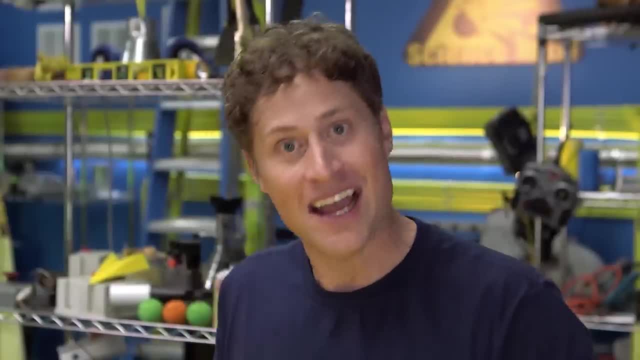 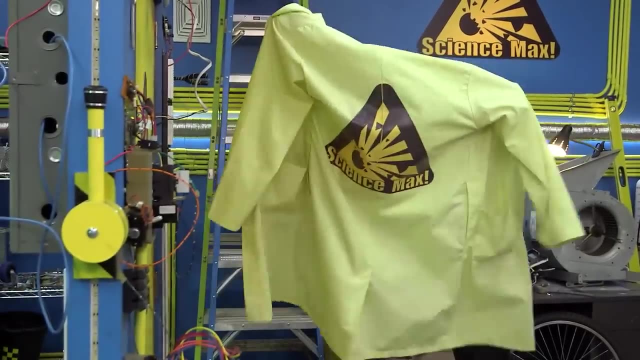 and find out what amounts work best. That's called science And that's what we're going to be looking at today: chemistry in all its forms And, of course, because it is Science- Max Experiments at Large. we're going to max out the vinegar and baking soda. 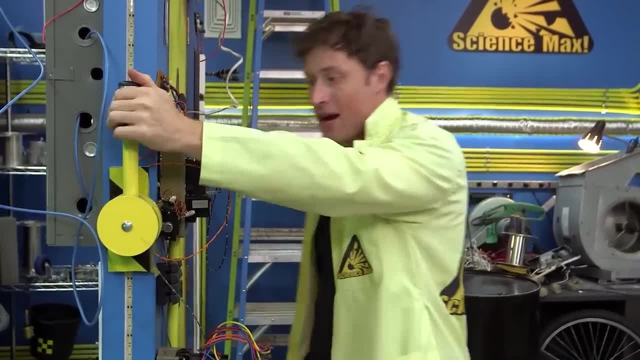 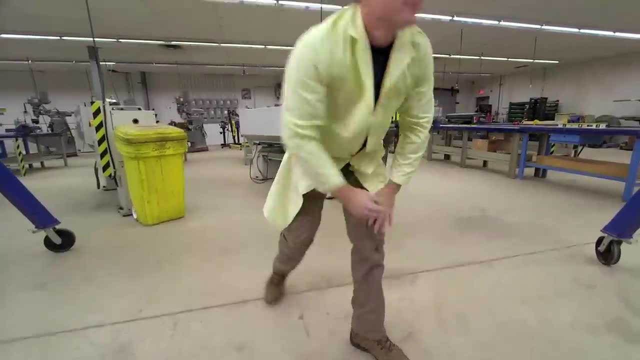 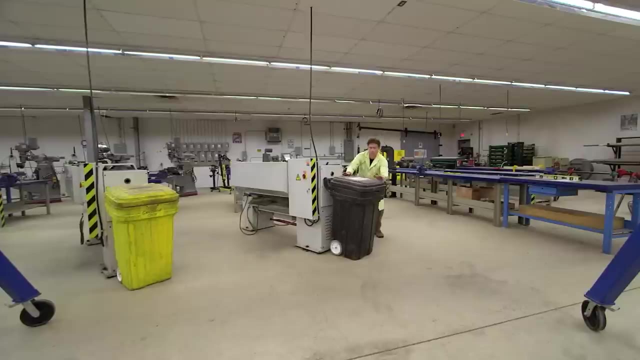 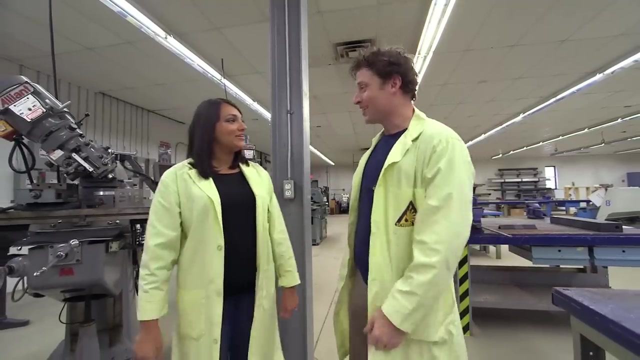 volcano. So I'm off to the Center for Skills Development and Training. Come on, Hey Talena. Hi Phil, How you doing Good? How are you Good? This is Talena. She's going for her PhD in chemistry from McMaster, right? 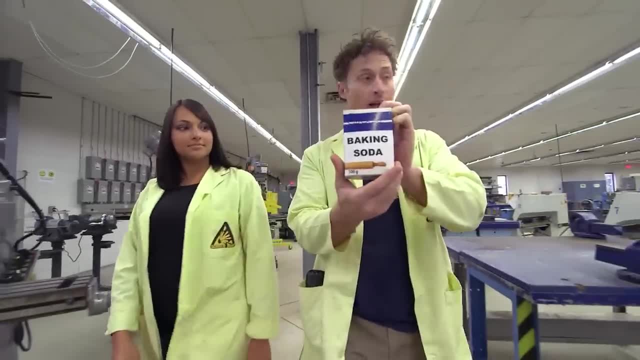 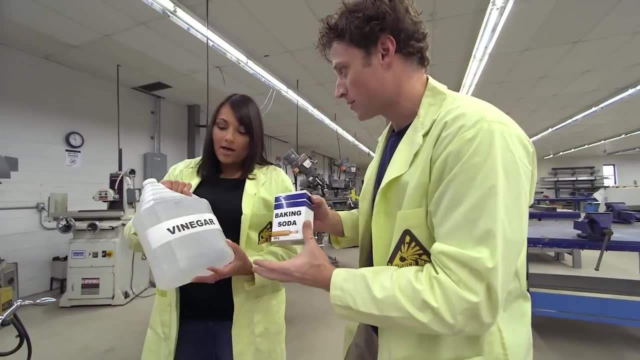 Yep, Awesome, Which means you can help me max out my baking soda and vinegar when you grab that vinegar And vinegar volcano. So what happens when we mix these two chemicals? Well, vinegar is an acid and baking soda is a base. 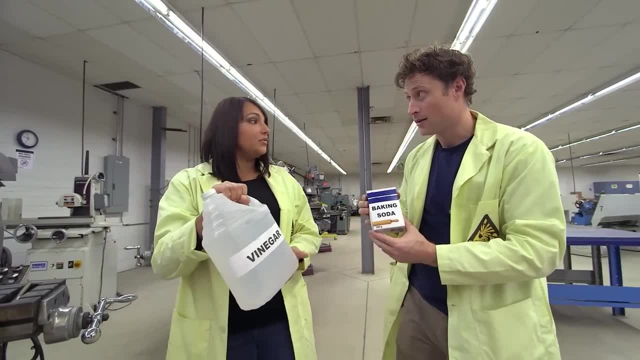 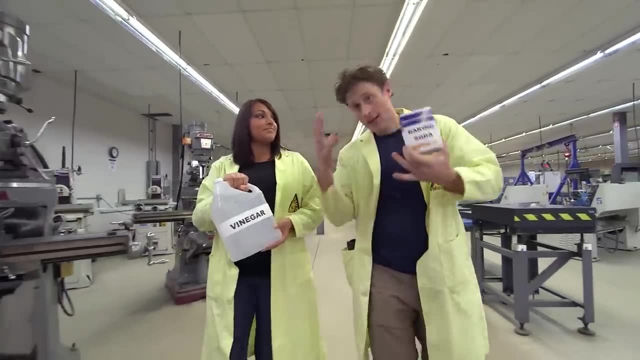 And when you mix them they neutralize each other to produce carbon dioxide and water as a byproduct. So acids and bases are kind of like opposites, Yep. So I guess that makes sense. When you put them together, crazy stuff happens. 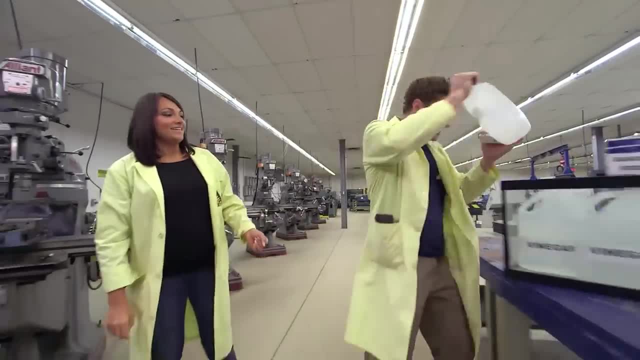 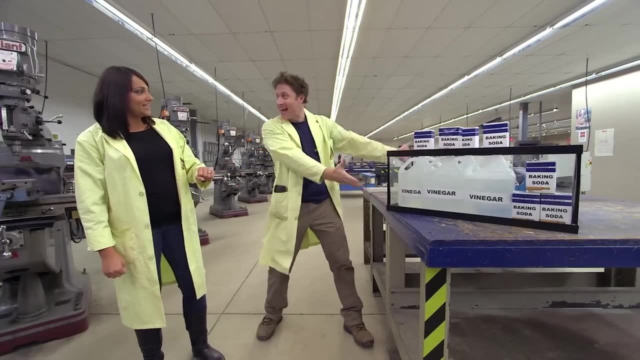 Yeah, Awesome Chemistry. OK, so I want to use this much vinegar and this much baking soda. What's with the fish? The fish tank. The fish tank is where I want to mix it all together. What do you think? Awesome. 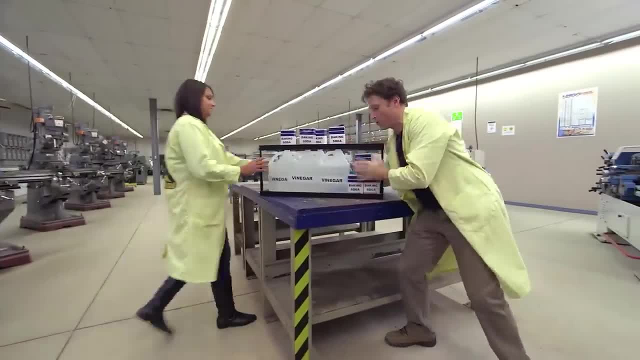 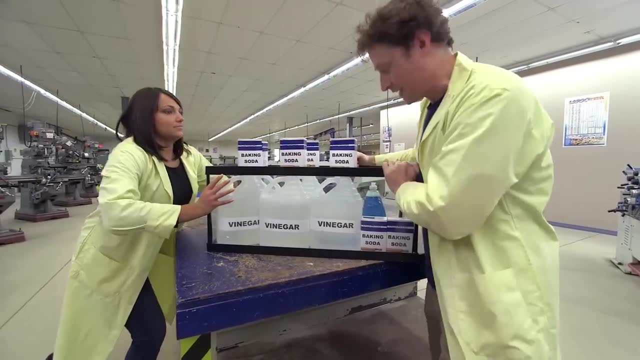 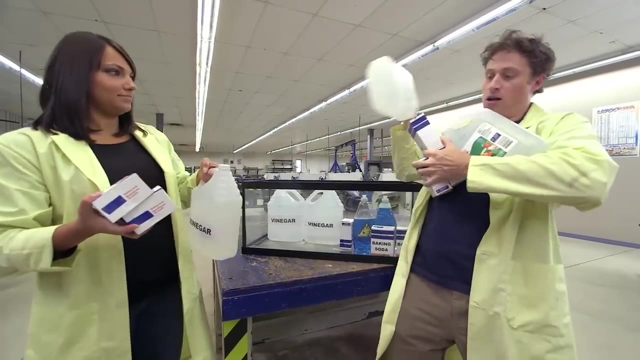 Maxed out. OK, let's move the fish tank somewhere where we won't make a huge mess. It's a little heavy. with all that We're going to have to take a couple trips. That's kind of heavy. OK, so we'll take this and that and then this and that. 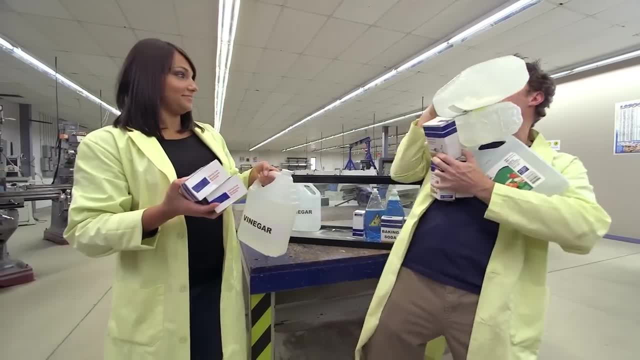 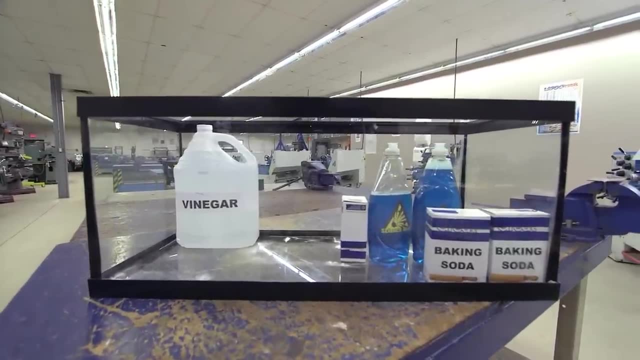 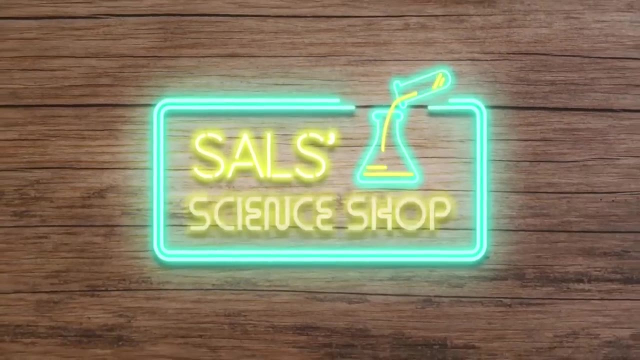 No, hold on, I can do it One more. OK, good, OK, good, Yeah, I took too much. I took too much. Uh-oh, Uh-oh, That's good, Ramona, Put it in the background. 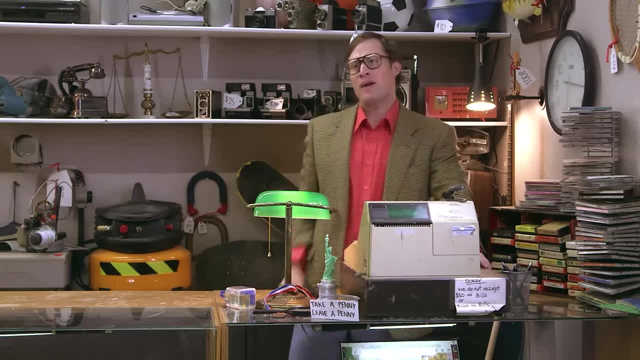 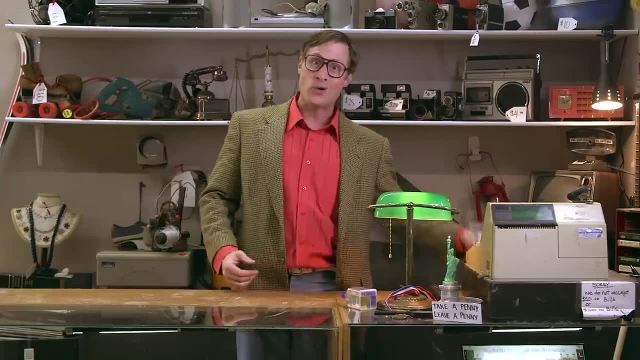 Put the sign in the background. Yeah, in the BG, I love the BG. Chemicals, Chemicals, Chemicals, Chemicals, Chemicals. What are chemicals? Are they things you have in a lab, in a jar that say chemical on them? 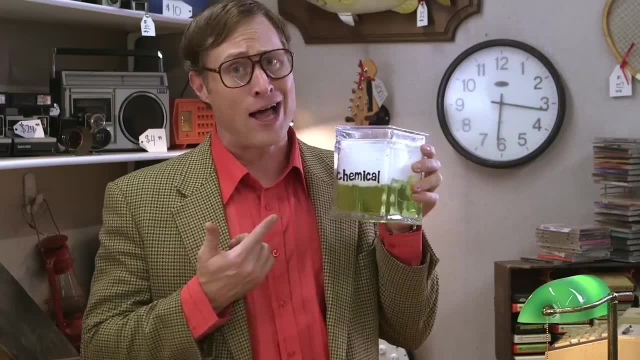 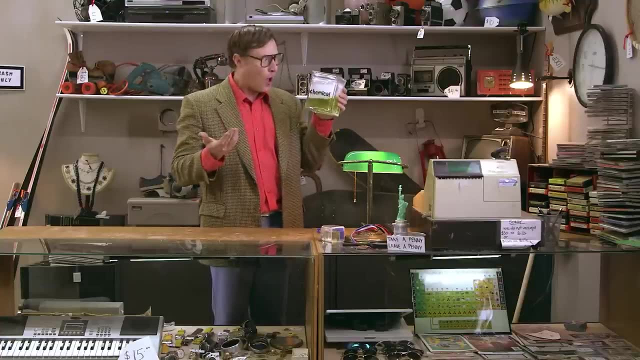 Well, yes, But if you're going to use them, if that's all you think chemicals are, then you need to know your chemicals. Turns out, the stuff in the jar is a chemical, but the jar itself also made of chemicals. The table I'm putting it on made of chemicals. 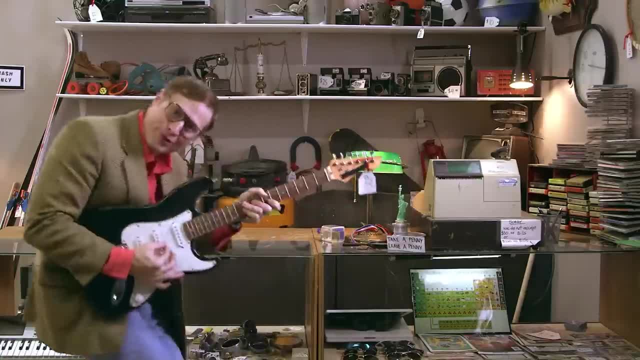 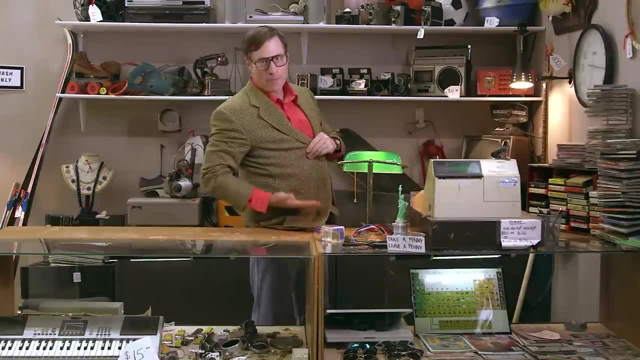 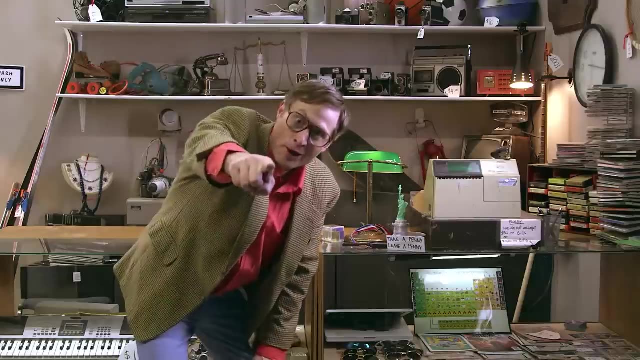 My lunch chemicals. Roller skate chemicals. My jacket chemicals. This guitar chemicals. My shoe chemicals. This watch chemicals. This fish chemicals. Chemicals, Chemicals, Chemicals, Chemicals, Me chemicals. 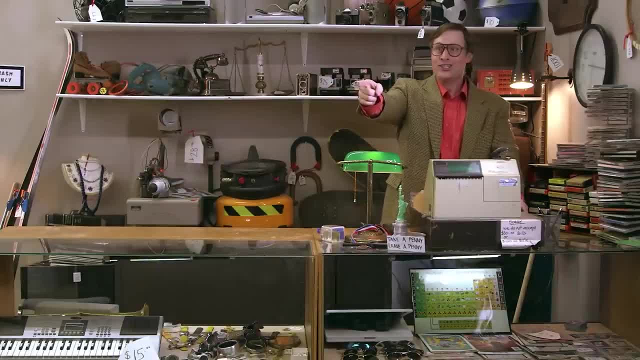 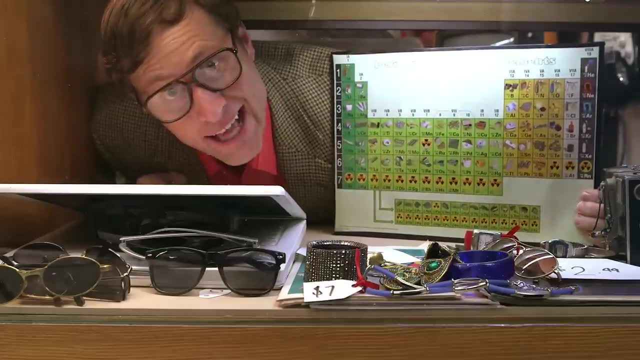 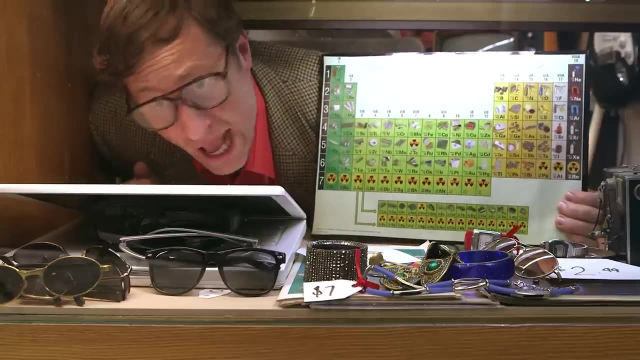 You chemicals, Ramona chemicals. No, I said you're chemicals, Chem, never mind. This is it the periodic table of the elements. All matter in the universe is made up of these pure elements. They go together in different ways to make up everything. 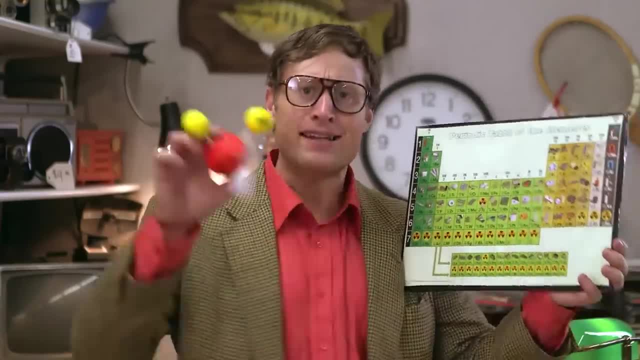 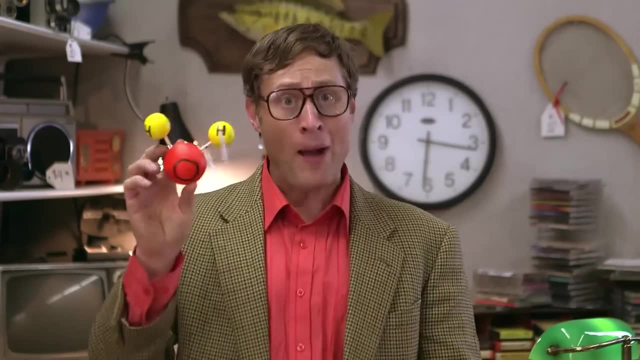 All matter. Think of it like building blocks. These little atoms are some of the elements on this periodic table. You got one oxygen, two hydrogen Bam. you got a water molecule. One carbon, two oxygen. hey, it's carbon dioxide. 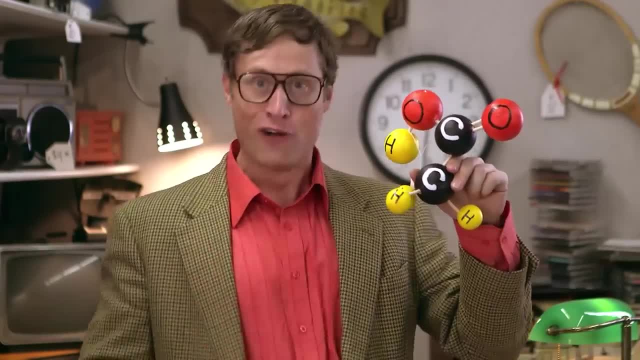 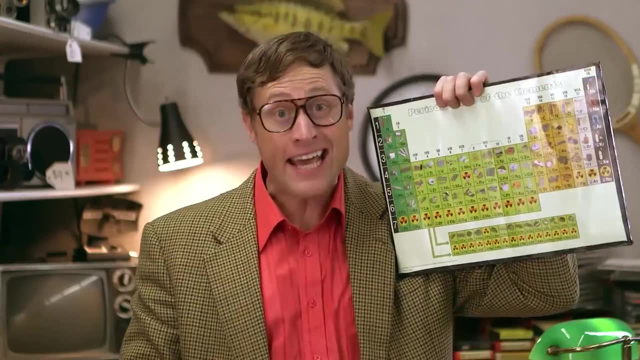 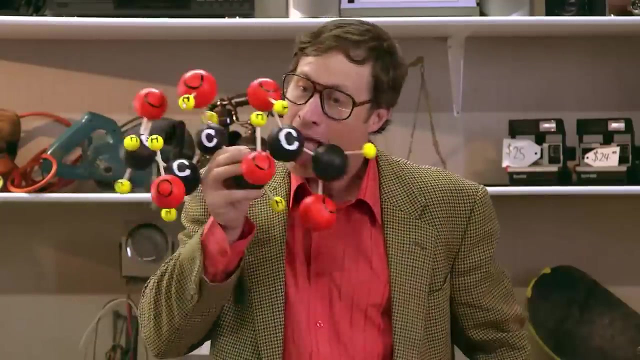 Two carbon, two oxygen, four hydrogen skadoosh vinegar, One sodium, one chlorine. hey, that's some. All matter in the universe is just the stuff on here combining into these. And now you know your chemicals: Mm sugar. 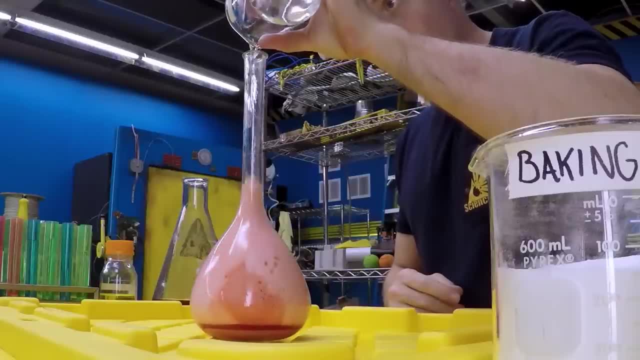 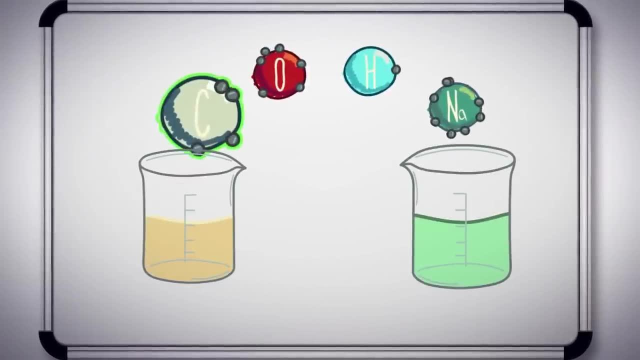 Let's take a look- Let's take a closer look- at what's going on when we mix vinegar and baking soda. All chemicals are made of atoms. There's only four types in our reaction: carbon, oxygen, hydrogen and sodium. When they go together like this, this: 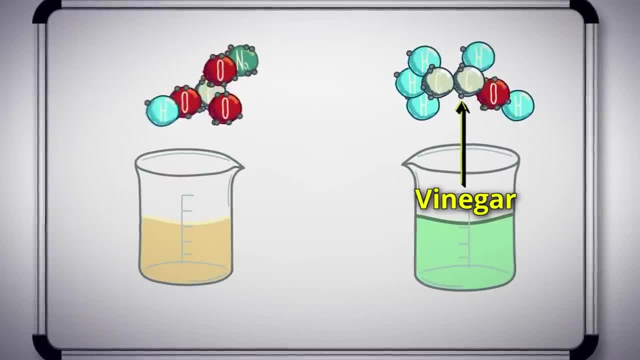 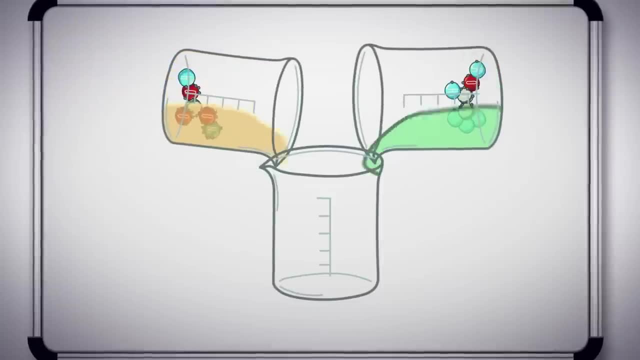 is a molecule of vinegar or acetic acid And this is a molecule of baking soda or sodium bicarbonate. When chemicals react, they switch atoms. That one goes there, this one goes over here, and then this one turns into this: 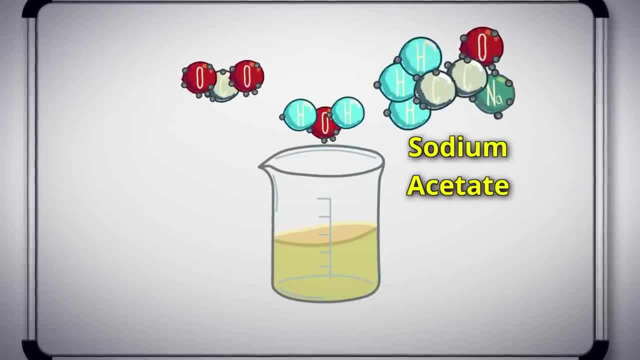 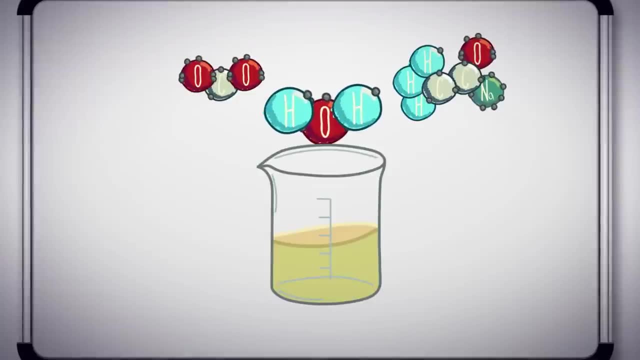 and then what you end up with are new molecules. This one is called sodium acetate and this one is carbon dioxide gas, the gas you breathe out. And do you recognize this one Right, water, H2O. Why all this happens gets complicated. 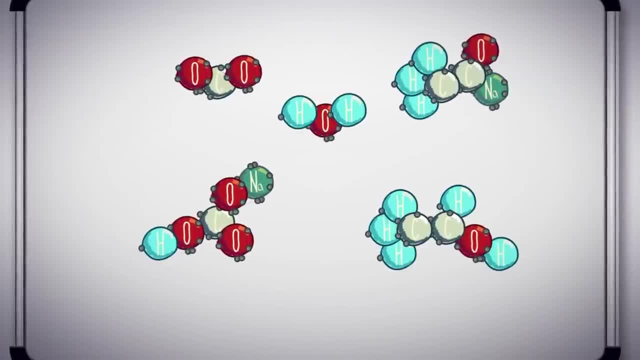 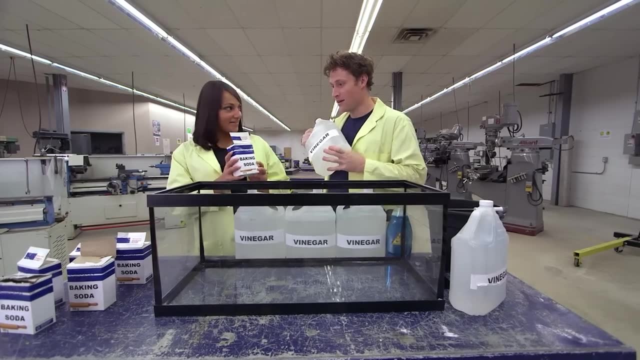 but the study of chemistry is all about how molecules are built and react with other molecules. All right, Tillian, are you ready? Yep, You're going to pour all your baking soda in the fish tank and I'm going to pour the vinegar into this bucket. 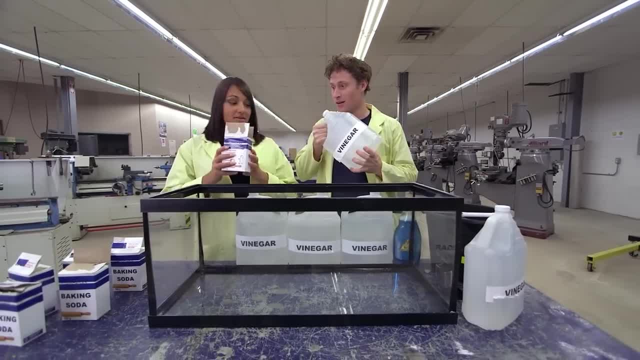 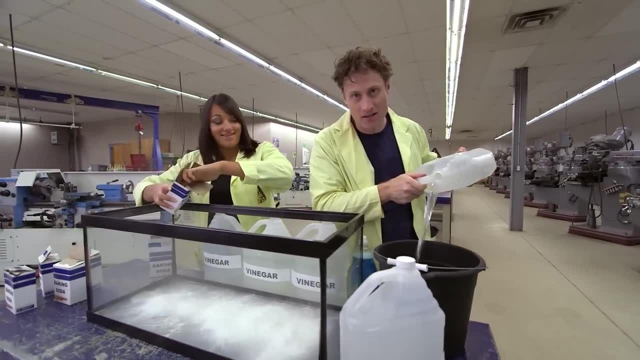 because you don't want to pour them together right away. OK, you ready? Yep, OK, go for it. When you're doing your PhD in chemistry, you get to do stuff like this. Yeah, Really, I get to do a lot of fun reactions in the lab. 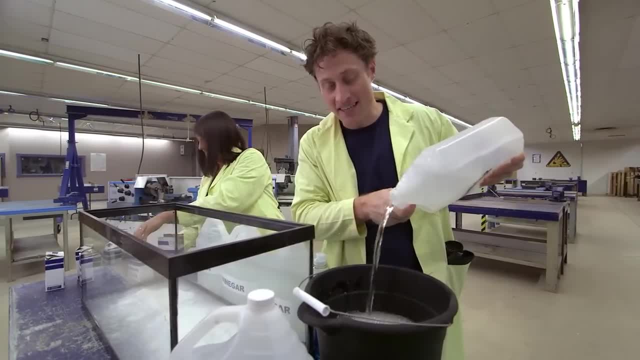 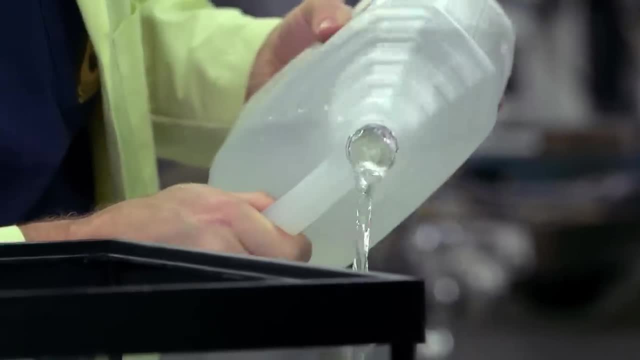 Oh, that's, I'm jealous. Have you ever done this much vinegar and baking soda in one time? I can't say I ever have. There you go. That's what I like to hear. I already put the soap in. I already put the soap in the bucket. 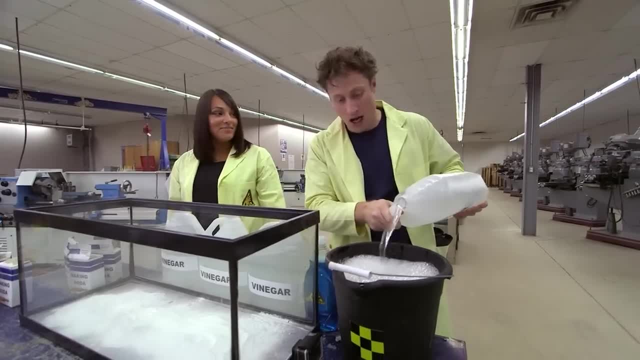 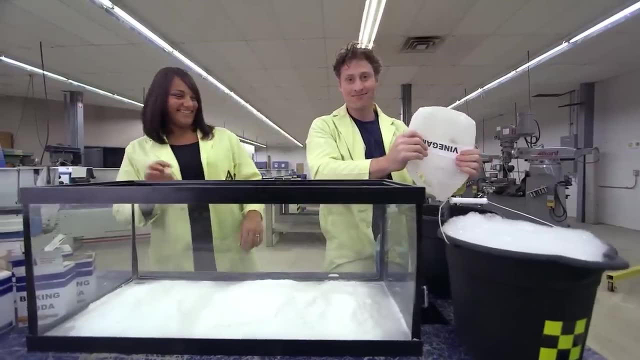 so it would mix with the vinegar when I poured it in. Are you done your baking soda already? I am. I'll pour faster, Oh faster. It smells vinegary, It smells vinegar. It makes me want french fries. OK, Tillian, you take this very full bucket of vinegar. 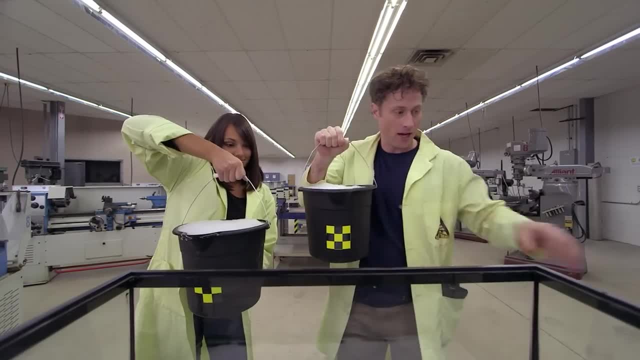 and dish soap. Thank you, I will take this one. Uh-oh, we still have our third bucket. OK, I'm going to. I'll do these both at the same time. OK, Ready On the count of three. 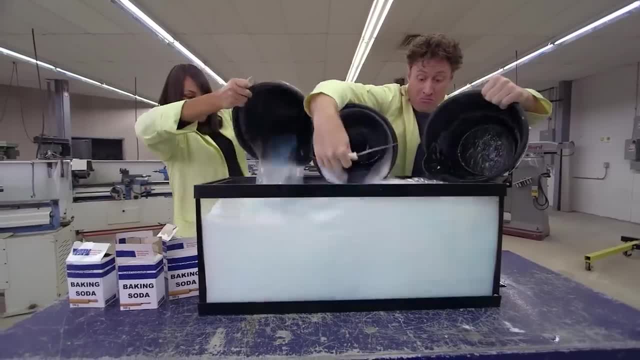 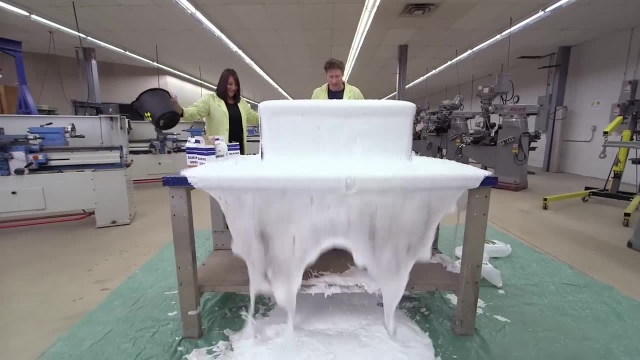 1, 2, 3.. Whoa, Whoa, Whoa, Whoa, Oh, ho, ho, ho, ho, ho, Wow. OK, That's awesome. So the one thing it didn't do, it didn't shoot up. 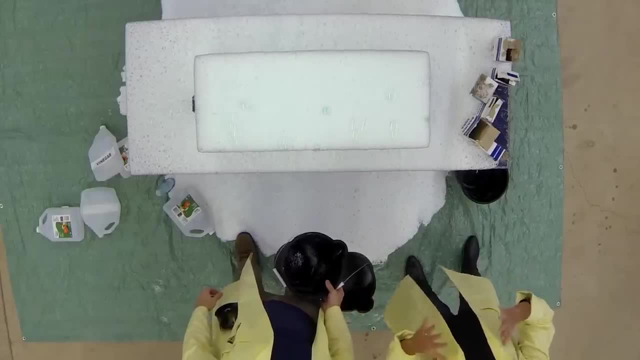 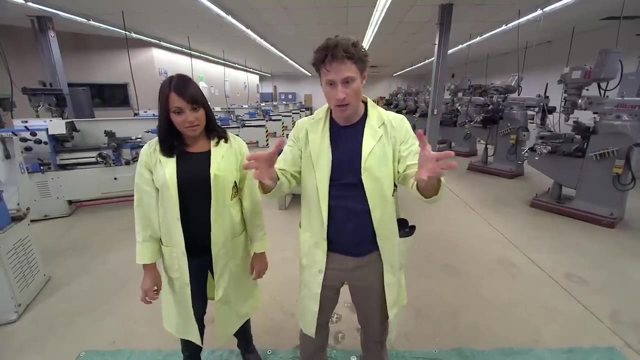 in the air though. Yeah, it's because the top is quite open, So you would need to constrict it to get it to shoot up. Oh yeah, because we're using just sort of a square, a rectangular prism container. 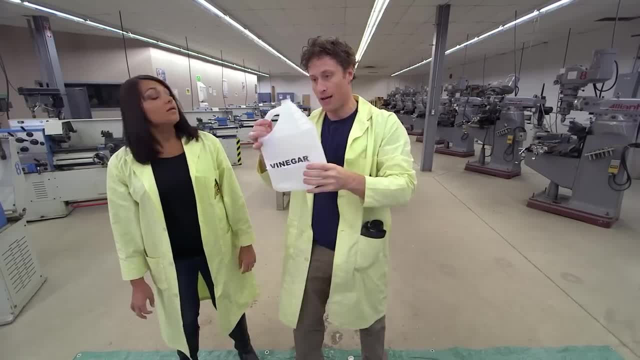 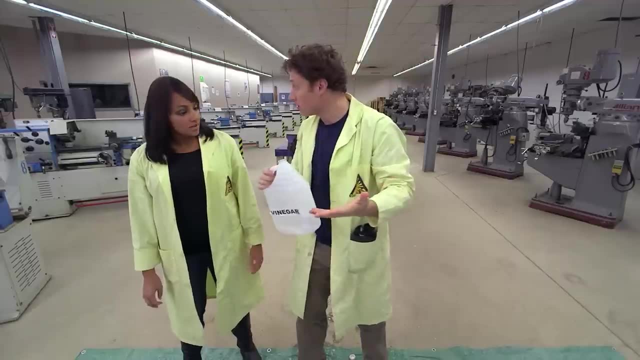 We should get something that's maybe something more like our vinegar bottle, right, Because there's lots of space down here, but then it forces it into a tighter opening at the top there like a volcano. Yeah, And what else can we do to make it even more powerful? 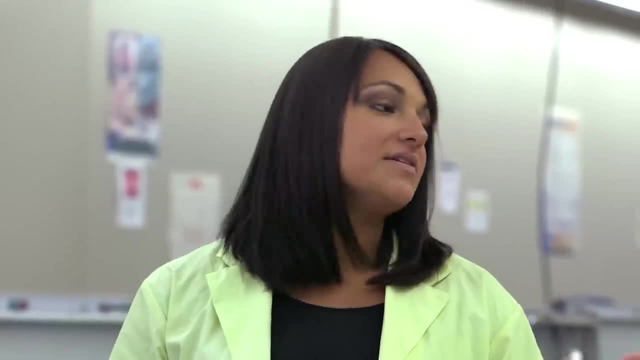 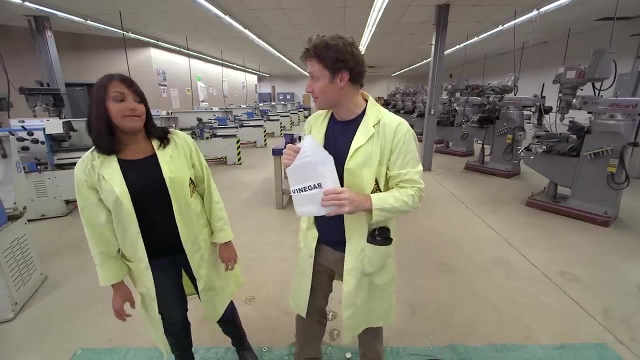 to max it out, Vinegar is only 5% acid. The rest is water, so you could try using 100%. So what kind of acid is vinegar? It's acetic acid. So vinegar is actually only 5% acetic acid and 95% water. 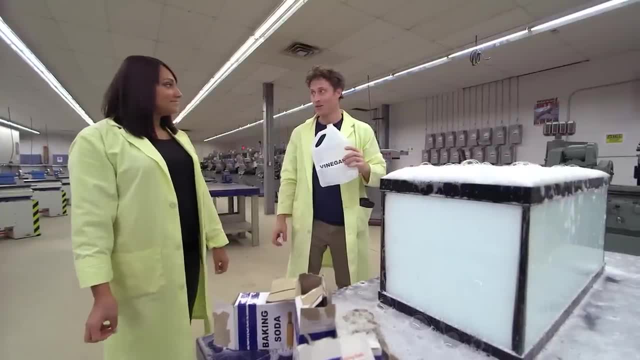 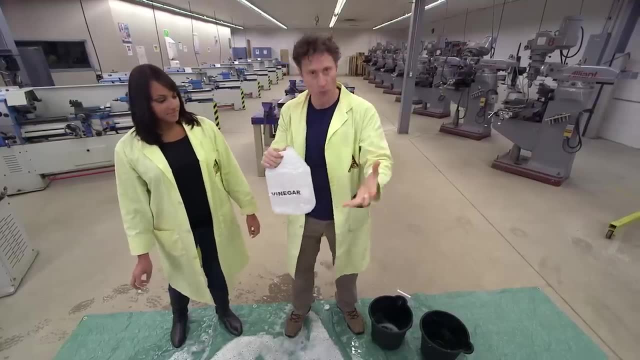 So you can get 100% acetic acid? Yeah, Can you get 100% acetic acid? Yes, Awesome. Why don't we get a container that's sort of shaped like a funnel, like a volcano? Yeah, And 100% acetic acid, and we'll do it again. 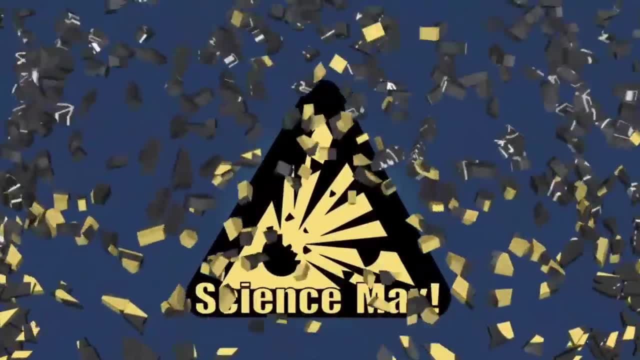 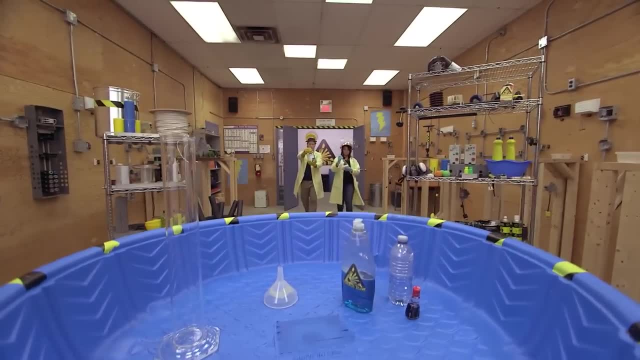 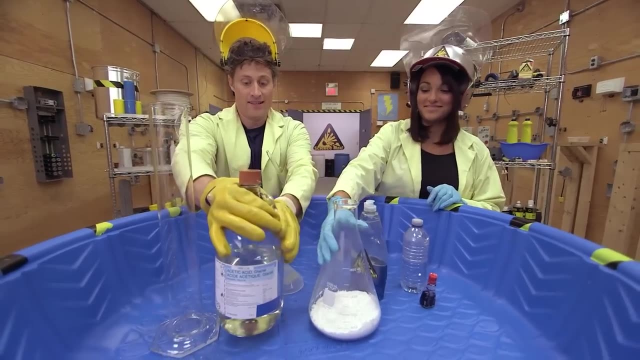 Sounds good? All right, let's do it. Our vinegar and baking soda reaction went pretty well, But now we're going to try it with a much stronger type of the same kind of acid you find in vinegar. Carefully putting this down. 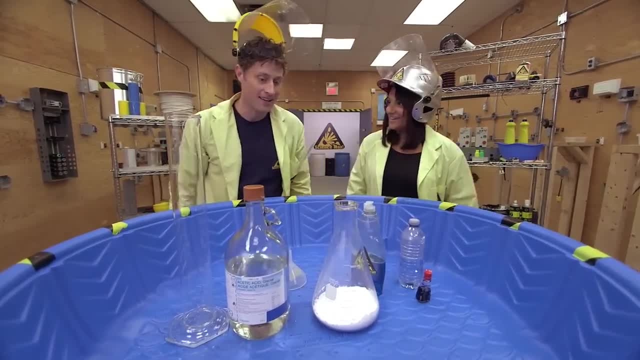 And watch out for the baking soda. You never know when it'll get out. And well, I guess that's just baking soda. huh, Yeah, that's pretty safe. Yeah, OK, good, So this is baking soda vinegar volcano. 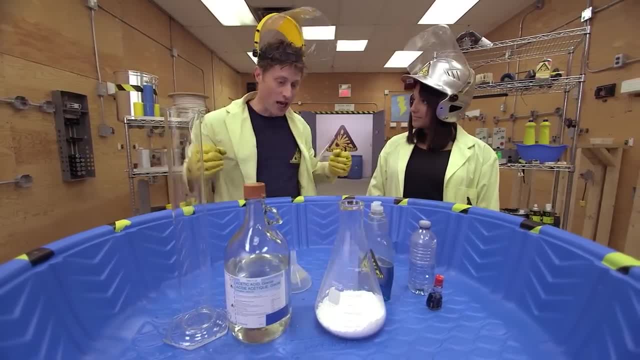 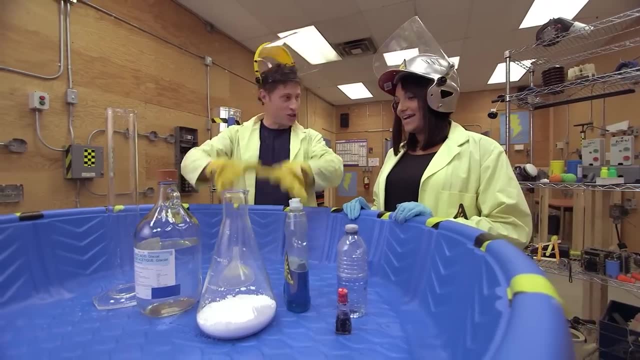 version two, We have this differently shaped glass. What do you call this? again, That's an Erlenmeyer flask. Why is it called that? It's actually named after a scientist. Did he look like that? Was he sort of shaped like this? 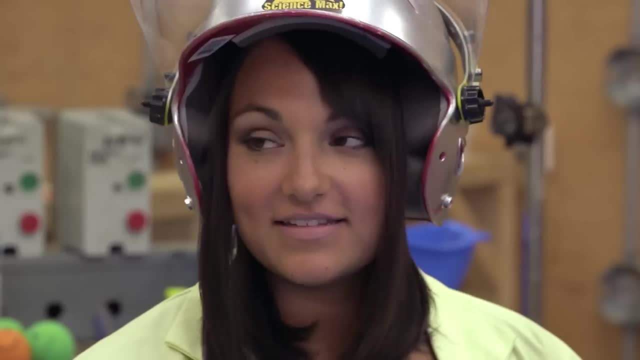 No, No, Was he just a good chemist, Good scientist, and I think he designed the glass. Oh see, there you go. So if you want to have a glass named after you, be a good chemist and design a glass. 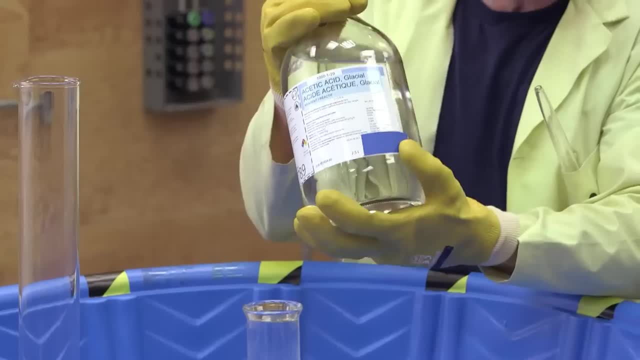 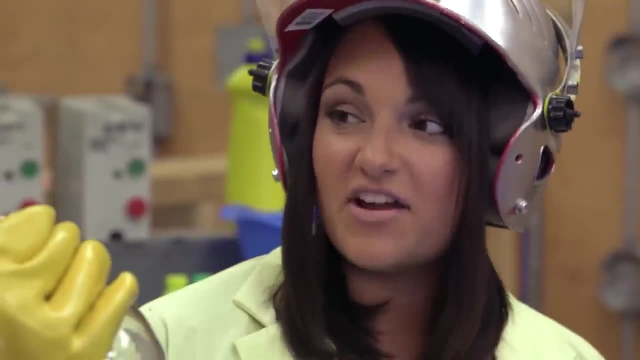 I want to make a fill beaker. So this is 100% acetic acid, Yep. And what's the difference between this and vinegar? Vinegar has a lot of acid. Vinegar has 5% of this and 95% water. 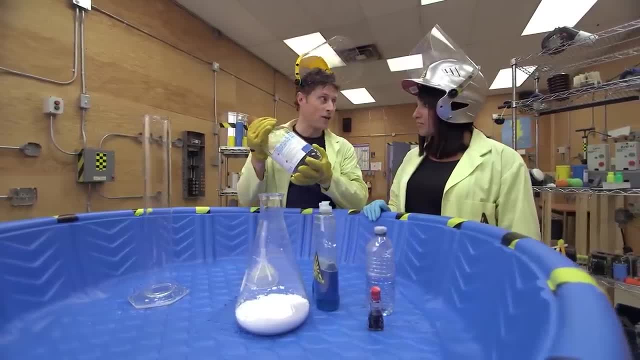 But this is 100%. so it's much stronger, Much stronger. Can you put this on your french fries? No, I wouldn't be putting it on your french fries. No, As chemicals go, how dangerous is this? It's not too dangerous, but you definitely. 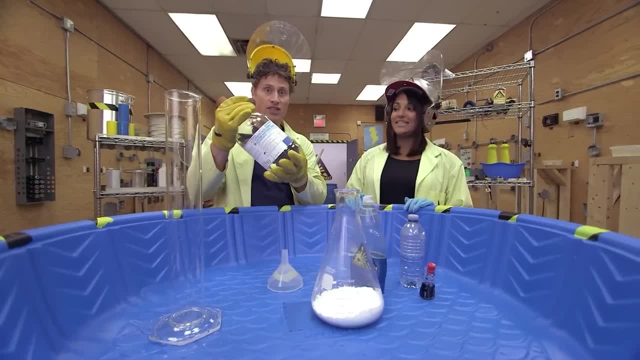 don't want to be breathing it in, and you don't want to be eating it Or getting it on your skin. That's why I'm wearing these fancy-pantsy gloves. So what I'm going to do is I'm going to pour the acetic acid. 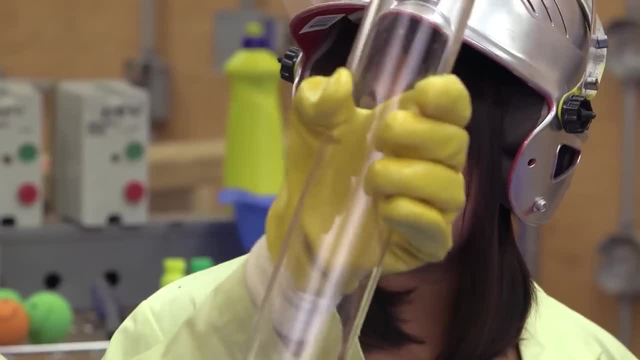 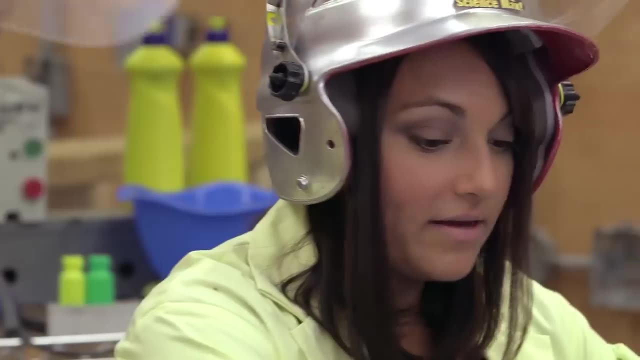 in this. What's this called? That is a graduated cylinder, Because it finished school, So it graduated. Now you're going to mix water and food coloring and soap all together, Yep, And pour it into there. It'll help dissolve some of the baking soda. 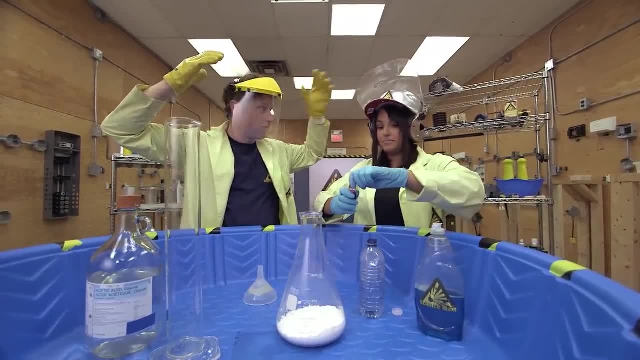 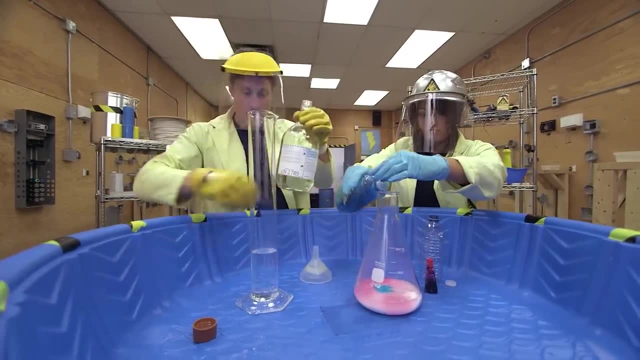 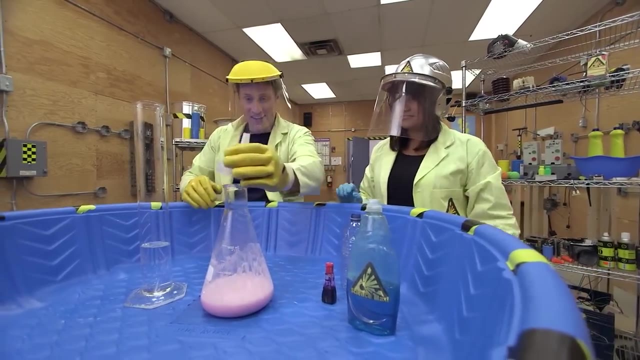 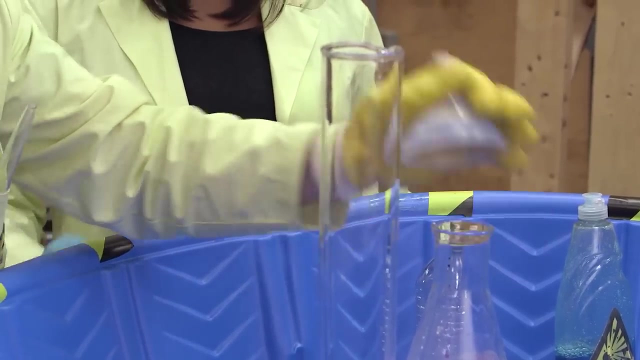 so hopefully it'll react better with the acid Sounds good. Face protection- Oh, All right, that's good. And now, when we do it, I want to add the funnel at the end to accentuate the concentration, But I don't know if it's going to go so fast that I won't. 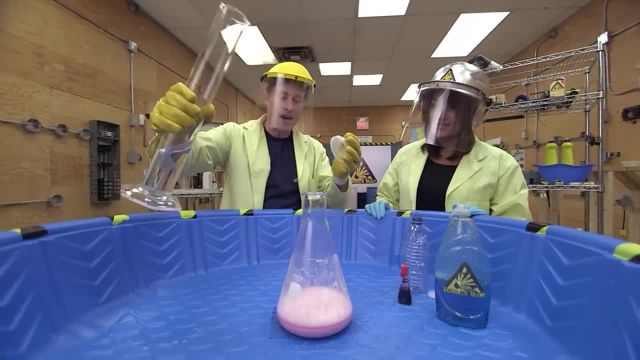 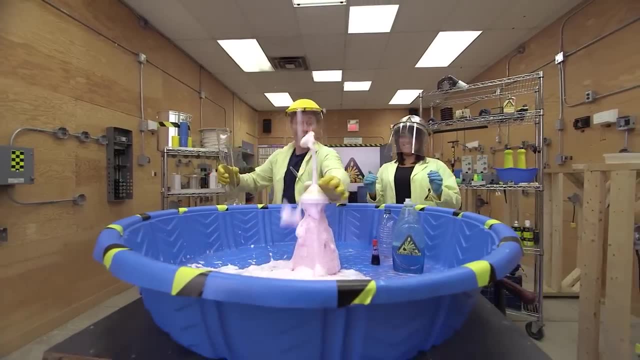 be able to get it in there, but we'll try it. We'll try it. Vinegar Baking Soda Volcano version two: Woo, Woo, Ha, ha, ha, ha ha. Oh, Good thing you got the mask. 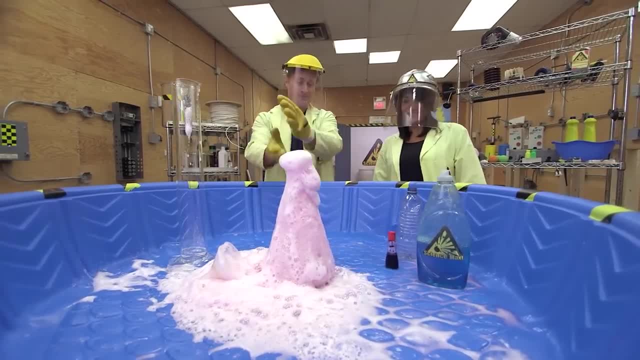 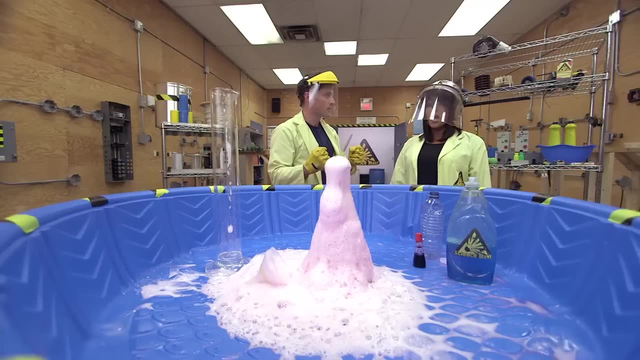 It smells a lot like vinegar. It's really strong. That was pretty good, But what can we do to make it even bigger? Well, you could try using a different chemical reaction. Oh OK, Like what? The decomposition of hydrogen peroxide produces oxygen gas. 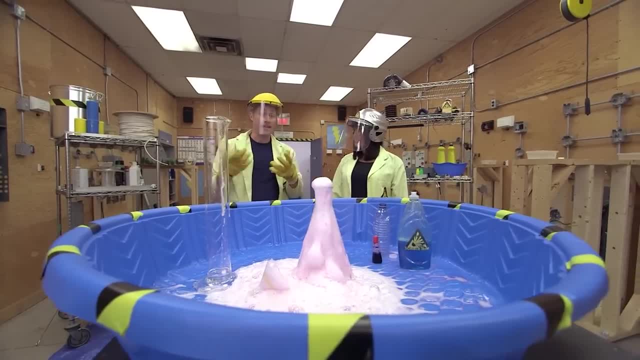 and so that one's pretty vigorous if you use a catalyst. So we want something that makes a lot of gas, so that it makes a lot of bubbles when you put the soap in it. Yep, Great, let's do it. And the sooner you leave that smell, the better, I think. 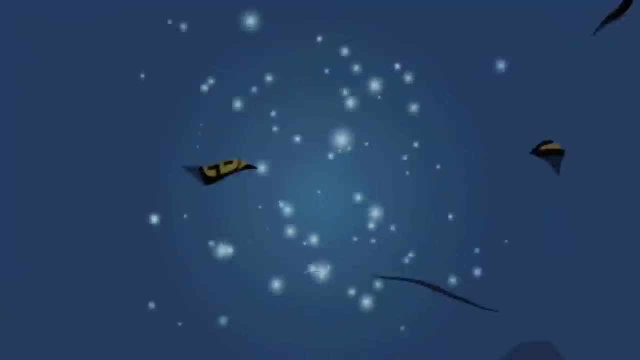 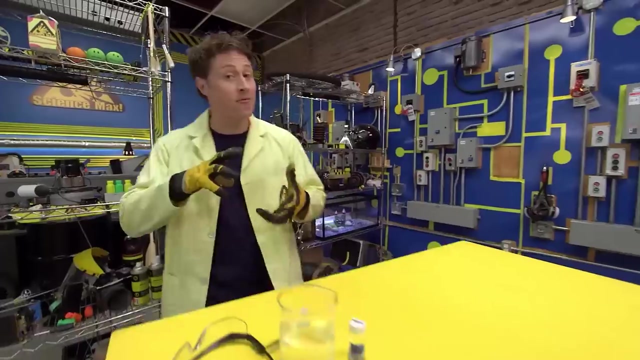 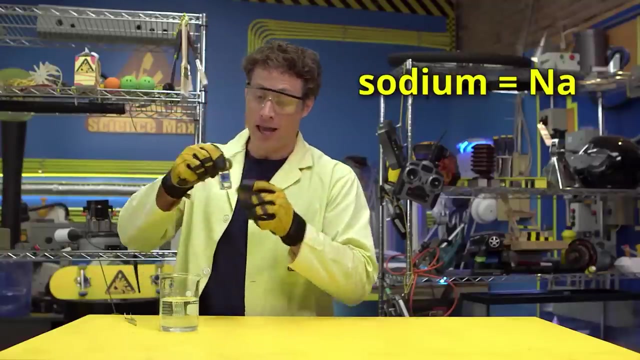 for my taste, Today we're combining two different chemicals to create a reaction. Sometimes chemicals can combine in a way that makes them very different from how they started out. For example, this is sodium or Na on the periodic table Now. the sodium tablets are in mineral oil. 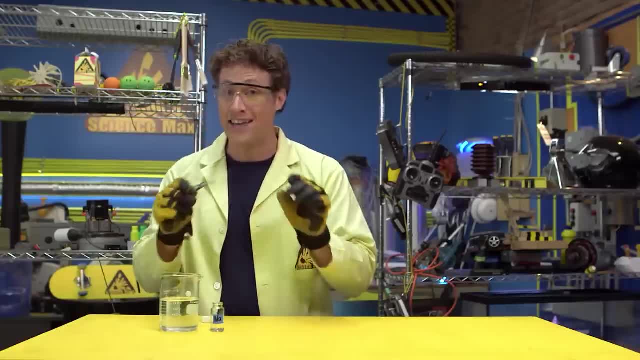 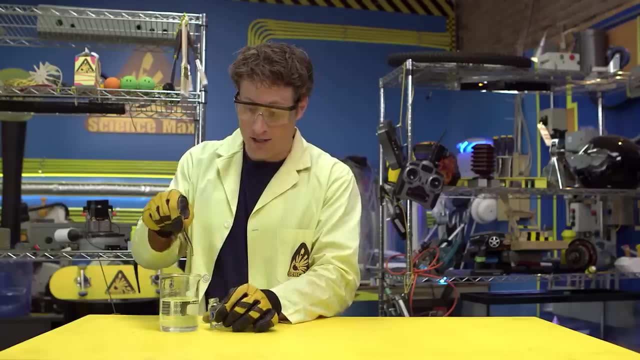 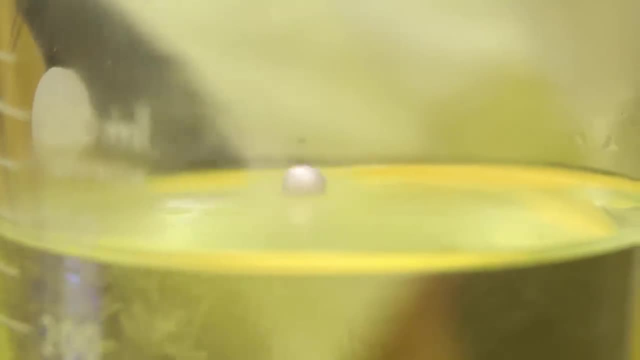 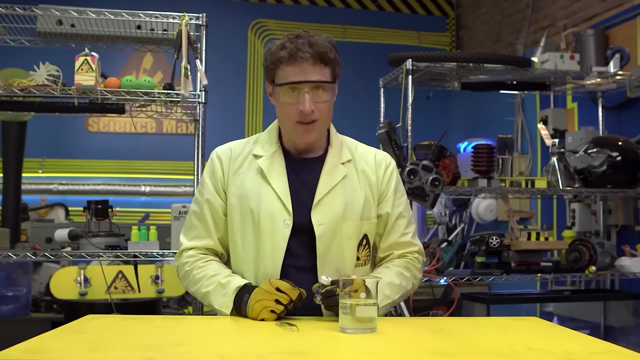 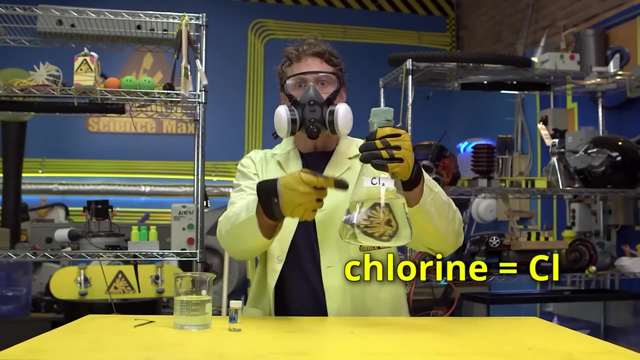 because sodium reacts very strongly with water, even the water in the air or especially the water in my skin. Watch what happens when I drop a sodium tablet into this beaker of water. Very cool and very dangerous. And this is chlorine or Cl. 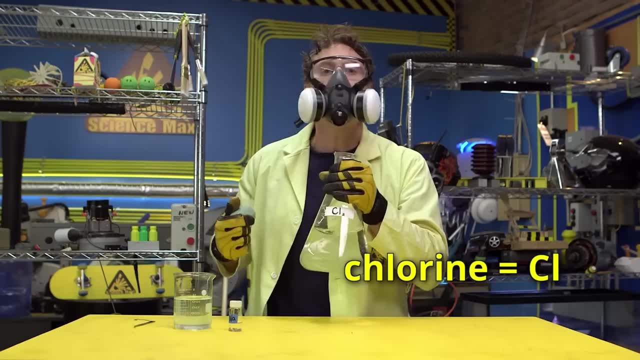 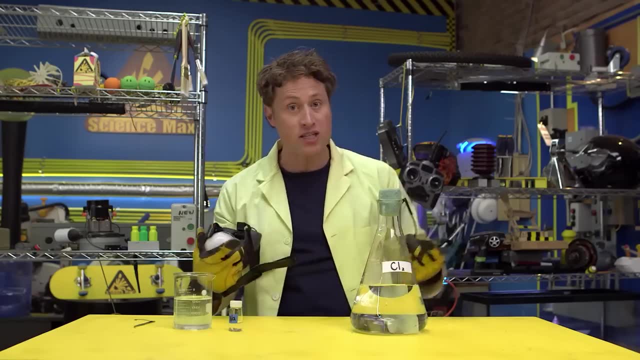 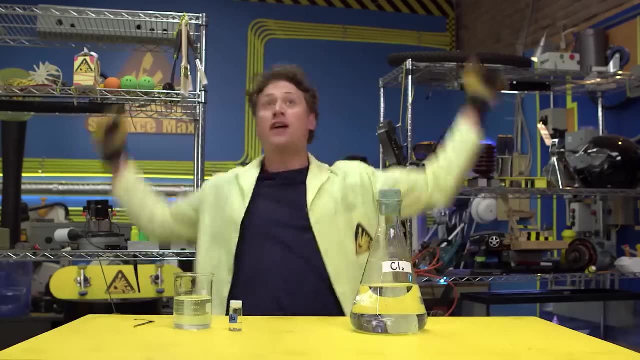 on the periodic table. Chlorine gas is very poisonous. So what happens if we combine these two deadly substances? Do we create some sort of super poison, something more deadly than anything else known to science, that causes fear and chaos in chemistry labs all over the land? 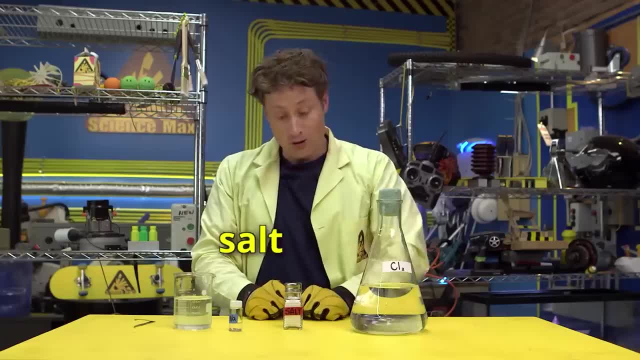 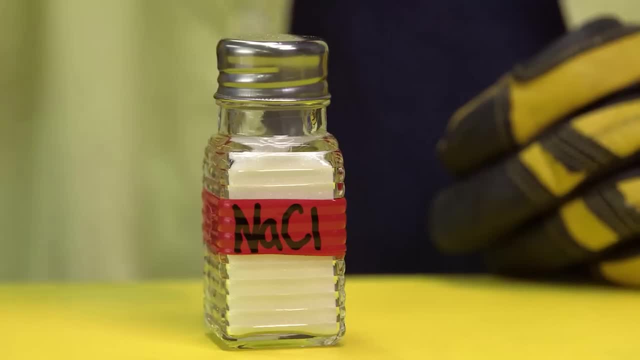 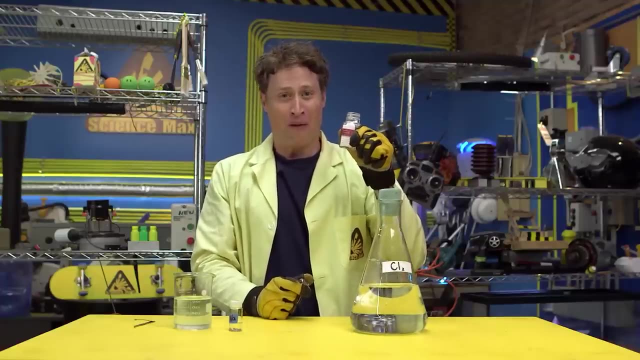 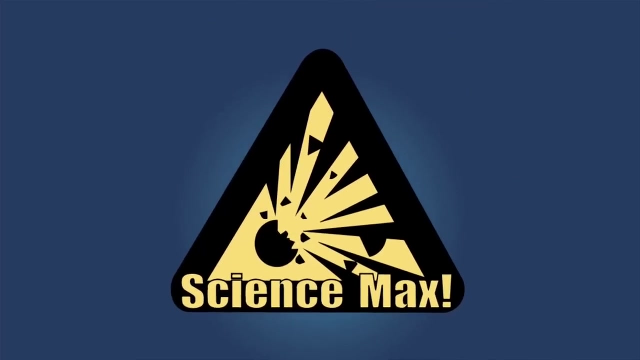 No, we create salt, good old normal table salt. These two substances combine to make Na Cl salt, something completely and totally safe. Come here Sprite. We've gone from vinegar and baking soda to 100% acetic acid in baking soda. 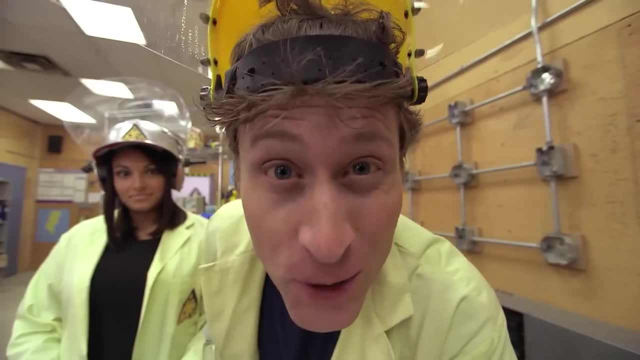 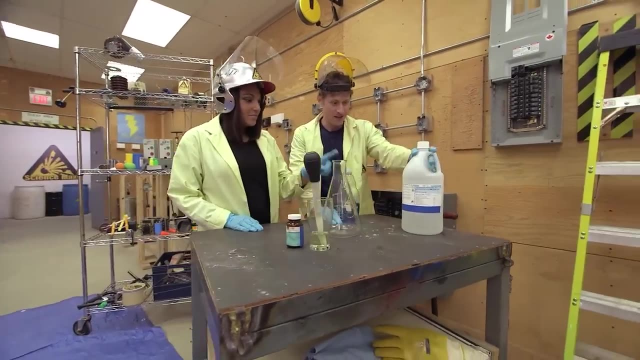 and now we're doing the vinegar and baking soda volcano version three. No longer vinegar and baking soda, No. So what are we using this time? So here we have some hydrogen peroxide. Oh, that's the stuff you use at home to put on a cut right. 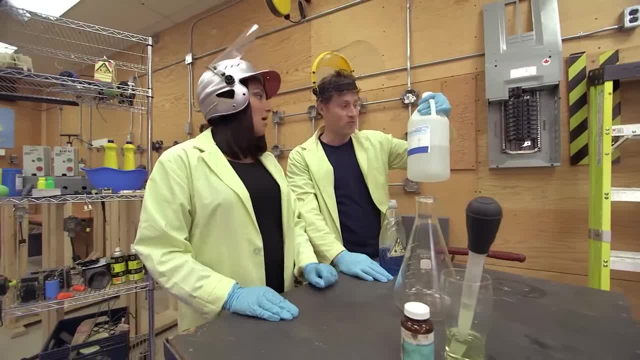 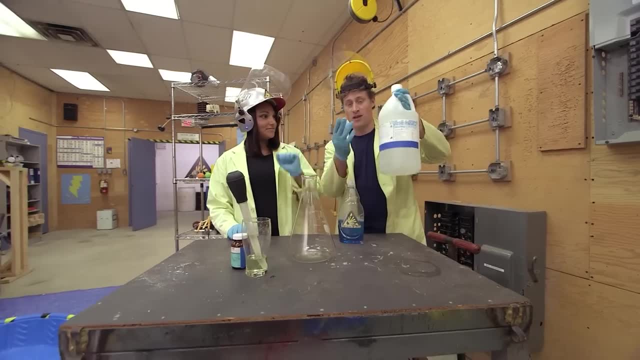 Yeah, but the stuff at home is only 3%, This one's 30.. So much much stronger, 10 times stronger. Yes, And is this more dangerous? It's definitely corrosive, so wear your gloves. Corrosive means it could eat your skin. 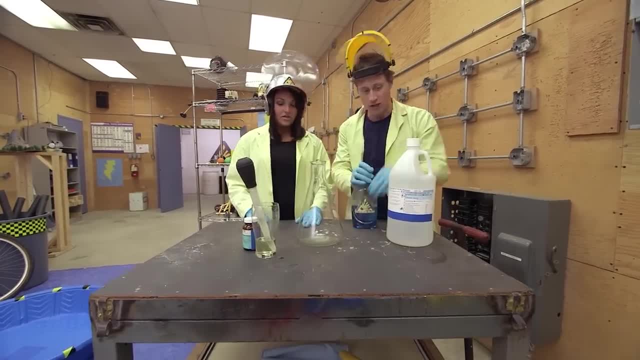 It can burn your skin a little bit, Which is why we're wearing gloves and blast shields. What's going to mix with this? So here we have some potassium iodide, which is a salt, and it's mixed in with some water. 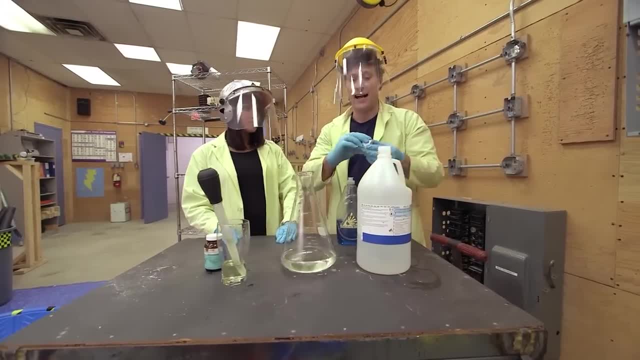 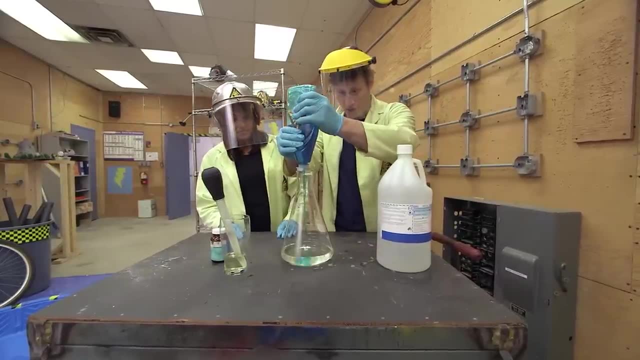 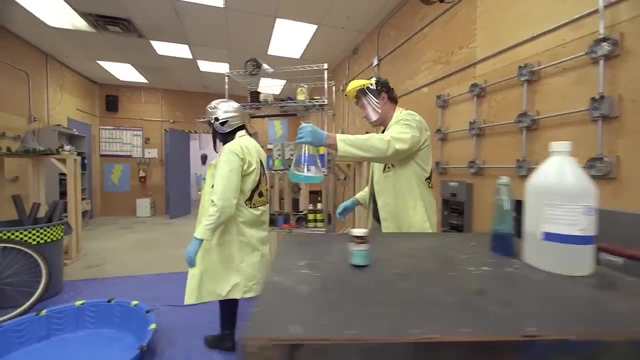 Mm-hmm. And what makes this reaction is the fact that it creates gas, Oxygen gas, Which makes bubbles when you put in dish soap, right, Yep? So one big squirt of dish soap like that, Mix it up. Now we go over to the blast zone. 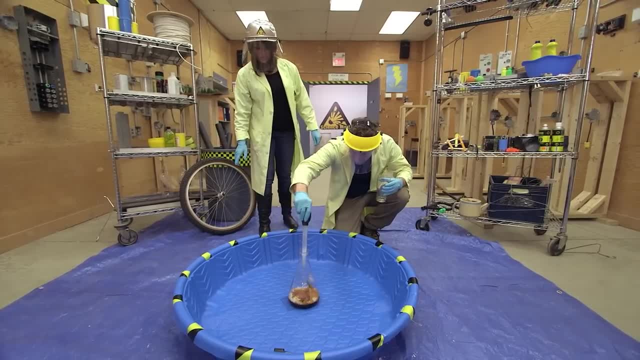 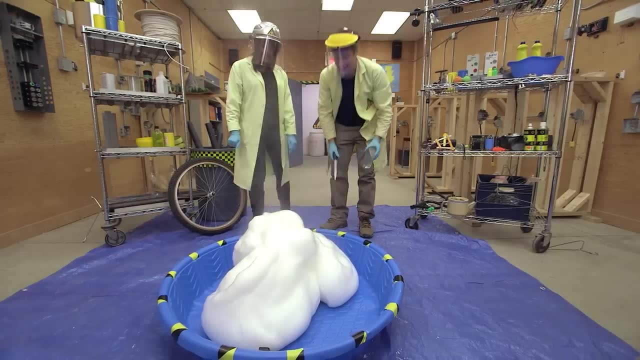 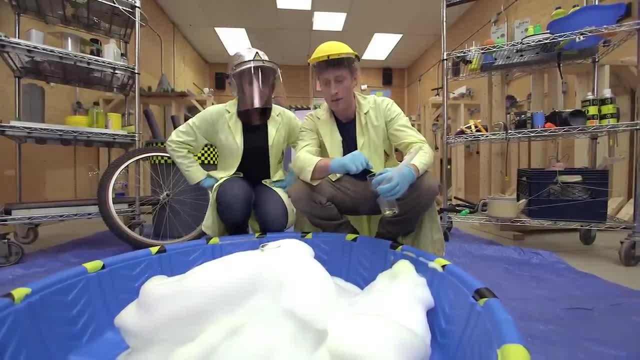 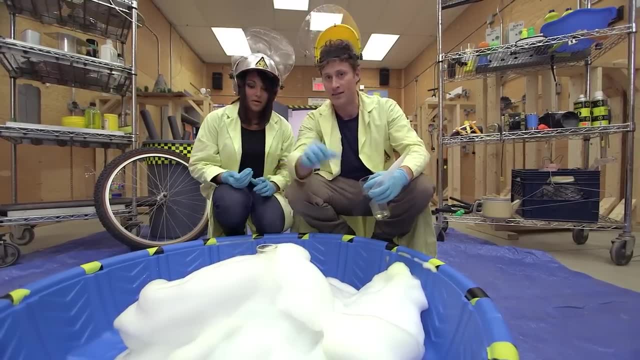 Why is that happening? Well, it is an exothermic reaction, so heat is being generated as the reaction proceeds. Oh, cool, Can we lift our visors now? Yep, Awesome. And what's being released? What's the gas that's coming off here? 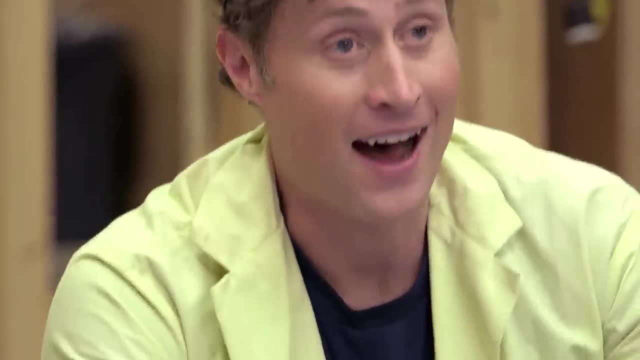 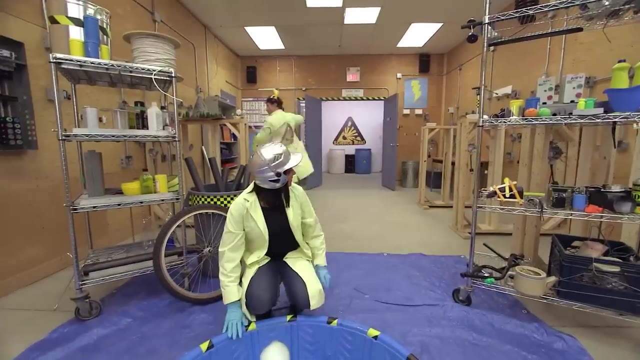 So it's oxygen gas that's being produced- Oxygen. What we want to do is make this even bigger, But first, can we do it again? Sure, Because I have an idea. Hold on, Ha, ha, ha ha. 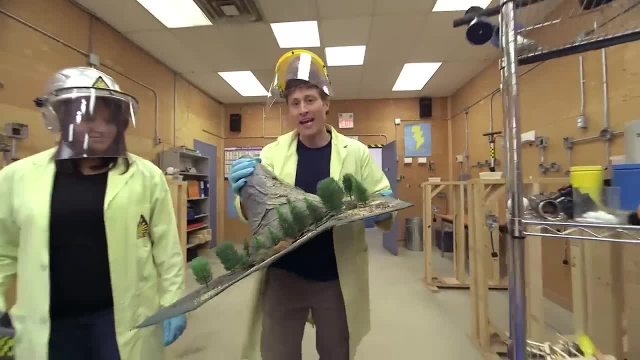 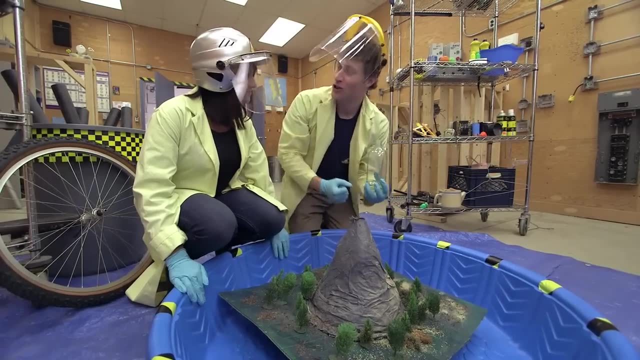 I think we need to do this. We should repurpose our old volcano. What do you think Sounds like a good idea? OK, so if we put it over here, All right. Volcano version 3.5, hydrogen peroxide, potassium iodide. 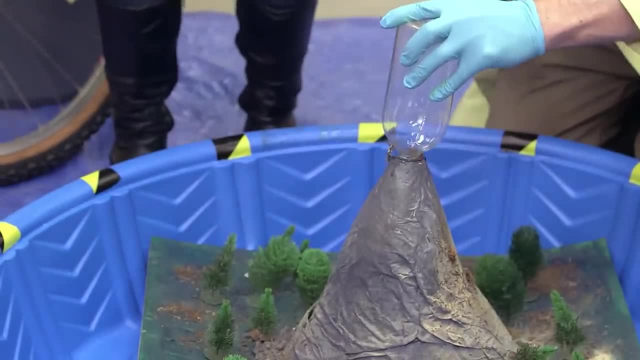 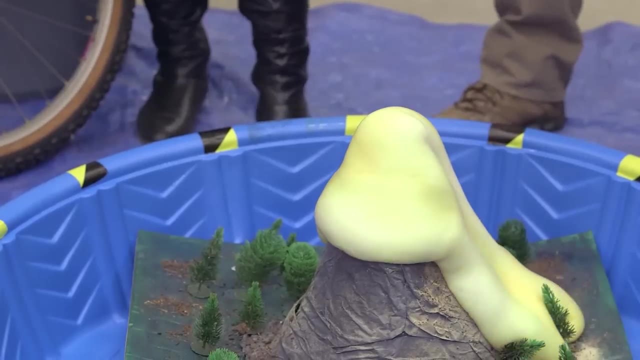 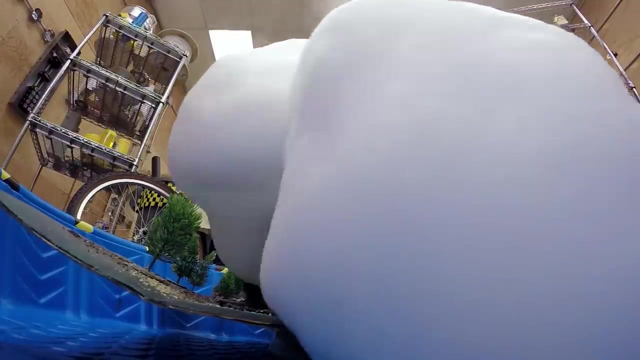 Right, Here we go. Whoa, Oh, Looks like lava. Whoa, Ha, ha, ha, ha ha ha. Look at that. That now that is a big volcano eruption Just covered the town. That is completely the yes. 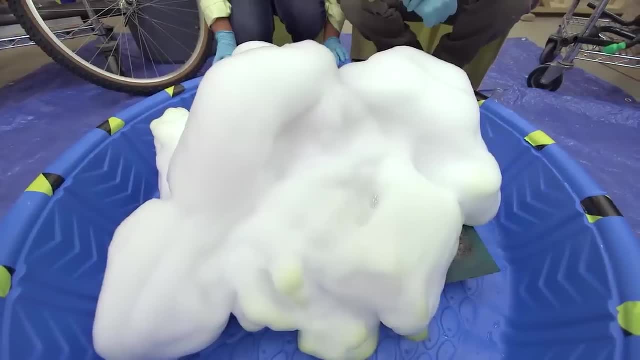 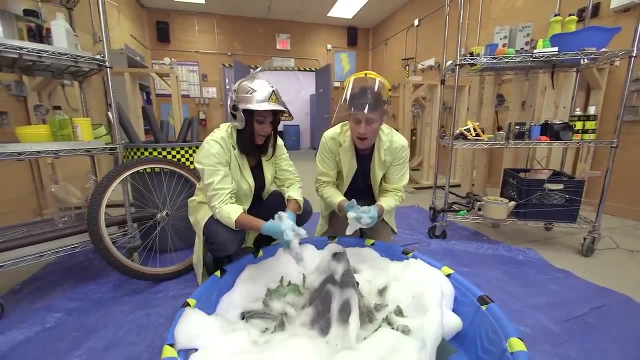 That town is going to be very clean because it's all soap bubbles. It's the cleanest volcano this side of Science, Maxaville. So I still think we can do this bigger, though, right, I agree. Oh, I know What if we use some sort of a tube, like maybe one of these? 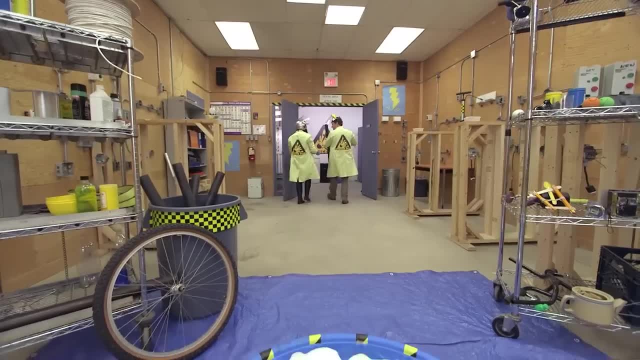 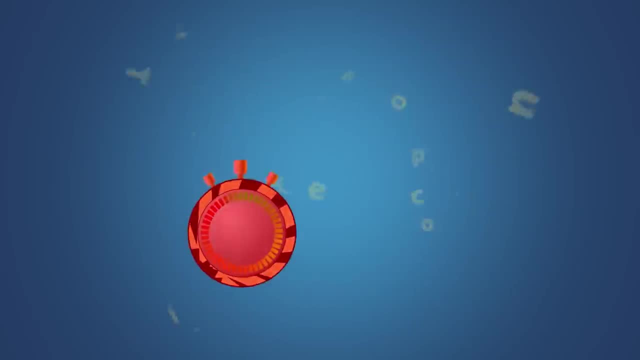 right and then we attach it to like an air compressor. I think you'd get some height, Yeah, and we go aside The atom in 60 seconds. The atom is the smallest unit in a chemical element. Atoms are made of three parts. 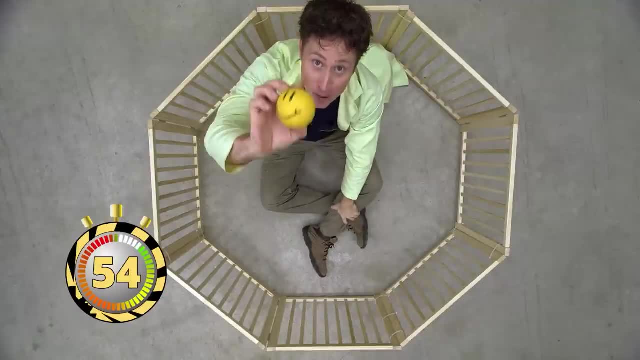 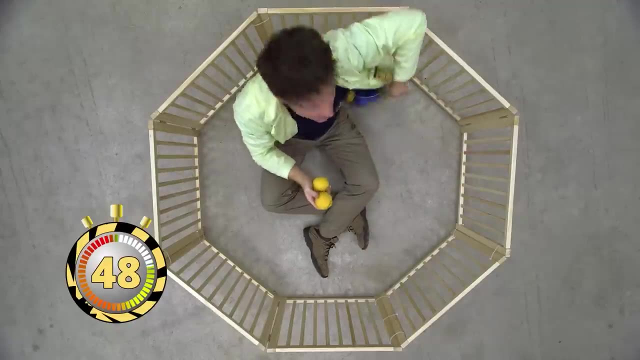 Part number one are these guys protons? They have a positive charge. The number of protons determines the element. One is hydrogen, Two is helium, Three is lithium, and so on. The protons sit in the middle here, which is called the nucleus. 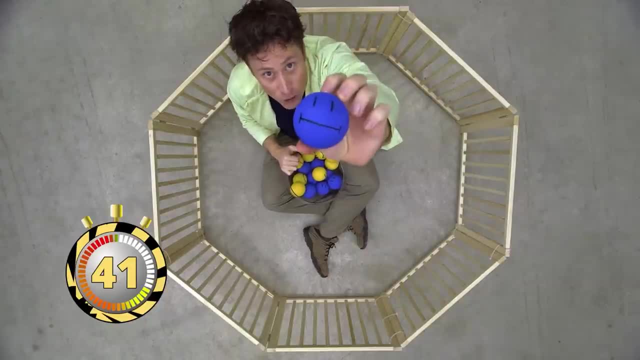 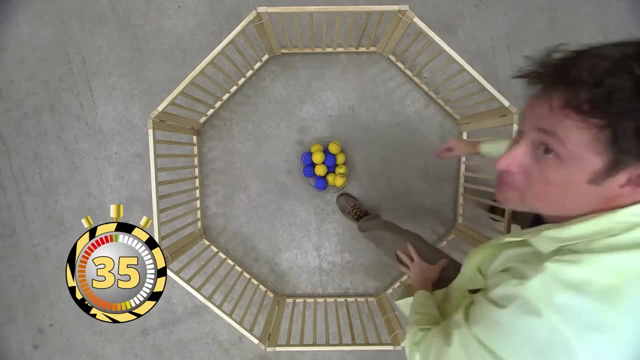 They sit in here with part number two, these guys. They're neutrons and they have a neutral charge. Now I've got eight protons and eight neutrons in this nucleus, making this an atom of oxygen Orbiting around the nucleus. are these tiny guys? 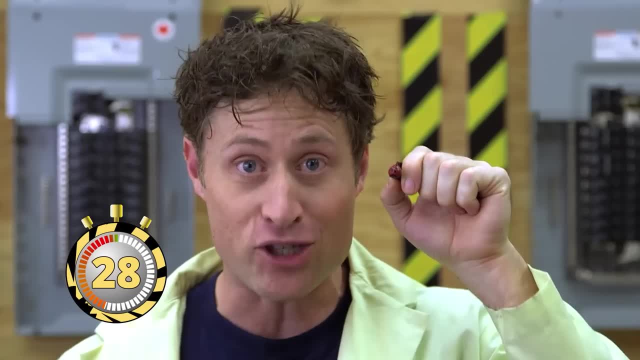 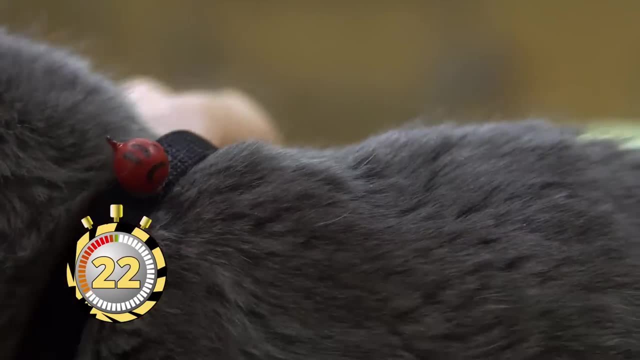 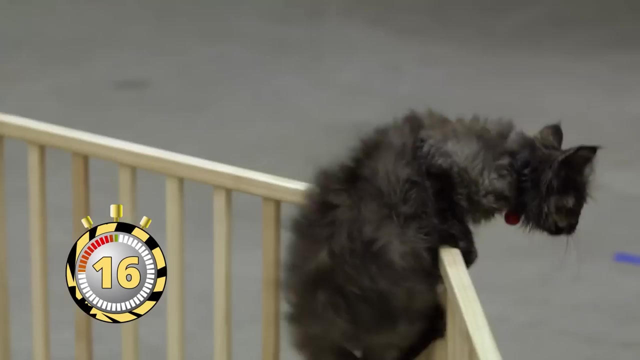 They're electrons and they have a negative charge. I will demonstrate using kittens. Kittens are perfect because, just like electrons, kittens are really small And, just like electrons, kittens move around randomly. You never know. You never know where they're going to be. 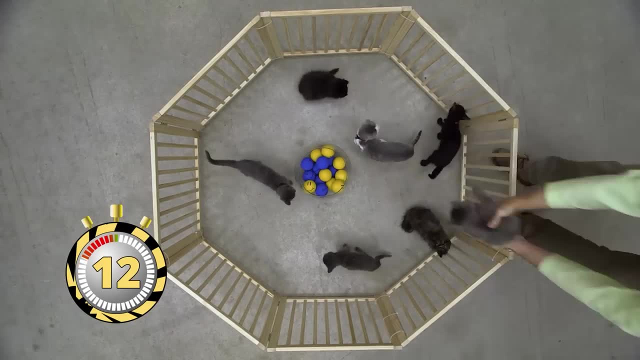 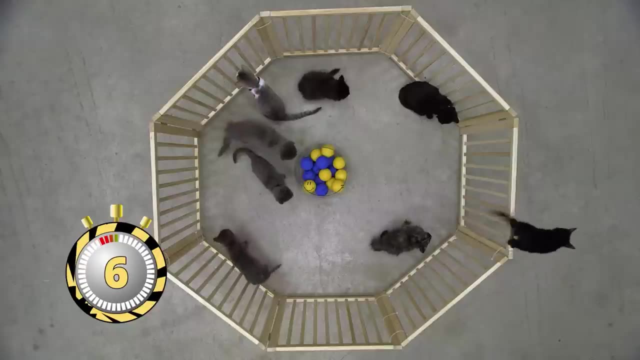 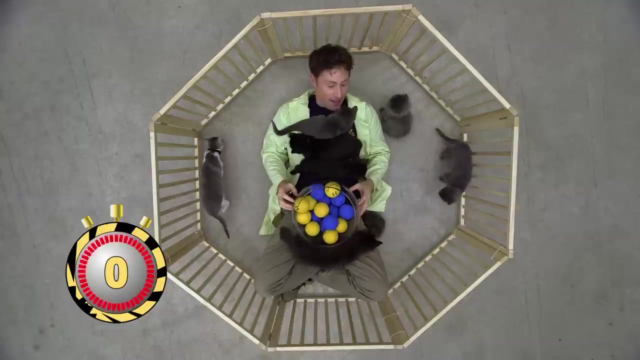 But an oxygen atom should have eight kittens or electrons somewhere inside. These kittens are constantly escaping, But guess what That happens with electrons too. There you go The atom: a nucleus of protons and neutrons surrounded by randomly moving electrons. 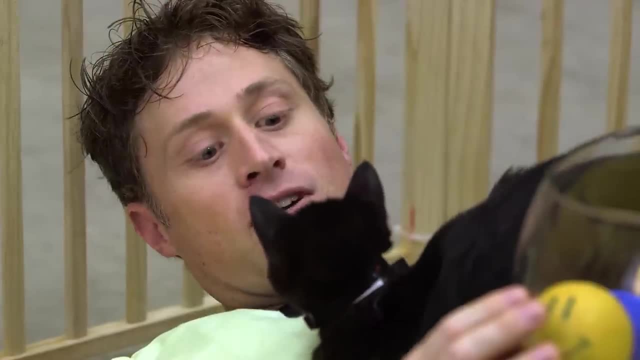 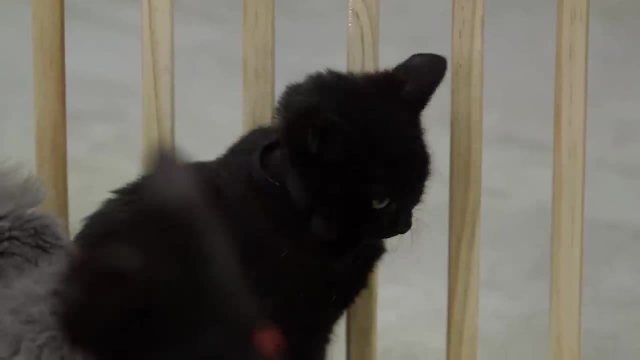 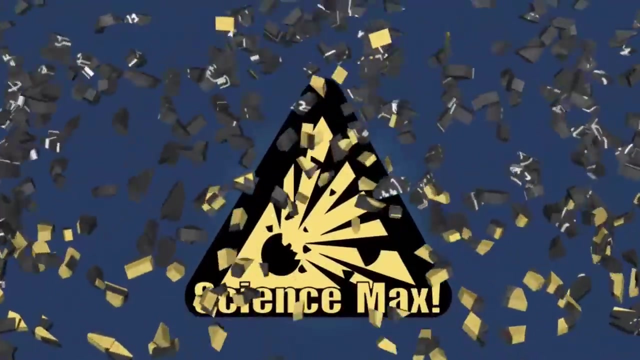 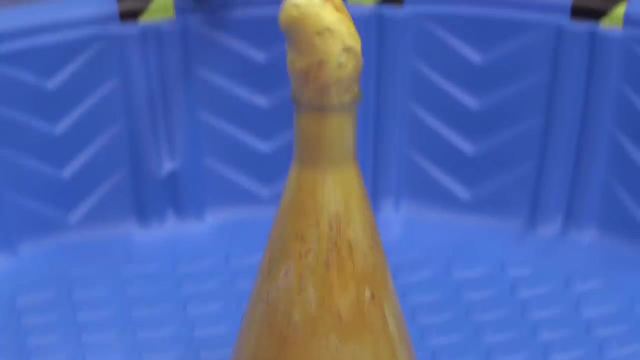 Cutest science ever. How do you guys feel? Did you learn something? Huh, Pause up. Huh, Telly and I have made a bunch of chemical reactions, but in our quest to max things out, we've got a new plan. 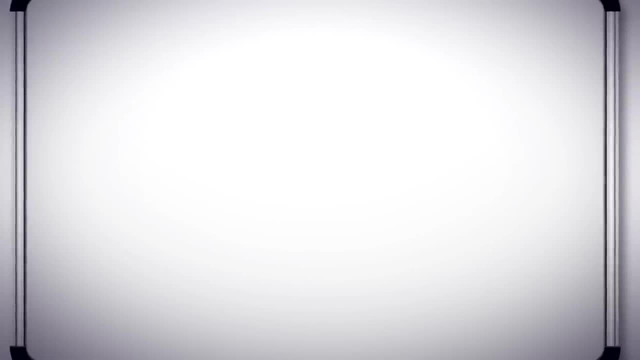 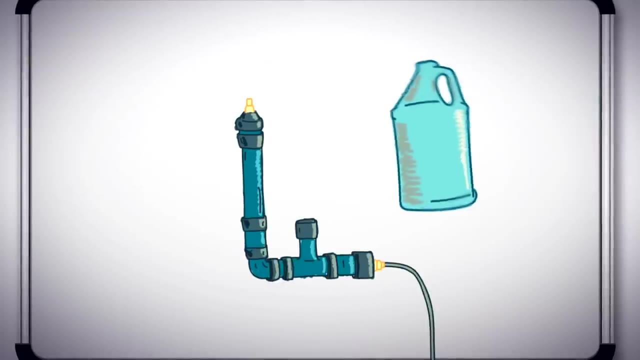 Hydrogen peroxide and potassium iodide create gas. One way to max out the reaction is to contain the gas in something like a tube. We're going to put the hydrogen peroxide in the tube, in the tube first, Then we're going to put in the potassium iodide in the top. 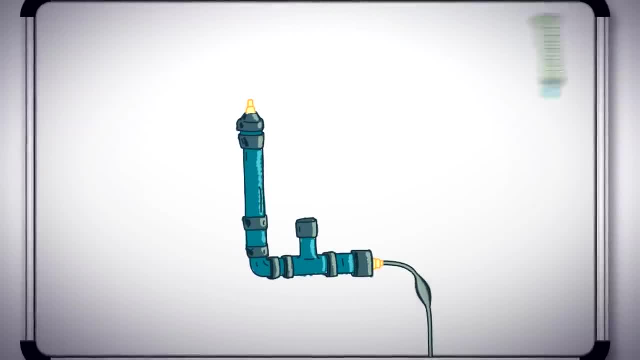 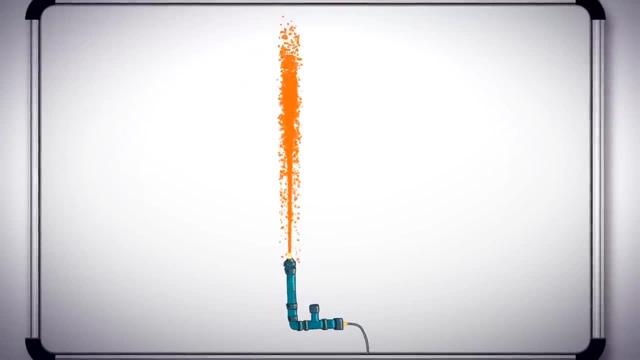 through a one-way valve. Then we're going to pressurize the container. When it finally reacts, it will shoot up through the valve and we'll see how high we can get our stream of bubbles to go. But be warned: capping anything and not letting it escape. 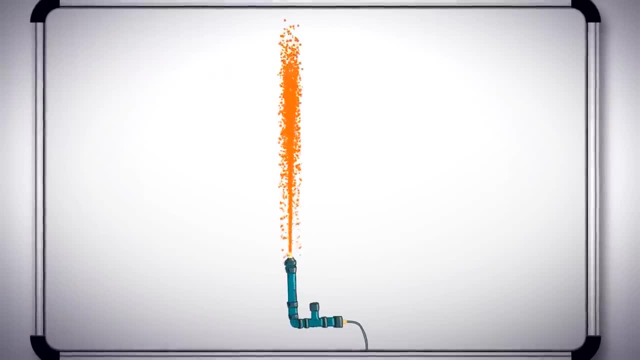 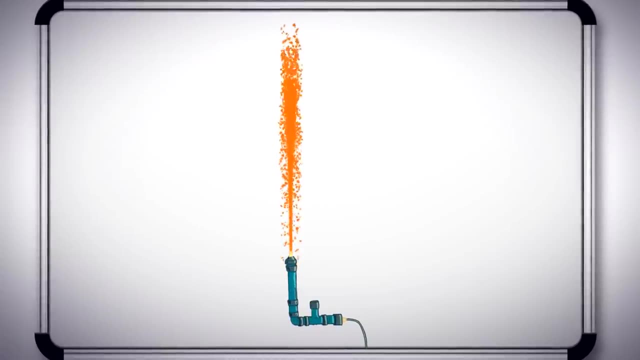 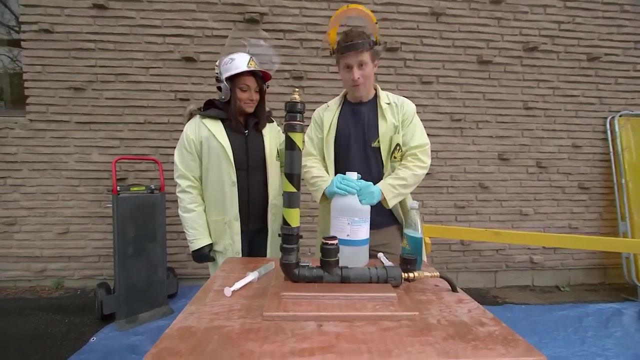 is never a good idea, So we've got a release valve to make sure things work out. This is one of those experiments that's definitely on the list of don't try this at home. Let's go. Vinegar baking soda volcano version four. 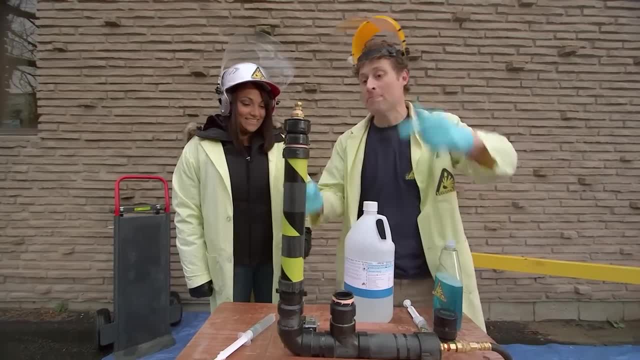 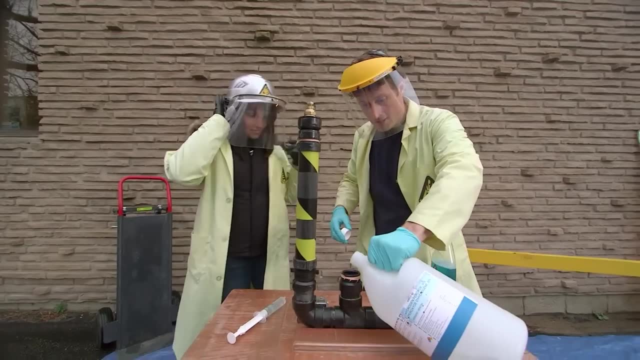 hydrogen peroxide, potassium iodide, And what we're going to do this time is we're going to put it in this tube. Hydrogen peroxide goes in here And we've got. Talena, do you have the potassium iodide? 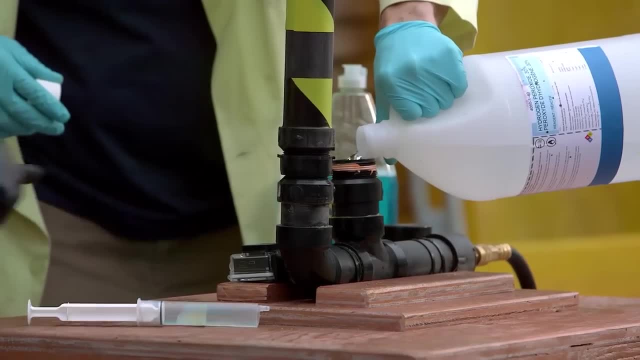 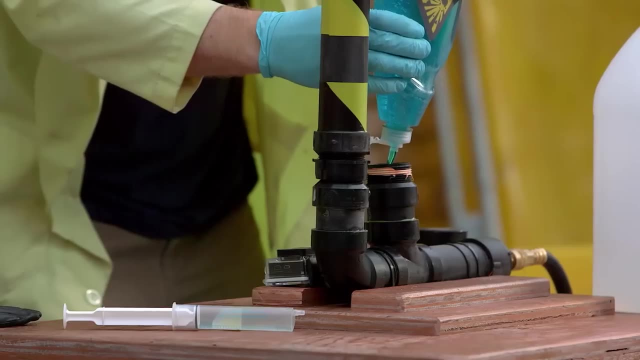 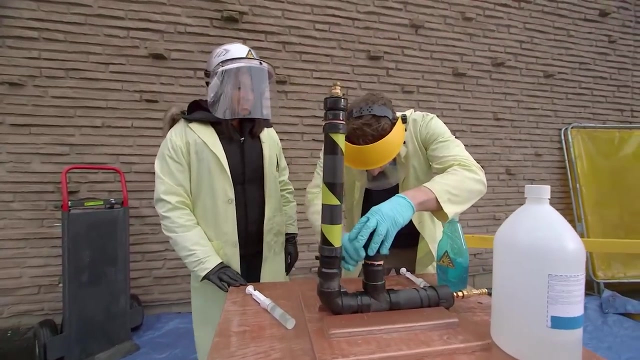 in syringes. Yeah, two syringes full. Two syringes full, That's good. And then soap- Good amount of soap in there. And so what we're going to do is we're going to close this off and tighten it up. 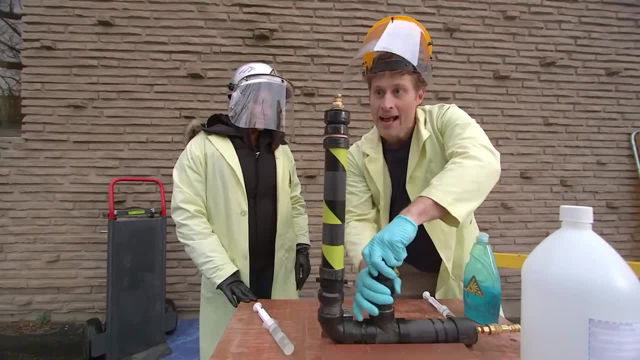 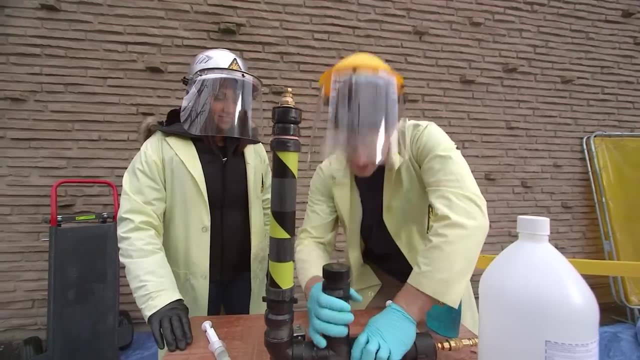 And then we're going to pressurize the whole system, And then we're going to add the potassium iodide And it's going to be spectacular, we hope. OK, that's on tight. This is all good Putting this down here. 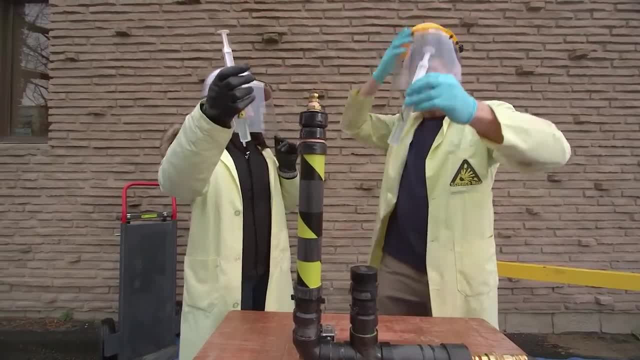 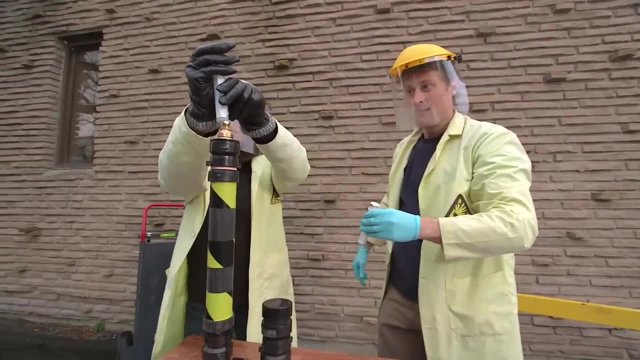 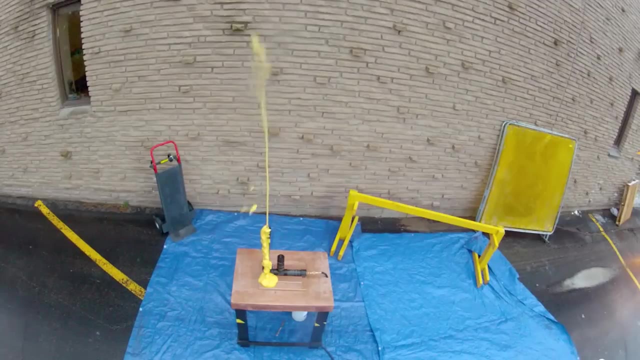 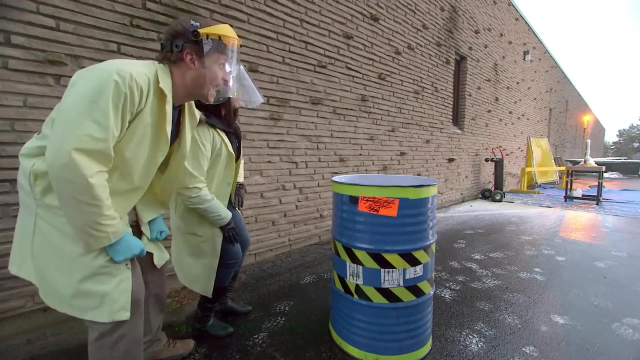 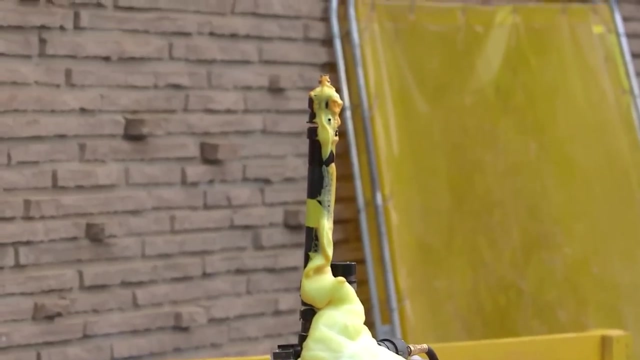 And potassium iodide goes in here, puts down Ready One, two, three go, And we back away slowly. Whoa, Whoa. Yeah, that's what I'm talking about. OK, Check it out, Whoo. 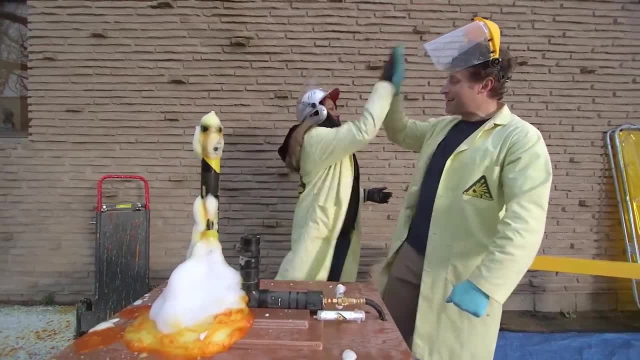 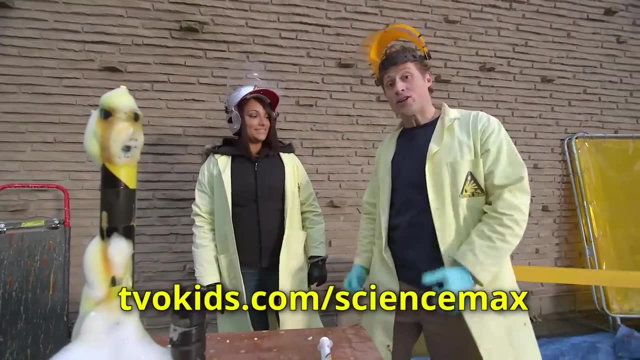 All right, there you go. Vinegar and baking soda: volcano maxed out. Thank you, Talena, That was great. If you guys want any instructions for the stuff that we've done today, they're all on the website And thank you very much for watching Science Max Experiments. 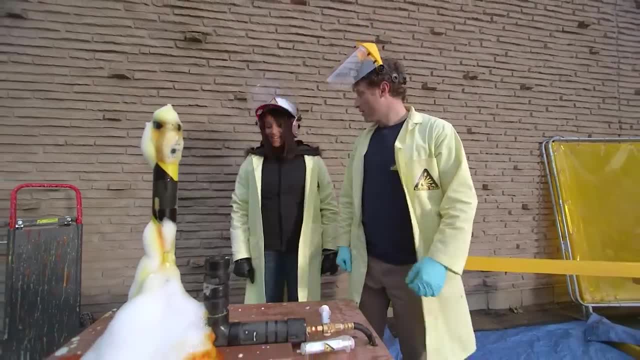 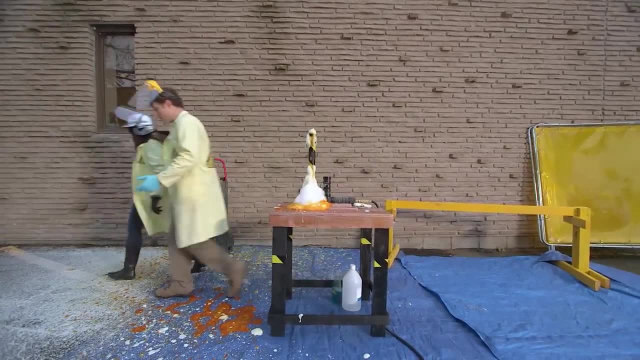 at Large. We kind of need to clean up a lot, don't we? Yeah, We have out here, we have the other room. So tell you what you get: a mop, I will get the hose and a wheelbarrow for the sun. 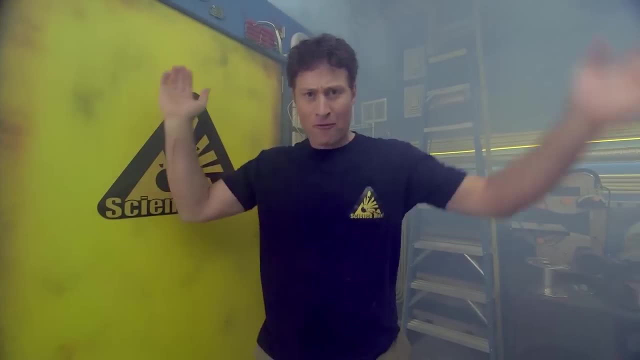 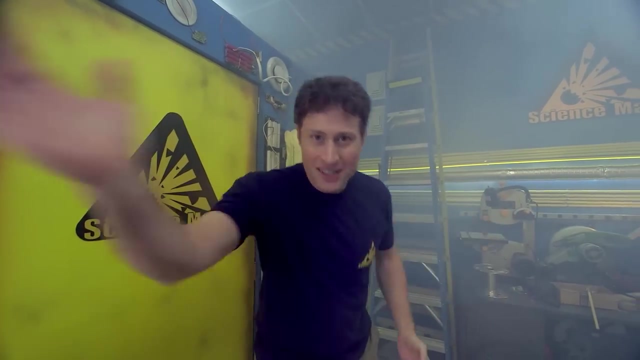 Greetings Science Max. Yeah, I'm Phil McCordick. I think I overdid it with the fog machine. This is Science Max: Experiments at Large. Can you even see me? Let's go over here. Today we're talking about states of matter. 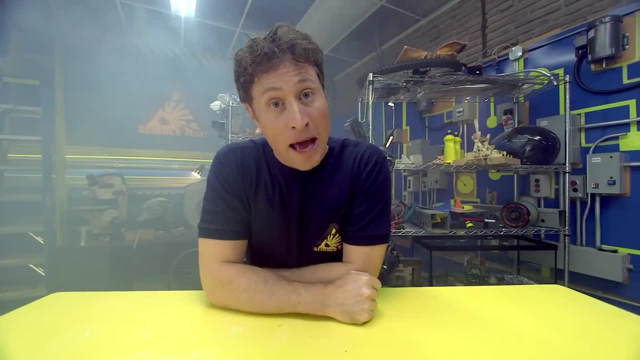 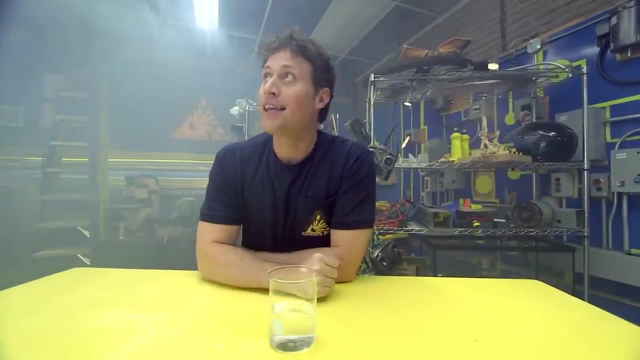 Now there are three main states of matter: Solid, like this table Liquid, like the water in this beaker. And gas. Yes, Thank you, And we're also going to be looking at the things that kind of go in between. 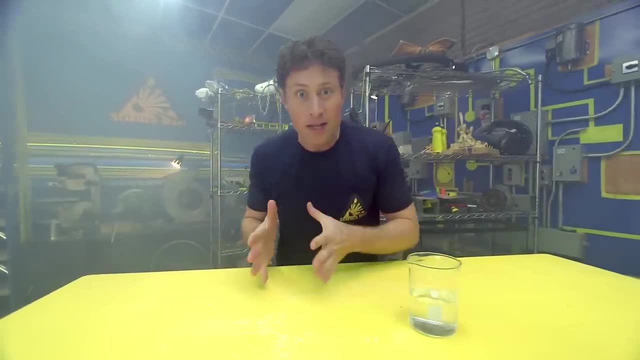 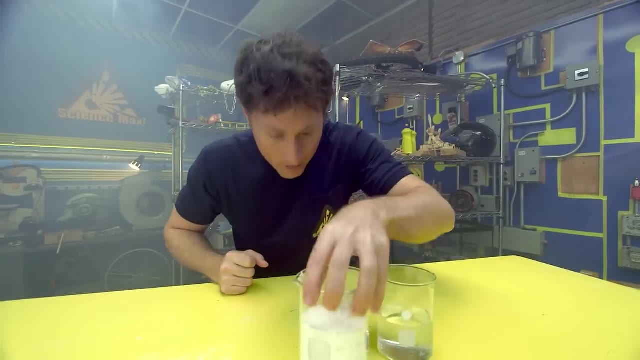 Things that are sometimes solid, sometimes liquid. So let's get started. Liquid, like cornstarch mud, which is very easy to make. All you need is water and cornstarch, which you can get at the grocery store. Mix it up however much you want. 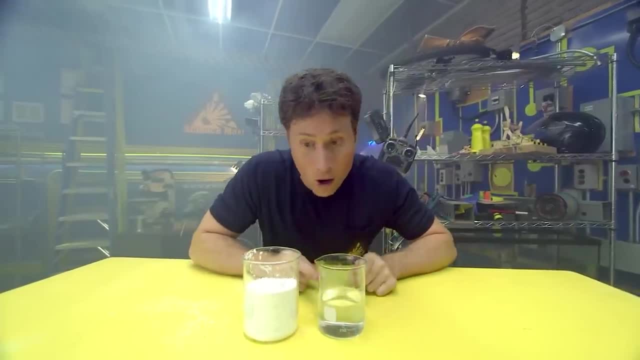 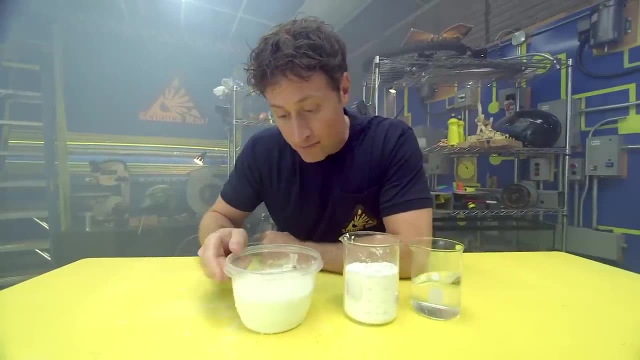 Just remember: two parts cornstarch to one part water. Twice as much of this than you have of that. Very easy. Mix it up and you get cornstarch mud which sort of seems like a liquid unless you hit it. 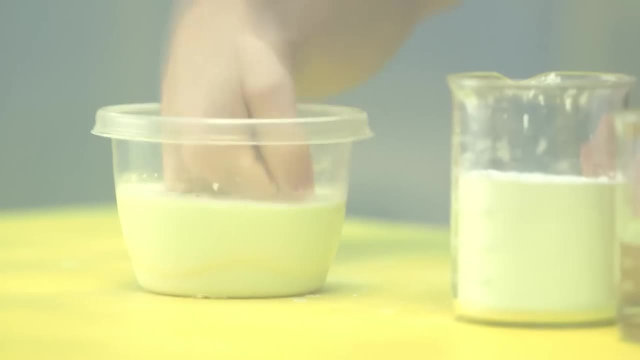 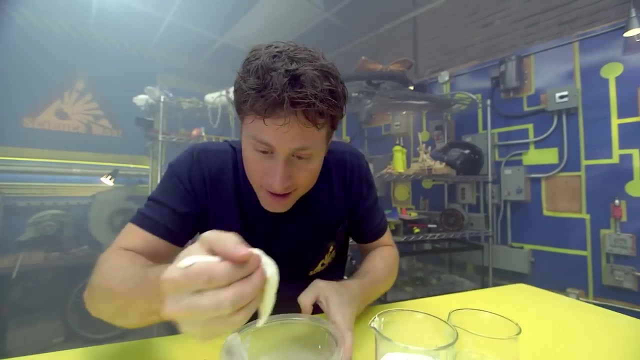 And then it becomes solid. But if I pour it It's a liquid. Even if I hold it in my hand and I hit it really fast, it turns into a ball, and it will stay in a ball as long as I keep hitting it or squeezing it. 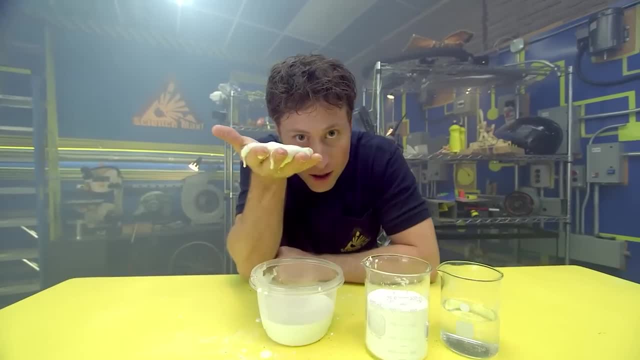 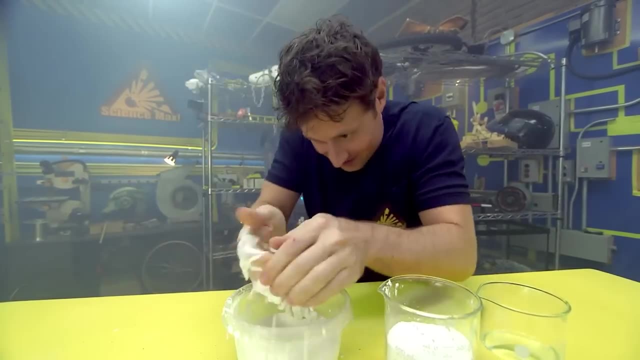 But as soon as I stop, it turns into a liquid again. Now we're going to max this out. We'll go through the portal and learn more about solids, liquids and gases. Yeah right, That's why I'm making this video. 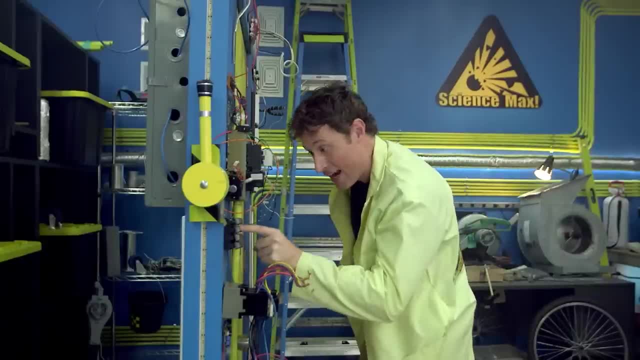 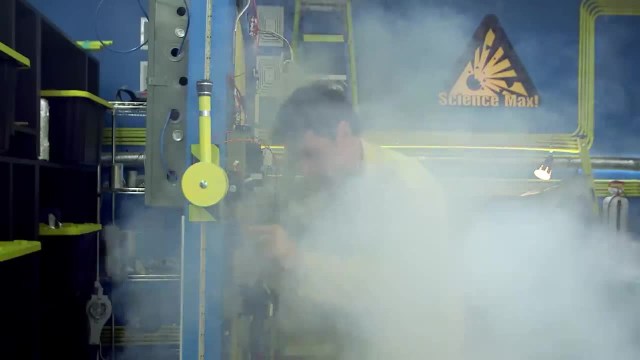 So let's get started. All right, That's why I'm going to the Center for Skills Development and Training. Oh, no wait, That's the code for the fog machine. Wait, Stop, Stop. It seems to be stuck. 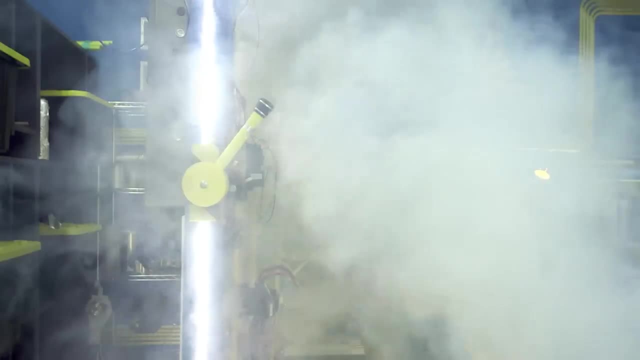 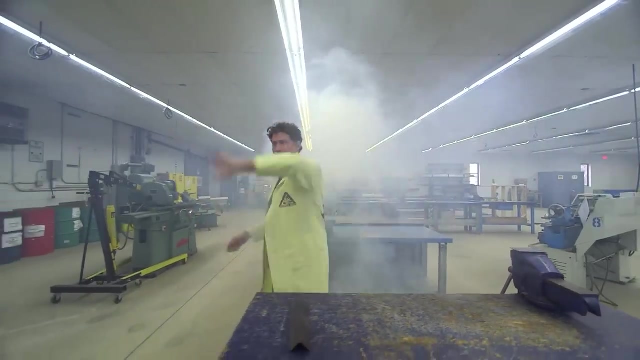 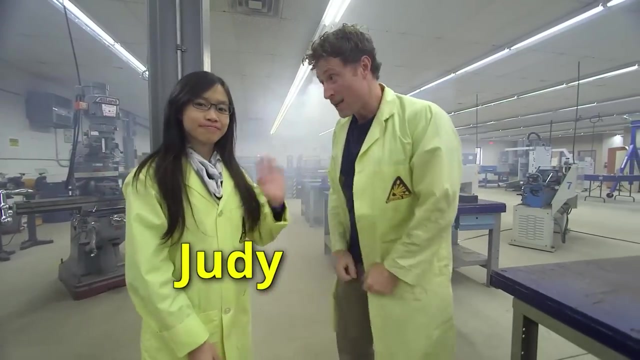 Oh, never mind. Never mind, I'll fix it later, Right? Hey Judy? how are you? Hi Phil, how are you? Good, Judy is going for her PhD in chemistry, right? Yes, So that means you can explain cornstarch mud to me. 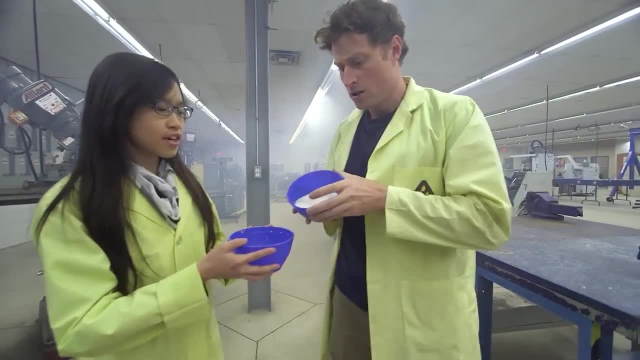 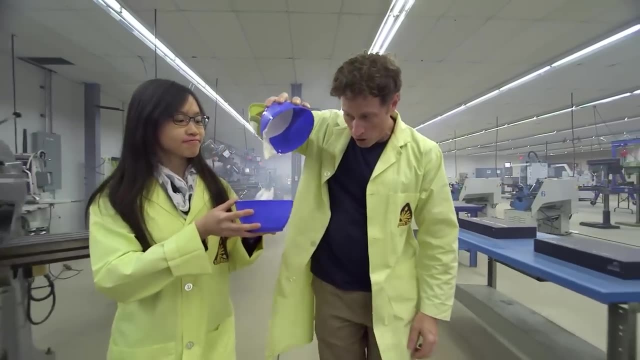 Now, is this a solid or is it a liquid? Well, it kind of has properties of both. It's called a non-Newtonian fluid, So that makes it a liquid. A liquid, Well, I mean it pours like a liquid. 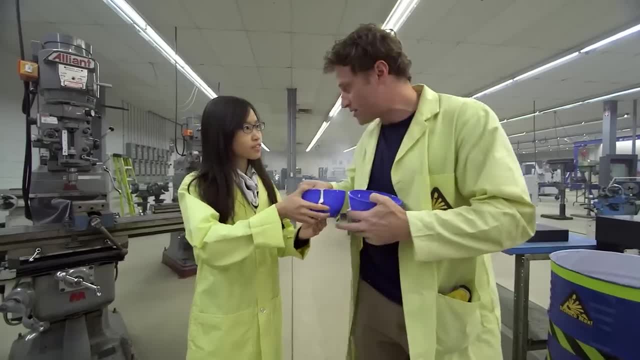 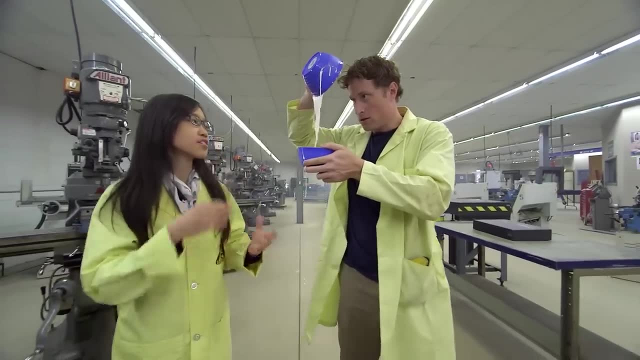 but when you hit it it's a solid. So why does it turn solid when you hit it? So, when you're pouring it, the particles are still far apart, So they can't interact with each other, and so they stay a liquid. 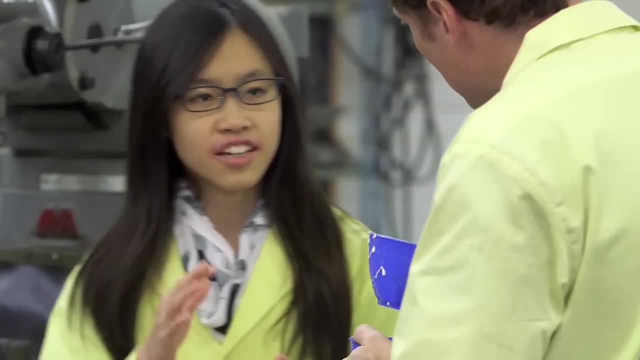 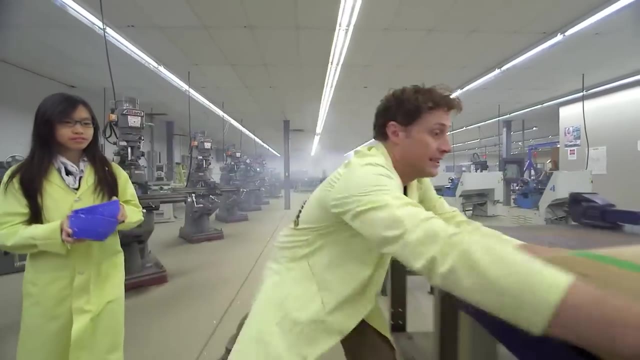 But when you're hitting it, you're jamming the particles together and they line up to become a solid. Now, does it still work the same way? if we have a lot more of it, It should. Great, because I've got this 20 kilogram bag of cornstarch. 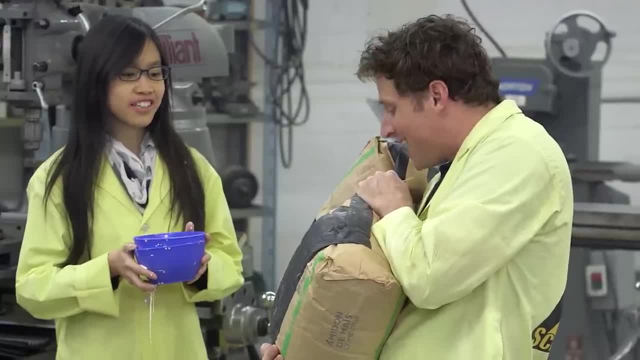 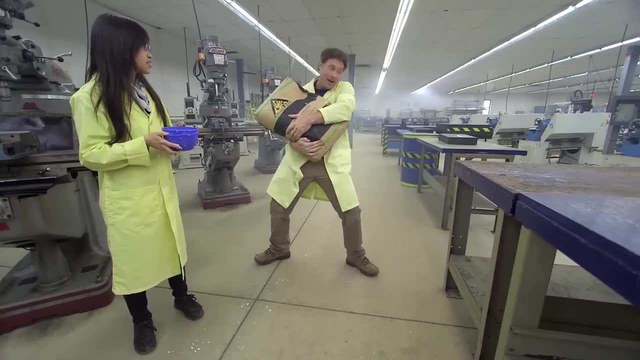 and I have 34 more of them. Wow, that's a lot, But I think you'll need a much bigger container, Much bigger container. great, I got some wood over there. Why don't you go? and I'll follow you. 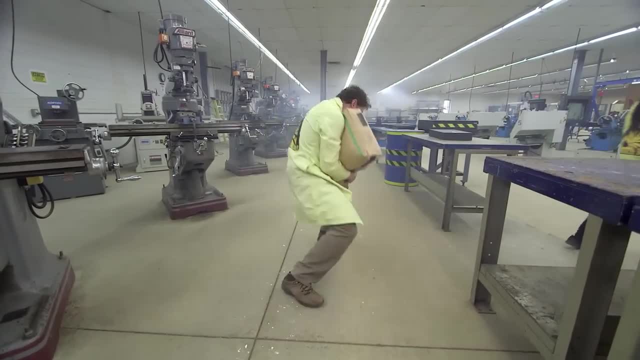 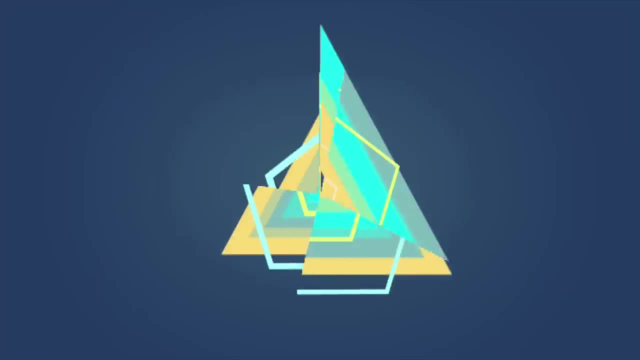 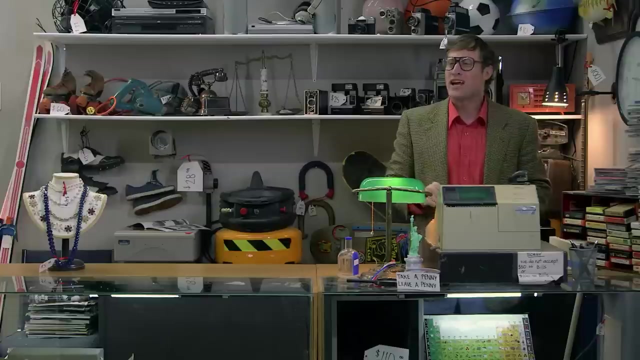 I'll follow you, I'm coming, I'm coming. Oh ugh, Yeah, thanks, Ramona, And give me one of them fizzy drinks, Not too fizzy, just sort of medium fizzy. Thanks a lot. 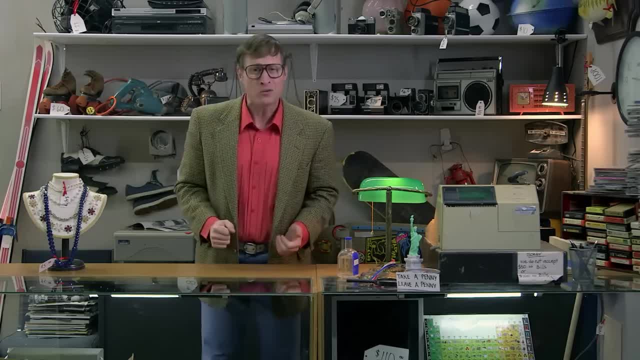 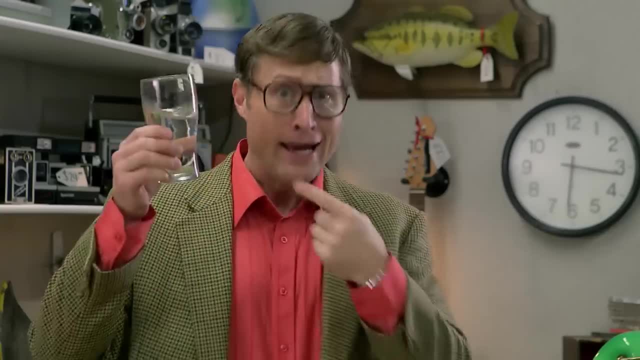 Hello, do you have trouble knowing what is a solid, liquid or gas? Are you confused by jello? I mean, which is it? Is it a solid or is it a liquid? Water is a liquid, but what about when it's ice? 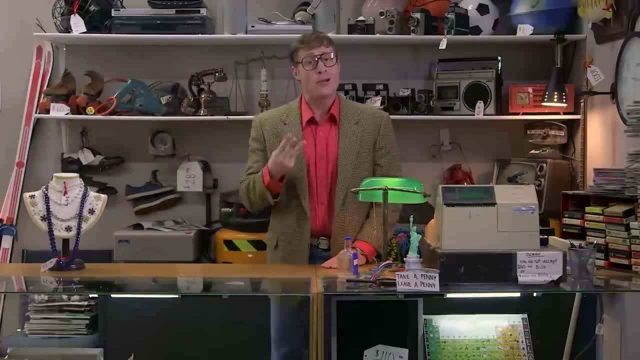 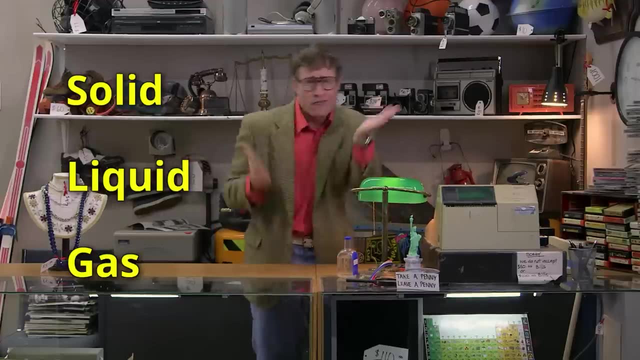 Well, you've got to know your state of matter. There are three main states of matter: solid, liquid and gas- And there are three rules that you need to figure out, which one of them is which Does it flow? Does it fit the shape of its container? 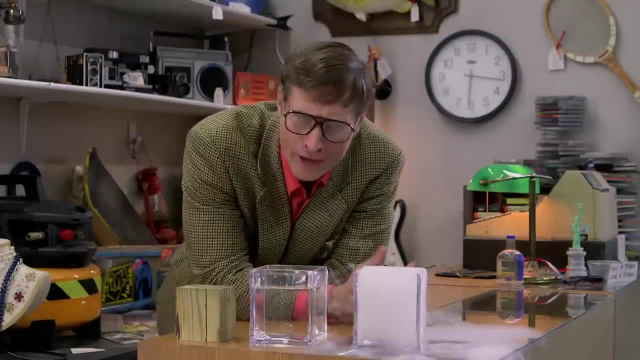 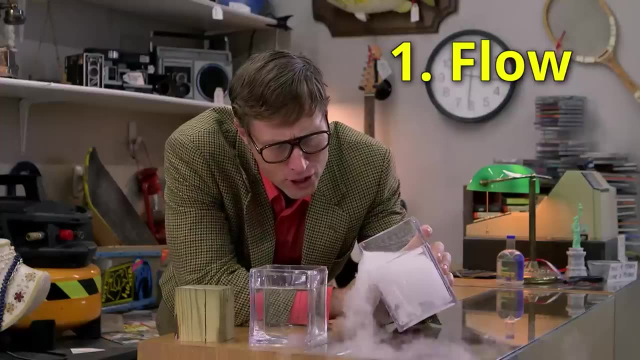 And can you squeeze it? Rule number one: does it flow? Solid liquid gas? Here's a guess. does it flow? Do the particles pour over each other and cascade down? Yeah, yeah, they do. Does the liquid flow? 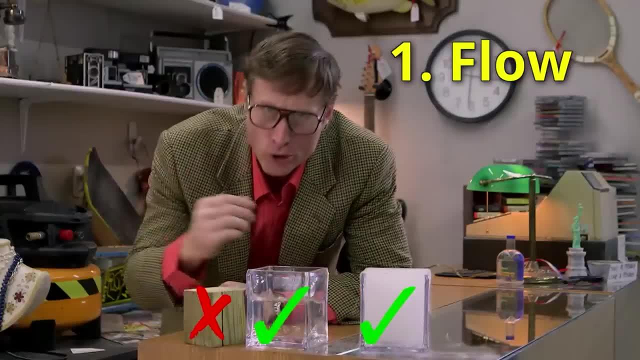 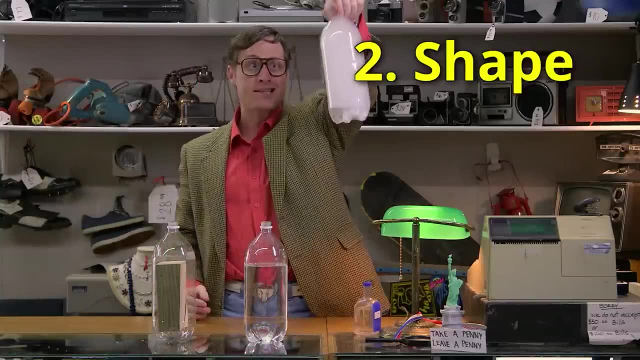 Yeah, Yeah, it does Does a solid Nope. Rule number two: what happens when you put it in a container? Does it take the shape of the container? Gases take the shape of the container. Liquids takes the shape of the container. 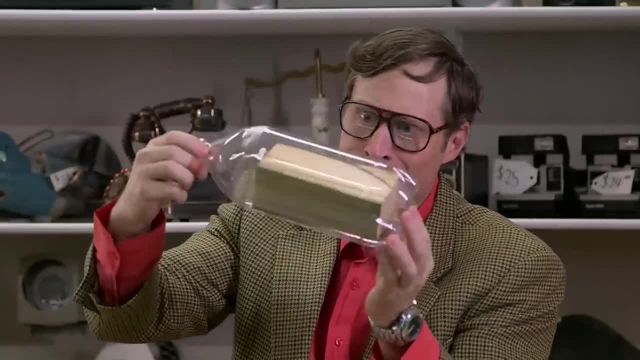 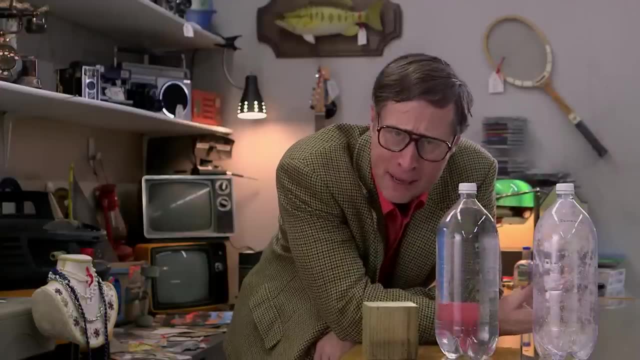 Solids do not take the shape of their container. No, I know what you're thinking. You're thinking I get the whole pouring and taking the shape of the container. but come on Liquids and gases. they do both of those things. 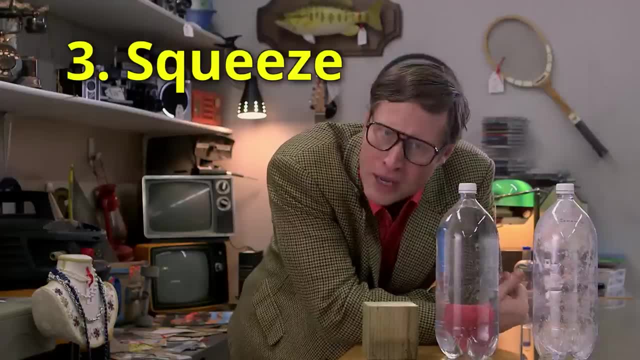 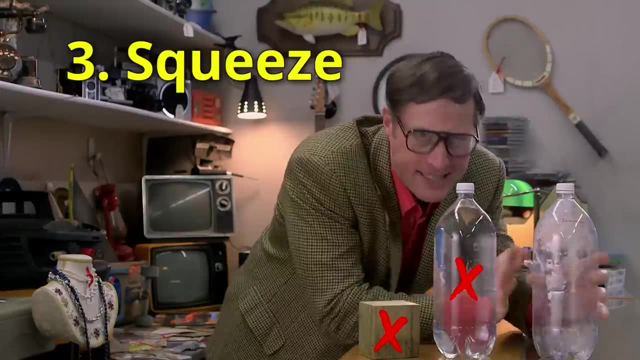 Well, it all comes down to rules. Rule number three: can you squeeze it Now? solids: you can't really squeeze them. Liquids: you can't really squeeze them. Gases: ha-ha bam, you can squeeze them. 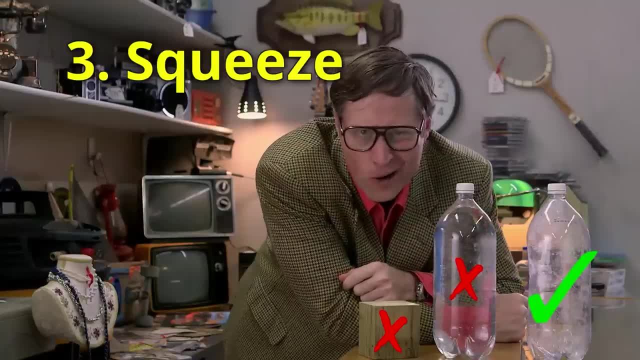 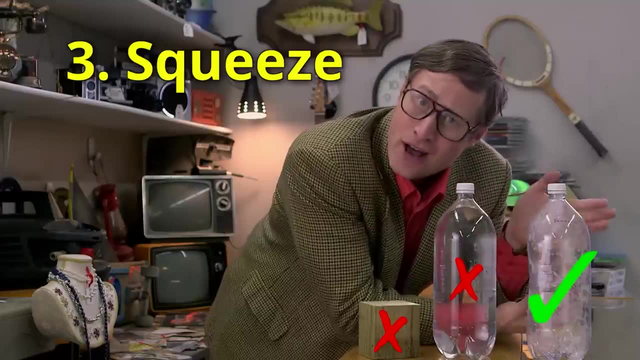 You see, gases compress Liquids and solids. they don't really compress very well. The other difference between gases and liquids is gases will take the shape and the volume of the container they're put in. Liquids don't do that. So there you go. 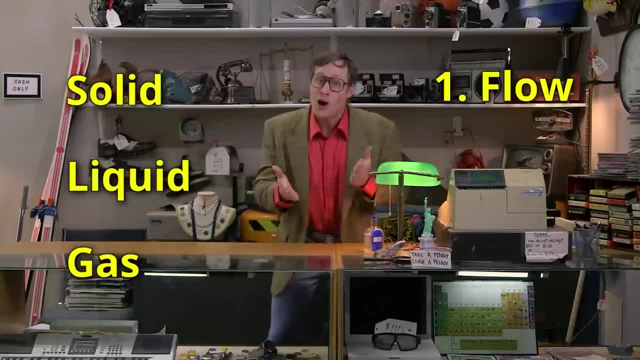 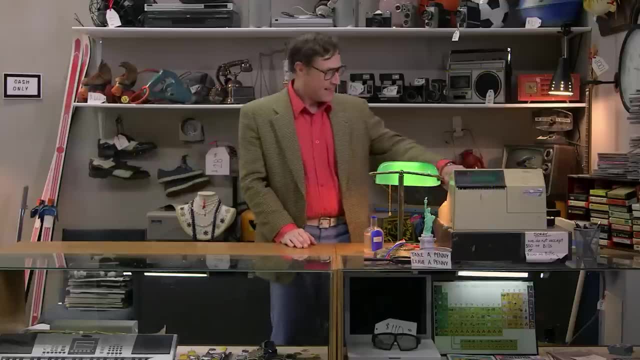 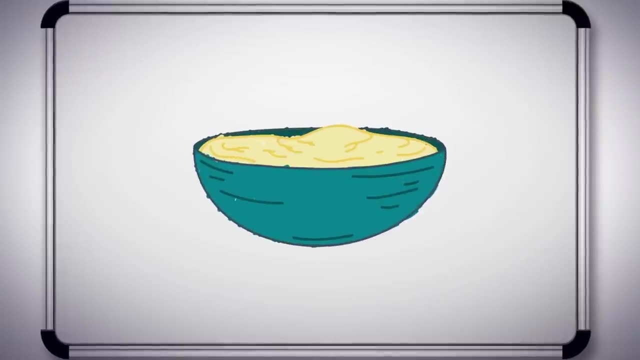 Solid liquid gas And the rules. does it flow? Does it take the shape of the container And can you squeeze it? Now you know your states of matter. That'll be $6.50, cash only. So what is cornstarch mud and how does it work? 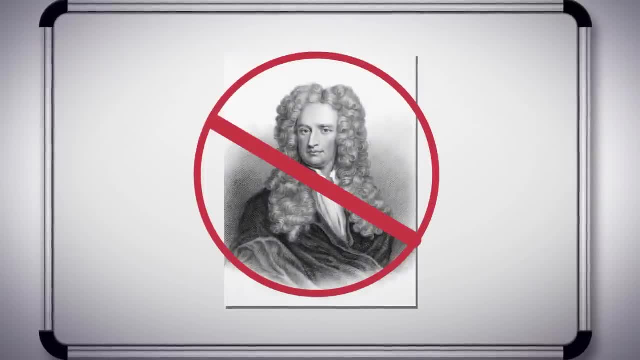 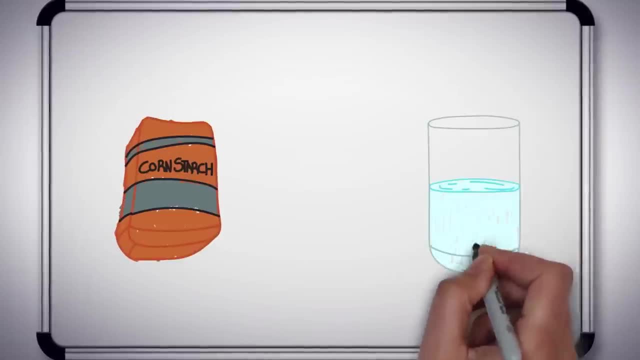 Well, cornstarch mud is a non-Newtonian fluid, which means it behaves differently than you or Newton would expect. Here's cornstarch and here's water. Cornstarch is made up of large blocky molecules like this: 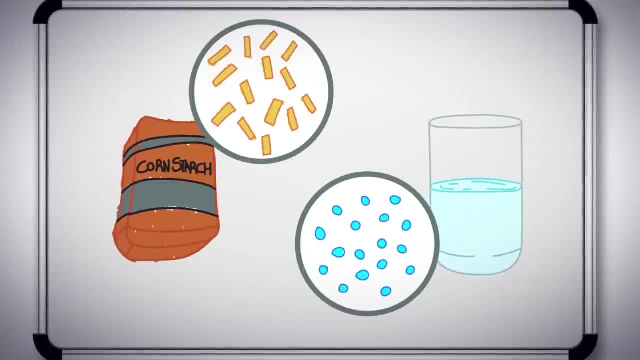 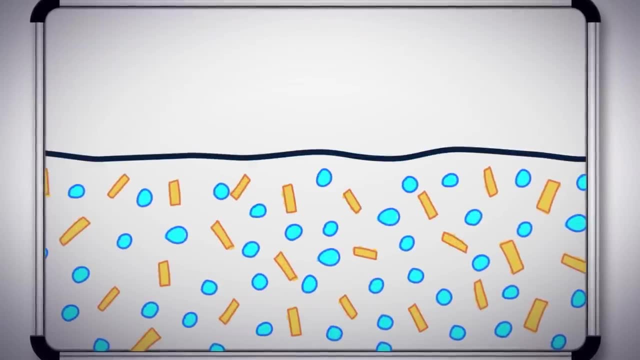 Water is made up of much smaller, rounder molecules like this. When you put them together, it looks something like this: It all has to do with how the molecules slide past each other When you put light pressure or slow pressure on the mud. 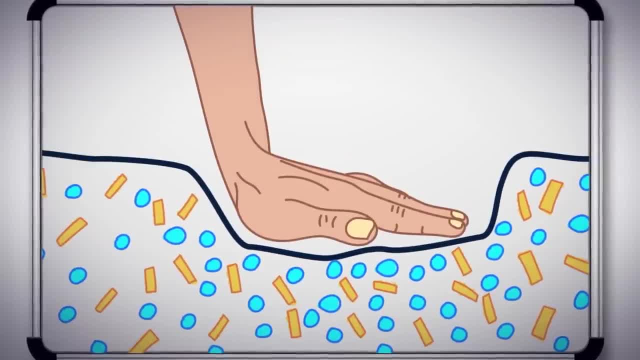 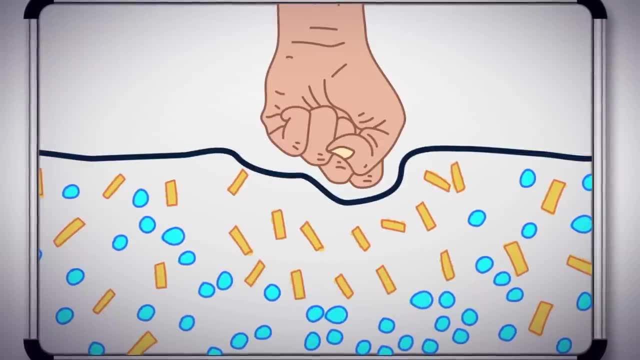 the water molecules and cornstarch molecules have time to shift out of the way, But when you put a sudden pressure on it, the water molecules squirt out of the way, but the cornstarch molecules don't have enough time, So you get a section that's nearly all cornstarch. 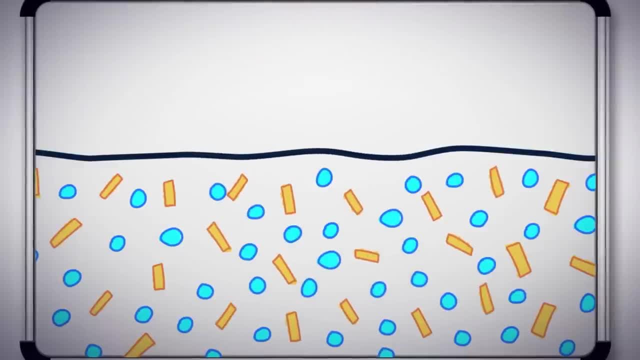 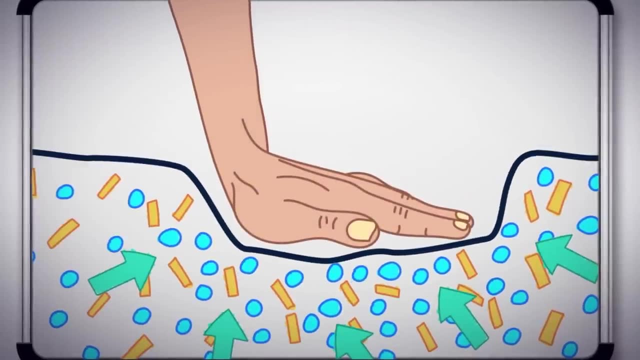 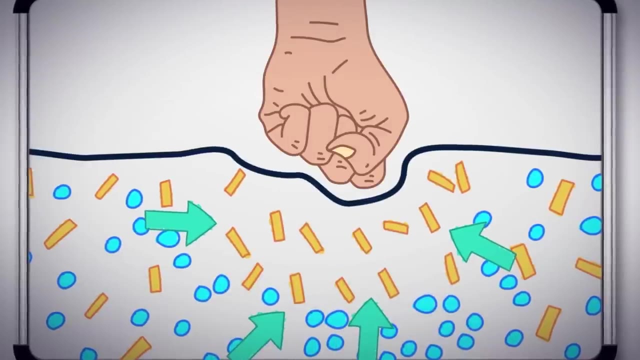 Which acts as a solid Cornstarch. mud is a shear thickening fluid. Shear is talking about the force of things sliding around, In this case the molecules. So when the shear force is strong, the fluid thickens, Shear thickening. 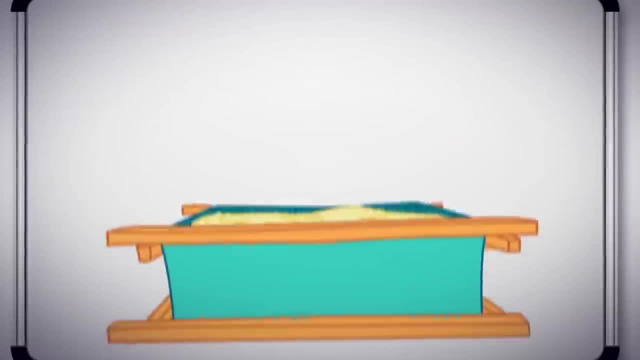 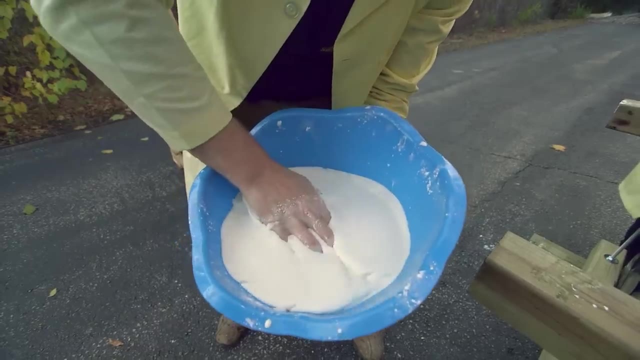 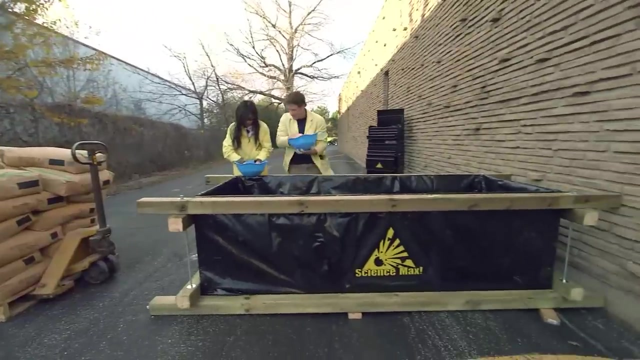 So here's the plan. If Judy and I make enough cornstarch mud, could we run across it? Let's find out. Yeah, I think mine is just the right consistency. How's yours, Judy? I think I'm ready too. 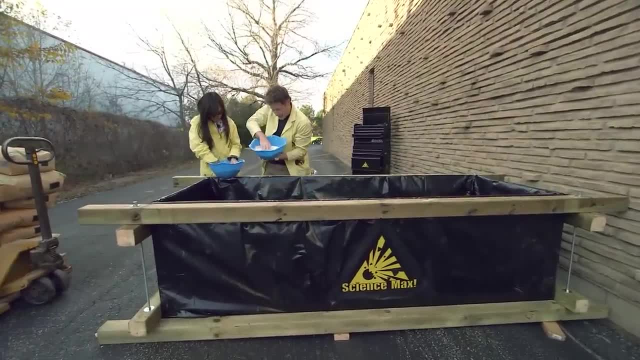 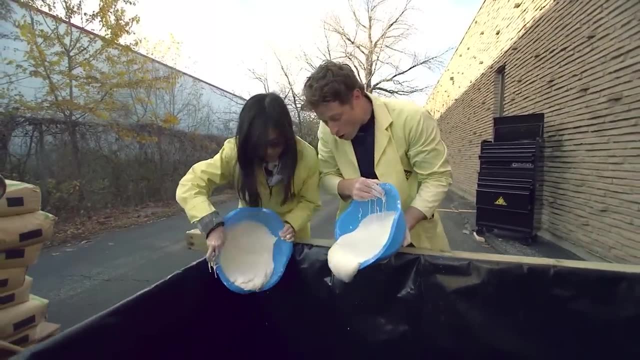 This is much harder than I thought. Yeah, it's really hard to get it mixed at the very beginning, But mine is ready to go. OK, here we go. First batch You ready? Yep, Dump it in Whoo. 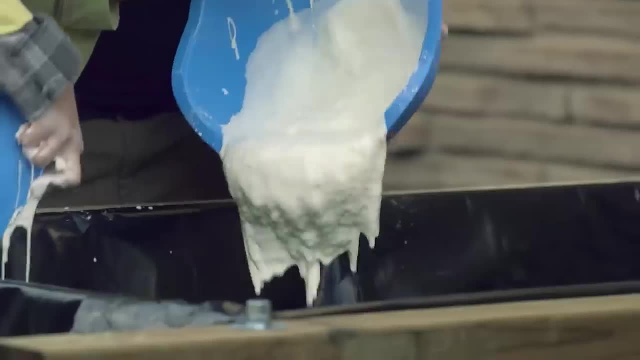 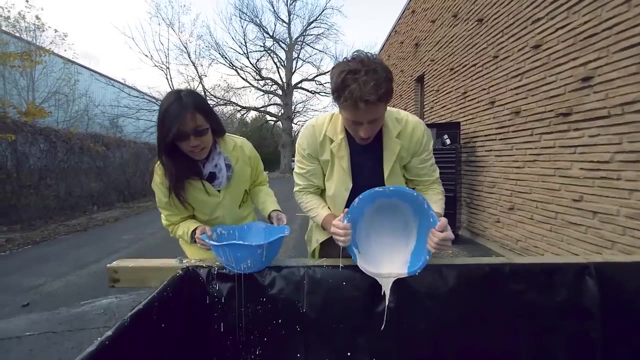 Whoo, Hmm, I thought that would be more. I thought so too. It's really not filling up. It's not filling this up very much, is it? No? Huh, that's a lot of cornstarch. 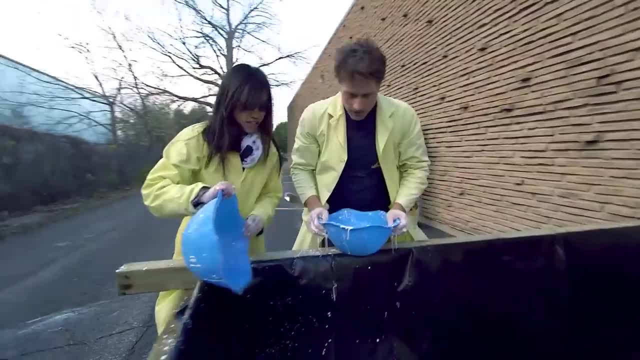 This is great, but I think we're going to have to go a little faster than this. I think we need some sort of mixing device. Yeah, I mean, we don't have to do this by hand. We can get some sort of machine to help us. 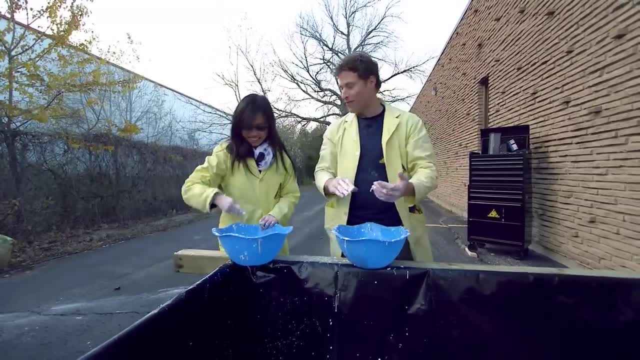 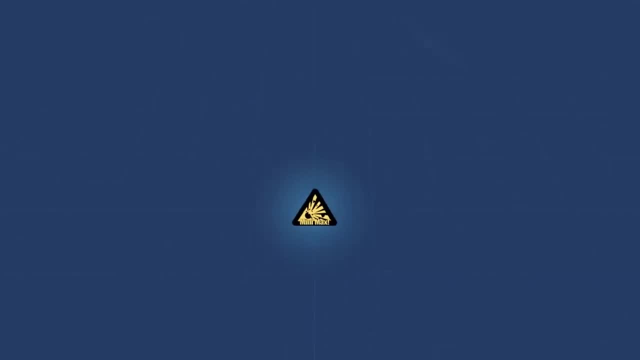 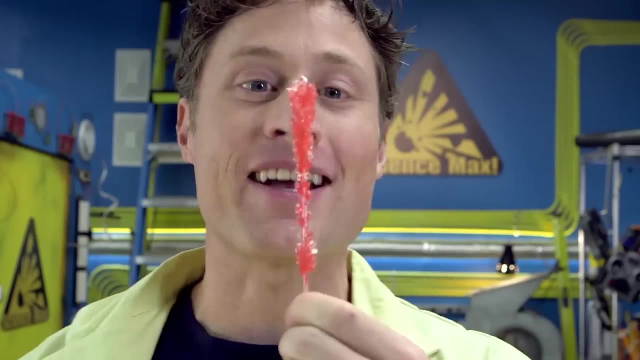 Yeah, Right on high five. Oh, We shouldn't high five when we have this stuff on our hands. Nope, Yeah, good call. This science is delicious. This is rock candy. It's basically crystallized sugar And you make it by turning a solid into a liquid. 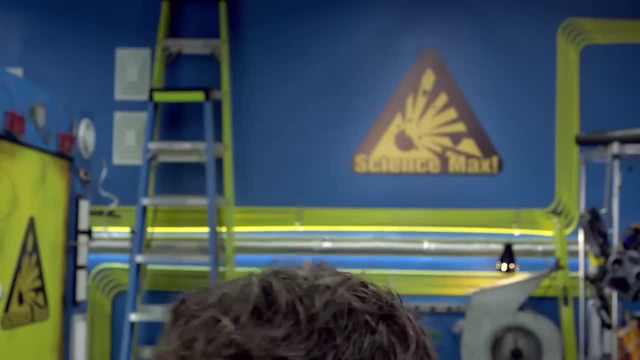 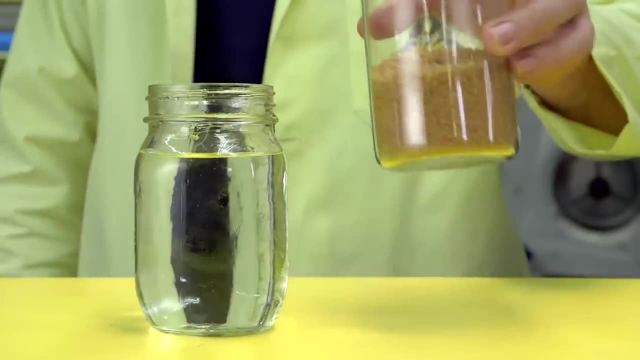 and then back to a solid again. Here's how you can make it at home. You need a container that you're not going to need for a while and some water, some sugar. You can use brown or white, I like to use brown. 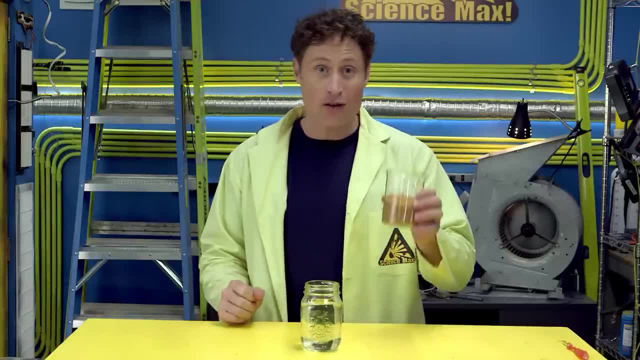 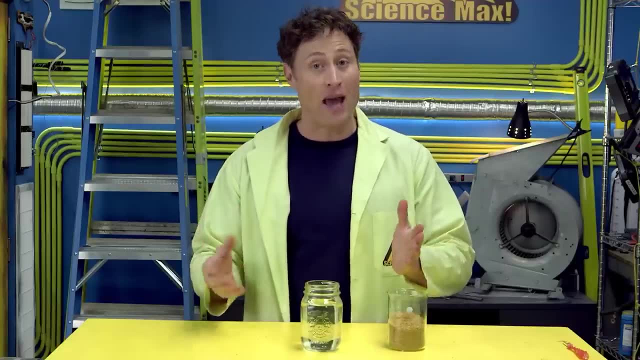 And an adult. Here's why you need an adult. You want to dissolve three cups of sugar into every cup of water, And you can't do that unless you think you're going to heat the water. So get an adult, a saucepan and heat the water up. 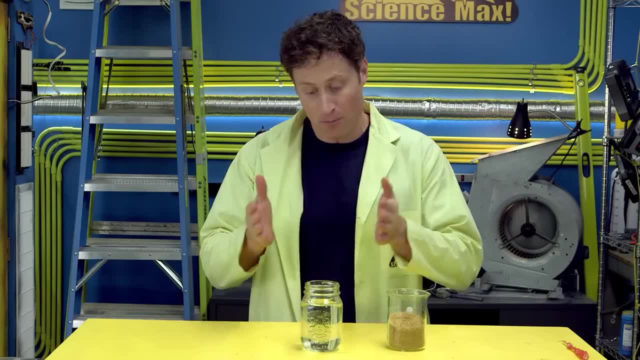 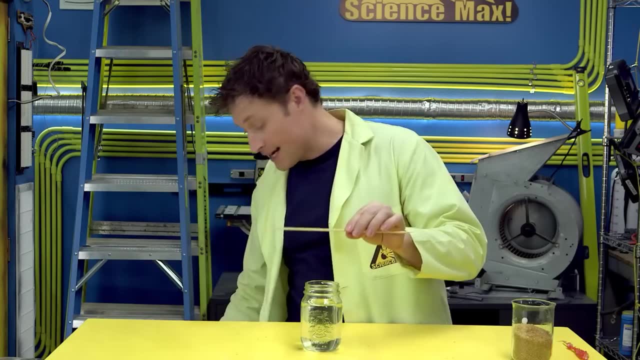 Pour the sugar in and keep stirring until it's all dissolved, Then pour it in your container and let it cool down. Then you'll need a shish kebab skewer, which is something you can get at the grocery store. Cut it down to the right size so it fits nicely. 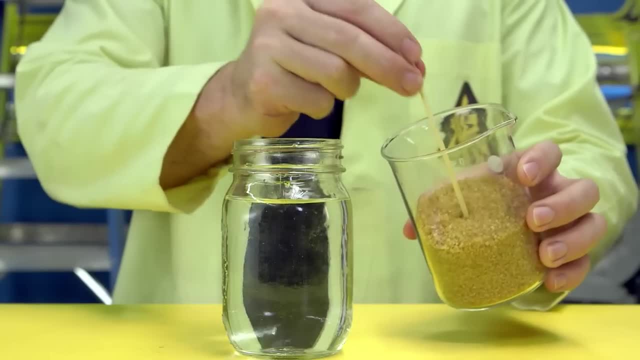 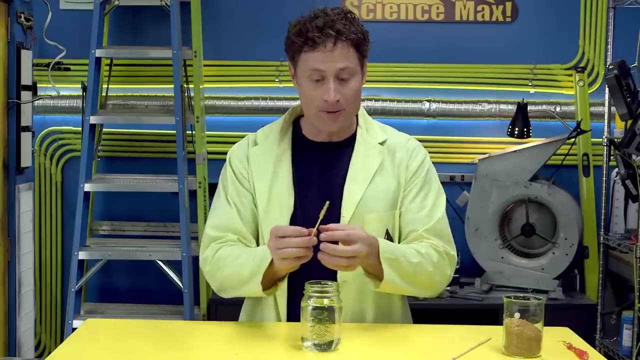 into your container And then dunk it in your sugar and get some crystals coated around the stick. These are seed crystals and they get the whole process started, And now you have to wait for these to dry, otherwise they'll just fall off the stick. 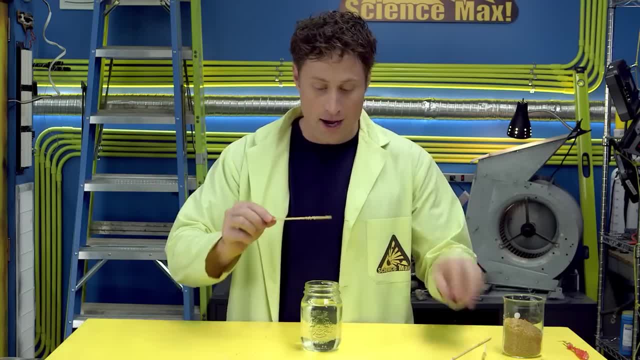 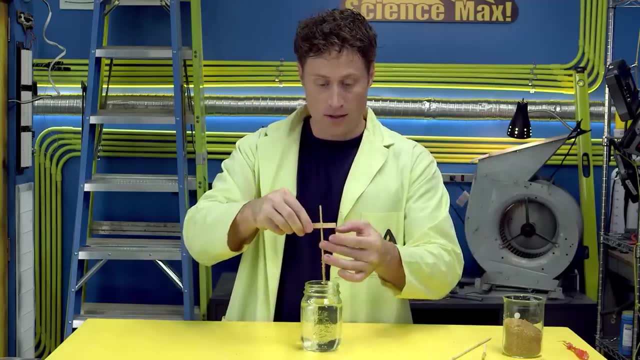 when you put it in the water. So I've got one here that has dried out. You'll also want something to keep it from falling in the top of the container, So I'm going to use a clothespin, Put it in there and dunk it in the container like that. 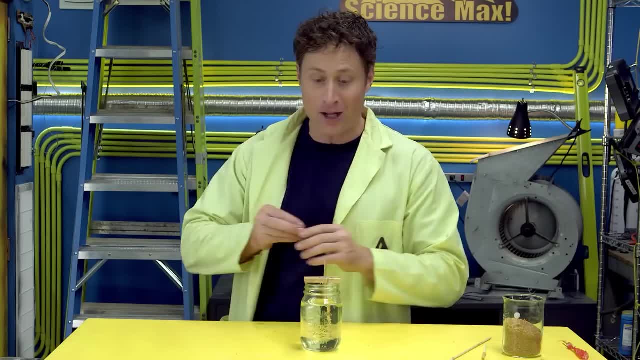 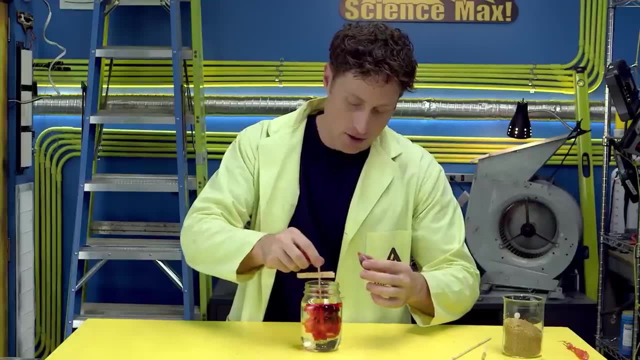 And now for the final step. if you want, you can add food coloring. I like to use red because it reminds me of science, And I'm going to use the stick to actually stir that up a little bit. Here we go Now: the dissolved sugar crystals in the water. 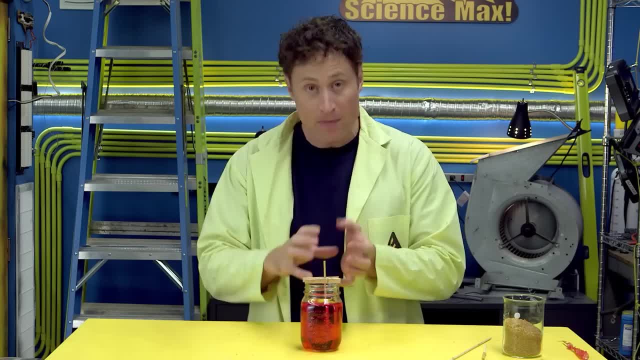 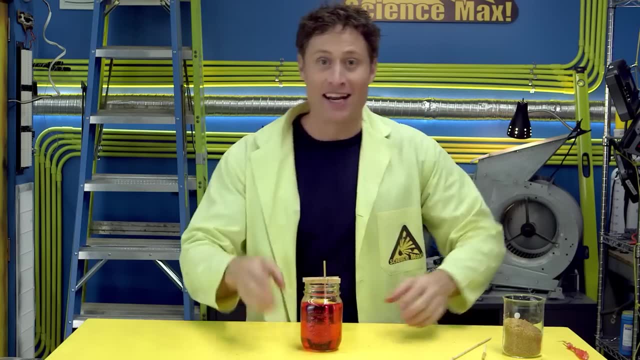 will slowly grow on the crystals that are already attached to the stick and it will eventually grow into a rock candy pop. But it takes about a week. No, I'm just kidding. I've already got one that's standing by. Here we go. 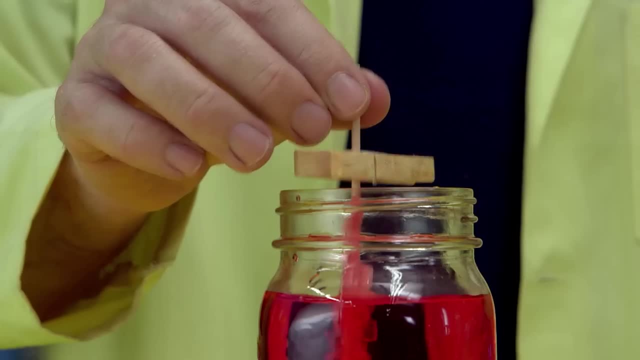 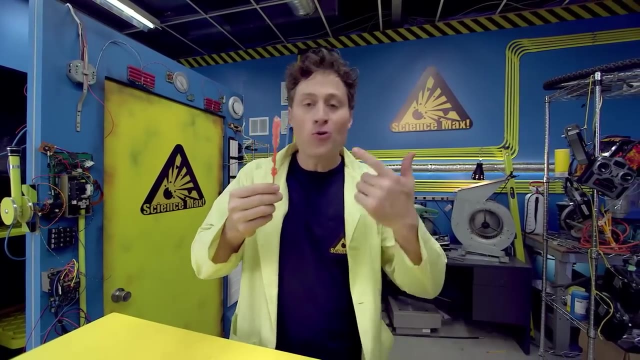 This one has been growing for about seven days And there you go: rock candy, Delicious science. Now how can we make this any better? It's crystallized sugar. It doesn't get any more maxed out than that, does it? 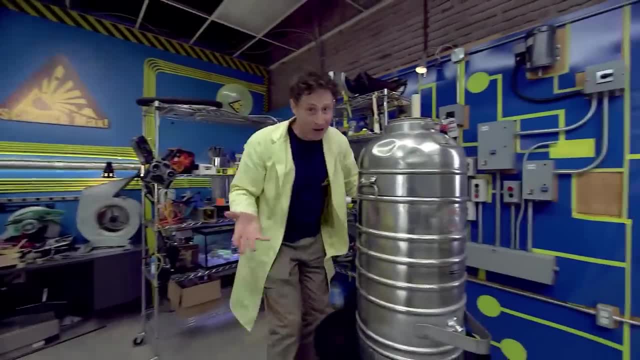 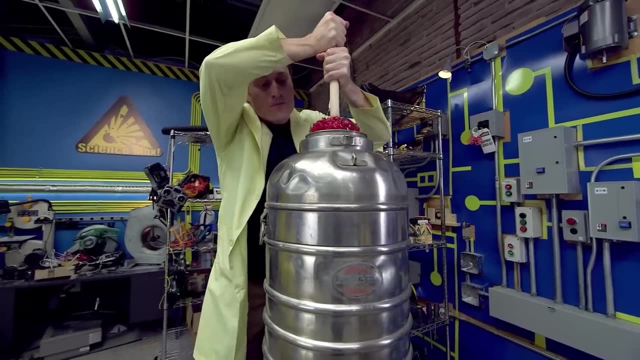 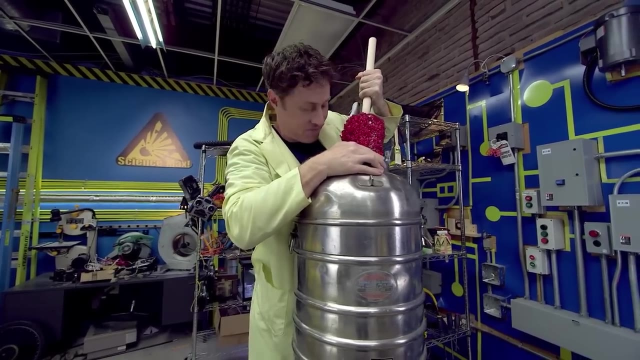 Yeah, it does, Come on. This is a giant container of sugar water And I've been brewing a massive rock candy crystal in it for a while, But it's sort of getting a little bit too big to fit out the top of the container. 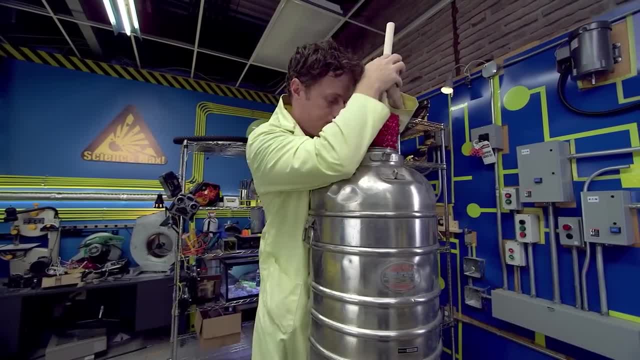 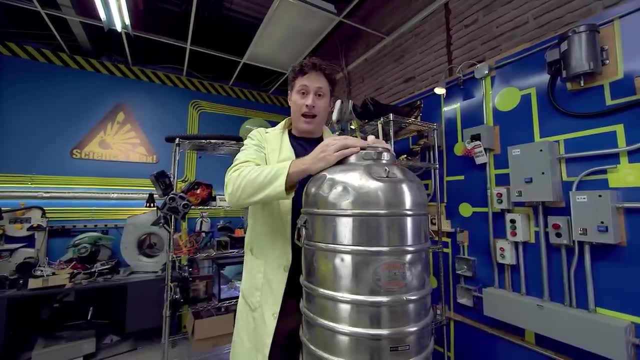 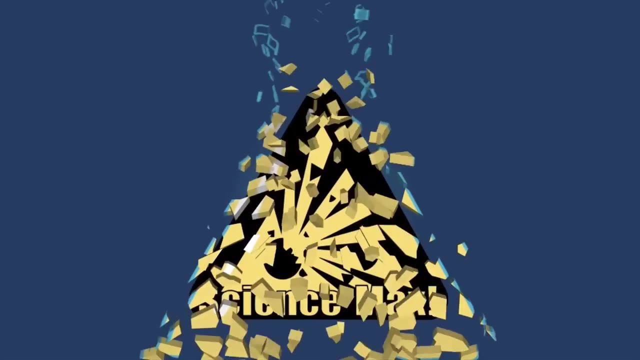 So you know what? I'm just going to put that back And chuck that one up to science, because, well, eating a rock candy crystal that big will definitely not be good for my teeth, So yeah, So our big experiment is to take a whole lot of cornstarch. 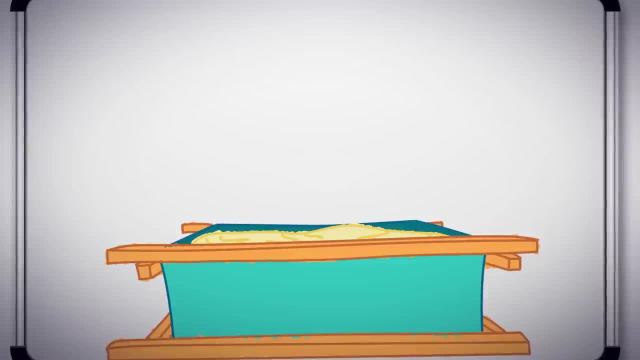 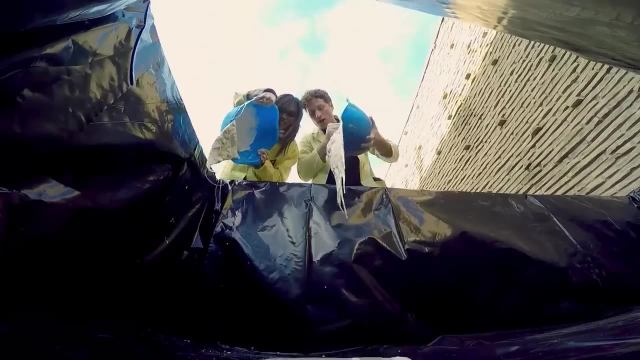 and fill a trough to see if we can run on it. But mixing it by hand was going to take forever, So Judy and I got a drill with a mixing attachment on the end. Whoa, I'm going to have to get this out of the way. 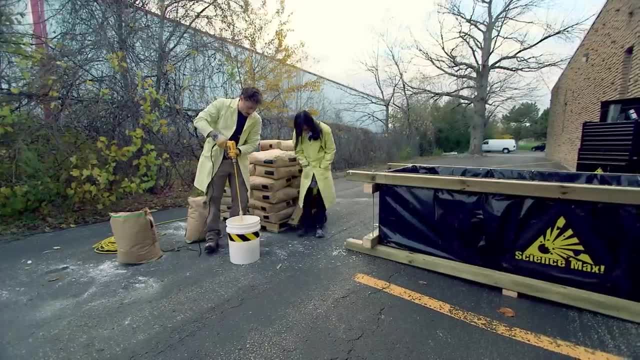 I'm going to have to get this out of the way. I'm going to have to get this out of the way. Whoa, Sorry, All right. So, Judy, I'm noticing a bit of a problem here. What is it? 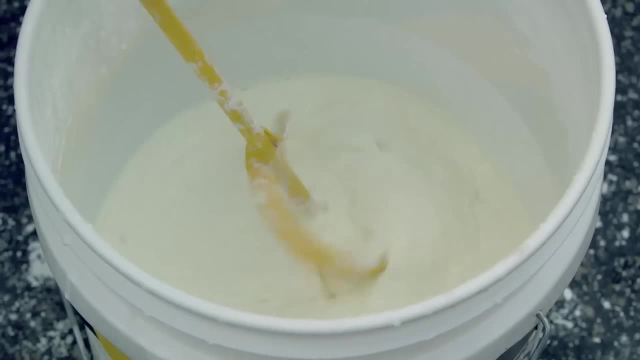 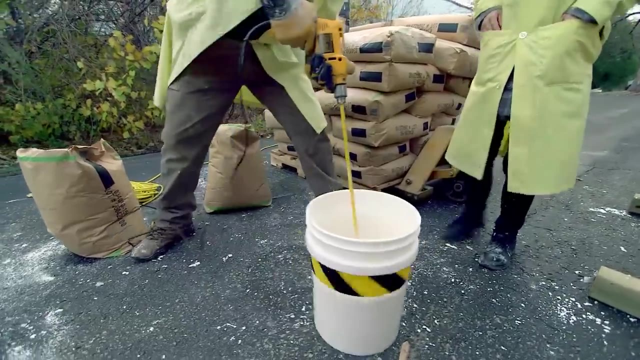 Well, if I mix at the top, everything's fine. But as soon as I get it a little bit deeper and then it gets really tough and the whole bucket starts to spin and the drill stops. Yeah, I think it's because the drill's. 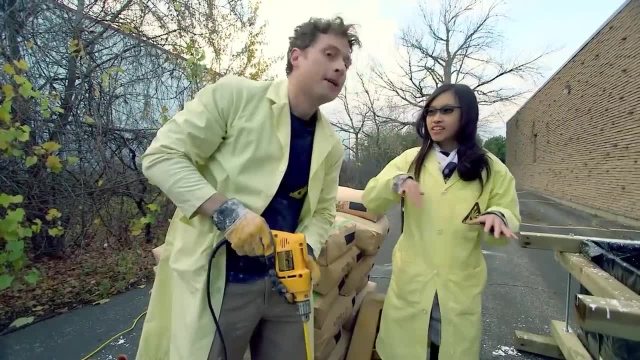 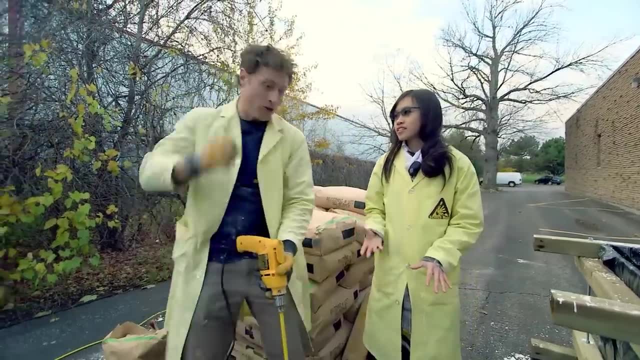 trying to mix it too fast. When we're mixing it by hand, it's slow and you can still let it stay a liquid, But now you're just making it solid. Right, because it's a sheer thickening fluid, Exactly. 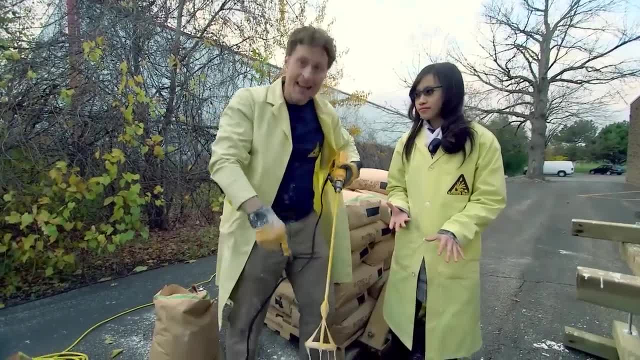 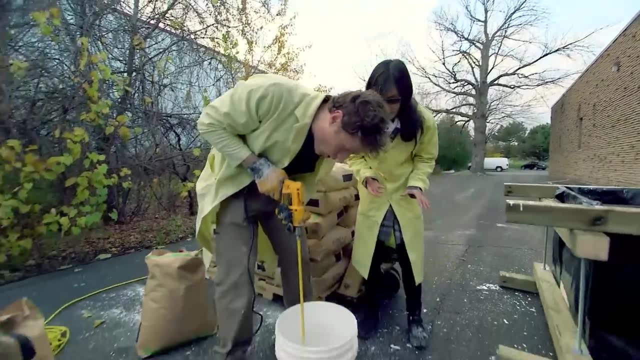 So if I mix really quickly with something like the blades of this spinning really quickly in the thing, it'll suddenly turn into a solid and it'll be really hard to mix. Yep, So we go slow, Going slow, Going slow. 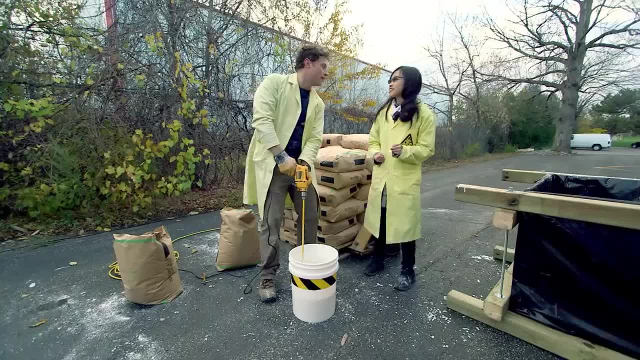 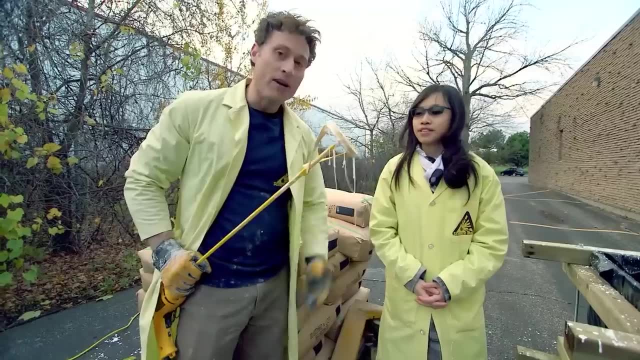 Suddenly realizing that if we go slow, we'll be here forever. Yep, You know what I think we need? Whoa, Sorry, You know what I think we need? We need a different way to mix this. Yep, We need a way to mix more of it and we need a way that it. 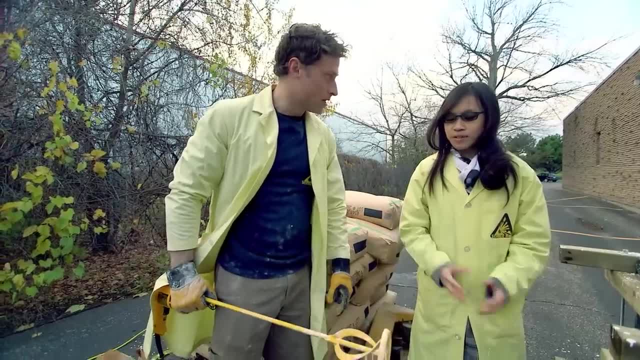 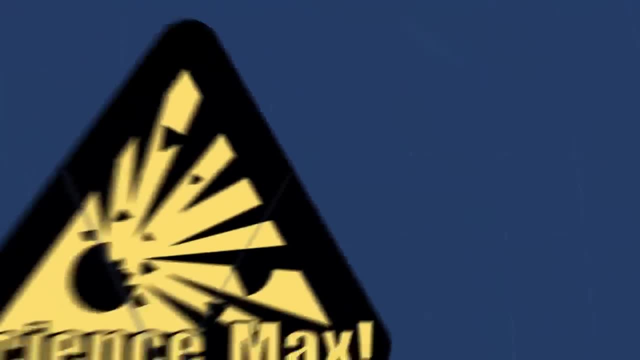 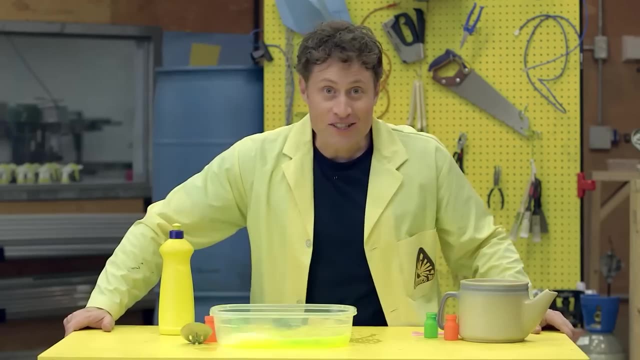 doesn't hit it with both hands. You know blades that suddenly go through it really quickly, Something that can mix on a large scale, but slowly. I have just the thing. Come with me, All right. The interesting thing about bubbles is they're a gas surrounded by a liquid. 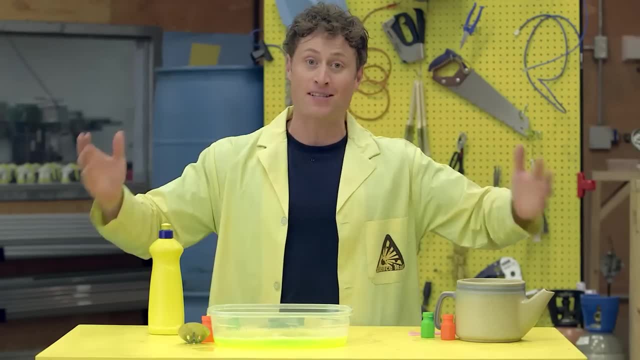 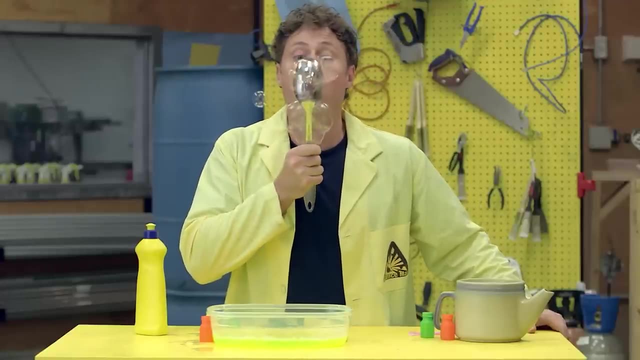 So get some dish soap and some water and then be science maximites and find things around the house that you can make bubbles out of. Just about anything that has holes will do Or mm-hmm, Or I like this one. 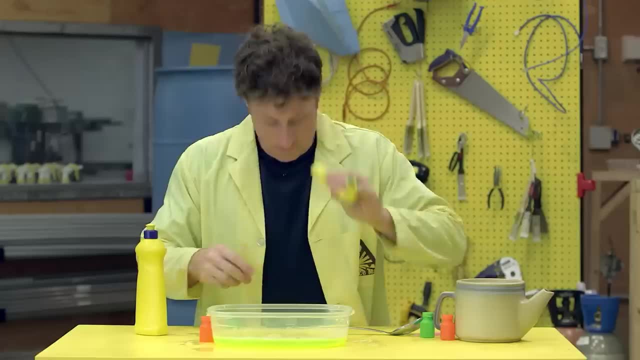 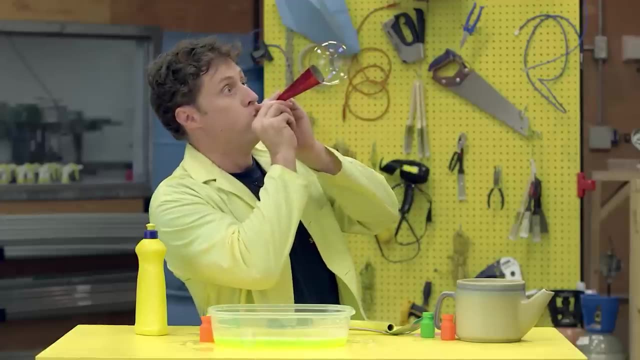 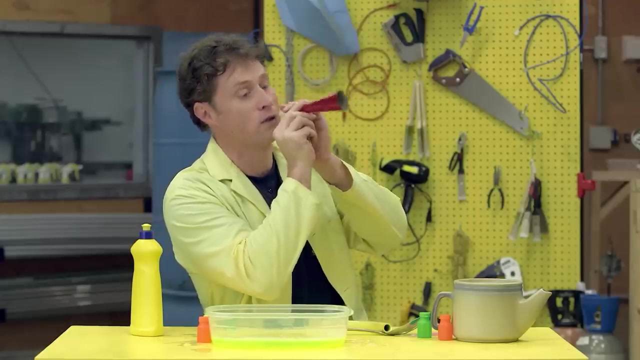 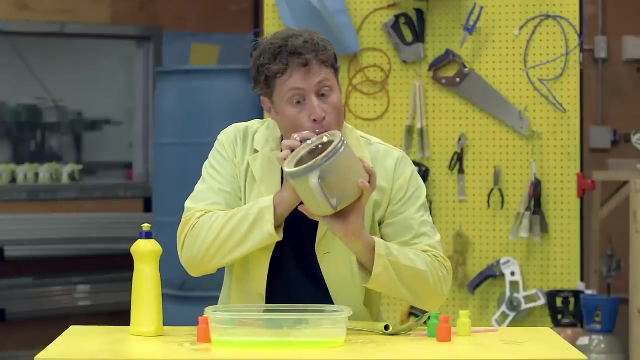 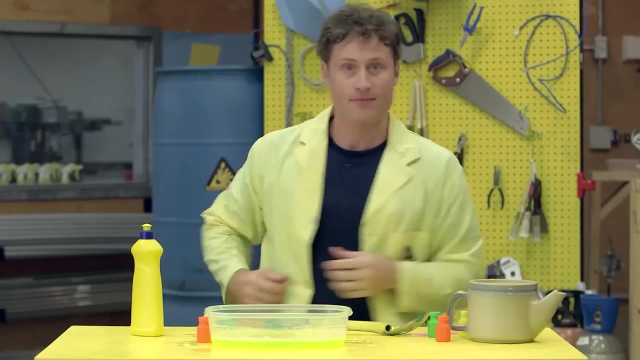 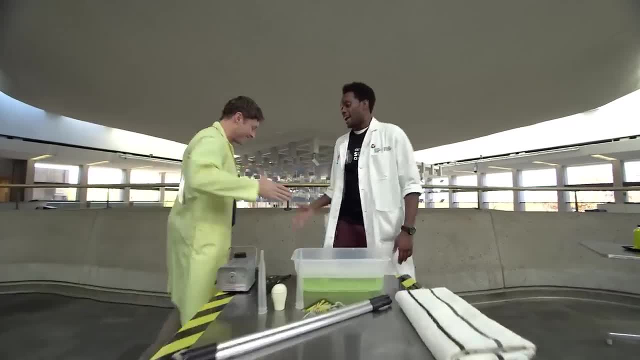 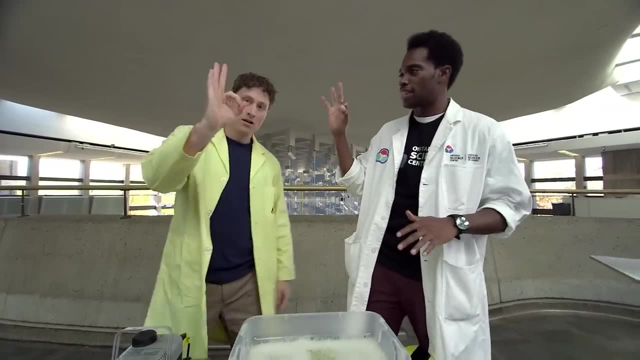 I'm here at the Ontario Science Centre and this is Anthony Hey. Anthony Hey, how's it going Good? So you are amazing at bubbles. I am. I've been practicing for a while. Let's get started, Okay. 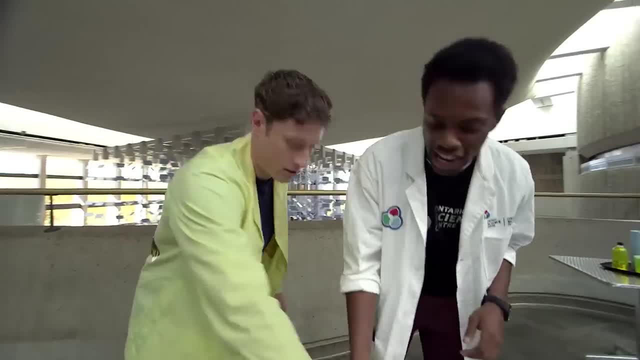 You're going to make an okey-dokey sign like this: Uh-huh, You're going to dip it right into our bubble solution. Come on, Get right in there. Right in there. Make sure you get it all up. That's a little too much. 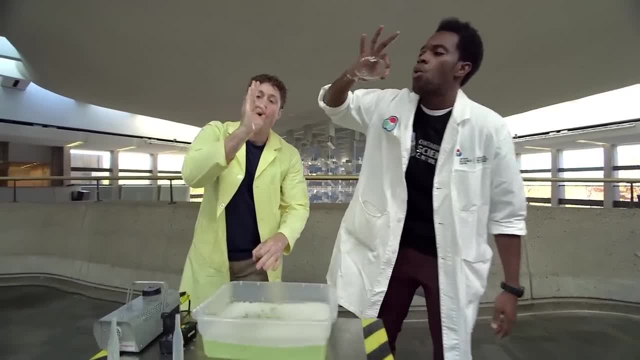 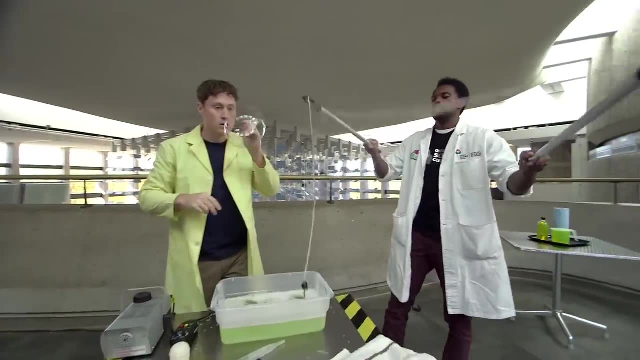 Well then I can make two, And then you're going to keep that okey-dokey sign. Very gently Nice. I brought these two giant sticks here and I don't know if you noticed, but I've got a smoke machine here. 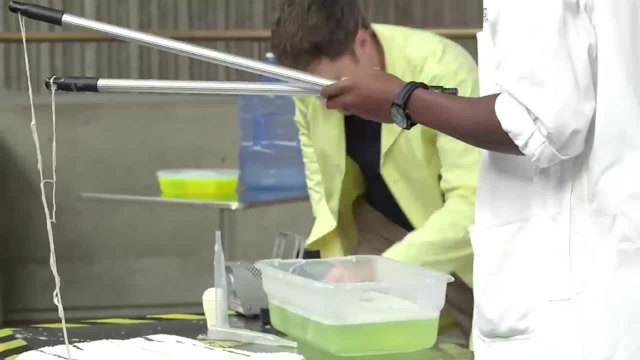 Right, So we'll turn that on and then if you press that green button there, you're going to shoot some smoke and we're going to try to catch that smoke in a giant bubble. You ready, Okay, I'm going to try to. 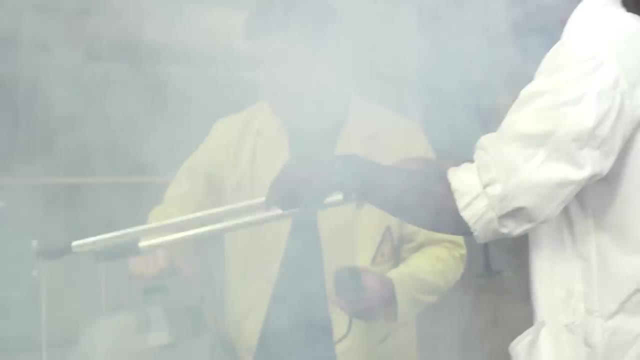 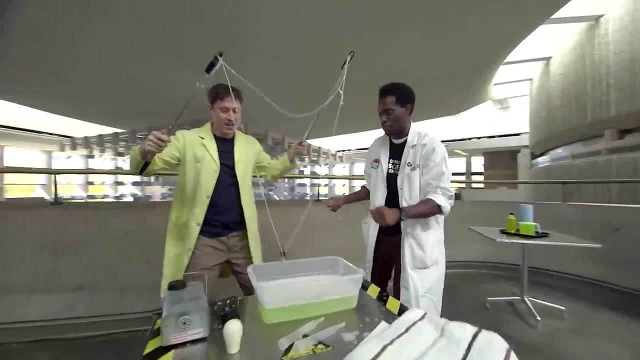 Oh, that was so close. Did you see that one? That was great. You give it a shot. Nice, Oh, check that out. Yeah, That's amazing. That was huge. Try it again. Let's see if I can get the smoke machine. 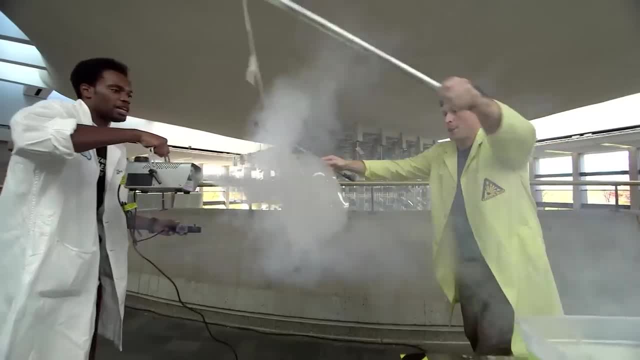 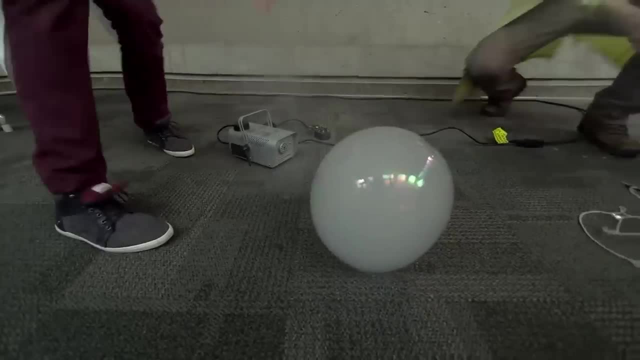 Here we go, Go for it, Go for it, Push right towards. Oh, check that out, You did it, Look at that. Look at that: No Smoke And it bounces. It bounces on the floor because the floor, it doesn't have any oils, like our hands do. 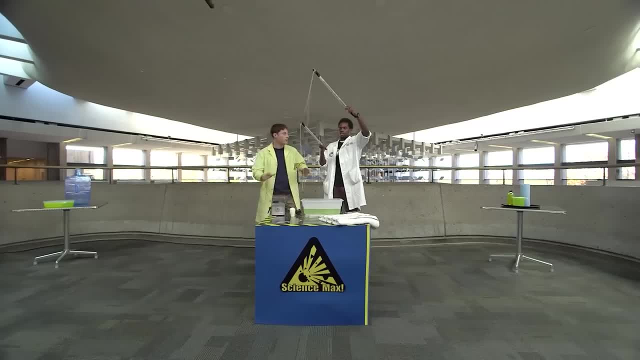 Isn't that amazing. That was great. Oh my God, That was so cool. That was great. You know what I think we should do? What's that Giant bubble? tons of smoke Done. Okay, here we go. 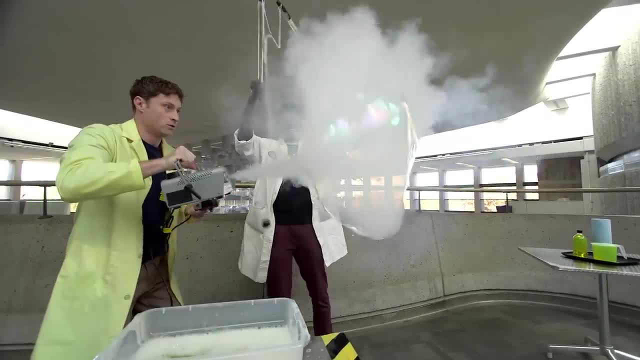 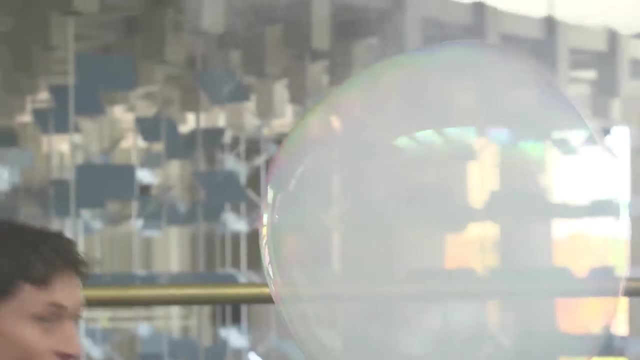 Let's do it. You ready? Here we go. Awesome, Oh my God. Look at that. Amazing. Look at that- That's crazy- Maxed out bubbles. Well, there you go: Giant smoke-filled bubbles- Awesome. 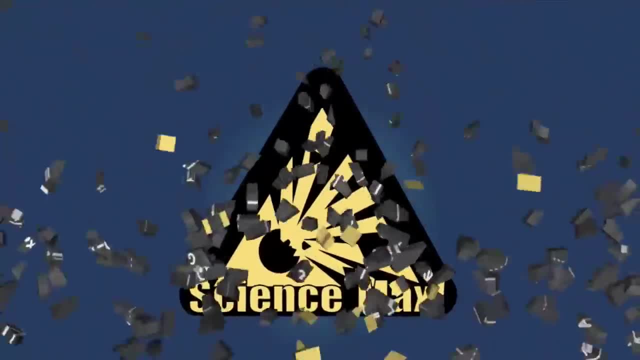 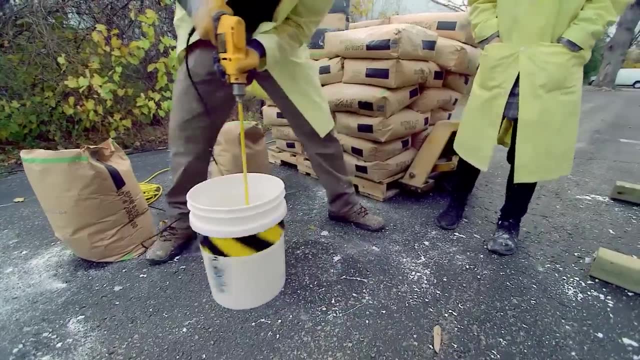 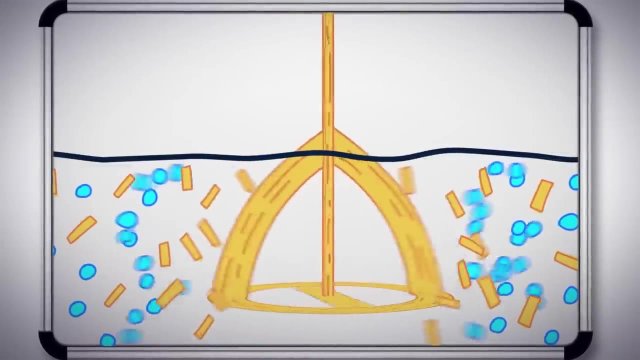 Yeah, Judy and I tried mixing the cornstarch mud using a drill with a mixer attachment, but it didn't work. We should have known better. Here's the mixer in our cornstarch mud. Usually a mixer works by going really fast. 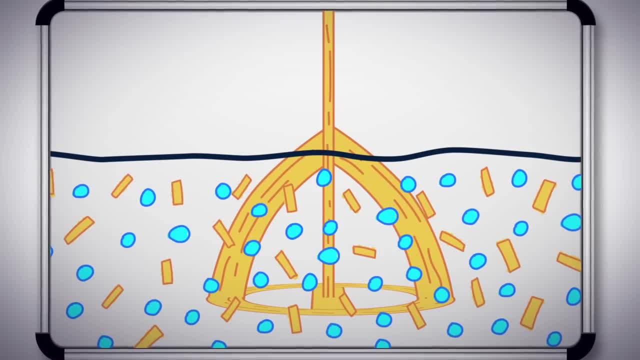 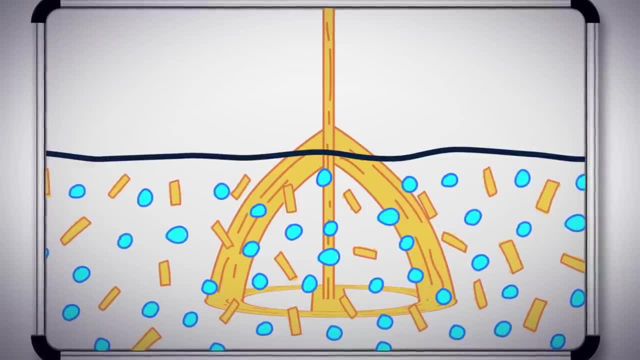 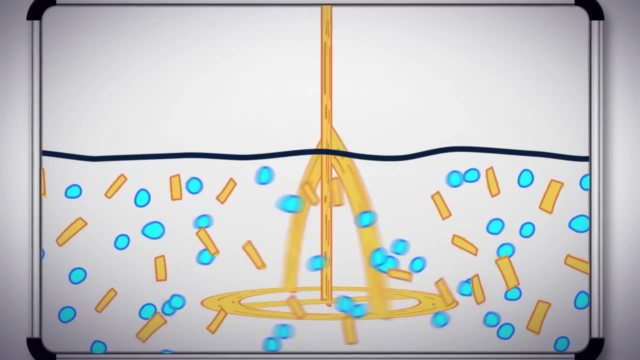 Really fast and mixing everything together. But remember that cornstarch mud is a sheer thickening fluid. So when the blades of the mixer tried to go fast through the cornstarch mud, it did what it always does: turn solid. The faster and harder you try to move it, the more solid it will become. 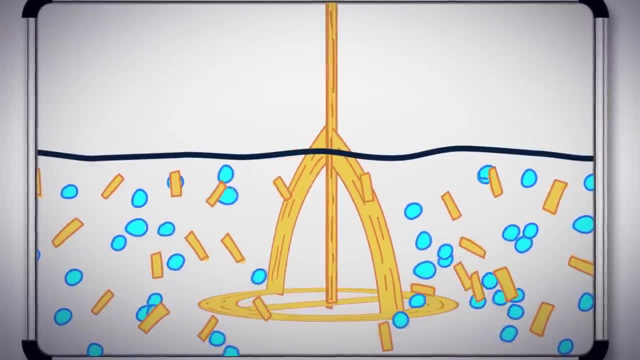 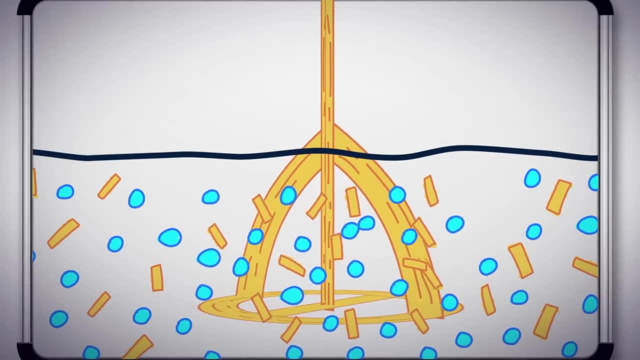 This means the only way to mix. it would be if we made the drill go very, very slow, which wouldn't speed things up at all. So with the drill and other lost cause, Judy and I need the biggest thing around that could mix stuff up. 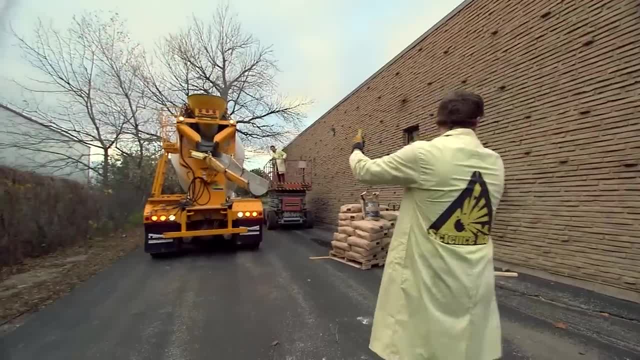 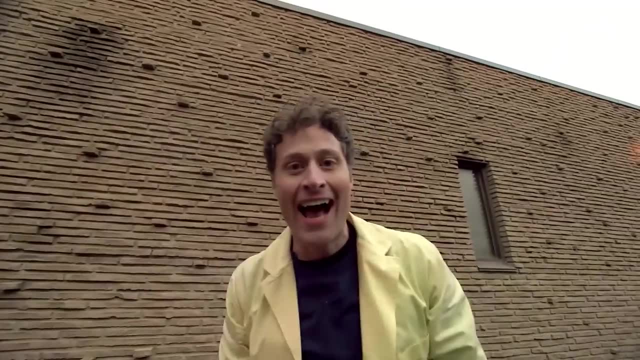 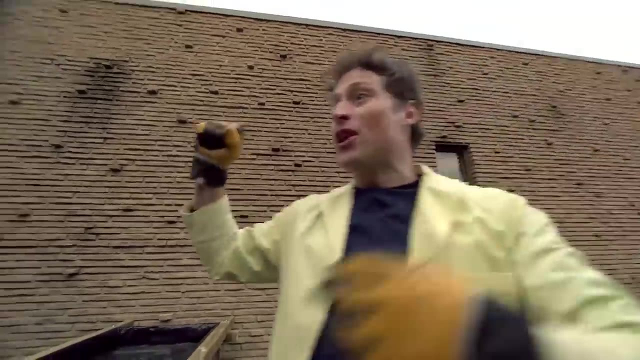 Come on back Good Little bit more. Perfect- A cement truck. A cement truck is the perfect thing to mix, because all we have to do is get all the cornstarch up in here and it'll mix it, and it doesn't move it too fast. 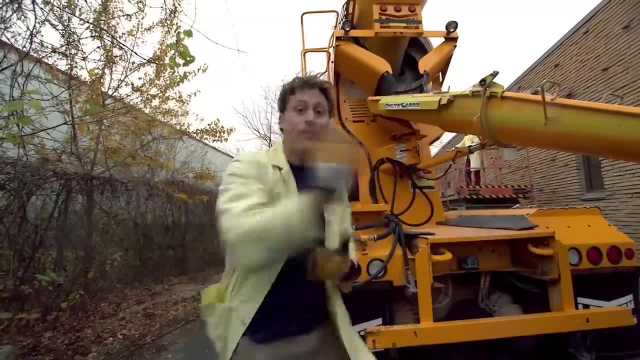 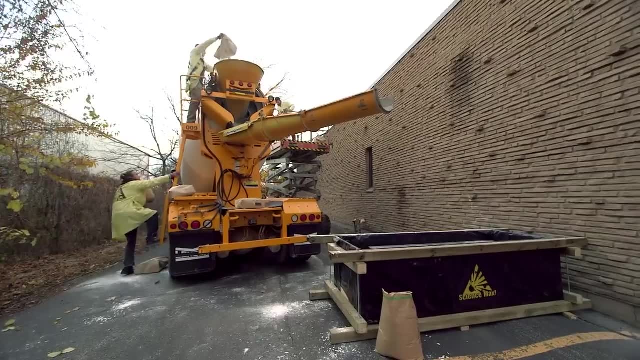 It goes nice and smooth, Nice and slow. So hopefully a sheer thickening fluid will be fine. I'm going to get Judy. She's driving the truck. Hey, Judy, that's perfect. The only problem is we needed to get all of those bags of cornstarch into the hopper of. 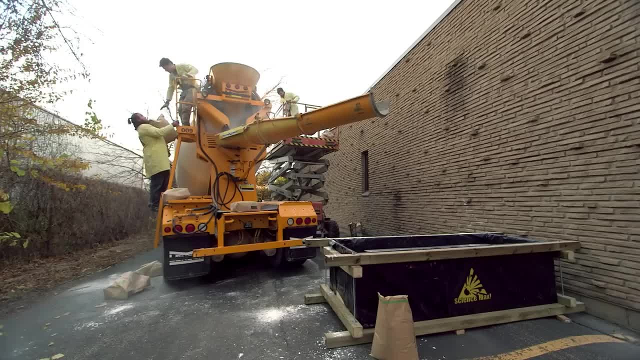 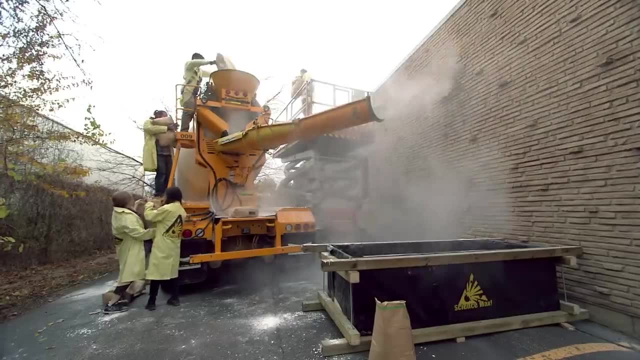 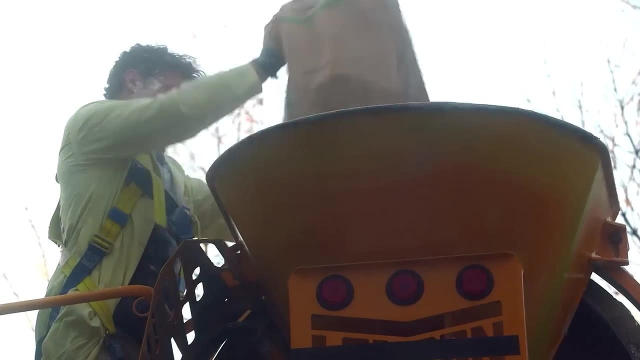 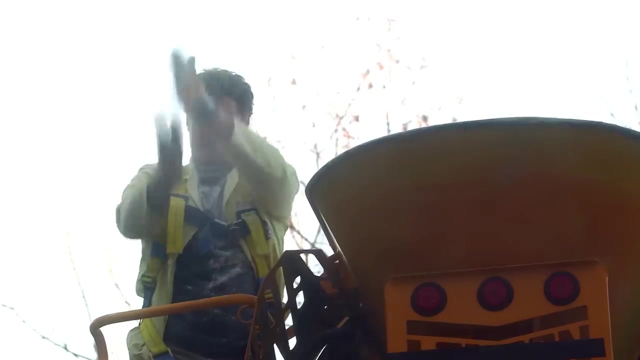 the cement truck. I didn't think it would be this messy. We needed to call the entire Science Max build team to help us out. This is possibly the messiest thing I've ever done. Awesome, Hey, Judy, you want to lift up any bags? 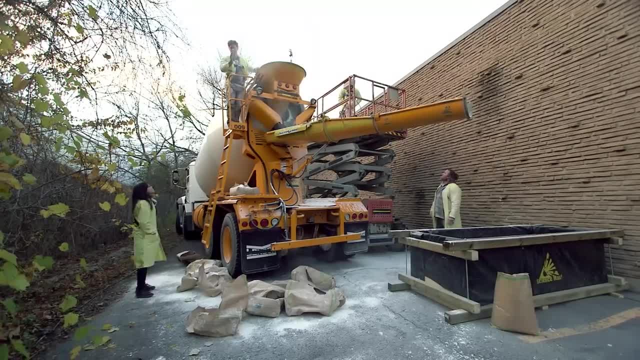 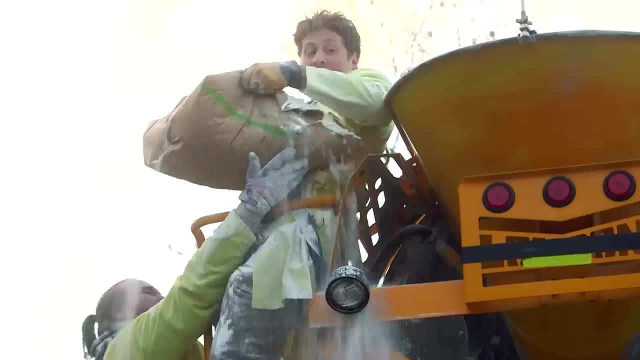 I'm okay, thanks, That's okay. I'm having a lot of fun, So I can do them Cool. Oh no, Oh no, Oh no. Yeah, I got most of it. I got most of it. 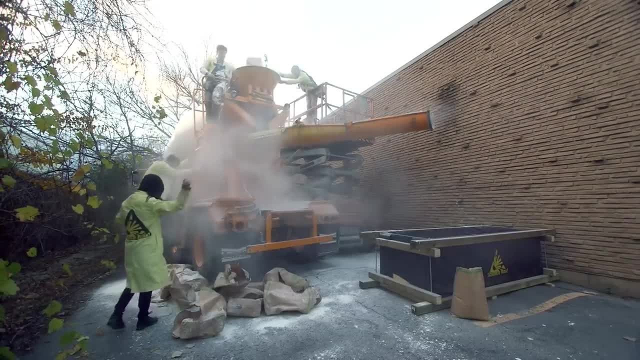 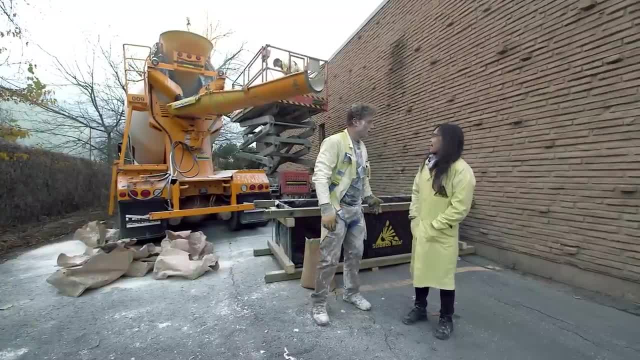 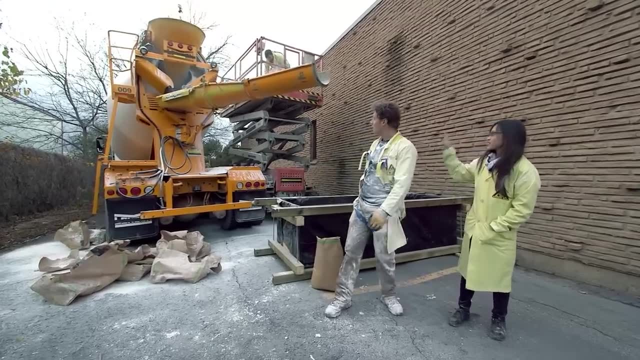 Do you think it's going to work? I think so, because you're mixing at a very large volume but at a very low speed. Yep, So throughout the process it'll stay a liquid until we're ready to run across it. That sounds exactly like the kind of science I like to see. 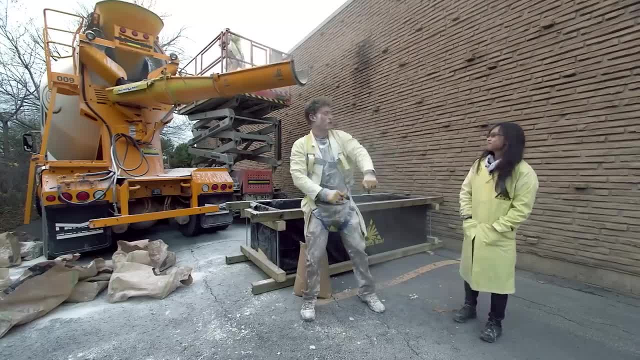 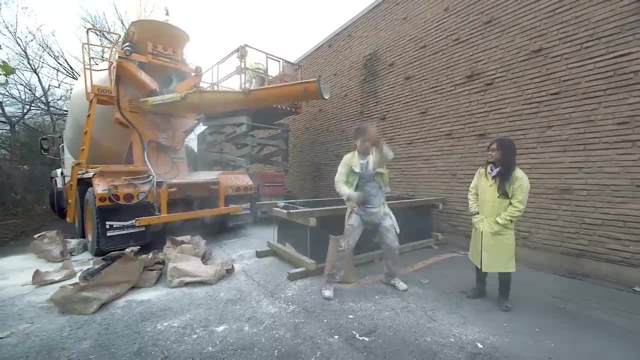 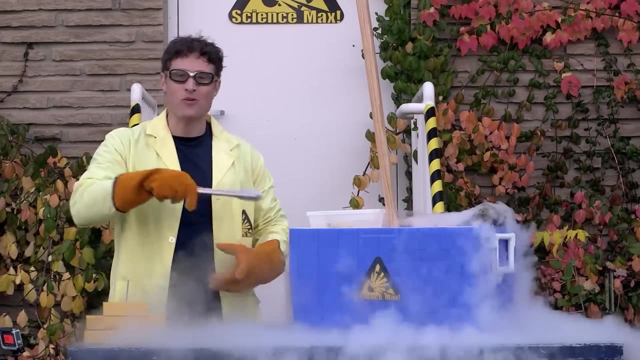 You know, what I really like is that every time I move, more cornstarch comes off. Okay, It's like I'm a human fog machine. This is liquid nitrogen. Nitrogen makes up most of the air we breathe, but if you get it really, really cold it. 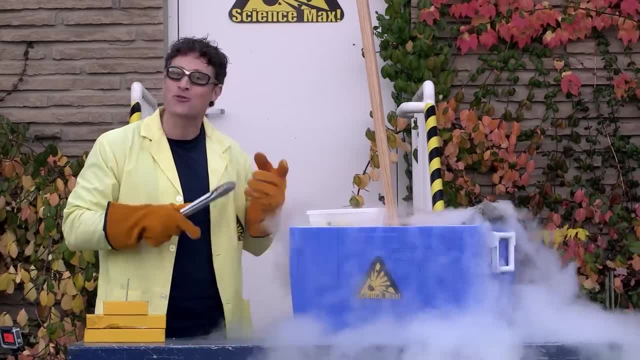 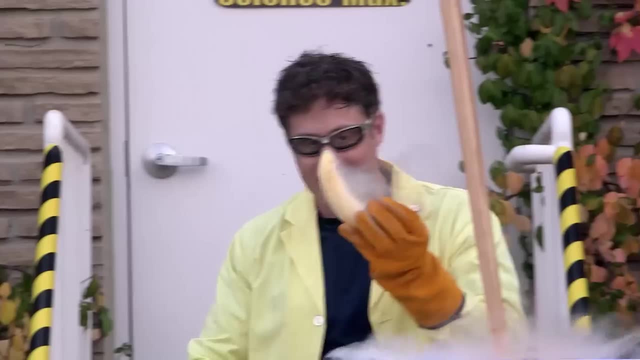 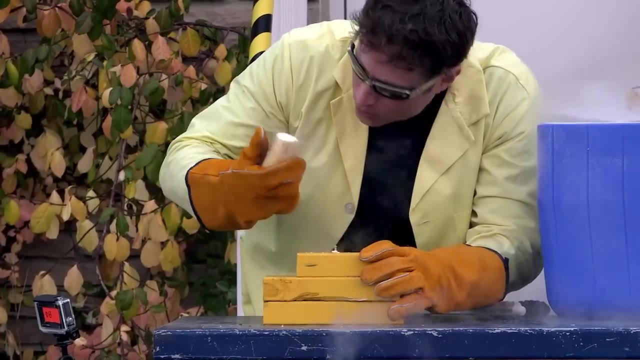 turns into a liquid. The fun thing is you can use it to make other things really really cold too, like this banana. I have frozen this banana solid thanks to the liquid nitrogen, and normally a mushy banana would not be able to hammer in a nail. but whoa, because it's frozen, I can hammer. 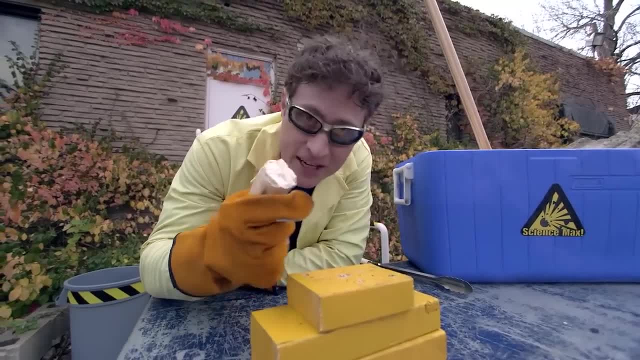 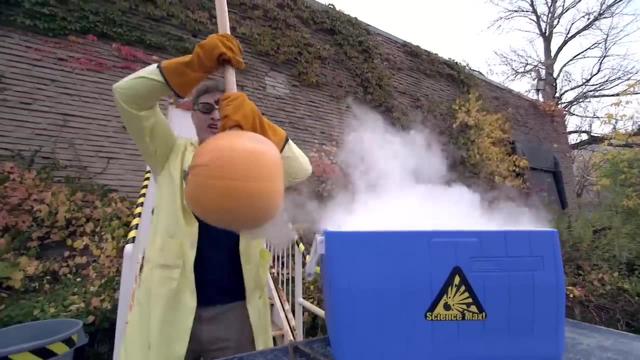 this nail into this block of wood. So that got me wondering if I can turn a banana into a hammer using liquid nitrogen, could I turn a pumpkin into a sledgehammer? Let's find out. Pumpkin sledgehammer, take one. 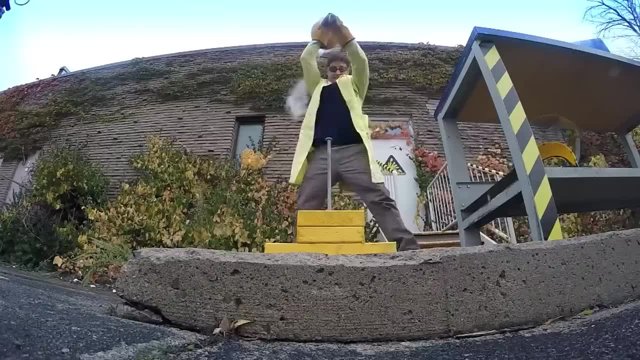 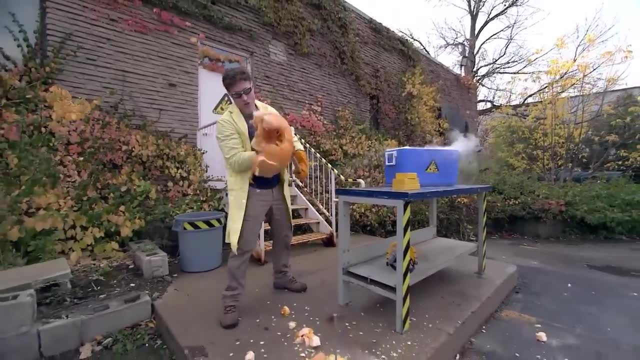 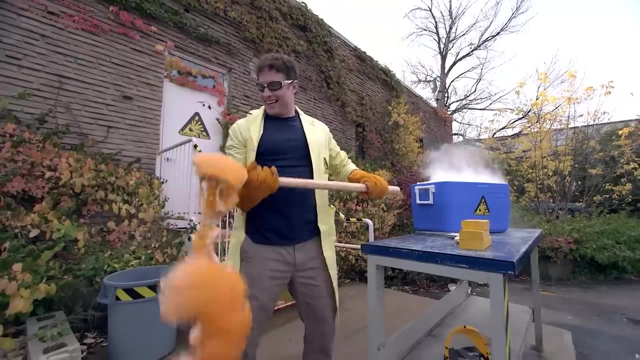 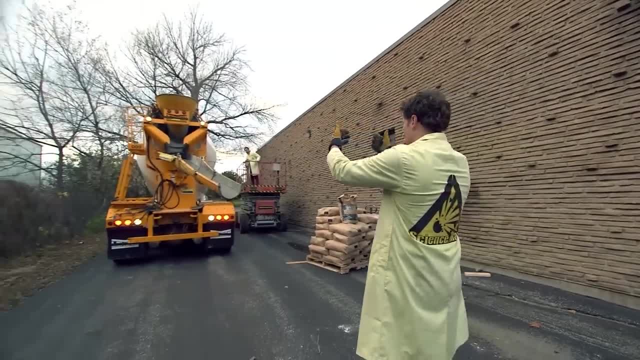 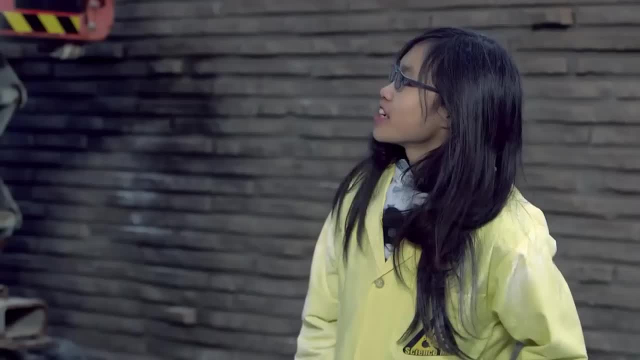 Now we have a cement truck to help us do the mixing for our cornstarch mud. After making a giant mess getting the cornstarch into the cement truck, it's time to see if it worked. Hey, Phil, how's it going? 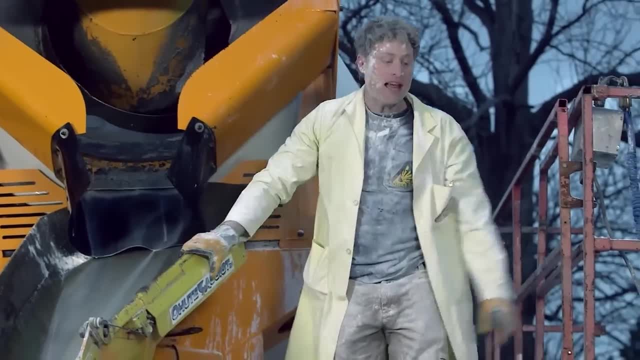 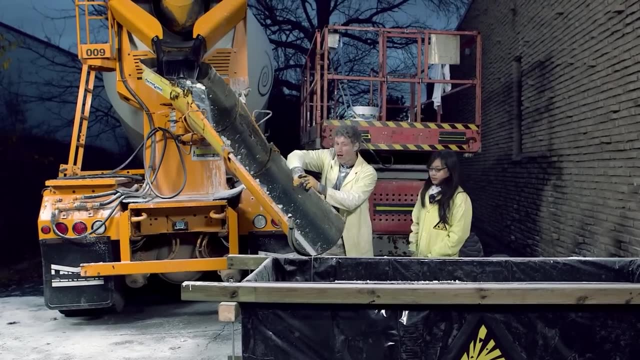 Yeah, it looks like it's mixing pretty well. I'm really glad we are not doing this by hand, because it did take a really long time. We've almost got it at the right consistency, but it's taking some time, but it's getting. 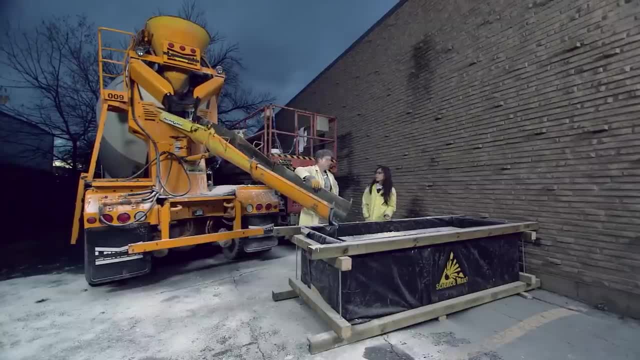 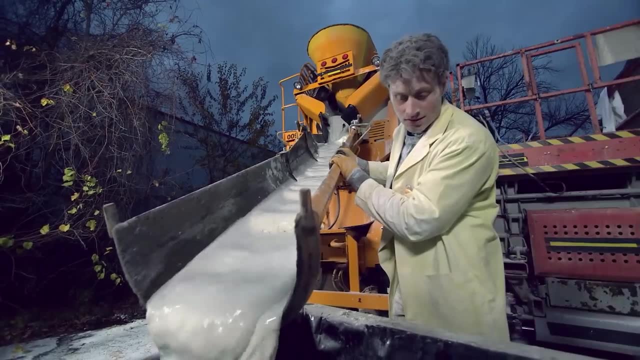 a little dark out. Judy, I don't know. Do you want to quit and go home? No, Of course not. That's not what we do in science. Oh, here we go. Yeah, Awesome, All right, Let's see it. 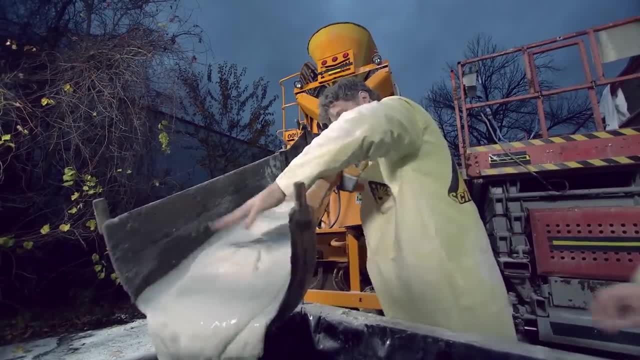 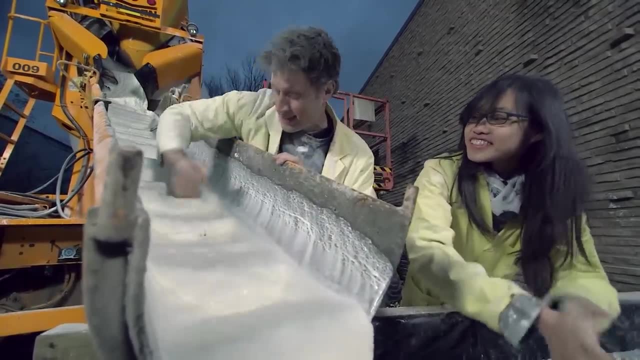 Let's see if it's. I like how it comes down a little steeper. Yeah, Yeah, I'm going to take a few more steps. Look, it's still. It's working, just like it should I hit it and it's solid, but you can see it's pouring like a liquid. 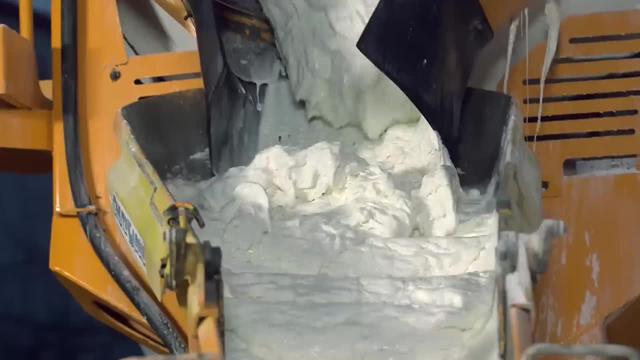 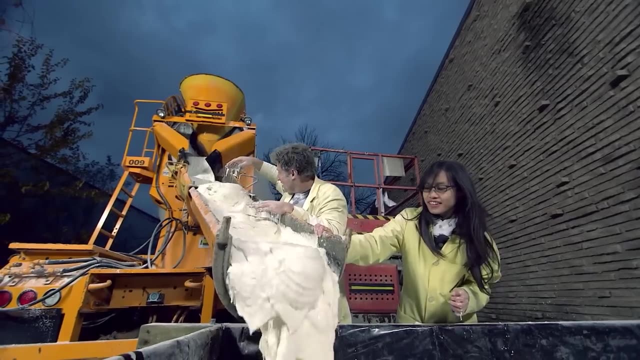 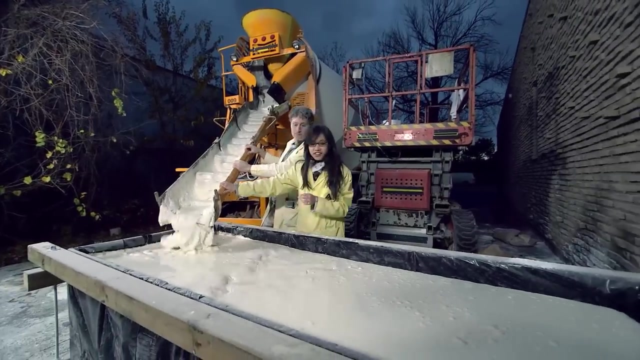 Here comes a big wave. Wow, Here it comes. It's totally filling up. Oh yeah, It's filling up really fast. I think we should stop pouring very soon. Yep, We may not have a big enough for us. We might not have enough. 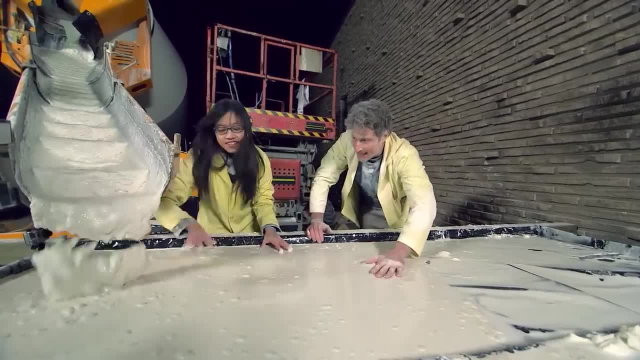 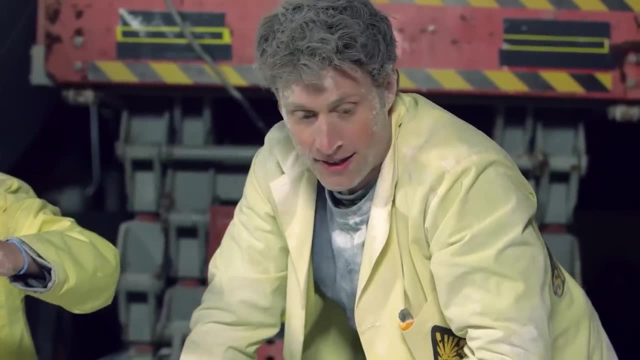 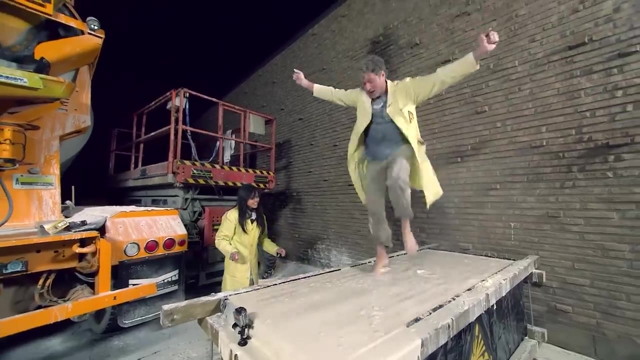 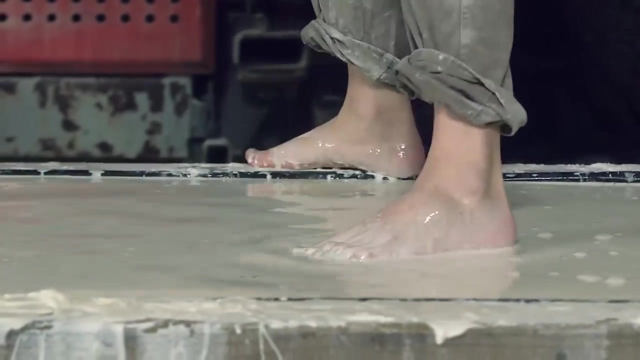 Yep, I'm liking it. It's good. Yep, I think it's time. It's not even done pouring, but I'm going to try it. Okay, You ready. Oh, you did it. Whoa, You can't. You have to get back onto the sides before you stop moving. 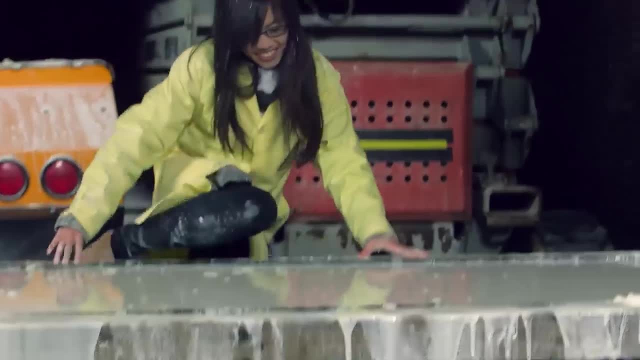 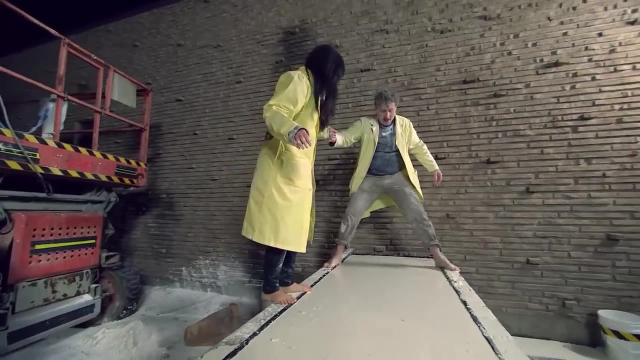 Or else it becomes a liquid. All right, It's your turn. Okay, Here, Go Okay, Ready. Okay, You got to hit your feet really fast. All right, Okay, Go Yeah. Oh, my God, This actually works. 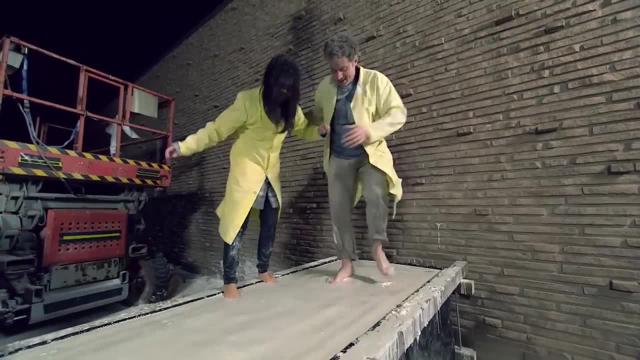 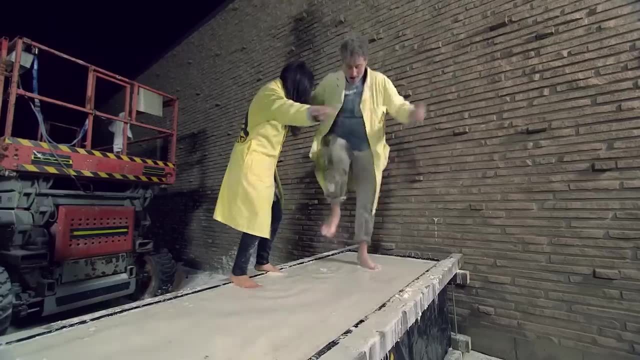 Because cornstarch mud is a sheer thickening fluid. it means it stays a liquid until you hit it suddenly, like with your hands or in this case, our feet, and then it turns to a solid. So as long as Judy and I keep slapping our feet down with the knowledge, we're going. 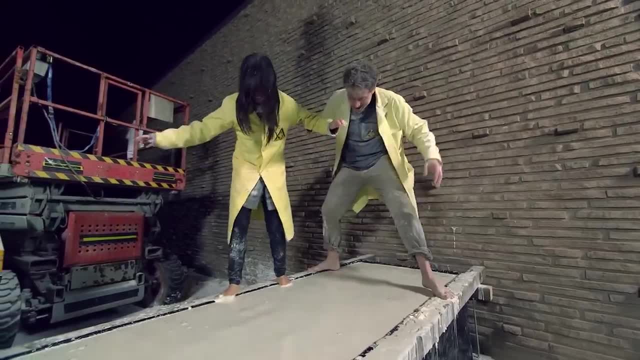 to do it. So as long as Judy and I keep slapping our feet down with enough force, we can walk on top of it. One more dance. All right, Let's do it And tell you what we'll do. one more dance. 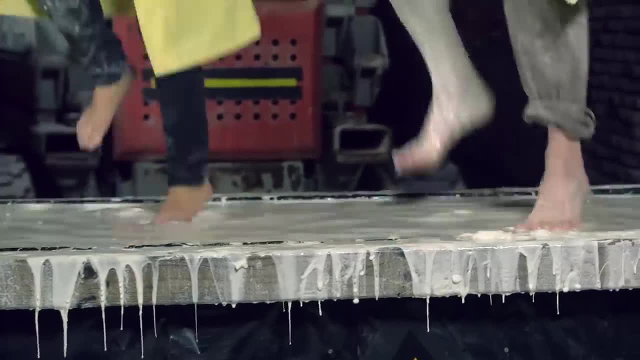 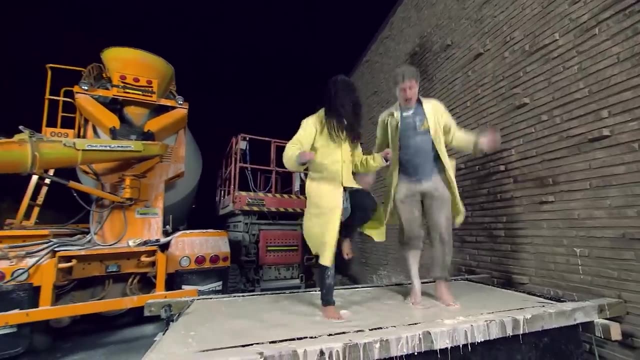 All right, Let's do that. Okay, Ready, All right And go. All right, All right, There you go, We've done it. Solid liquid gases. Thanks very much for joining us on Science: Max Experiments At Large. 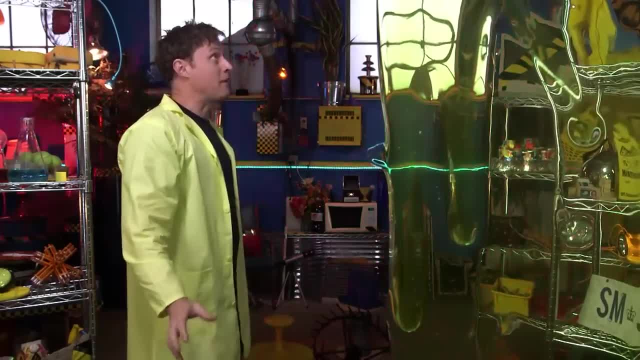 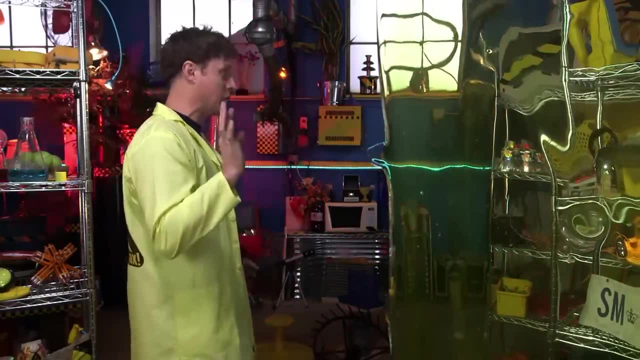 Woo Greetings. Science Maximites. My name is Phil and I think I might have overdone it. What's your name? I'm Phil. I'm Phil. What's up with the science? I mean, what's a better use of science than creating a whole bunch of slime? 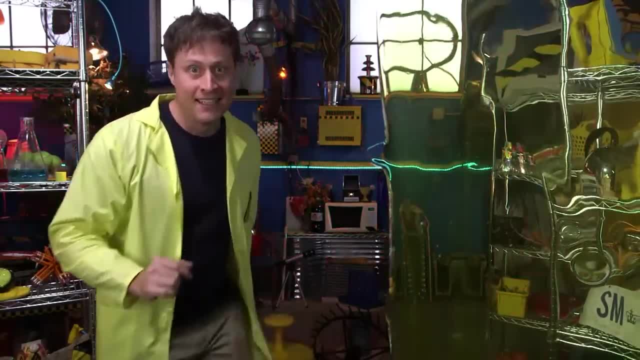 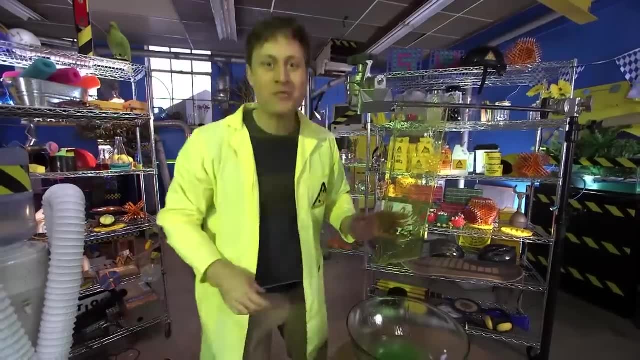 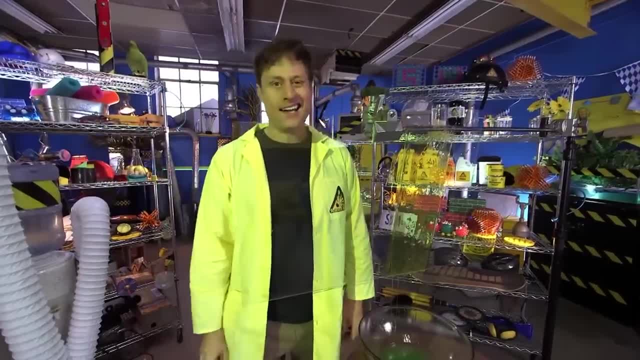 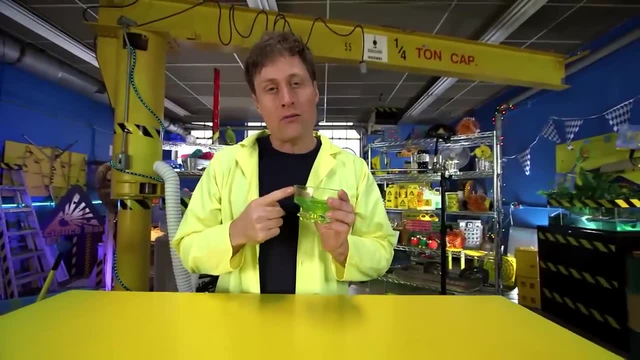 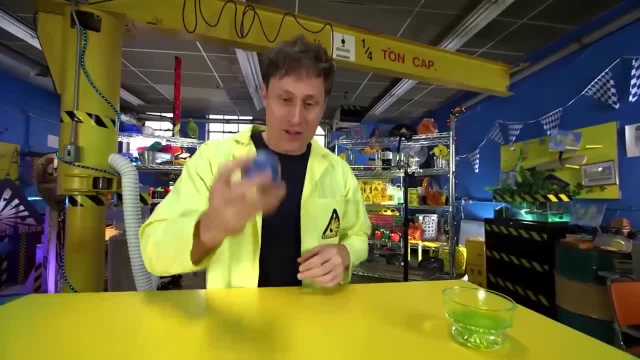 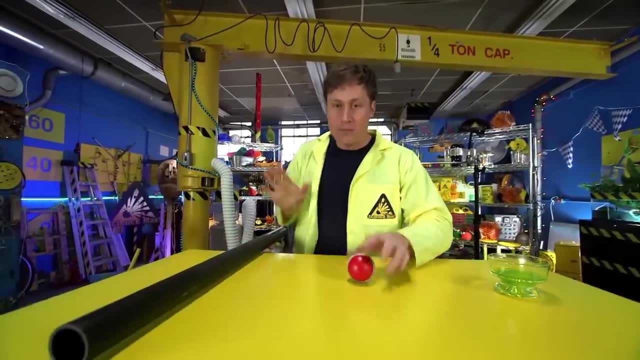 There's slime, obviously, and rubber polymers like well, like rubber, and there's also hard polymers like plastic. Now, polymers are all kind of constructed the same way, like this: This is a chain, Yeah. 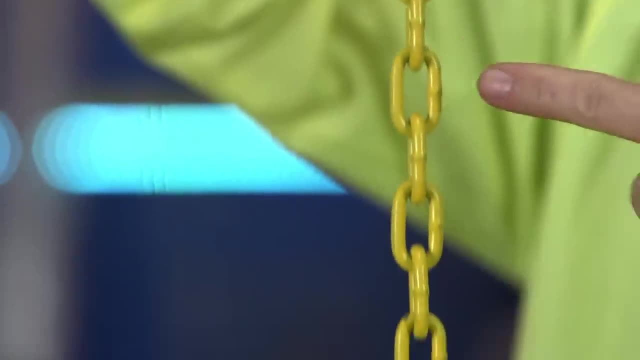 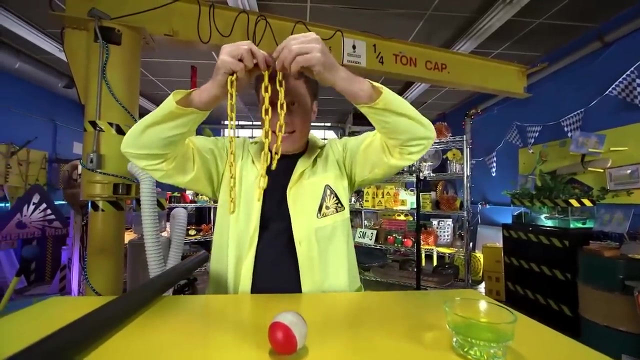 So imagine this is a chain of molecules and all the molecules are the same and they just repeat in a long line. Now, when you get a polymer like slime, all the chains are not connected or very loosely connected, which means that they can flow over each other like a slime or sort of like. 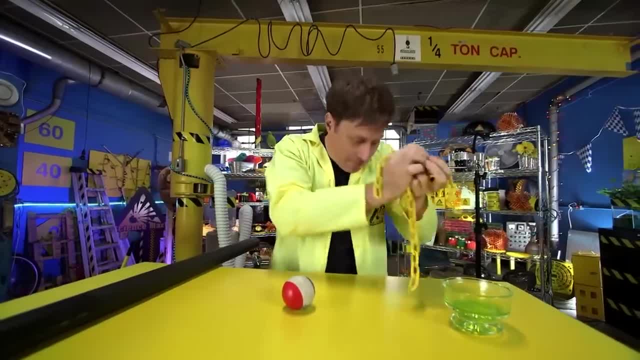 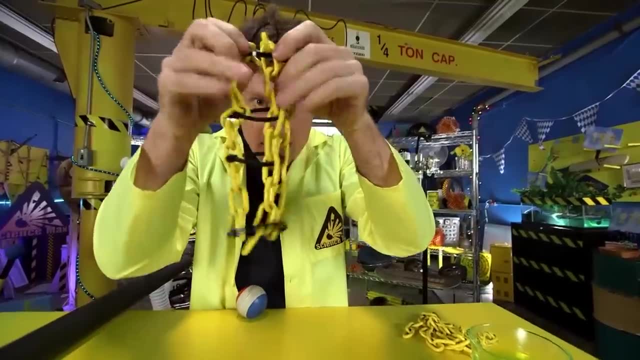 a liquid and they behave like that. So that is slime. But when you get to a rubber polymer you start to get little bonds in between the chains of polymers that work like this. You see, they still move around a little bit, but they can spread apart and they become 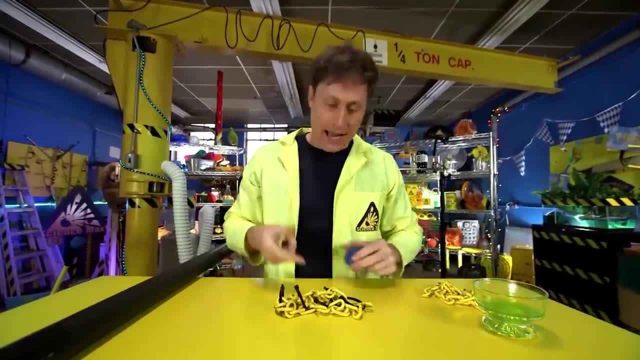 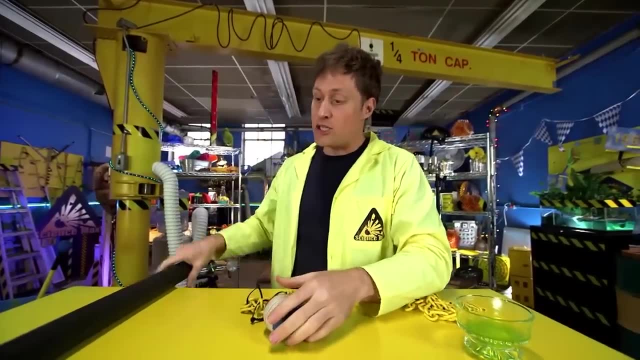 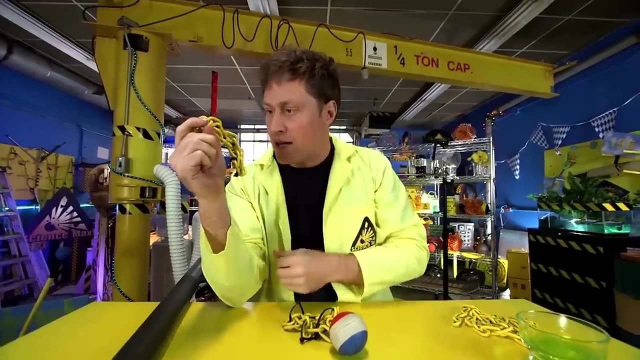 flexible and bouncy. Yeah, I know a chain doesn't really bounce, but rubber polymers do. Now, when it gets to a solid polymer like plastic, there's a lot more links and it's all kind of interconnected and it doesn't move at all. 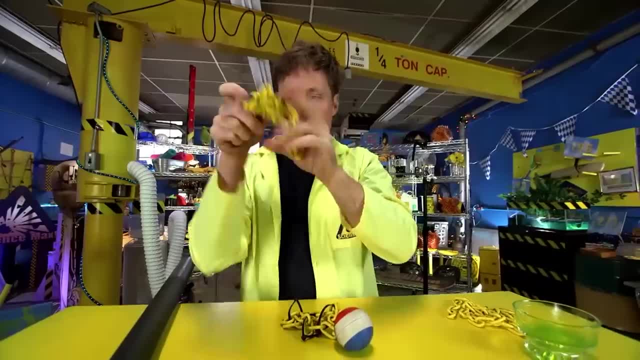 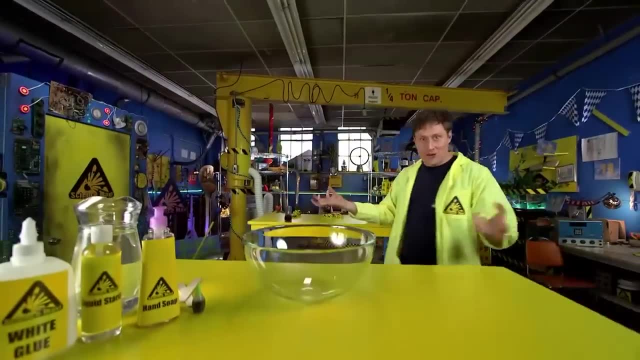 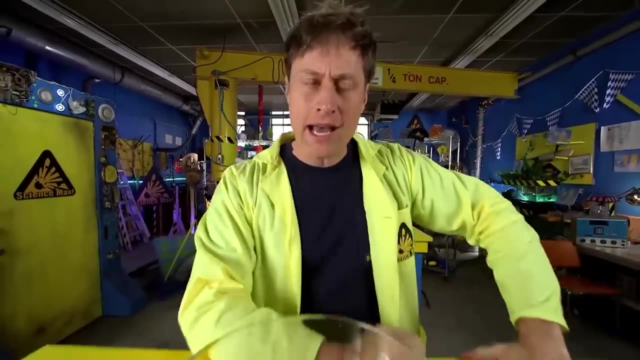 It doesn't move. Okay, again, harder to tell with a chain, but plastic is very hard and rigid. So let's dive into the world of polymers. Let's dig into the world of polymers and make some slime. Yeah too mad, not enough scientist. 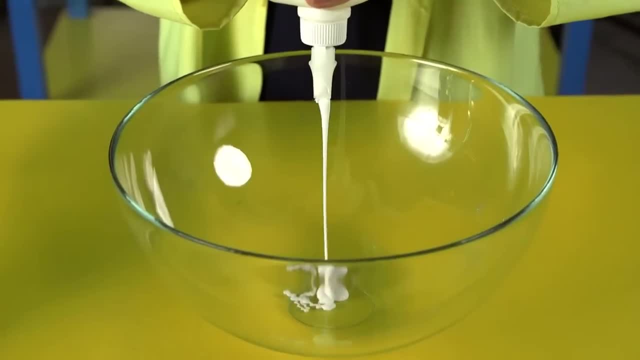 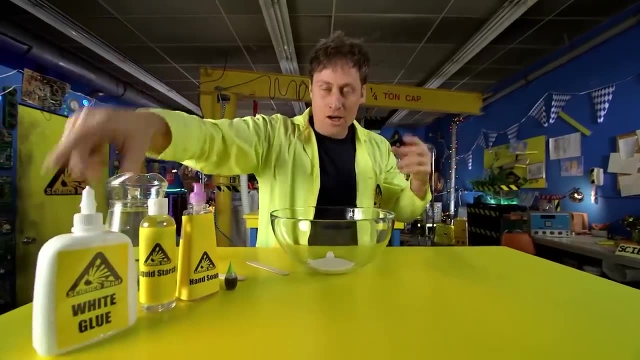 I'll keep working on it. Anyway, to make slime, take your white glue and pour in an amount. It really kind of depends on how much slime you want to make. Now you want to add about twice as much water as that. 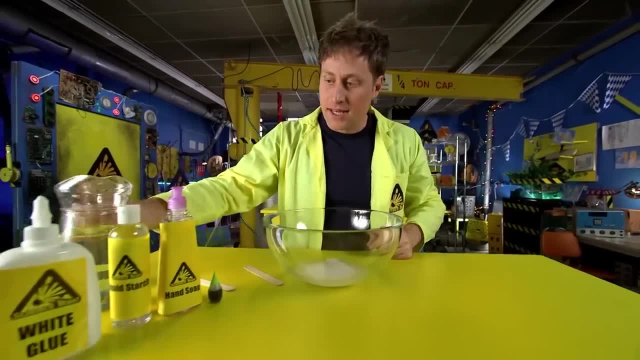 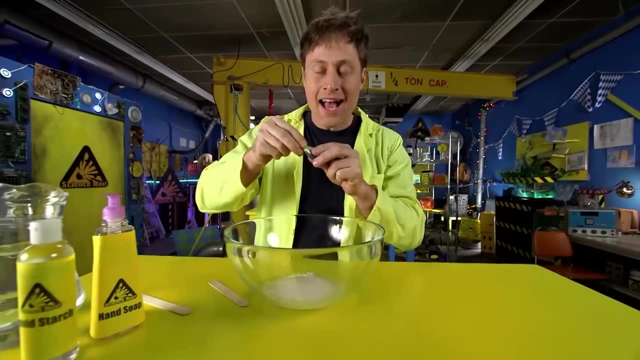 Somewhere around there. Great. Now we want to put in just a little bit of soap, Maybe there. That's good. And you want to put in your food coloring. I like green. Green seems like the right slime color to me. 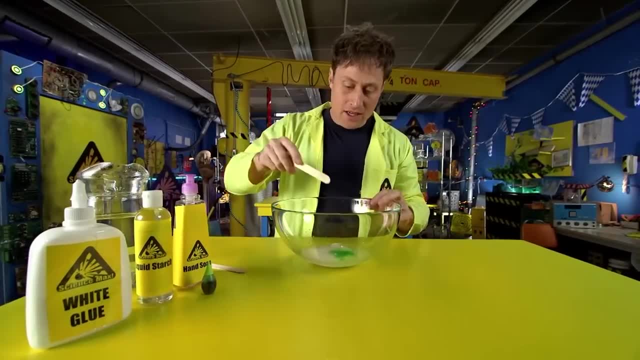 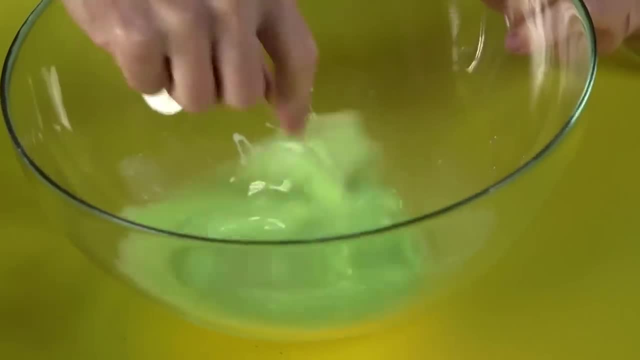 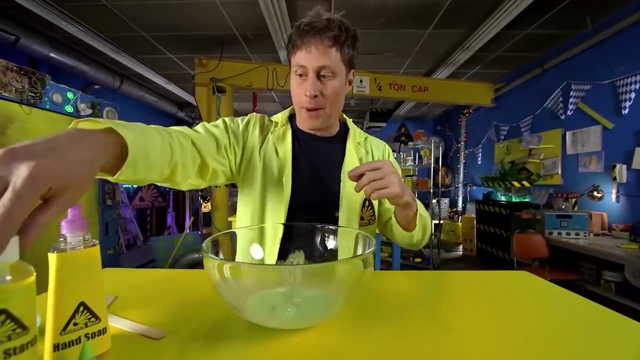 It's the right, appropriate mad scientist kind of slime. And then you want to start mixing that up until you get the right kind of consistency. That means make sure the glue and the water are equally mixed up. Good, And now we're ready to make it an actual slime by bonding the polymers together, by adding. 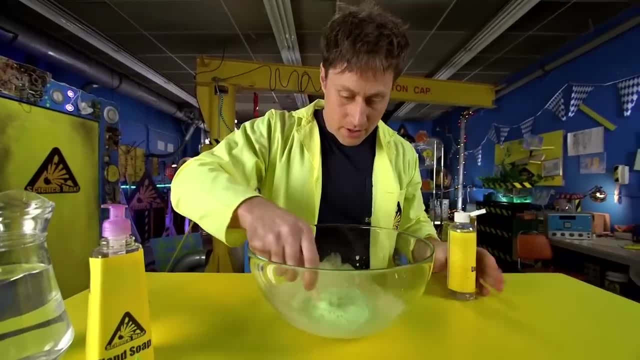 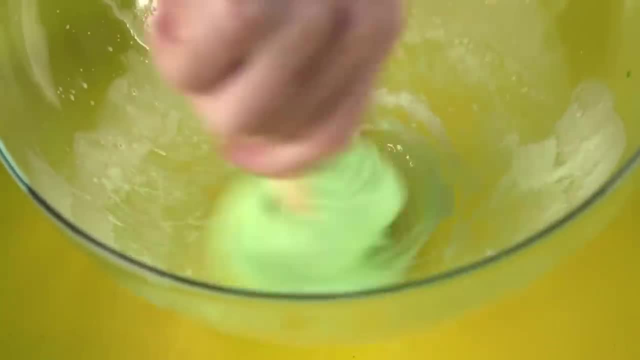 liquid starch Mm-hmm. Very good, And you want to mix it up. When you add the liquid starch, it starts to bond the chains of molecules together, changing it from a liquid to a slime. It's coming along And there you go. 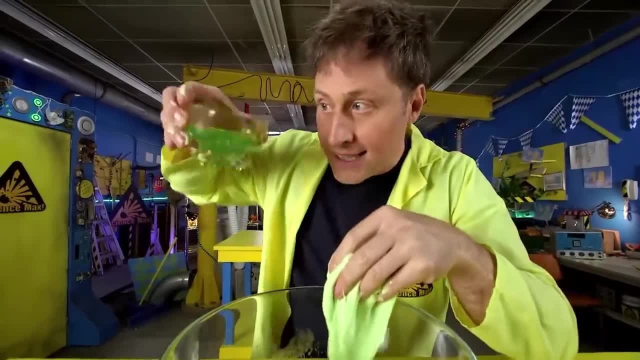 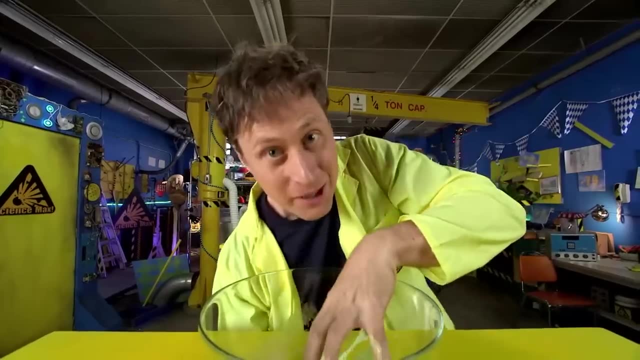 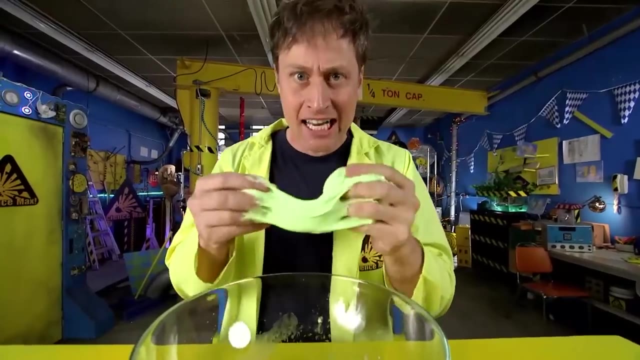 Slime. Now, if you want clear slime and not opaque slime, you want to use clear glue and not white glue. But that's basically the recipe. So there you go: Slime, Mwahahahaha To supervillain. 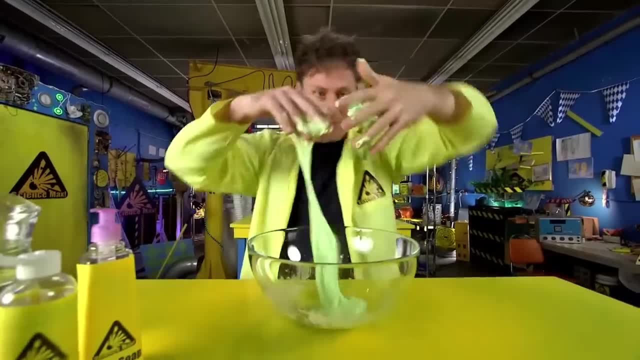 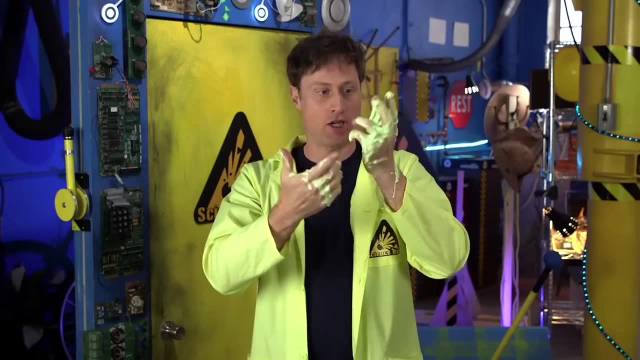 Yeah, Supervillain, Yeah, OK, Well, anyway, We got it All right. Now all you need is an expert to help me max it out. Of course, my interface is hand gesture based, so I don't know if the slime 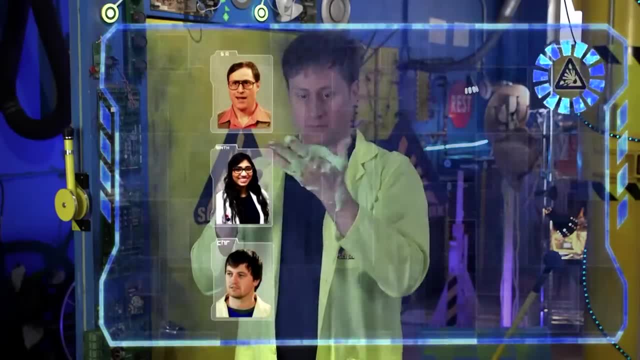 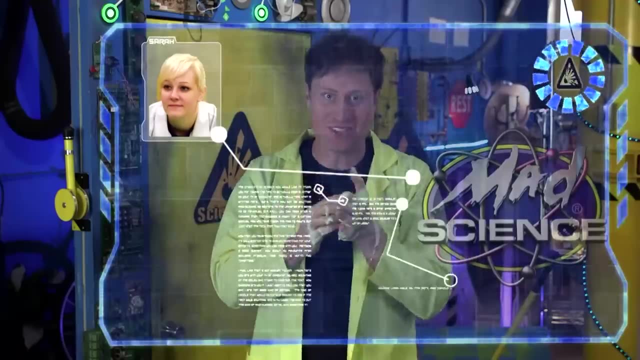 Oh, hey, There we go. Great, So you got it. Uh-huh Good. Oh, of course, Sarah from Mad Science. Mad Science, They really know their slime. This is great. OK, I got it Close. 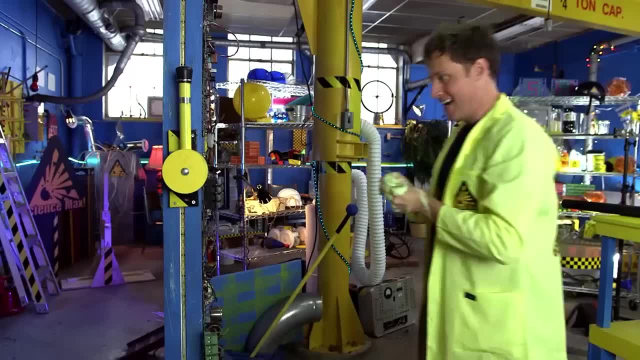 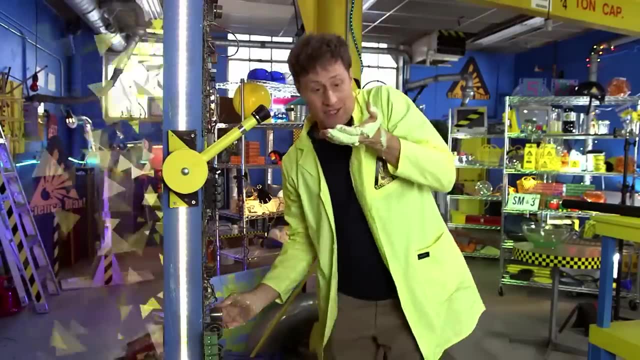 Close, Close. OK, There we go, All right. Ugh, I'm not sure if bringing it through the portal is such a good idea, but at least I'll have it on the other side. Ugh, I have a pot. 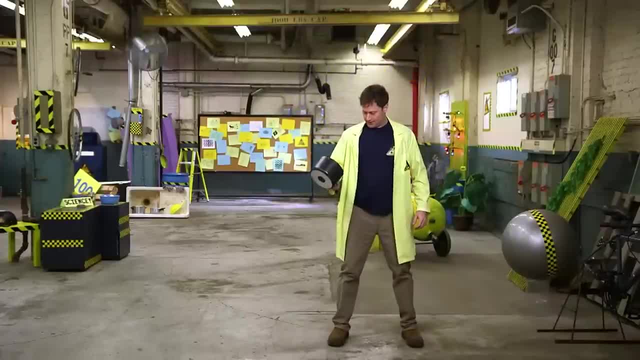 Why do I have a pot? I didn't have a pot when I went through the portal. Is someone somewhere missing a pot? Or did it just create this pot out of nothing? Huh, Hey, Sarah, Hey Hi. How are you doing? 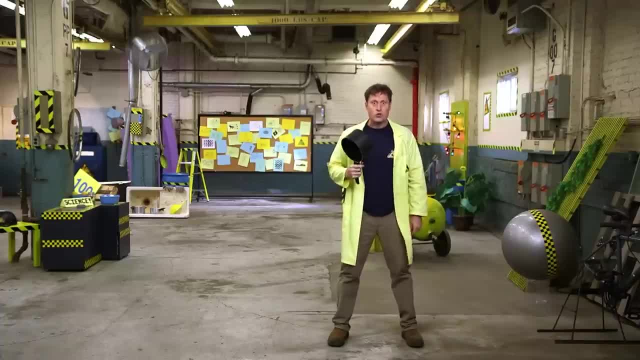 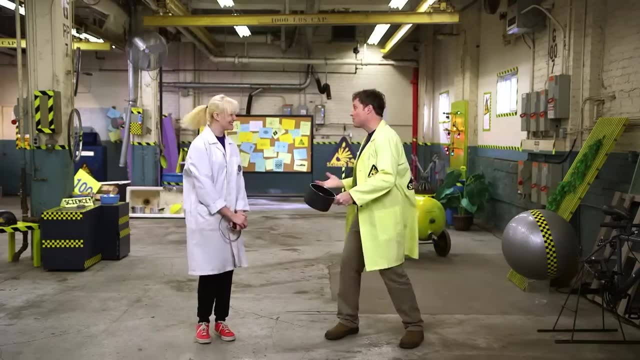 Good, Sarah from Mad Science, You're going to help me mix the slime. Oh, Oh, Oh, Oh, Oh, Oh, Oh, That's great. So, besides, you're going to help me make some slime. Yes, I actually brought some. 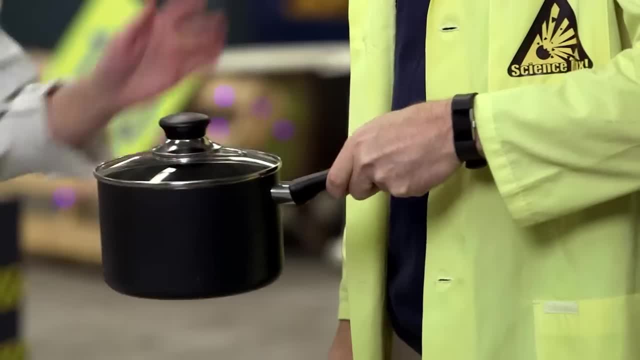 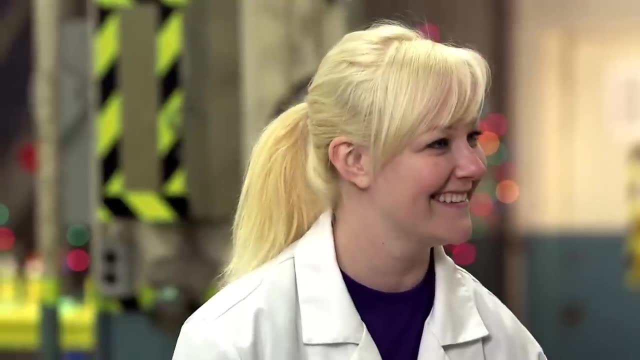 Oh, This isn't slime, This is a pot lid. Hey, Oh Well, at least we have a set. It doesn't answer any questions, though, and I guess we're going to have to make some more slime, Definitely. 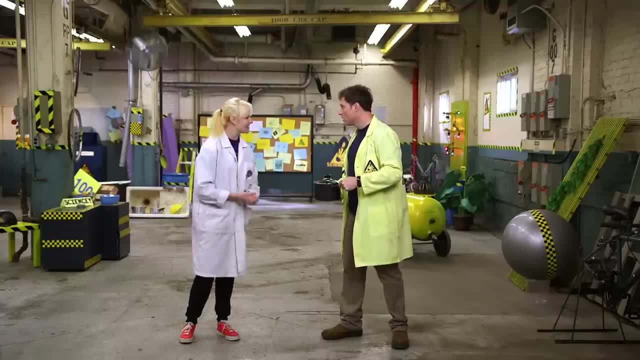 What kind of slime do you want to make? Uh, What do you mean? What kind? Is there more than one kind? Oh yeah, There are tons of different kinds of slime with lots of different ingredients and recipes. Oh, I only know the one. 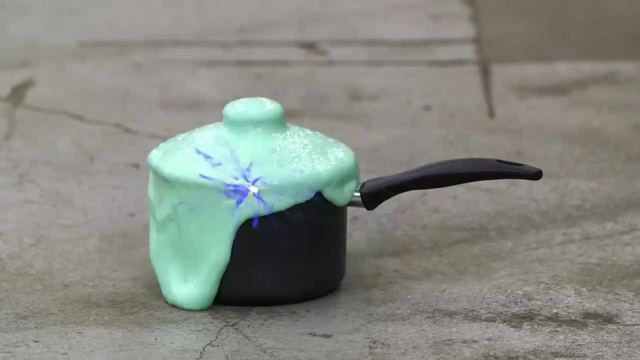 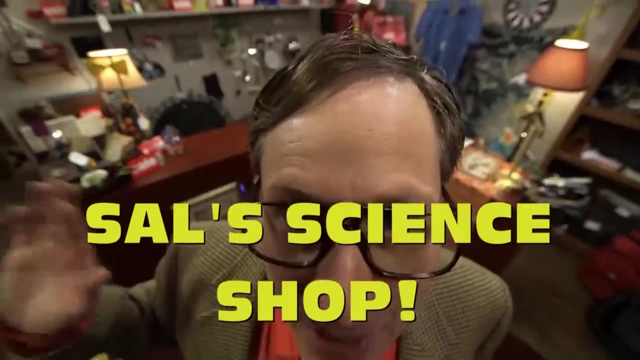 Can you show me all the others? Of course, Let's go make some right now. OK, Great, Awesome. Come on down to Sal's Science Shop and see me, Sal, while you shop for science. This week, only Sal's one-of-a-kind, once-a-year polymer sale. 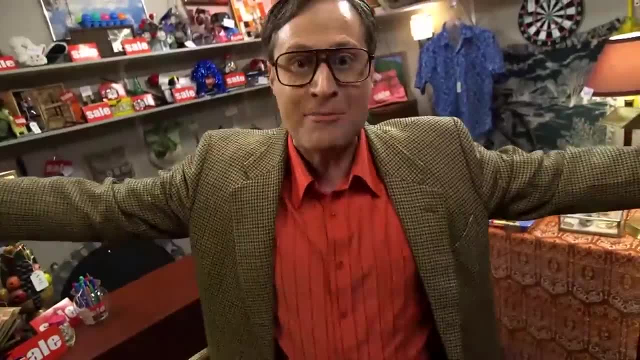 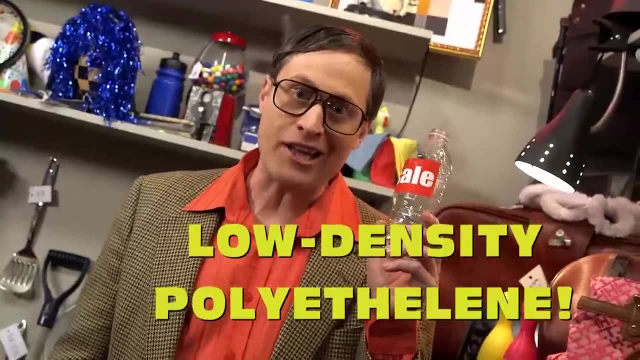 50 to 75% off anything made of polymers. Rubber, That's a polymer Polystyrene. When you're eating your next meal, I recommend some polypropylene- Low-density polyethylene- High-density polyethylene. You want some polytetrafluoroethylene? 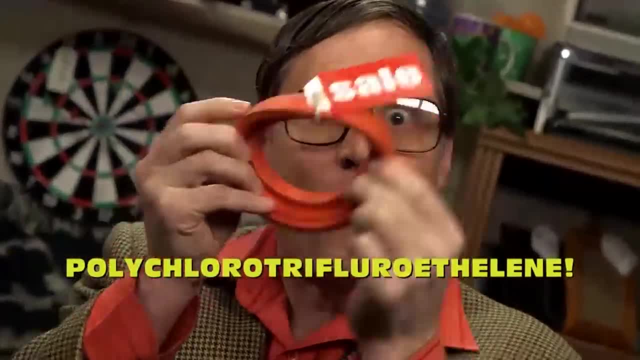 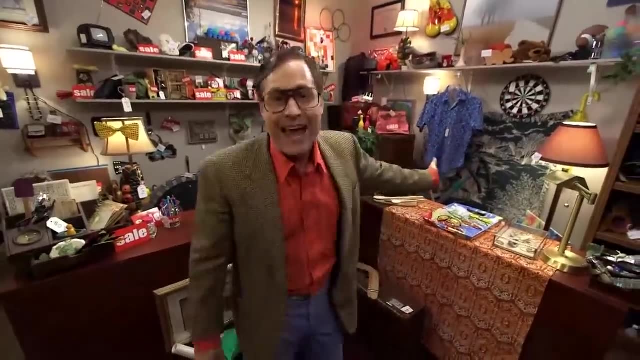 We got it. We've even got polychlorotrifluoroethylene. Do they even know how good a deal this is? Because you're not going to find that kind of deal just like every day. But hold the phone. Polymers aren't just plastics. 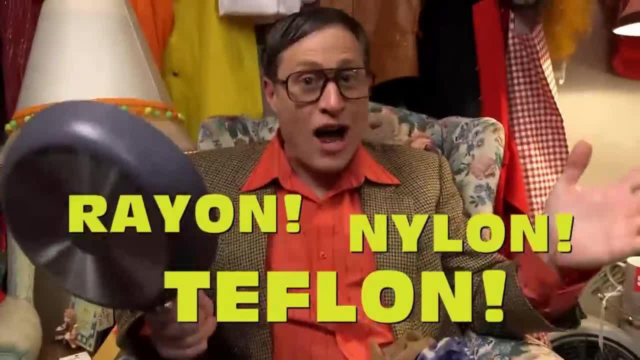 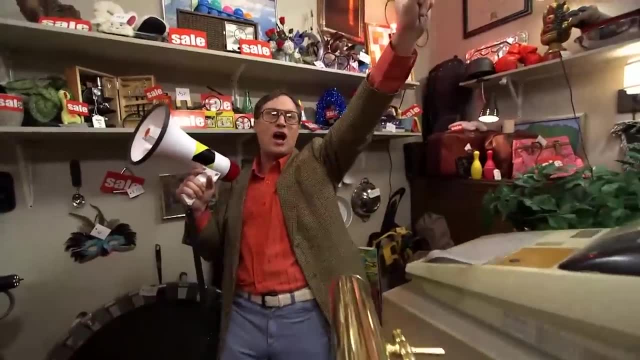 Rayon, nylon, teflon, you name the lawn. we got it on Sale. What do we want? Polymers? When do we want them? Anytime, during normal business hours. Wool, Silk, Even cotton, Polymers, polymers, polymers. 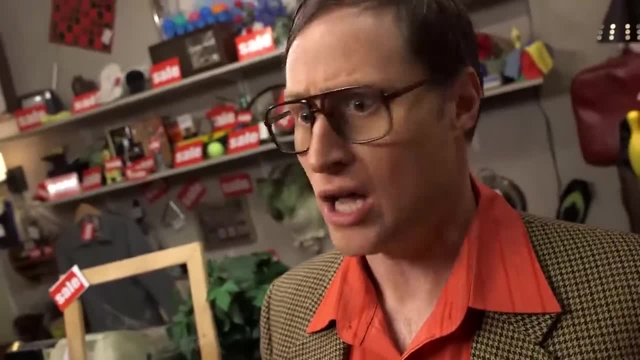 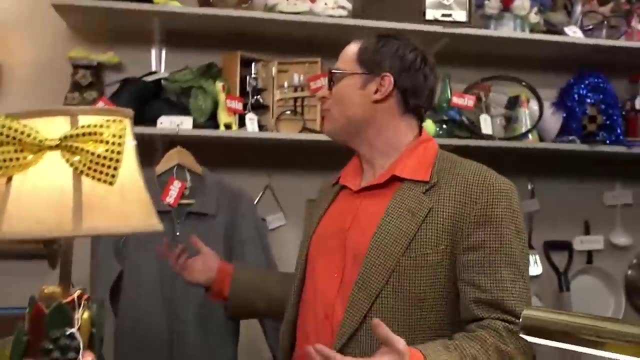 Polymers, polymers, polymers. Word is lost. all means. Glue, Paint, Umbrella fabric. Oh yeah, Carpet. You bet that's on sale, Roberta, I'm running out of sale signs. Buy it and I'll put it in a plastic bag, also made of polymers. 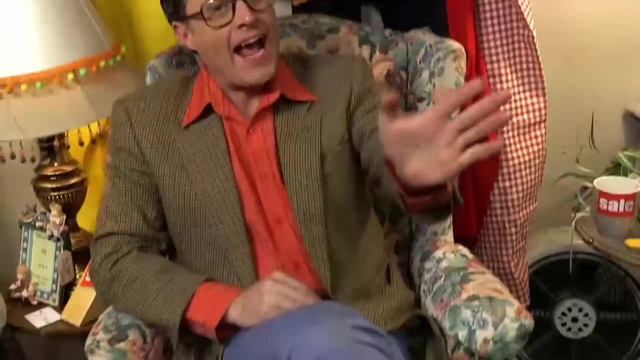 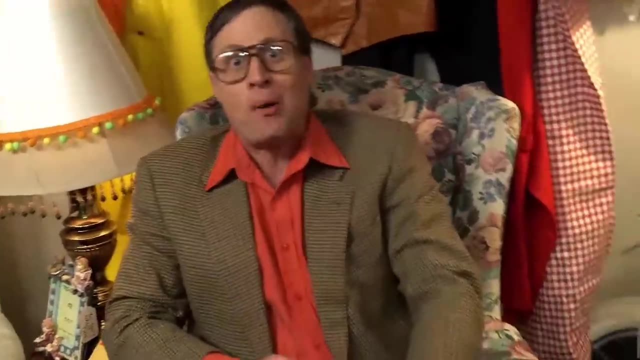 Seriously, Roberta, we can't have a sale on everything. Oh, hey, hey, even you, even me. the proteins in our bodies, even our DNA, all polymers. So come on down to Sal's Science Shop and get a great deal on your polymers. 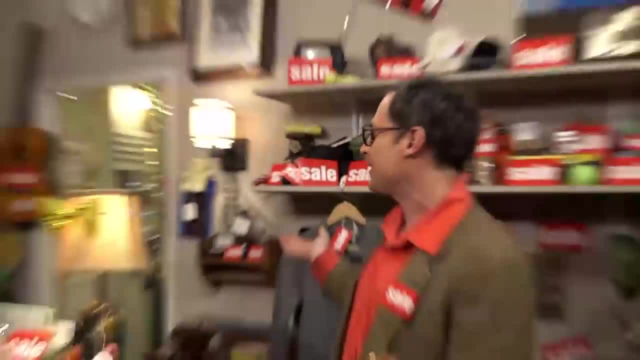 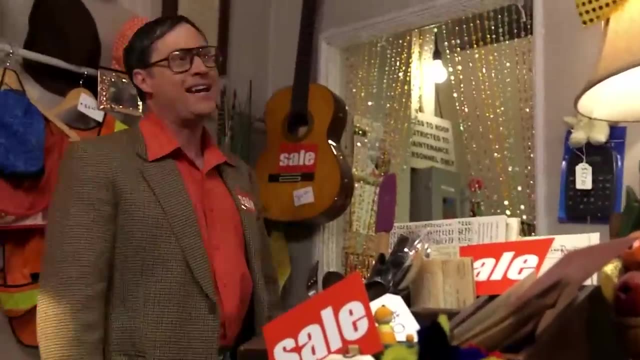 For a limited time. I mean, it'd have to be a limited time, right, Roberta? Because I mean I can't discount everything in the store to 75% off. How am I going to make any money? I mean, are we still rolling? 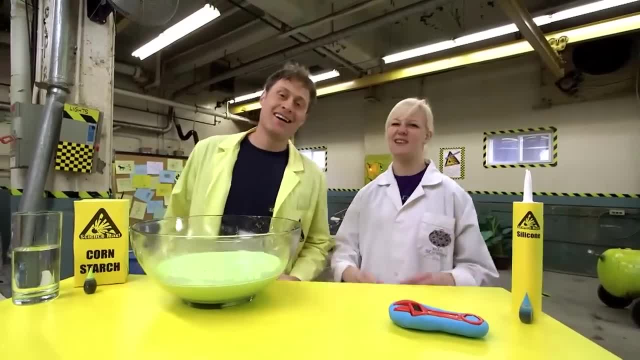 100 different kinds of slime. Yes, it's going to be so much fun, but we're not going to make 100 today. Yeah, I know we're just going to do our top favorites. Yeah, it's going to be super great. 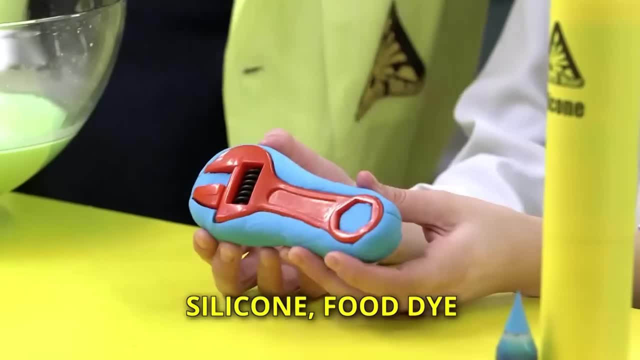 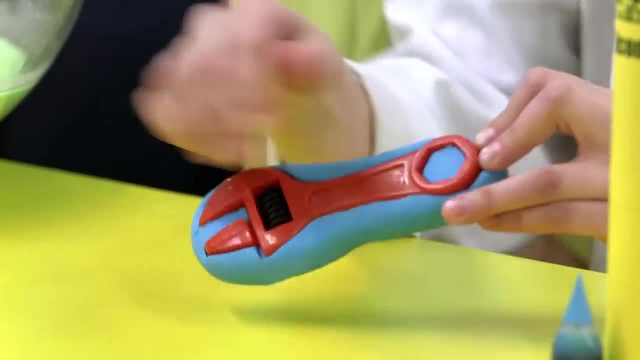 All right, what are we starting with? So our first slime we're starting with today is some really cool molding slime. Now, this slime, actually, if you leave it out overnight it'll harden and you can make an imprint of whatever you like. 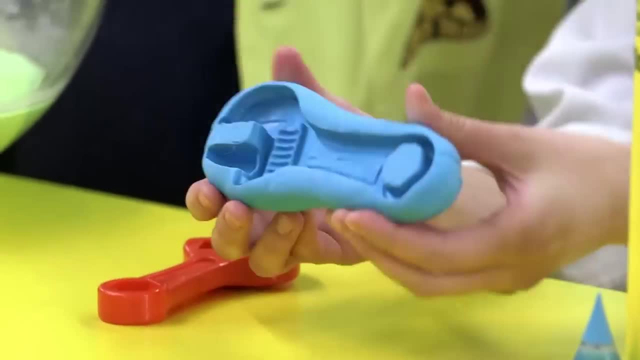 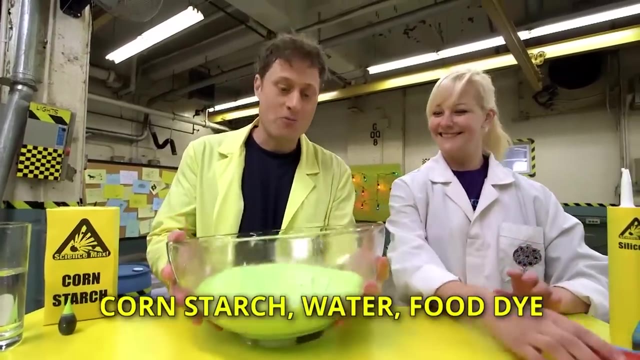 So here we made an imprint of our little tool there, So we're going to look at a little bit more liquidy slime, starting with this one over here which I believe you already know about. This is cornstarch mud, Exactly. 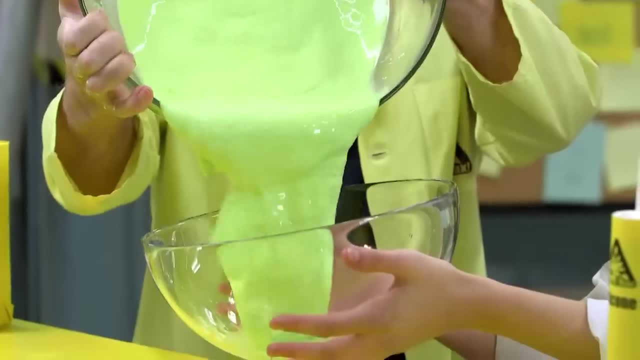 You hold, this Sounds good. I'm going to hold this and we're going to try pouring it. Whoa, Oh. so see, it's like a liquid, but then you do it fast, it's like a solid. 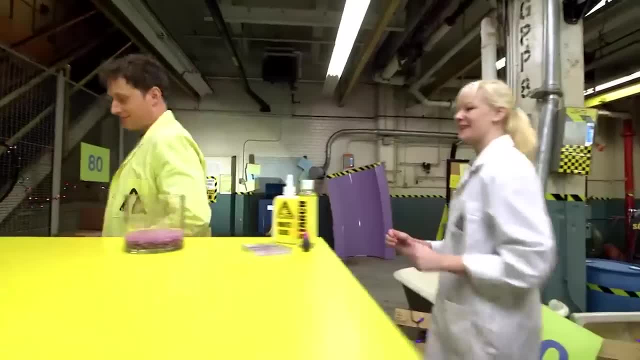 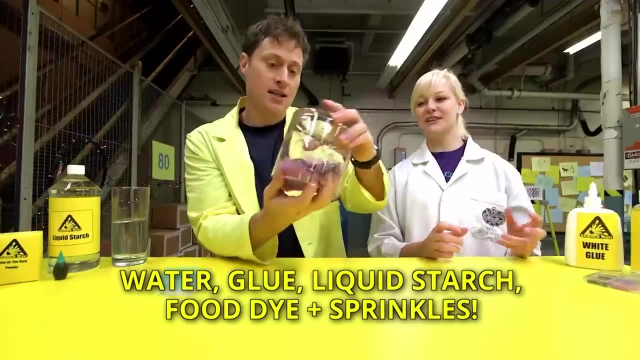 All right, what's next? Over here we have some other really awesome types of slime. So right over here we have some crunchy slime- Crunchy slime- Exactly Why is it crunchy? Now, it's crunchy because we've actually added a few beads inside of it to make it crunchy. 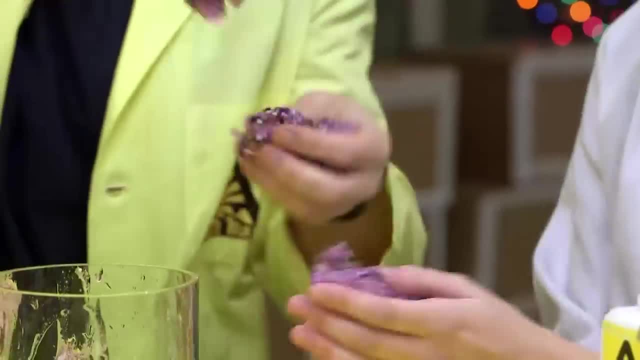 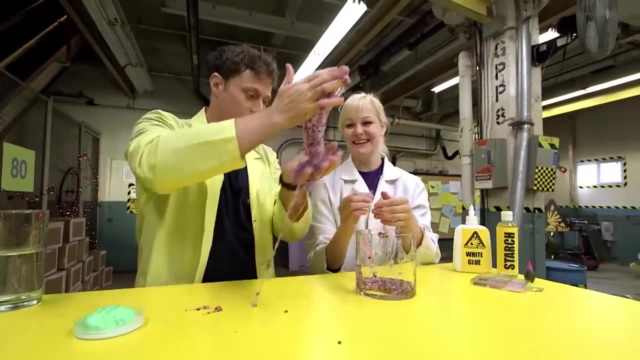 This is some really cool, awesome slime Here. you take half And you can feel the beads as you get to stretch it out. It's so cool. This is why this one is a little harder to clean. Exactly, I'll just do that. 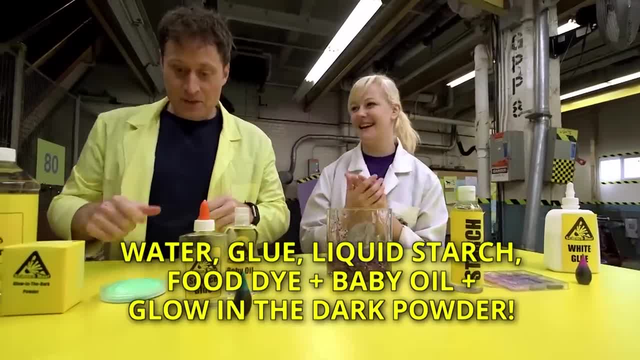 All right, so what's next? So next we have some really cool glow-in-the-dark slime. Glow-in-the-dark- Yeah, it's so awesome. Ooh, Look at how much it glows. That glows a lot. 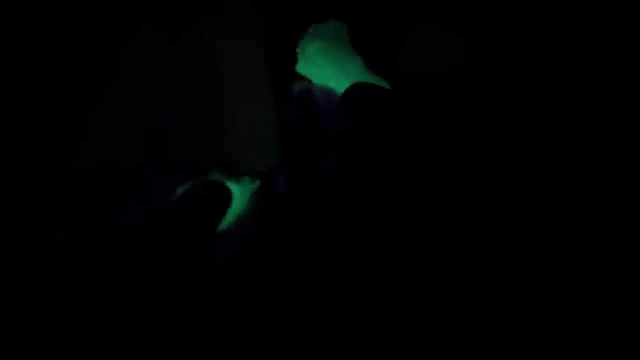 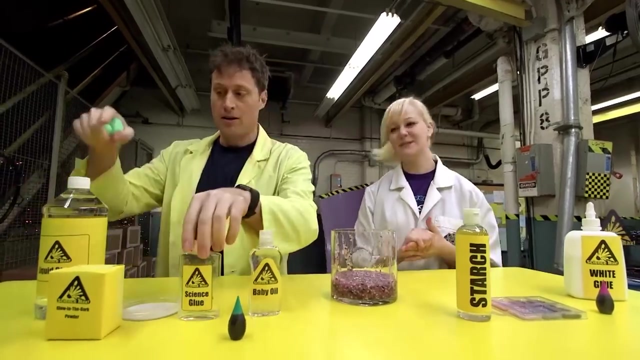 That's super glowy slime. So to do the different kinds of slime, we need the polymer, Yes, And then the thing that sticks the polymers together, Exactly So: the glue is the polymer. Glue is the polymer. 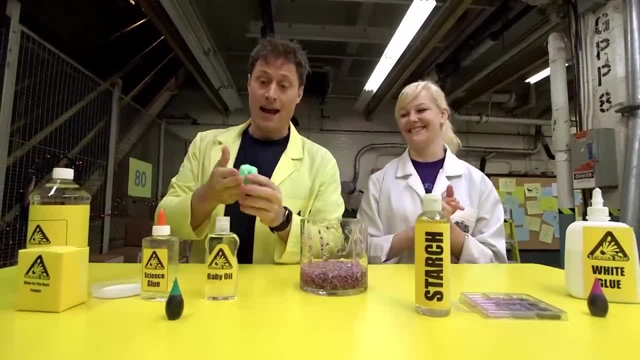 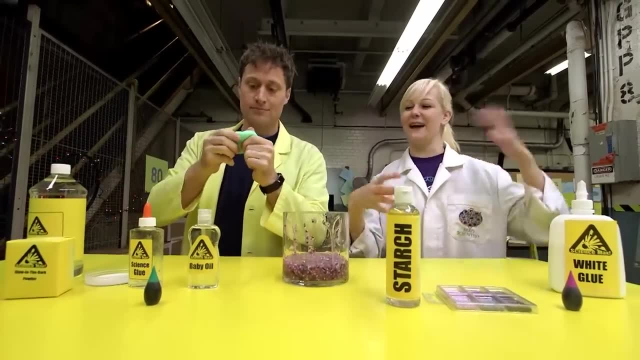 And the starch is the thing that bonds it. Yes, Uh-huh, There you go, And then you put the thing in that makes it the kind of slime. Yes, right before you add the bonding component, because if we keep adding stuff after it's. 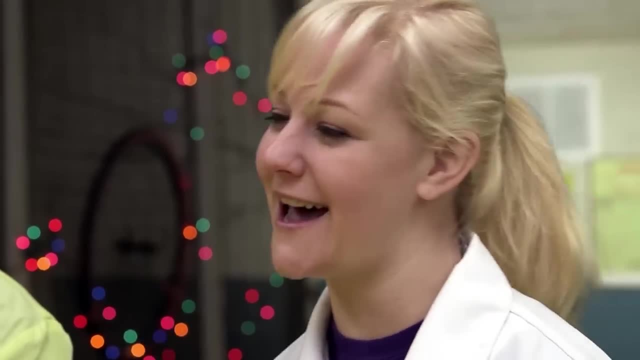 already made it unfortunately won't be able to take it, So we add our powder before we add our starch. in this situation, Should we go on to the next thing? Yeah, let's move on to the next one: More slime. 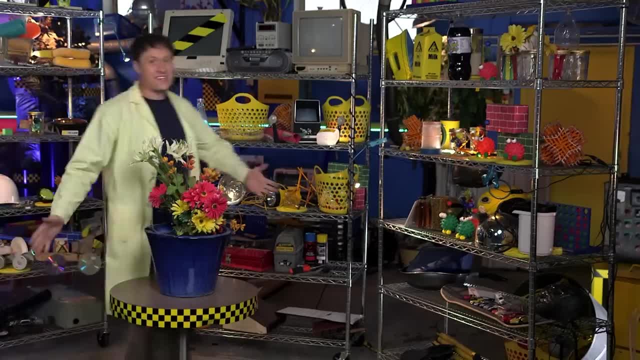 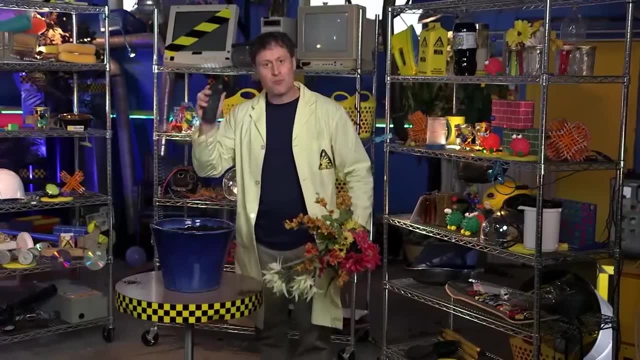 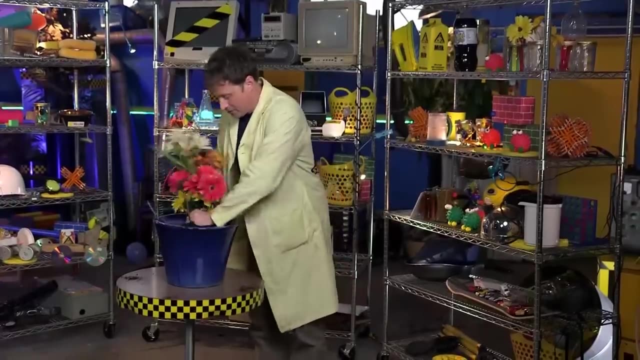 No, Max, Plastic is great and plastic is everywhere. But the problem with plastic is it isn't very biodegradable. It doesn't break down in the environment. I'm still on hold. Oh well, There you go. Not for another couple years, I guess. 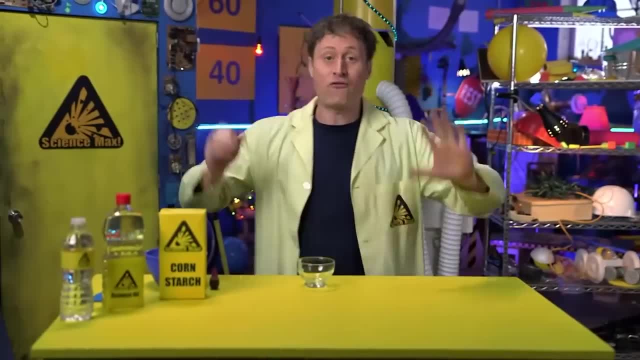 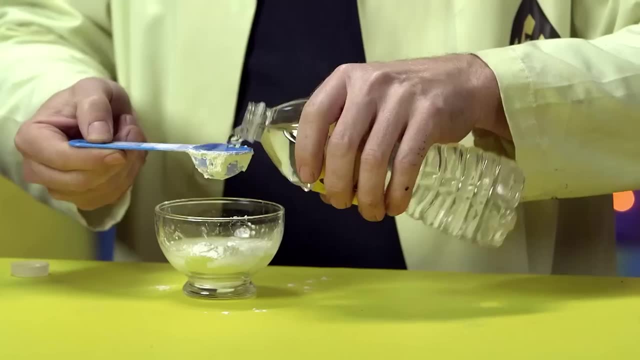 But here's a way that you can. You can make bioplastic. It's fully biodegradable because it's made of natural materials. The recipe is easy: Two parts cornstarch, three parts water, a few drops of cooking oil and some food coloring. 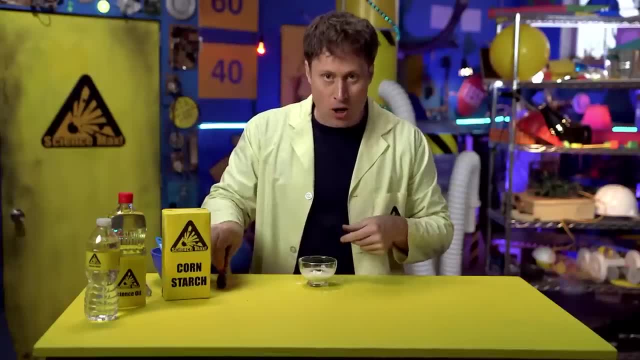 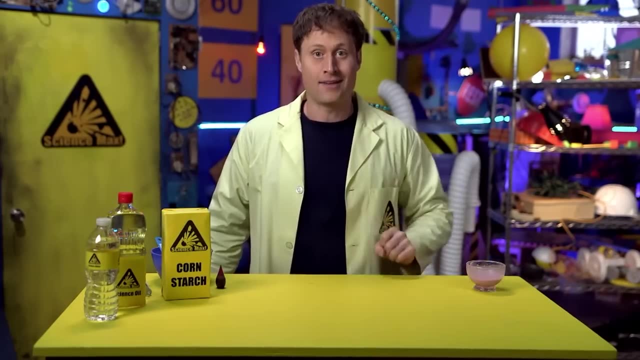 to make it whatever color you want. Purple Science, purple, Mix it up and it turns into a paste. Now what you'll need are two things: One an adult and two a microwave. Put it in for 30 seconds. 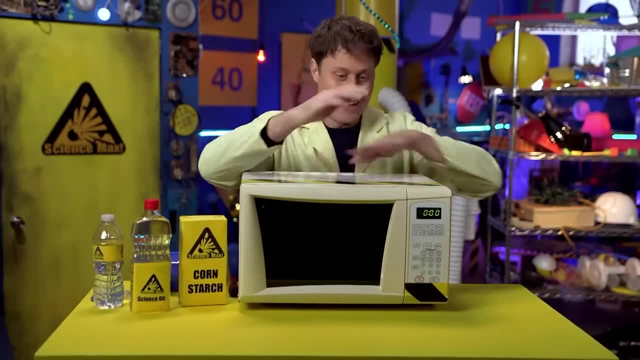 Clockwipe. There we go. Then take it out and mix it some more until it cools down. Then you can pull it out and use your hands to sculpt it into a shape or take the shape of something else. Once you put it all the way around, you can turn it into a little flower pot. 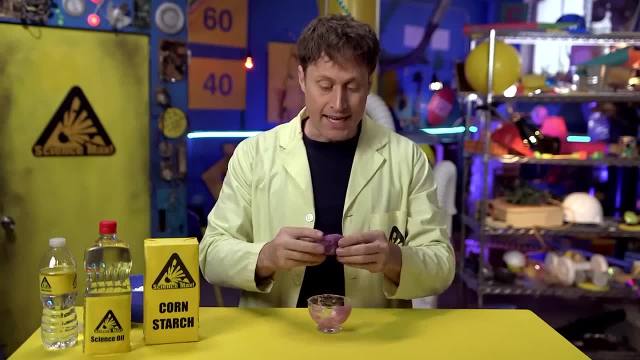 Once you've sculpted it, you need to wait for it to dry, which will take about a day. Clockwipe After waiting a day. Huh, What, It's been a day. Oh, It's been a day. It's been a day. 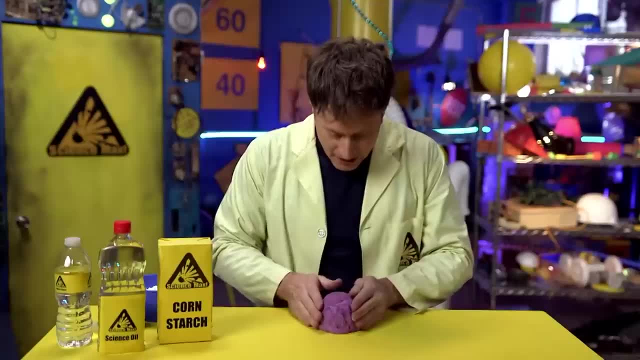 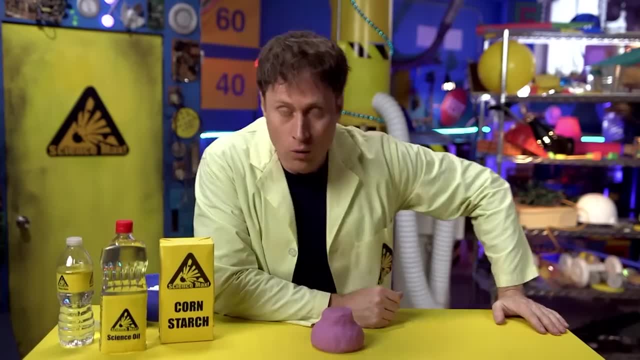 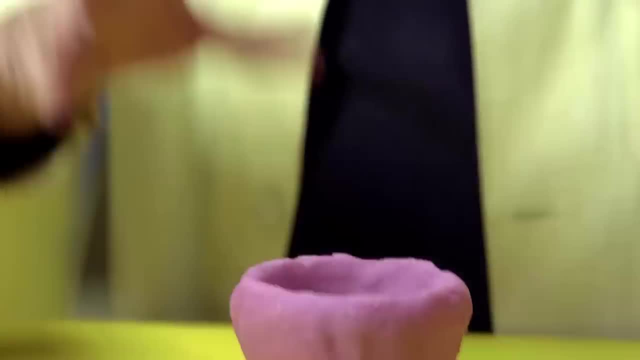 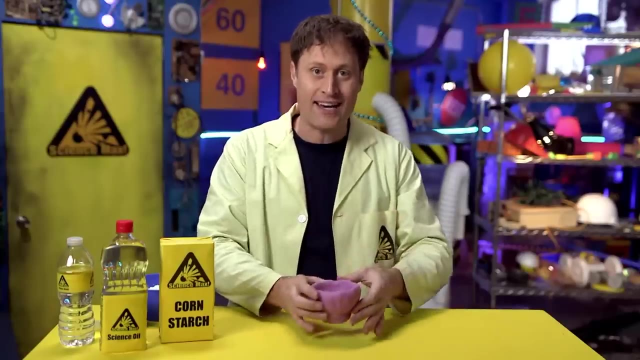 Oh, You have something made out of bioplastic like this little flower pot you can use to grow a small plant And then, when it grows big enough, you can take this biodegradable flower pot and plant it right outside in the dirt, and this pot will biodegrade and turn back into dirt. 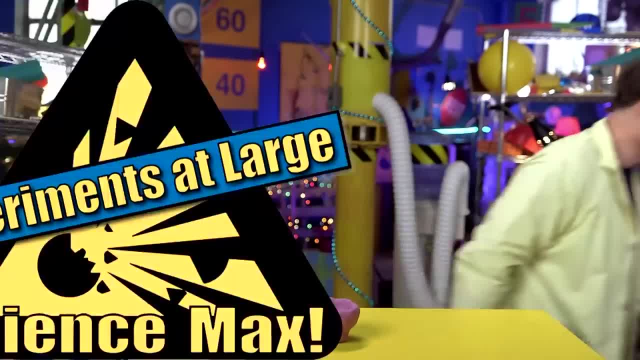 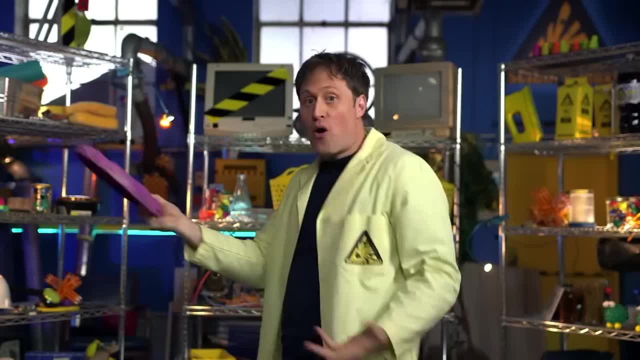 Pretty cool right? Well, let's max it out. Biodegradable Frisbee. Check it out. It's a frisbee, but it's biodegradable, So you throw it around in the park, but if you lose it it turns back into dirt. 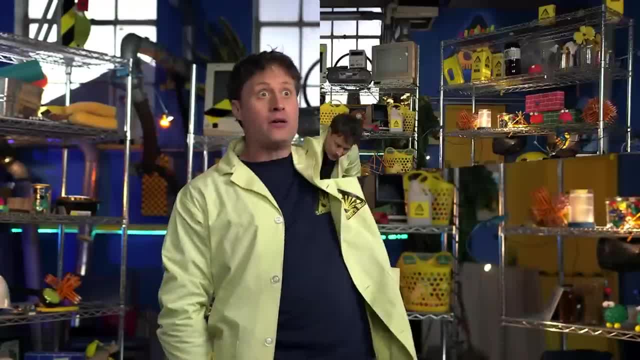 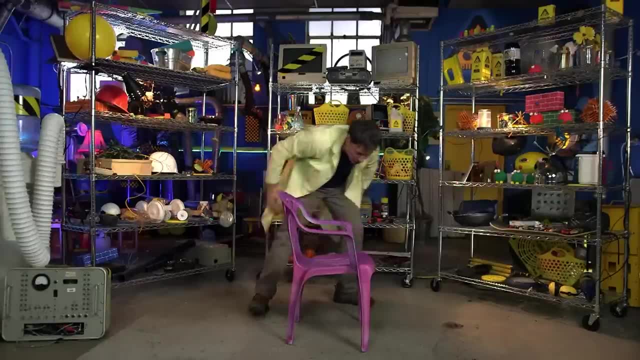 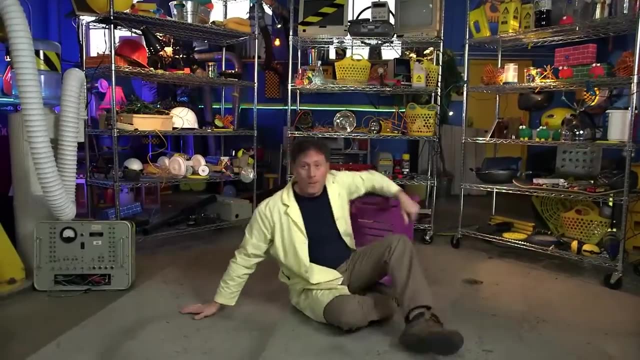 Ha ha, What, not enough? Okay, clock wipe Biodegradable lawn chair, Use it for one season and then return it to the earth afterwards. I think this is one of my best science Macs. Okay, bioplastic lawn chair. 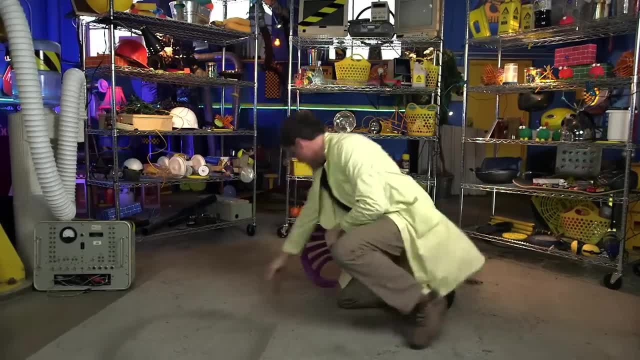 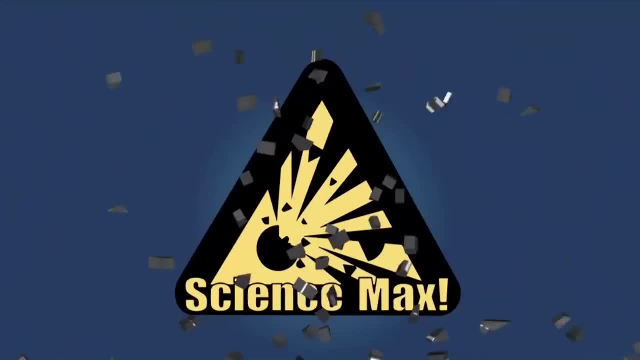 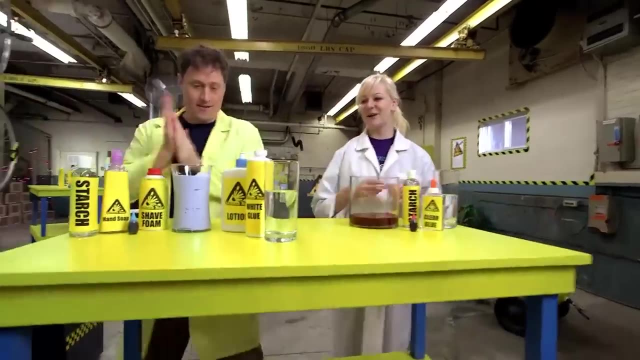 not as strong as regular lawn chair. We've learned that lesson now, so that's good to know. I mean, how would I have known if I hadn't tried it? Sarah and I are looking at different recipes for slime. All right, what do we got here? 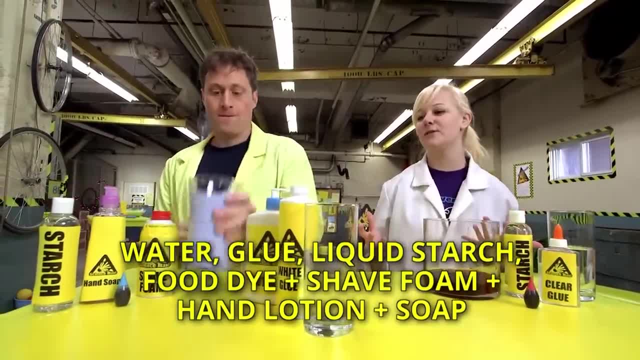 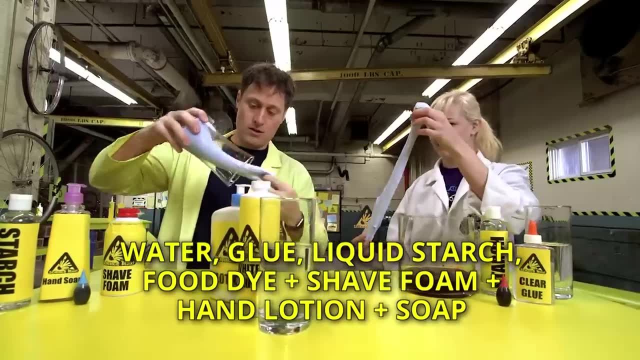 Over here. we have some amazing foamy slime which has so, so many ingredients in it Here. watch what happens when we start pulling it out: Ooh, wow. So it's like Super stretchy and super fluffy Here. 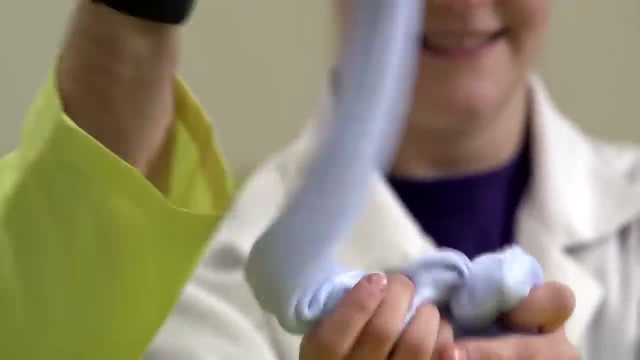 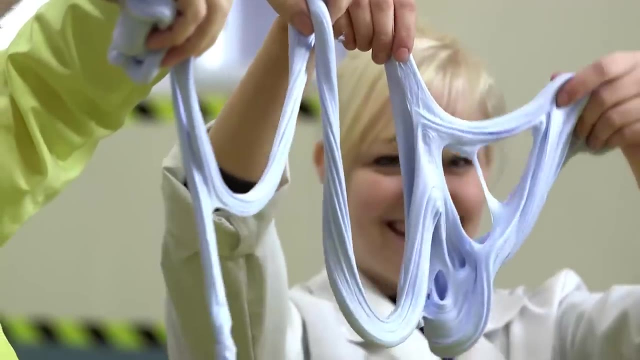 Oh, that's great. Okay, now you gotta hold yours, You gotta hold this end And then take some more, And then we take that And then, Yeah, It gets thinner and thinner and it becomes more and more lines of foamy slime. 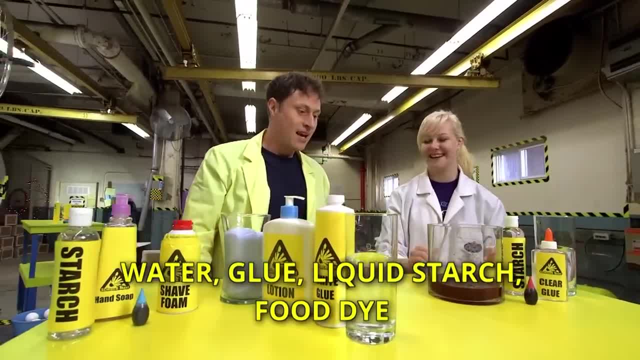 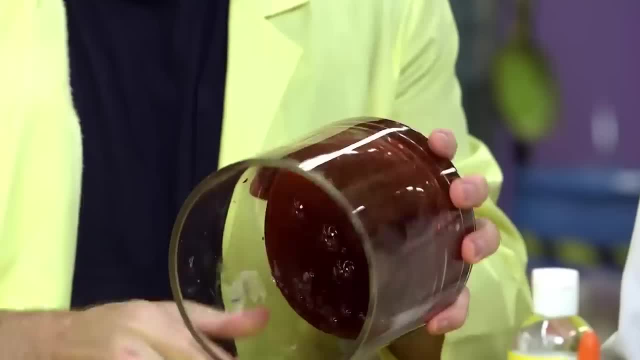 Yeah, And the last kind of slime we made today is some classic flubber slime. Ooh, It's so much fun. Now, why do you think it's called flubber slime? Because it's. Is it really a slime? It is a slime, yeah. 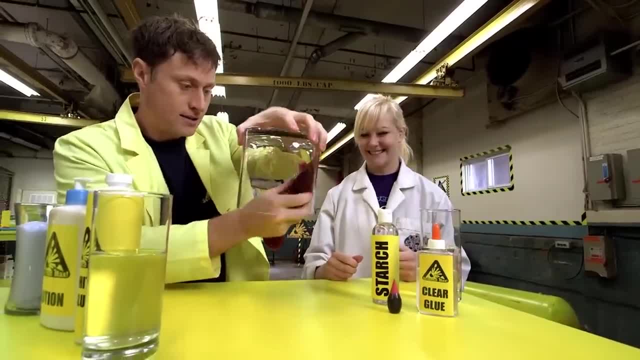 It's super fun and it's super stretchy. Oh, okay, I get it. Look at that And it's sort of like a little bit like gelatin. It is almost like gelatin. Here you can have some, There you go. 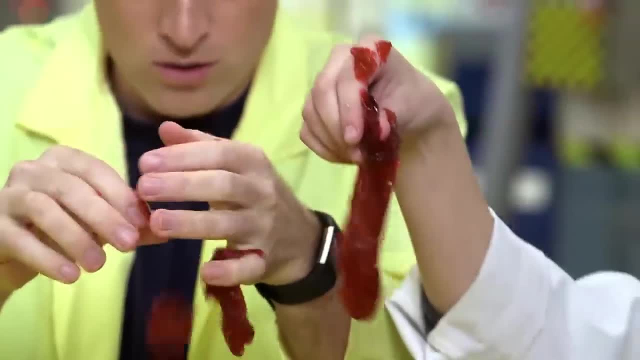 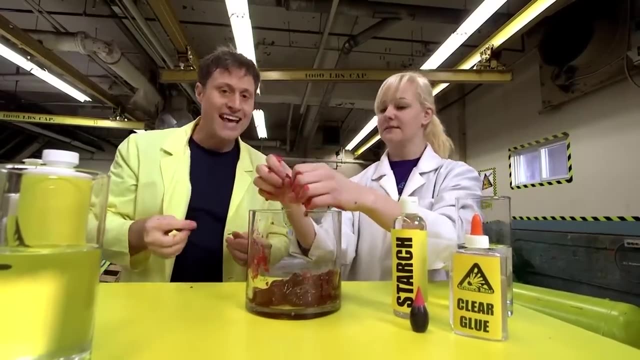 Whoa-oh-oh-oh-oh, Oh-oh-oh, All right. so, Sarah, now what we need to decide, Mm-hmm, is how we're gonna max it out. Right, Like, should we just get a lot of slime? 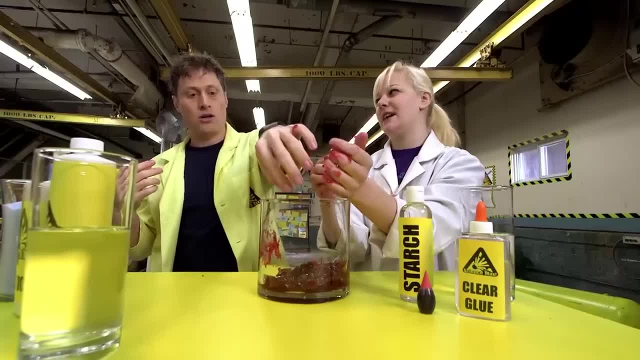 That sounds like a really good idea, but we are gonna need something to put it in, because we can't just have slime all over the floor. Okay, you're right, So we'll get some sort of container thing, Yeah, and we'll see how much slime we can make. 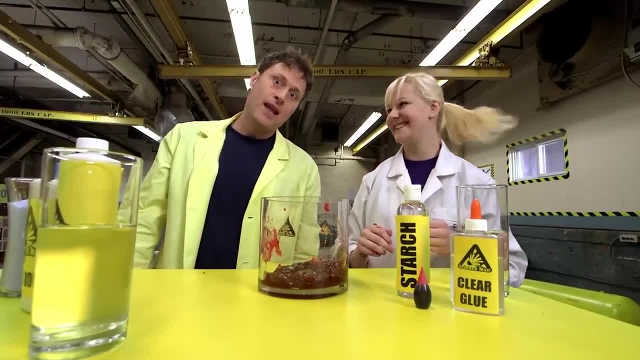 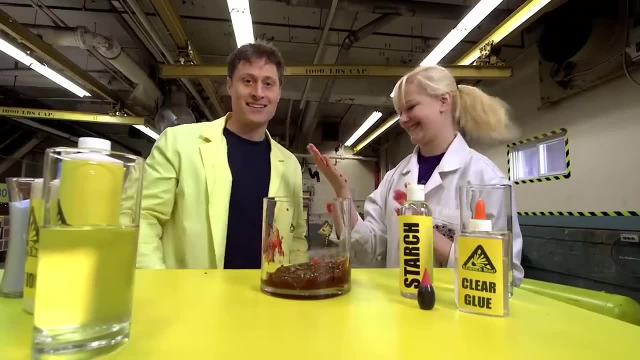 and then we'll just play with it and see what happens. Sounds good, And we will experiment, because it's science. Yeah, Okay, high-five, Careful, high-five, so we don't splatter. Okay, good, Okay, let's go. 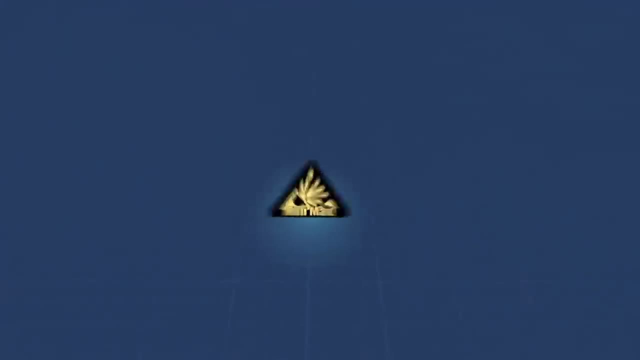 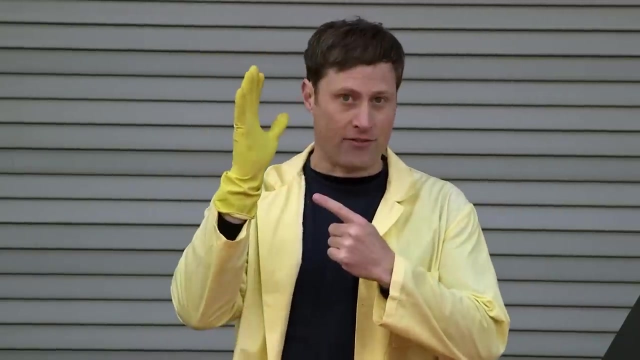 This is like: This is a rubber glove. Well, actually it's a latex glove. What's the difference? I will get to that in a second, but I'm sure you can agree it's super stretchy. How stretchy. 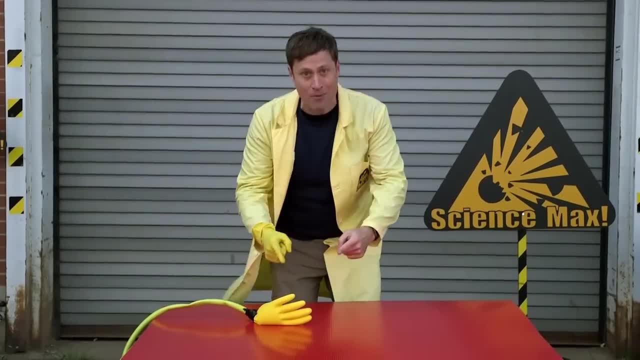 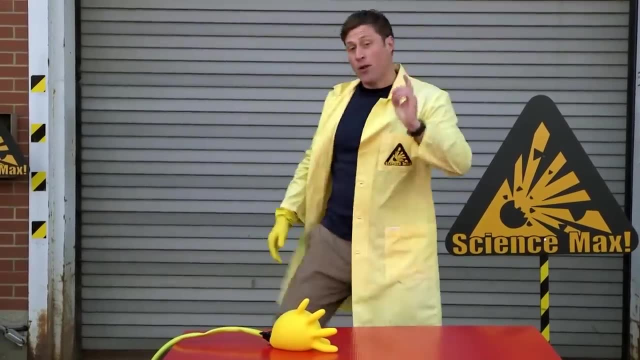 Let's fill a rubber glove with water and see how big it gets. So difference between latex and rubber. Well, it all comes from a rubber tree. Well, actually it's a fake tree. It's just to show you how it works. 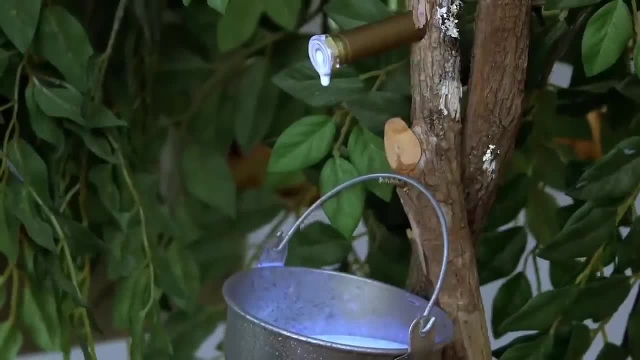 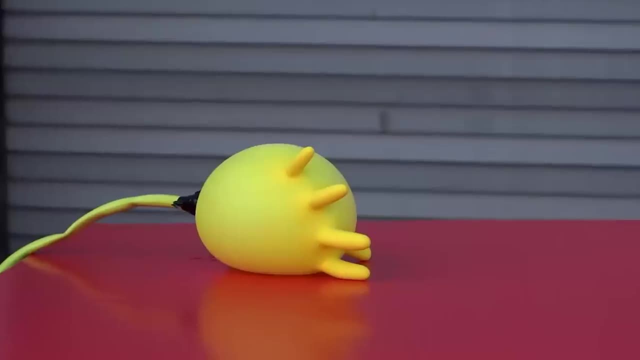 The sap of the rubber tree is collected just like this: There's a spigot and then the sap goes out and it's collected. It's the same way that the sap for maple syrup is collected. And this, This is natural latex. 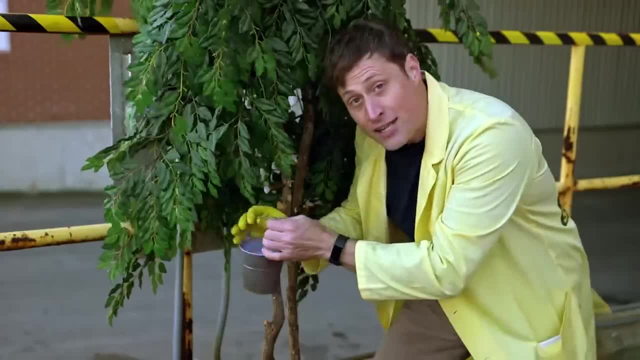 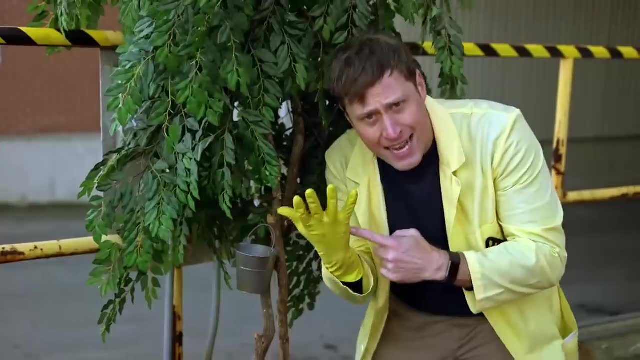 If it's dried out, it becomes natural latex. This is natural rubber. Latex generally means the liquid form and rubber means the solid form. But wait then, why is this a latex glove? The glove is not liquid. What's the deal? 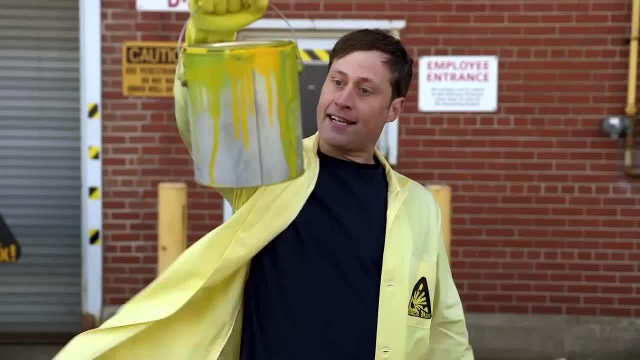 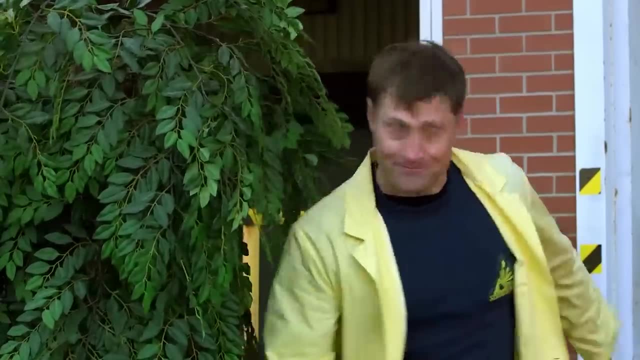 Well, generally latex means water-based or liquid, like latex paint, But it could also mean synthetic latex, That's latex that's man-made and doesn't come from a rubber tree, So we call rubber gloves rubber gloves because they used to come from rubber trees. 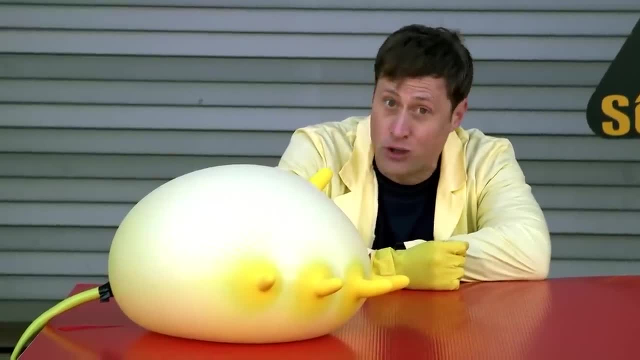 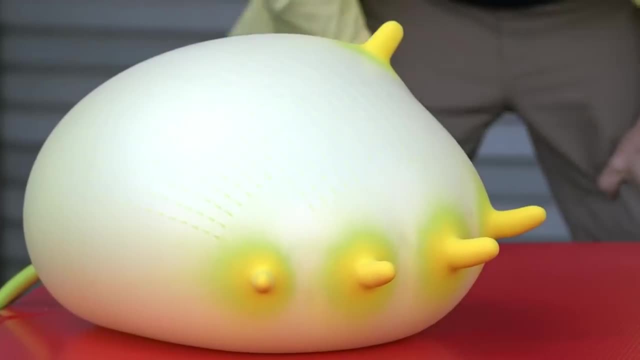 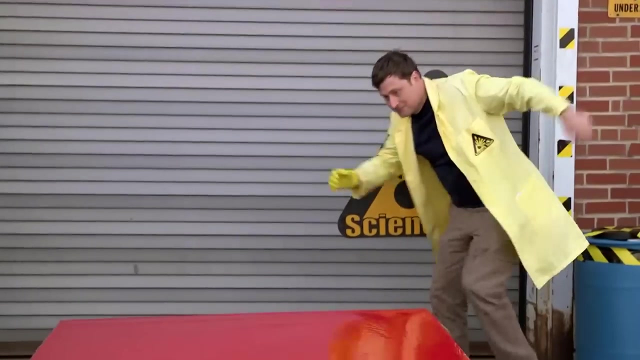 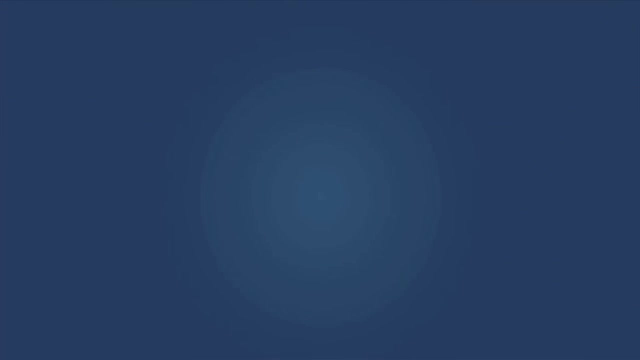 but now they're usually made out of man-made latex, But either way they're super stretchy. I wonder how big this is going to get Science. Sarah and I are maxing out polymer slime. How Maxed out tub of slime? 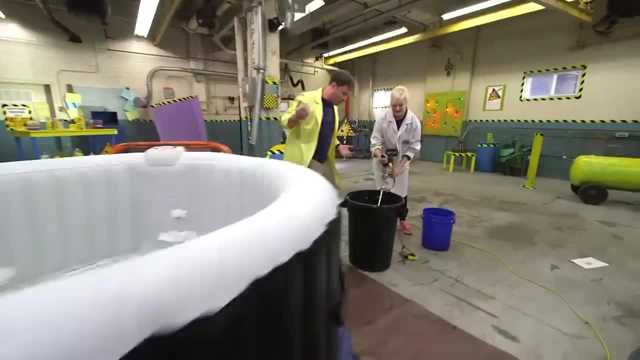 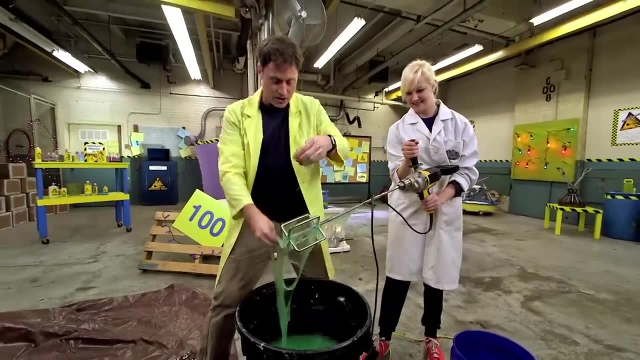 Whoa Okay. so how do you feel Is it? are we mixed up enough? First, we mix up a bunch of slime in a garbage bin. So with the polymer chemistry, the polymer is generally a liquid right. 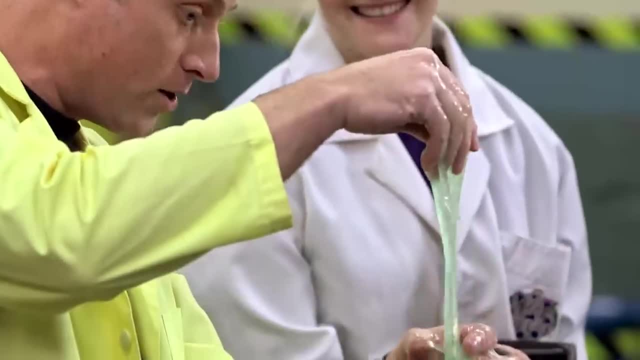 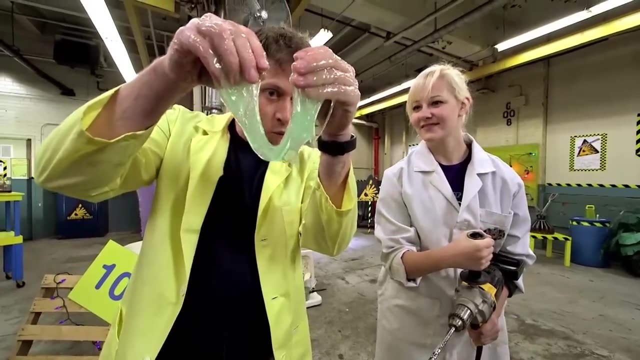 Yep, And the bonding agent makes it stick together. So the more we use, the more of a solid we get. Exactly yes. So we want to split it and make it sort of halfway between a liquid and a solid, and I think we're exactly at the right stage. 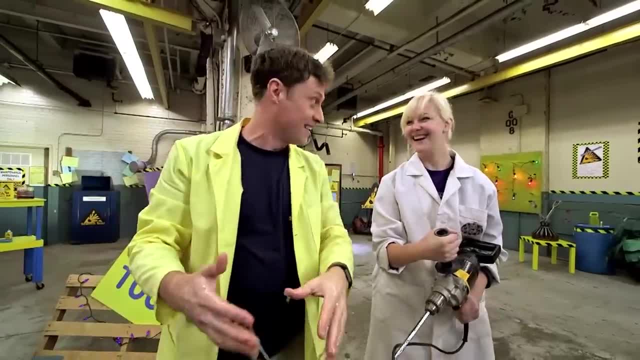 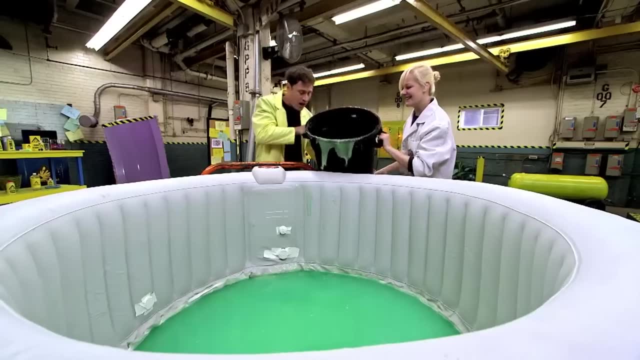 It looks perfect. Oh yeah, Okay, so let's dump this garbage can in. All right, All right, Then we dump it in. Ah, So gross Whoa. It turns out we needed more slime. Um, I don't think that's going to be enough. 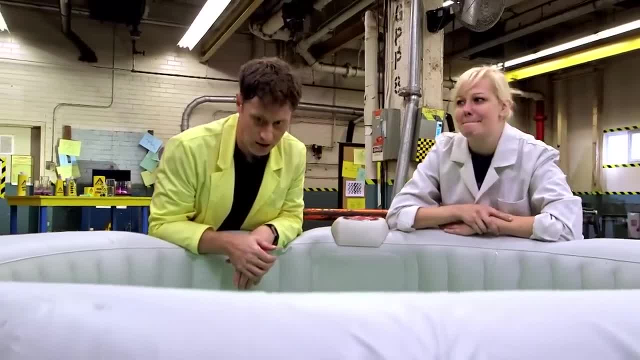 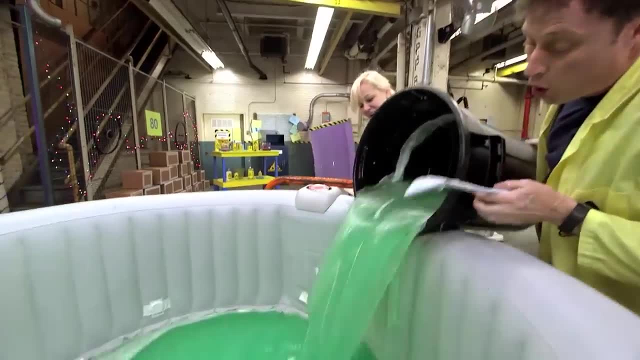 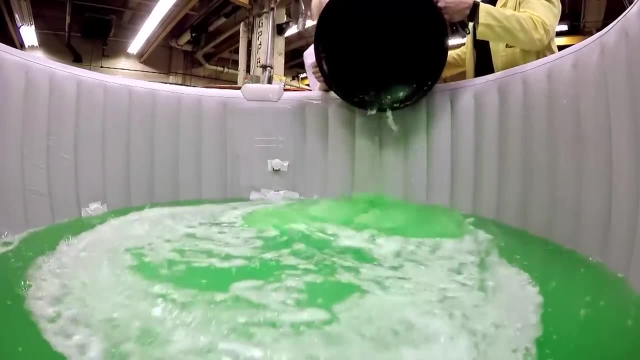 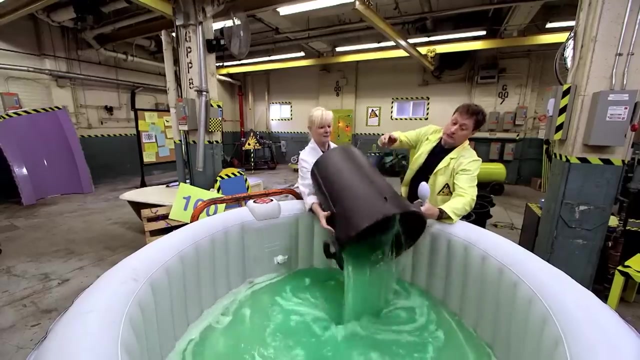 I think we might need some more slime. Yeah, how much more do you think we need? So we added 11 more. Ah, delicious, Ah, ha ha, Perfect, Yeah, Oh, ho, ho, ho ho. 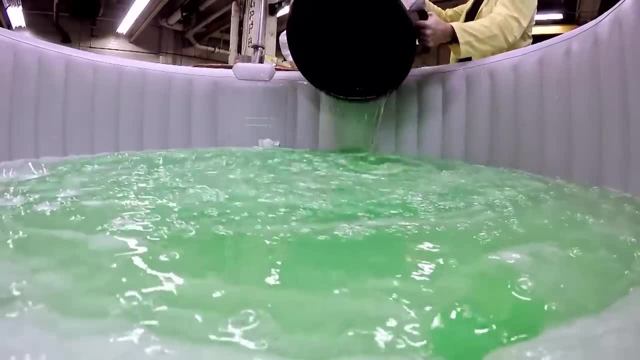 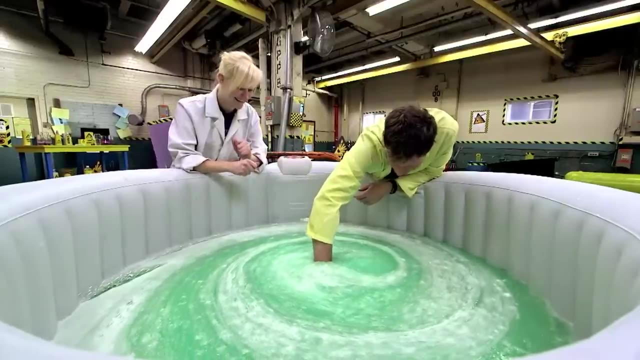 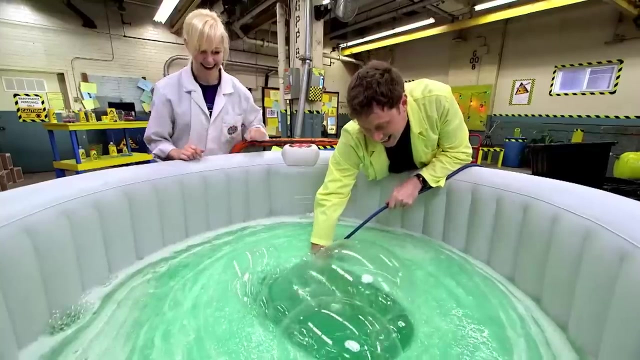 Last one, Last one, Oh yeah. Then we experimented. Oh yeah, We have a giant, giant tub of slime. Ha ha, ha, ha ha. Because the slime is stretchy, it created amazing bubbles. So do you think I could blow a bubble with the slime? 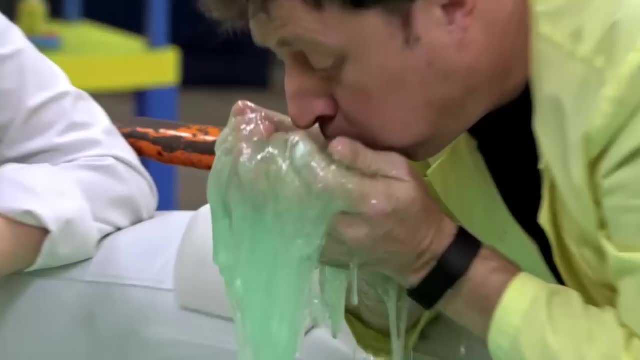 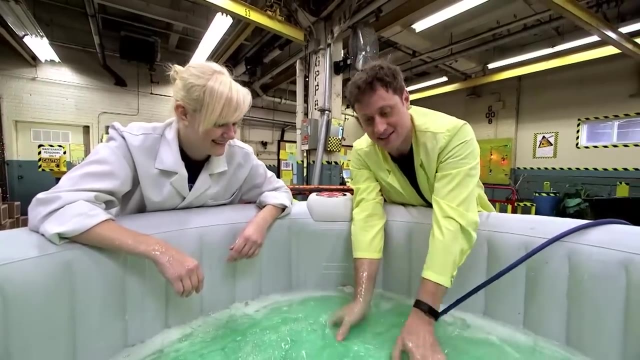 Uh-huh. Maybe not you, but definitely the air compressor. Do I want to try this? No, either. No, I'd have to just put it on my face. I think I've already got it on my face. Then there was only one thing left to do. 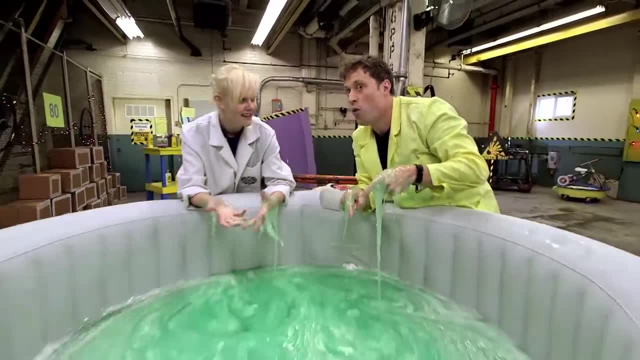 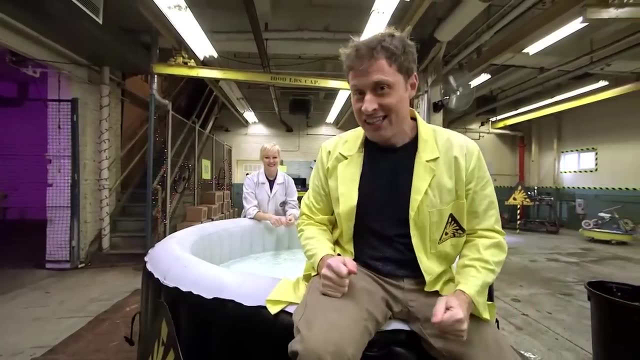 We get in the slime. Can we do that? We can totally do that. This is Science Max. That's so exciting: Going swimming in slime. Yes, Who's going first? You are, I am obviously All right. this is how Science Max does polymers. 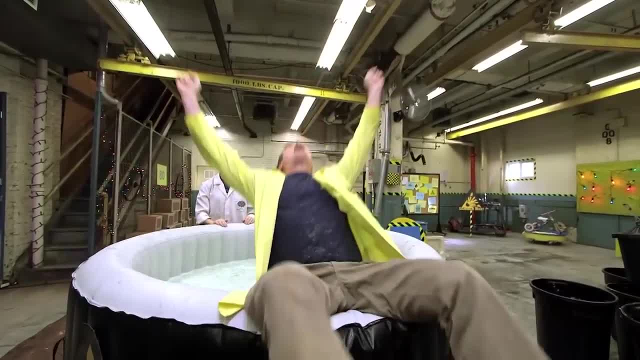 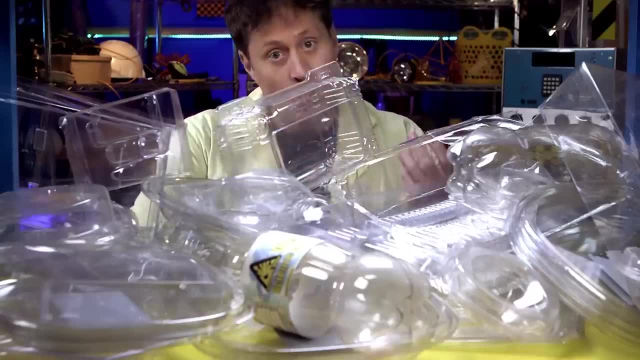 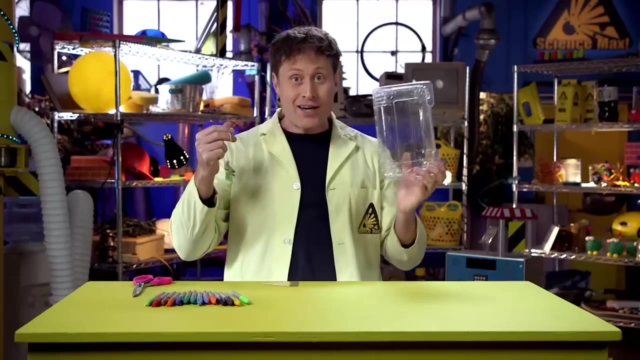 Three, two, one. Plastic is everywhere, but what can we do with it, aside from recycle it? Well, we can reuse it to make cool plastic charms, But you're going to need the right kind of plastic and you need polystyrene. 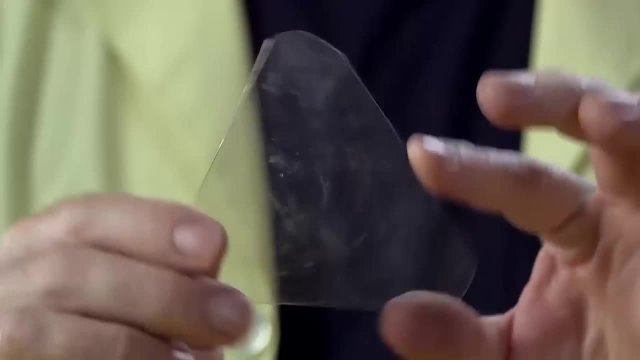 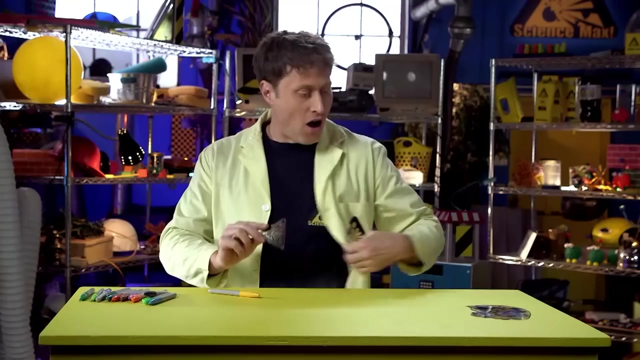 Just look for the little number six inside the recycle symbol. Cut out some plastic and decorate it however you want. There we go, Ha ha, check it out. The Science Max logo Logo. Also, I've made a couple other things. 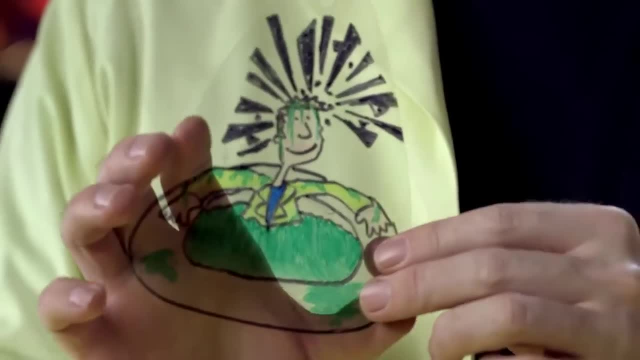 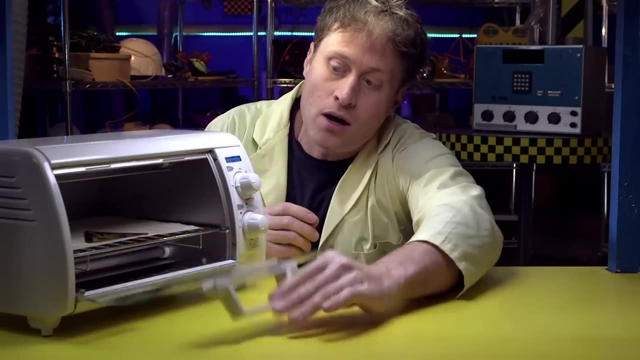 I've got a chemical symbol, an atom, and this is me in some slime. Then get an adult to help you put it in the oven, or Toaster oven. At 350 degrees It only takes a few seconds for the plastic to shrink to one third its size. The reason why this happens is when plastic is manufactured it's heated and stretched out and then cooled and it sort of freezes in that stretched out shape And when you reheat it it shrinks back. It goes back down to the unstretched shape. 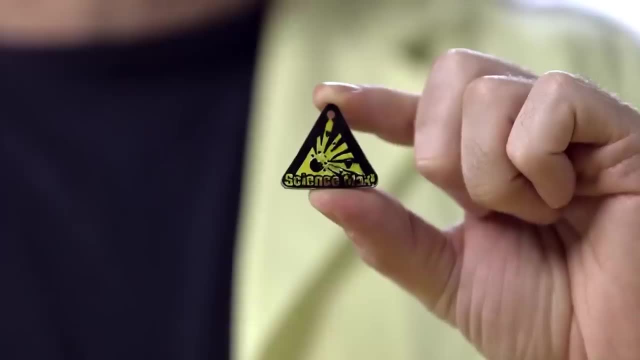 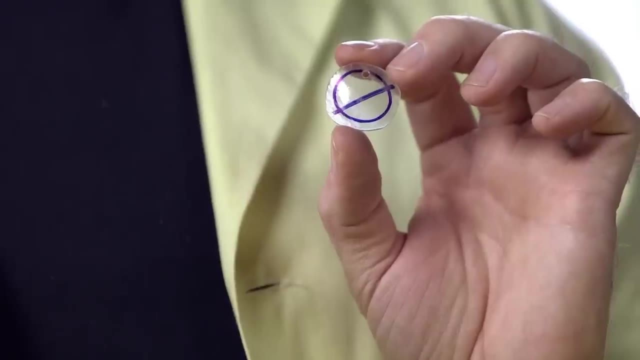 Get your adult to take it out and wait for it to cool and you'll have yourself some small plastic designs you can use for key chains, bracelets, name tags, bookmarks, whatever you want, All using the power of polymers. Awesome, I'm going to make all of those. 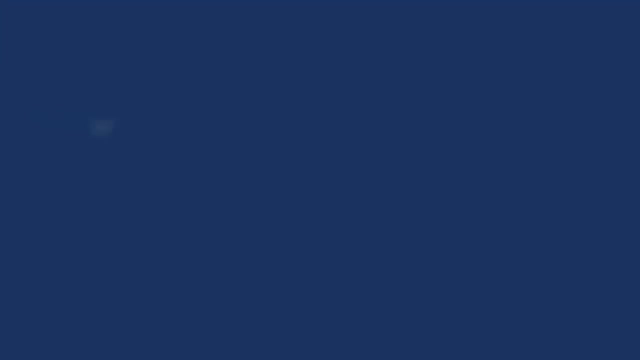 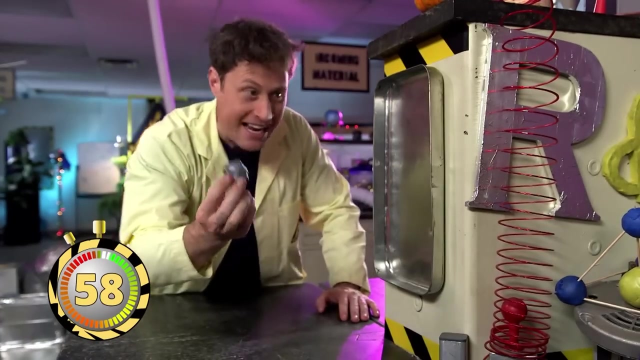 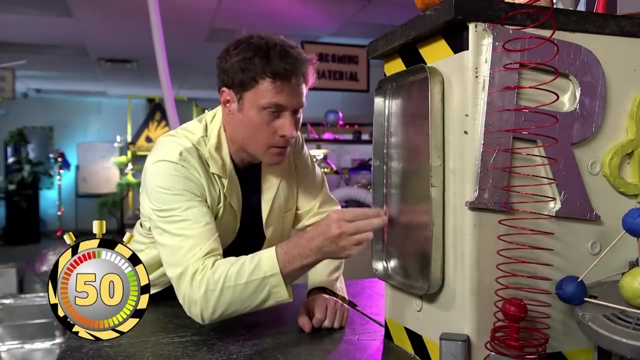 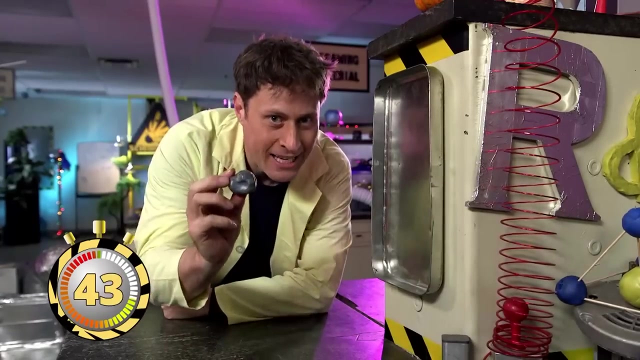 What was that again? Key chain ornament magnet um Magnetic Putty in 60 Seconds. This is Magnetic Putty. Take it. This is Magnetic Putty Ten. take. This is Magnetic Putty Twenty-six. This is Magnetic Putty. 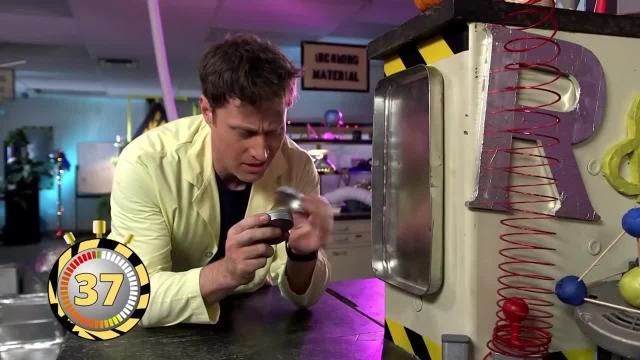 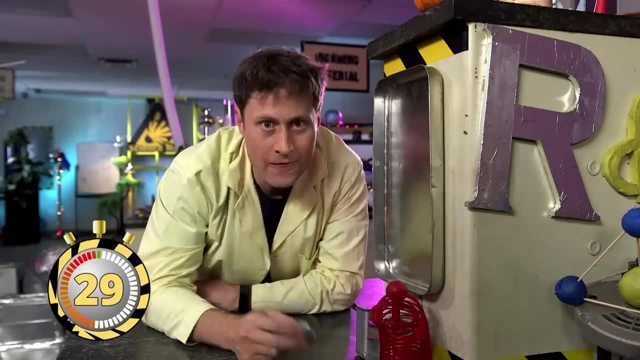 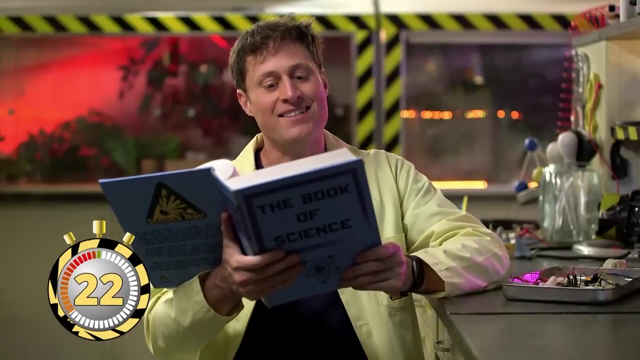 2,635.. This is Man. this is Magnetic Putty. I can't count this high. This is Magnetic Putty. Ha, Magnetic. Oh, it's not a magnet, It's attracted to magnets. Oh, that makes more sense. 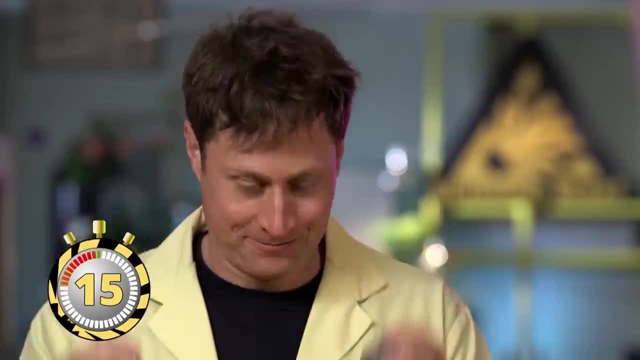 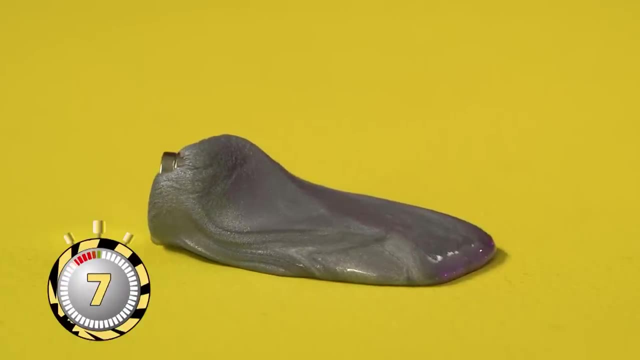 This is Magnetic Putty and this is a magnet. The putty is made of polymers, which means it can flow over itself. It also has lots of iron filings in it, which is why it's attracted to magnets. This is what happens over several minutes. 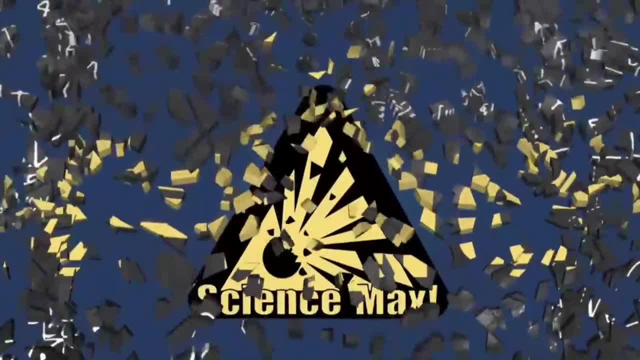 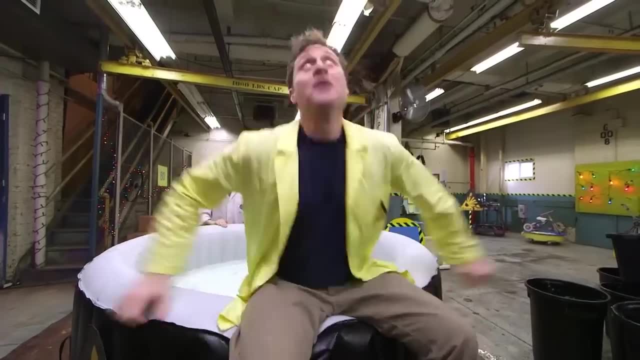 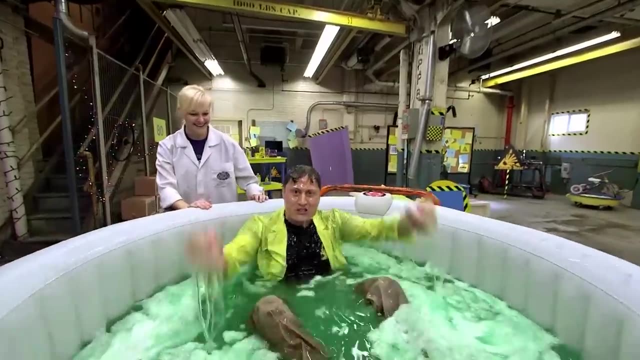 And there you go, Magnetic Putty. Okay, so where were we? Oh yeah, Three, two, one Yeah. And remember, don't try this at home. Ah, Ah, Slime. Sarah and I enjoyed our maxed-out tub of slime. 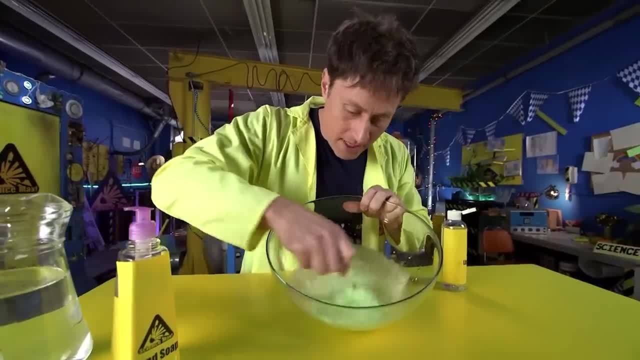 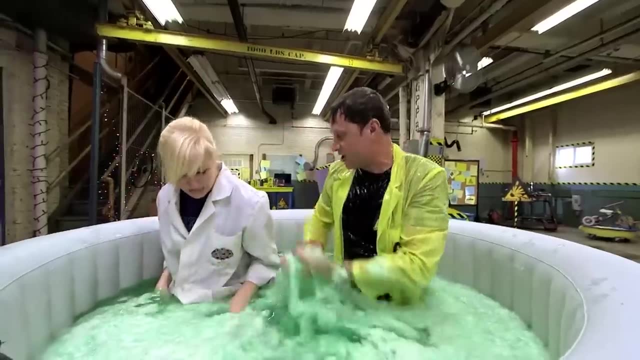 So let's recap. Slime is made of polymers. Polymers come in a lot of different forms. It's all about long chains of molecules, And none are more fun to swim in than slime. Do I have slime here? Ooh Yeah, definitely. 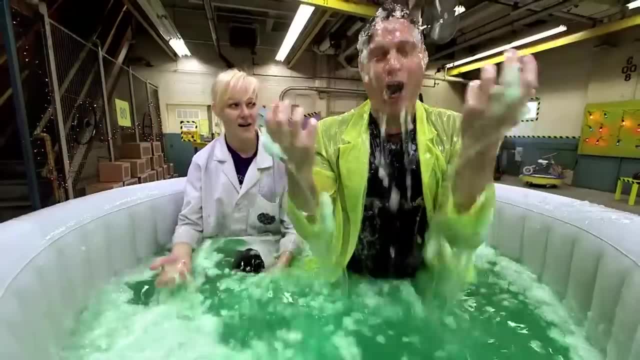 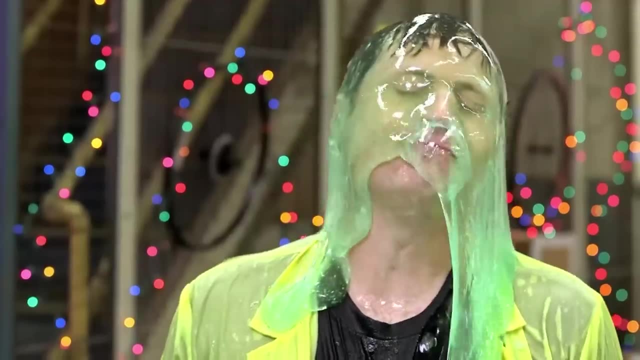 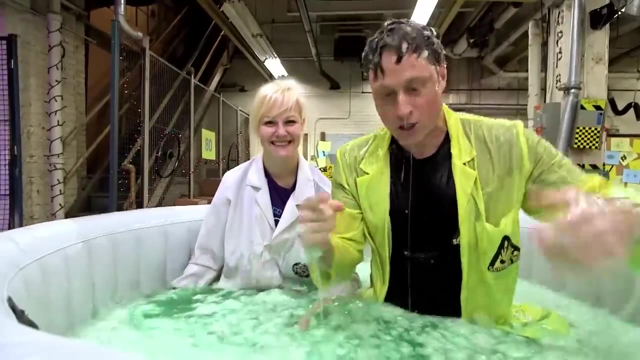 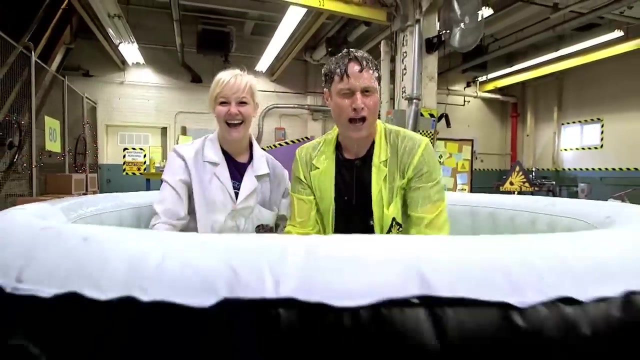 Slime here, Slime. Well, there you go. Science makes experiments at large. Polymers Slime, Yeah, High-fives Yeah, Slimey, high-five, Slimey, high-five Slime. Greetings: science maximites. 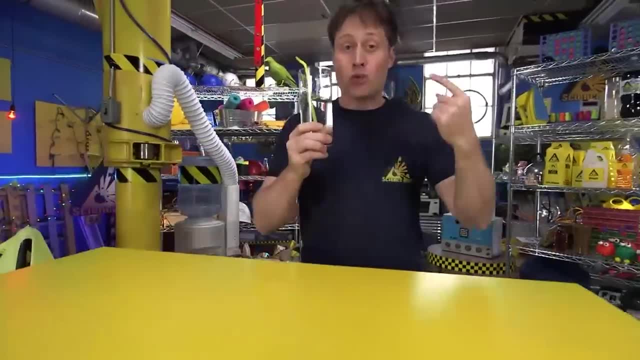 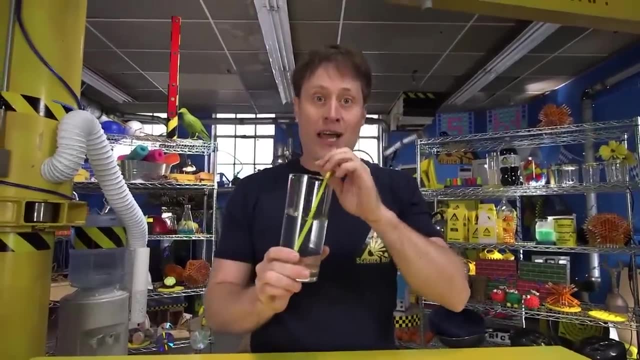 Today we're using fizzy drinks in our experiments, And a fizzy drink is just water with bubbles of carbon dioxide gas dissolved in it. So I thought, since we exhale carbon dioxide, I could make a fizzy drink by just blowing bubbles in this water. 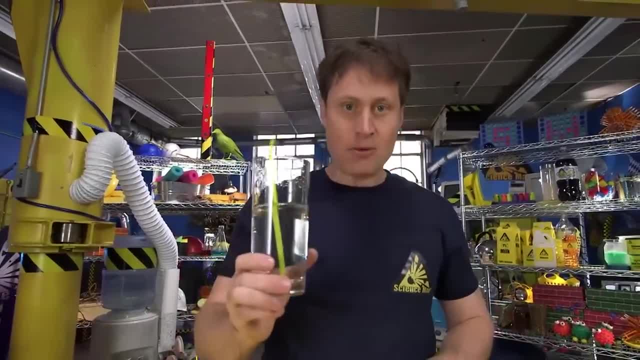 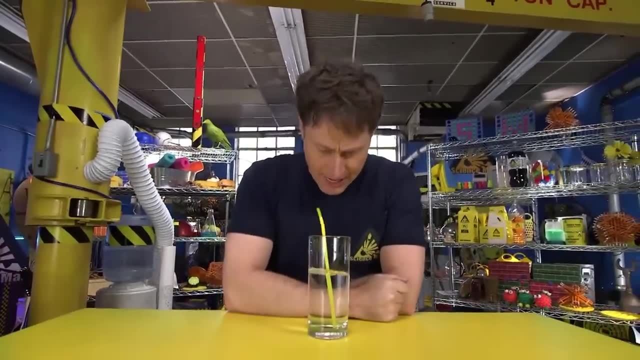 Doesn't seem to be working, though, does it? I don't see any bubbles, Do you No? Hmm, Water does absorb carbon dioxide gas, but I don't have a fizzy drink. don't have a fizzy drink. weird time to check the book of science. oh, in order to. 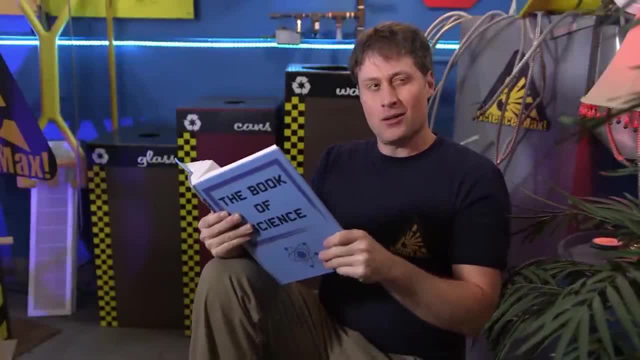 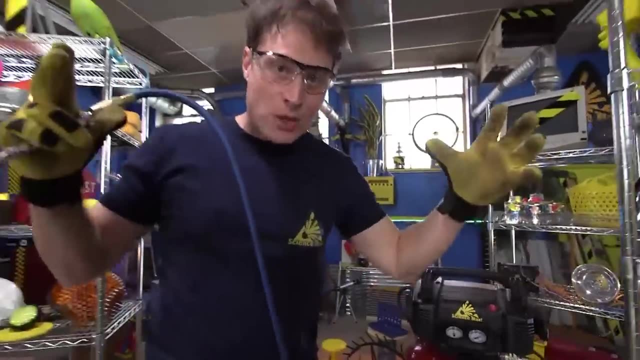 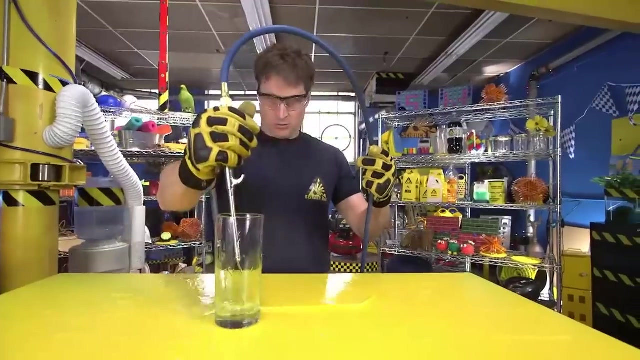 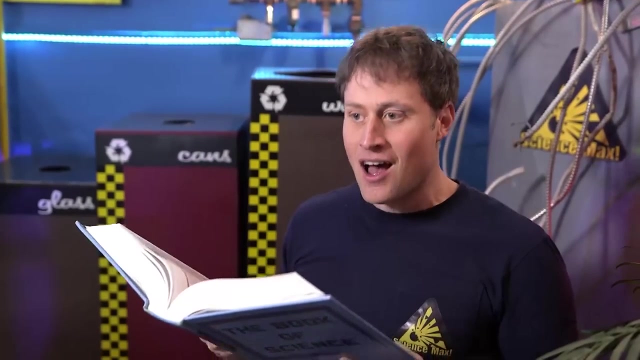 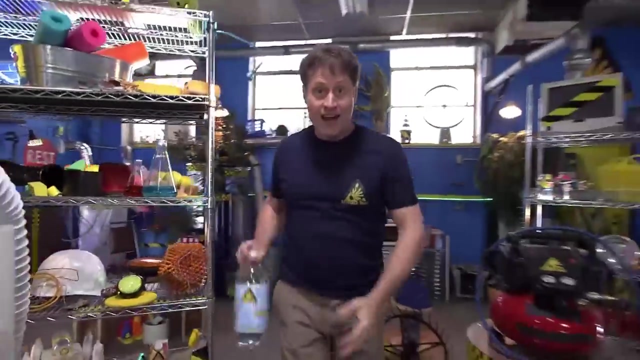 make bubbles, you have to have pressure. so this is an air compressor. it takes air and compresses. it puts it under pressure. so, hmm, the container needs to be pressurized. okay, when you get a container of a fizzy drink, the carbon dioxide gas is put in there under pressure and it stays in there under. 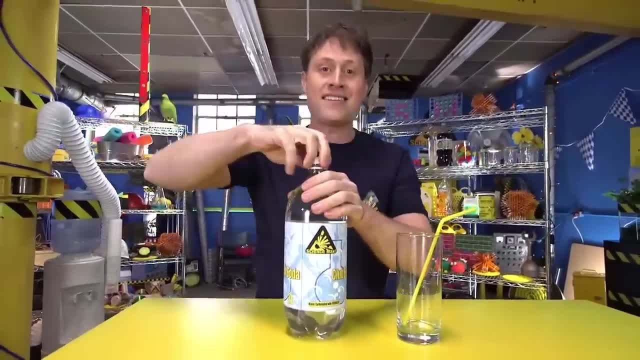 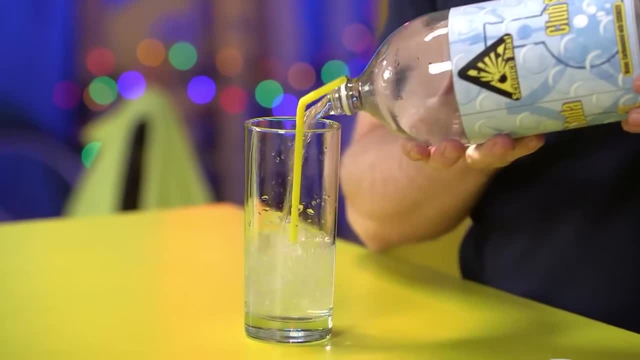 pressure until you release it. that's the sound of the pressure being released. and when it is released, the carbon dioxide gas starts to expand, and when it expands, it creates bubbles, and that's what makes your fizzy drink. this process takes a while to run out, but eventually it's a fail. 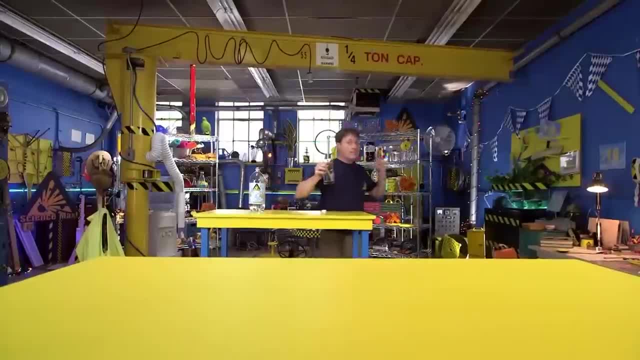 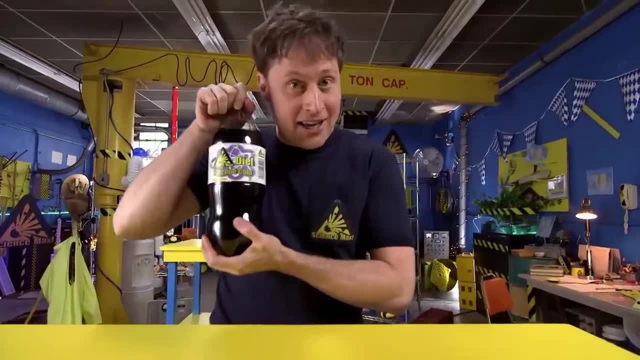 it will become flat, no more bubbles. But what if there was a way to release all of that carbonation all in one go? Well, there is, and for this experiment, all you need is your favorite brand of fizzy drink: Science Max brand, Diet, Science Cola. 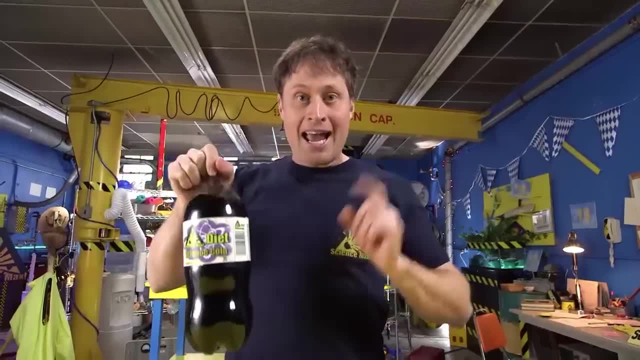 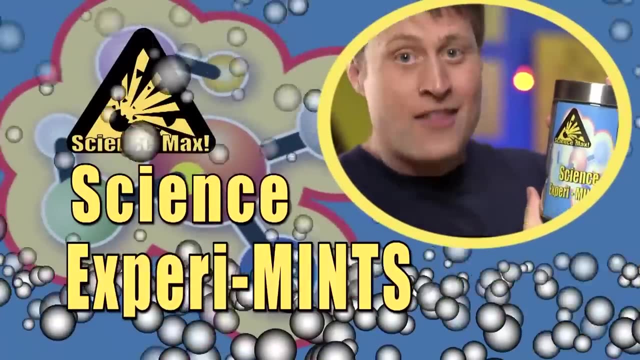 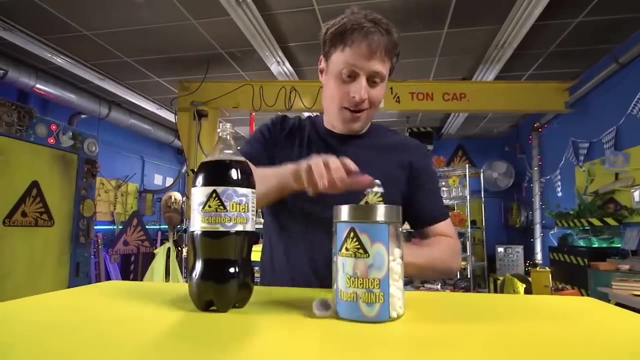 100% science, zero calories. And your favorite candy, like these science experiment mints- All the minty flavor that comes from pure science. So all you need to do is open this up. open this up, take one of these. 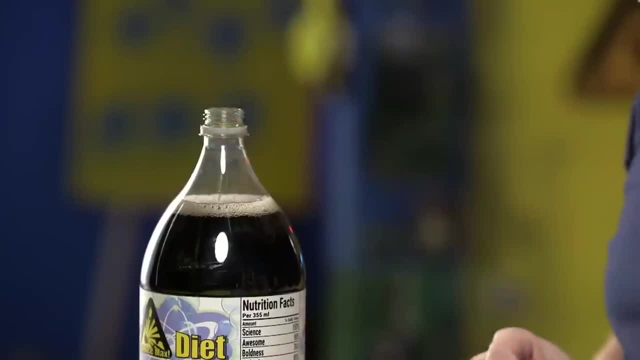 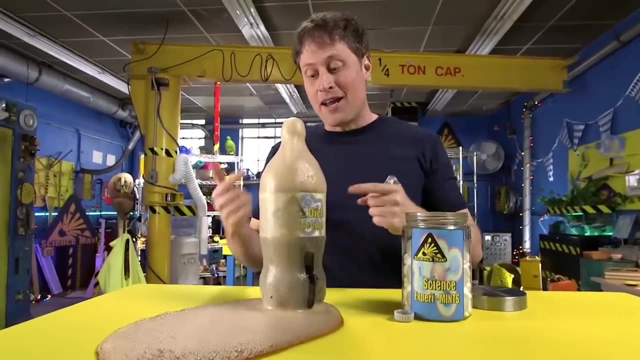 and put it in here with an adult's permission, because it can get kind of messy. Whoa. What's going on here is all of the carbonation that was in the bottle is now being released much more rapidly than it would have been before. 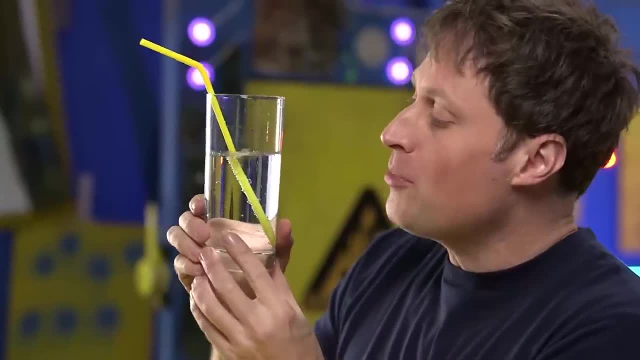 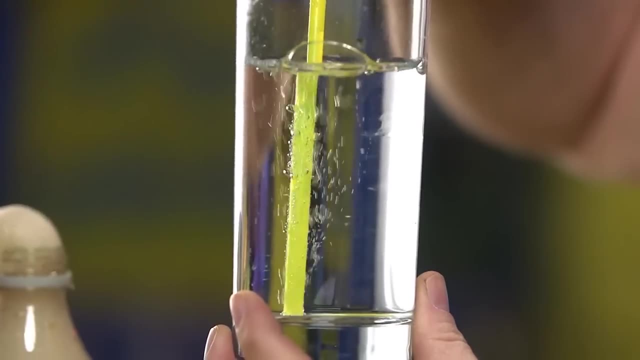 Now, why does this happen? Well, if you look at a carbonated beverage, you'll see that the bottle bubbles don't come from everywhere. They come from the inside of the glass or, in this case, a lot are coming from the straw. 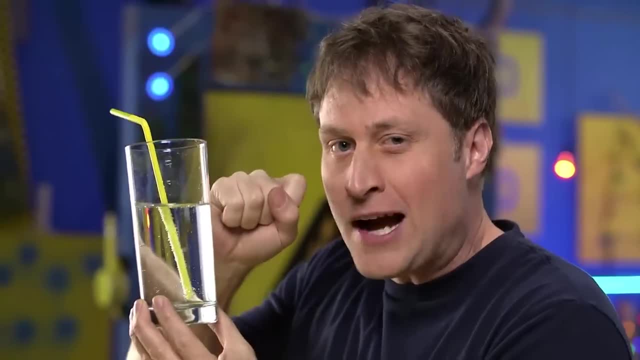 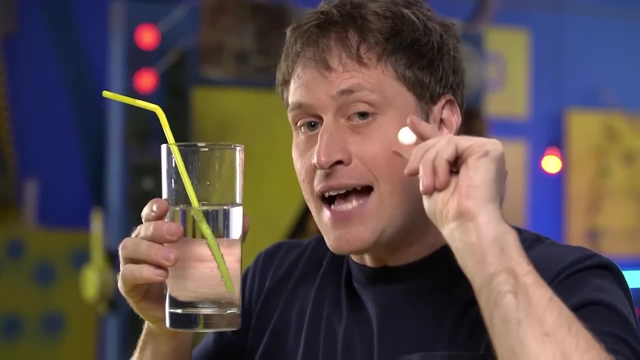 And that's because the carbon dioxide bubbles like to find a little imperfection, something to hold onto in order to expand and bubble out, And a candy such as this has a ton of little, tiny, microscopic imperfections, So when you drop it in, 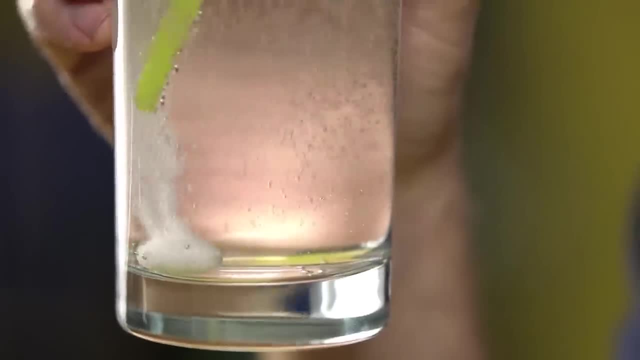 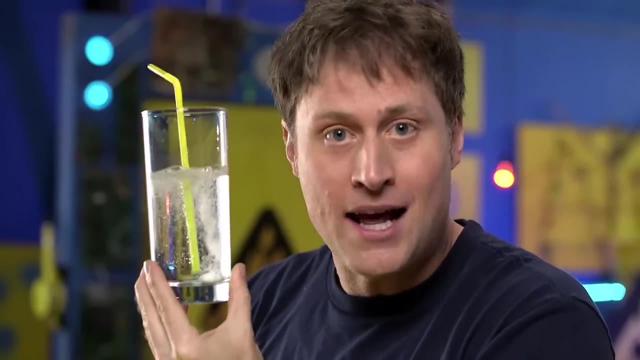 there's a lot more places for the bubbles to attach, and that makes the carbonation happen a lot quicker. But remember: this is not a chemical reaction. It all has to do with carbonation. So that's what we're going to be looking at today. 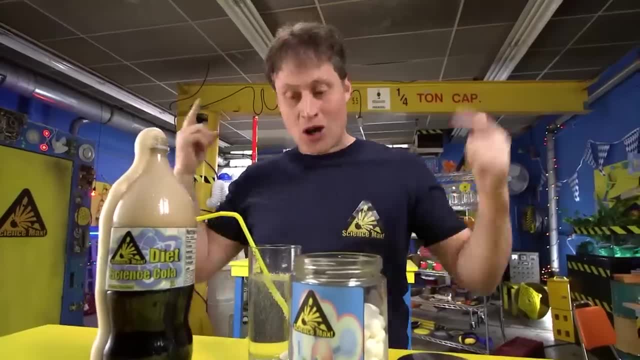 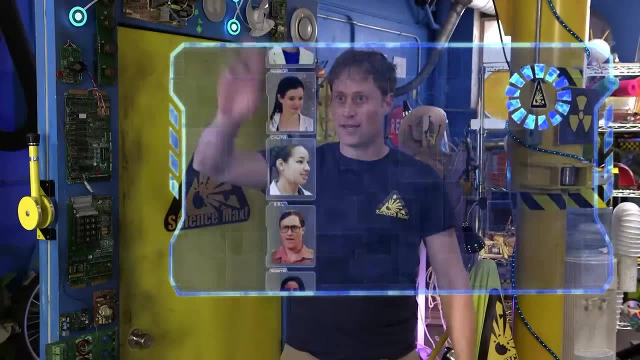 Air pressure, more pressure, less pressure, and, of course, we're going to be maxing out this experiment. All right, I just need an expert to help me max this out. Let's see, Oh, Cynthia from the Ontario Science Centre. 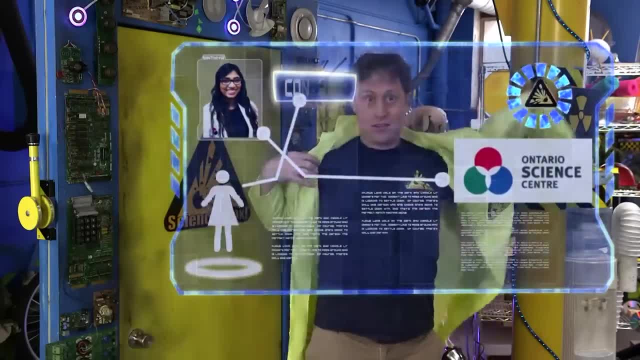 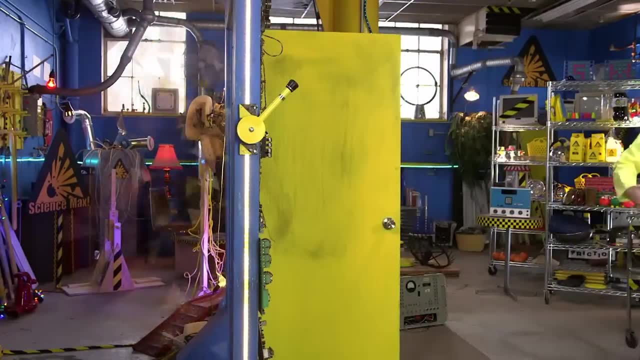 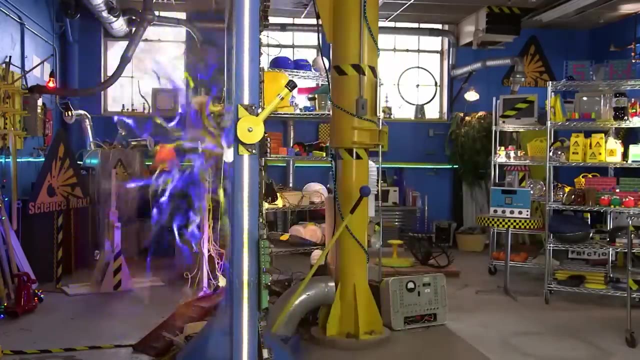 She'd be perfect for this. All right, Good, Okay, come on, let's go. And yup, that's good. All right, Let's go. Oh, hey, Cynthia, Hey Phil, How's it going? 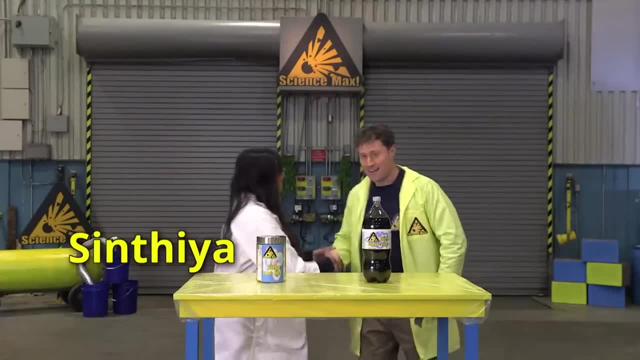 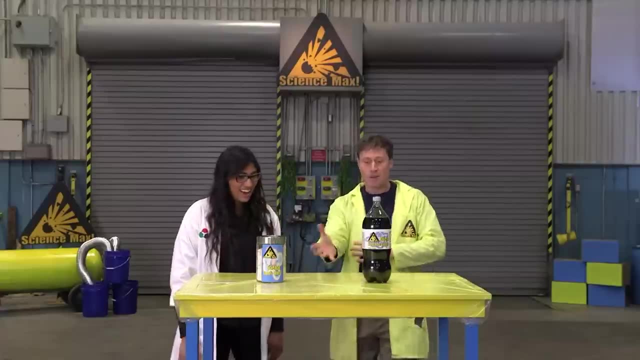 Cynthia from the Ontario Science Centre, you're going to help me max out the science experiments and diet science cola experiment- I think we need a better name for this, Okay, Well, we have the mints that have tiny little pores, called nucleation sites, on them. 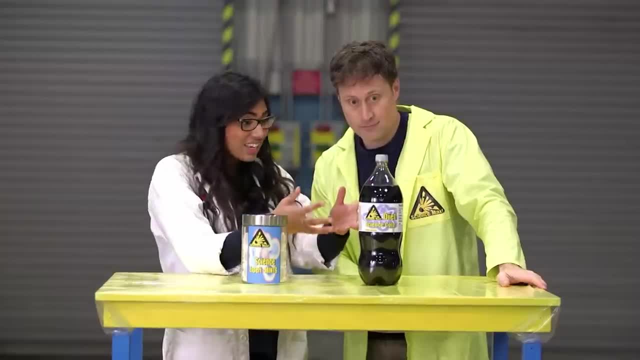 The gas inside the cola is going to go through these nucleation sites, create a giant fountain- Uh-huh, So we're going to need a little bit of a mix. Uh-huh, So why don't we call it a nucleation fountain? 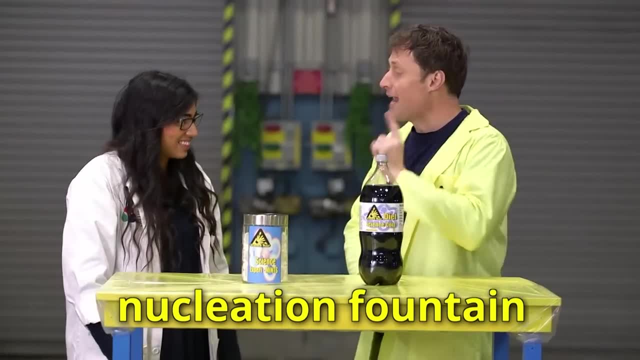 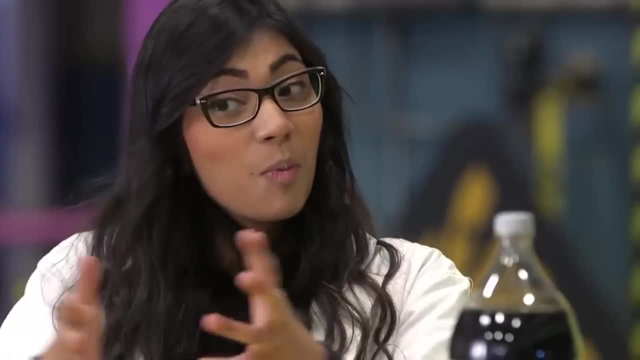 Ooh, nucleation fountain. I like that. It's accurate and it sounds awesome. There we go. Okay, so we want to max it out. So how many should we put in? Let's say, five more nucleation sites, More reaction. 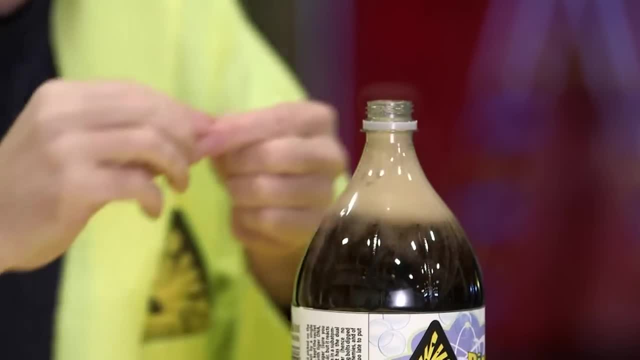 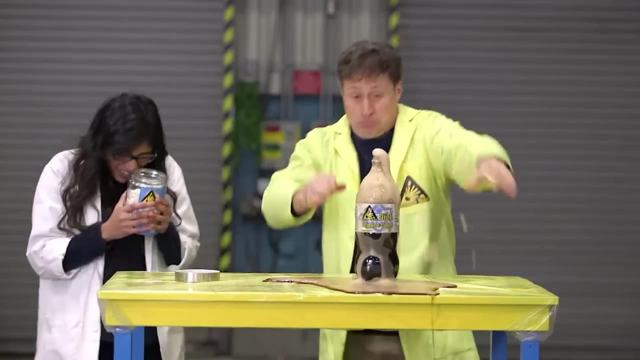 Ah, I tried adding more mints, but one at a time didn't work. It doesn't. No, It's not. The bubbles are pushing it back out again. There we go, There we go, And then, Yeah, I think, if we put them all in at the same time. 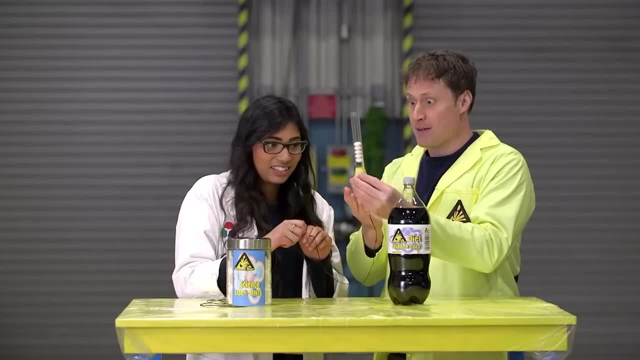 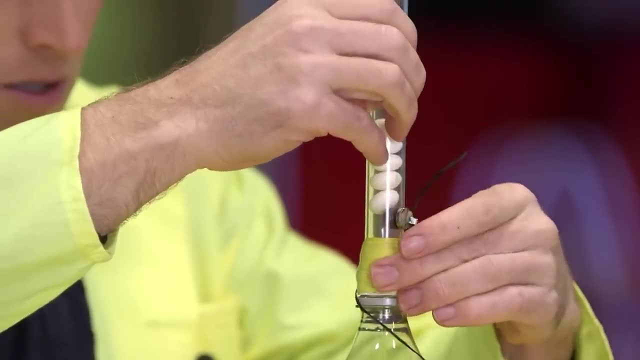 it would work better. So we came up with a delivery mechanism to get all the mints in at the same time: A tube with a magnet holding the mints up which we screw onto the top of the bottle, pull the outside magnet to release and 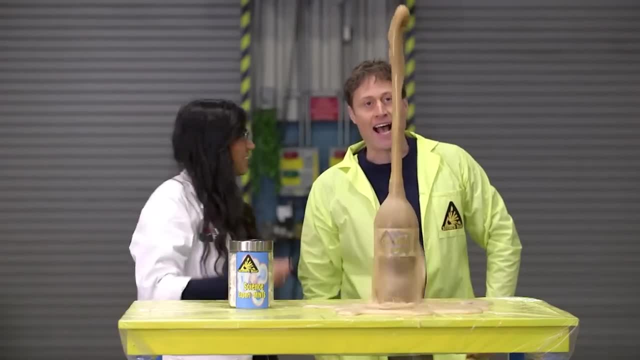 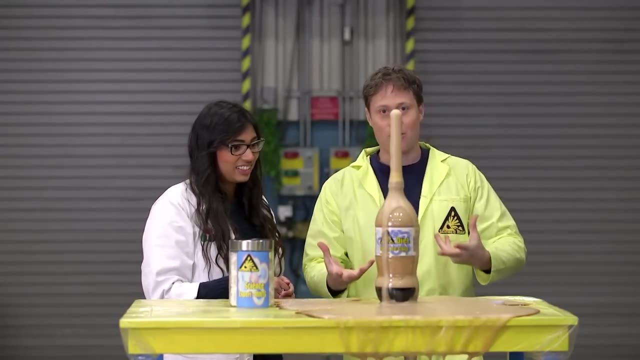 Ooh Nice. Yes, Oh yeah, That's a good fountain. That is a good, A good nucleation fountain. A nucleation fountain worked very well. There we go, Cynthia and I decided to try some other ideas to max it out even more. 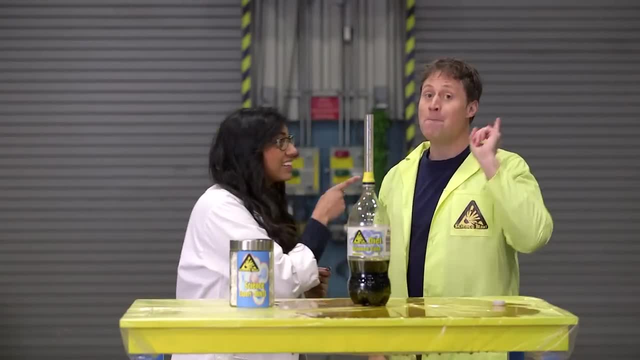 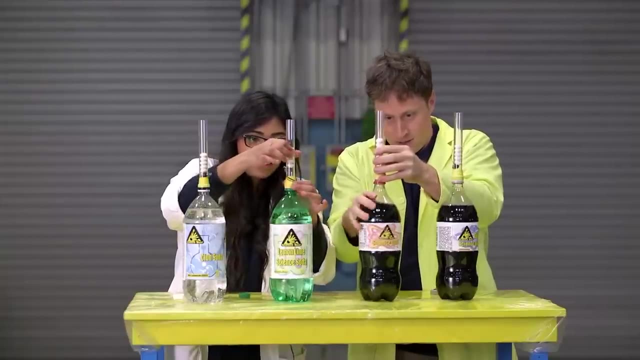 We decided to do some Experimentation- Experimentation- Oh, that's a good one, Yeah- And see if diet cola was the best carbonated drink to use. We tried four different kinds: Diet cola, regular cola, lemon-lime soda and club soda. 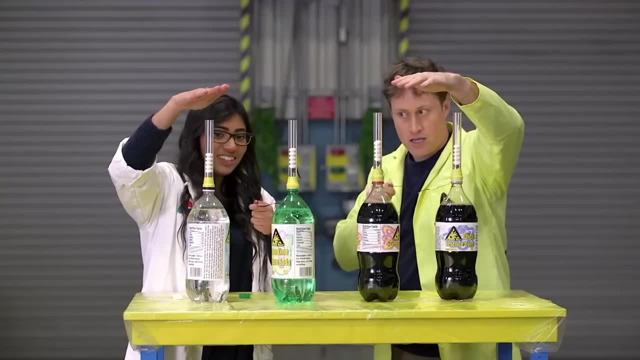 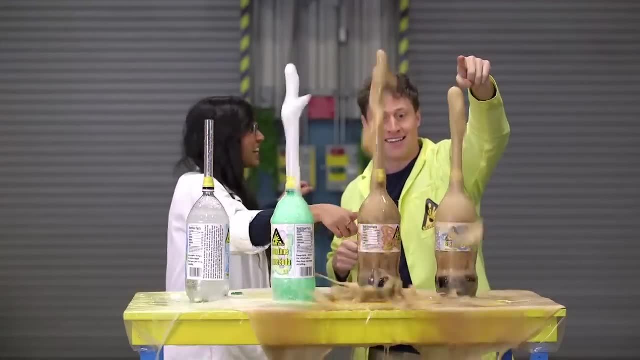 Really just, It's just carbonated water. Carbonated water, Three, two, one go. Ooh, Oh, Oh Ooh, Science cola, Science cola. But I think the It was close. I think it was the release. 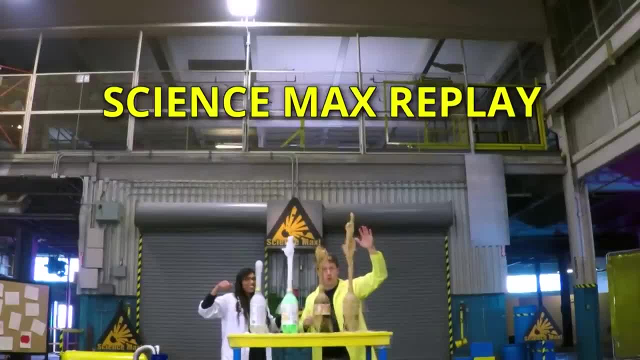 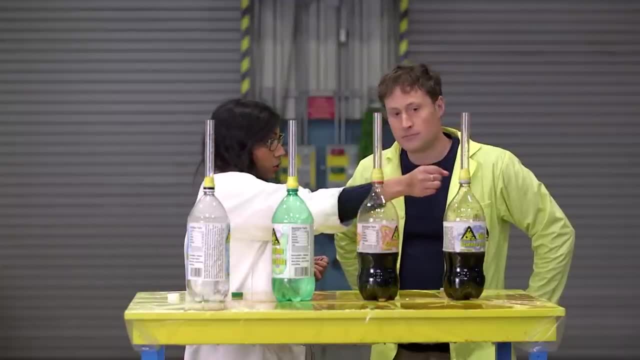 Let's watch the replay. Okay, Yep, Diet science cola went the highest. So the next step is: Maybe, if we want to max the size of the fountain, we have to make a narrower stream. Ooh, So a smaller aperture opening will be higher pressure. 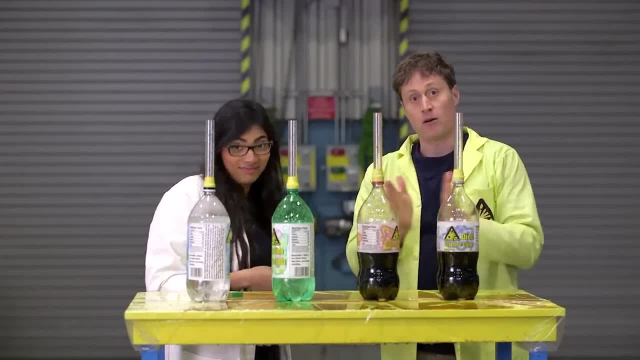 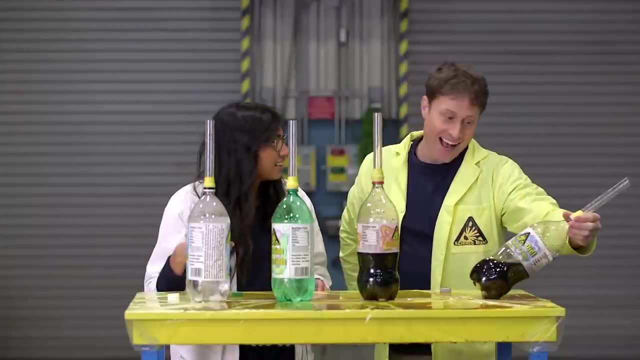 That's what I'm thinking, Because it'll be forced at a smaller opening. What else can we do? We can launch it. We can launch Well, you mean like sideways. Yeah, Yeah, I love that idea. So we'll put it on wheels. 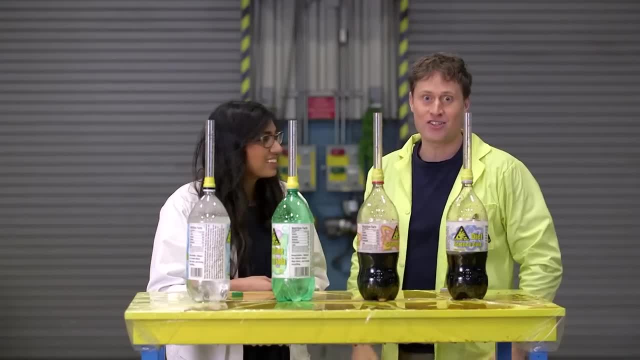 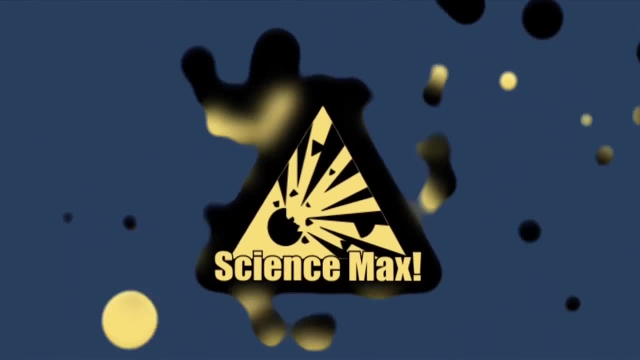 We'll put it on wheels, Okay, And then we'll launch it sideways. Okay, We have a lot of things to do. Okay, Let's get. We need time. Let's do it. Get to it. Okay, We'll go to the lab. 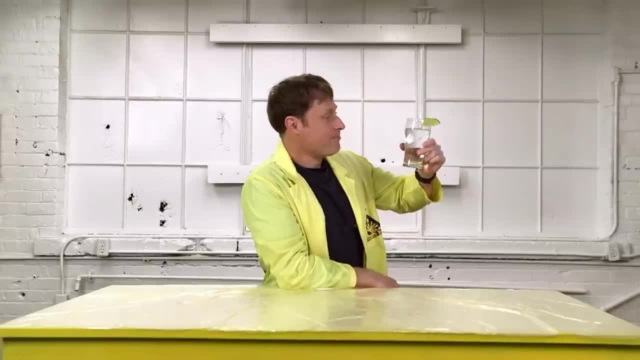 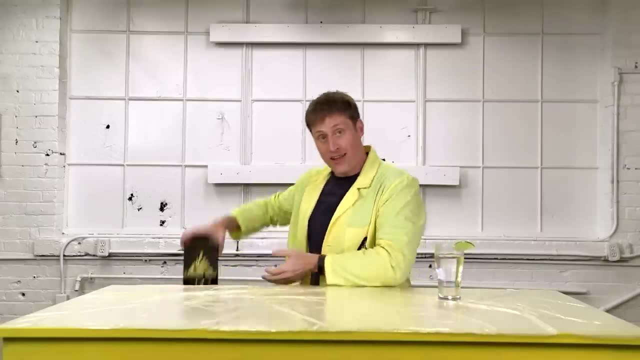 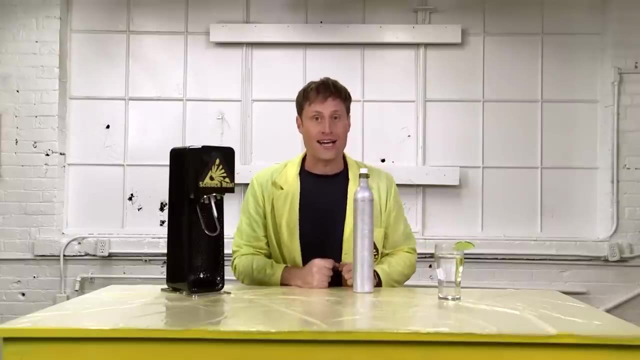 I'll get a mop, Nothing like a fizzy glass of water. And now there are ways for you to carbonate water at home with something like this, This Science Max carbonation station. You have a bottle of compressed carbon dioxide gas that's hooked up. 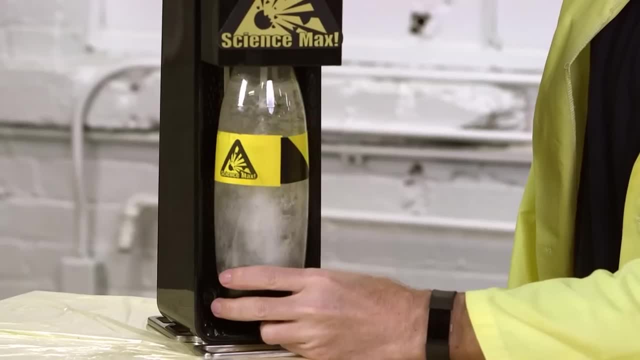 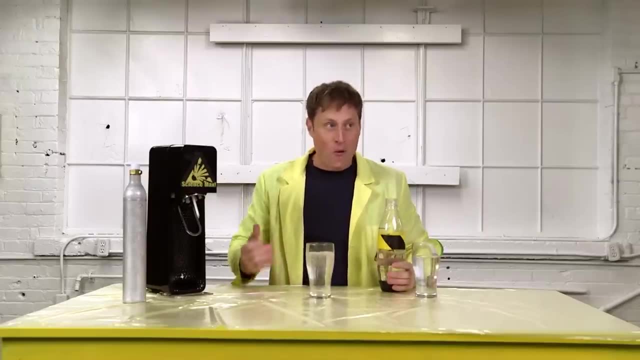 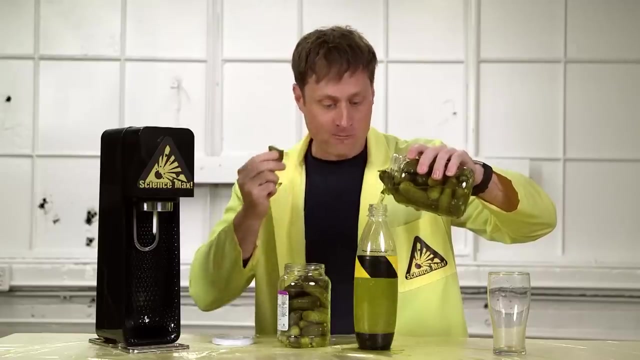 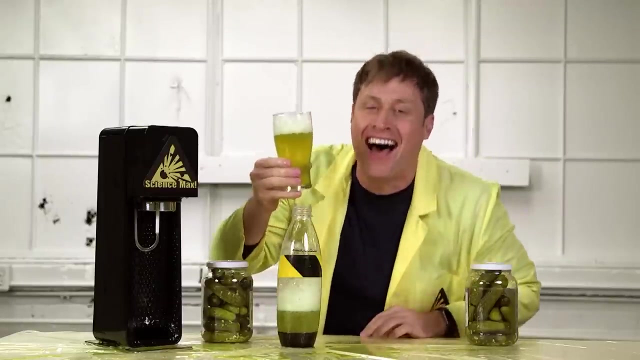 You take a bottle of tap water, attach it and carbonate it. Voila, Carbonated water. But this is Science, Max. Why just carbonate water? Let's carbonate everything. Let's carbonate pickle juice. It's actually amazing Milk. 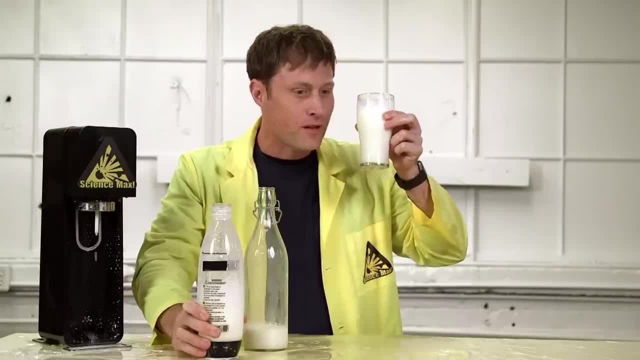 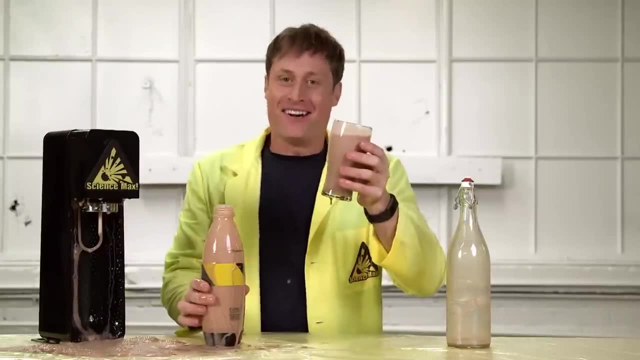 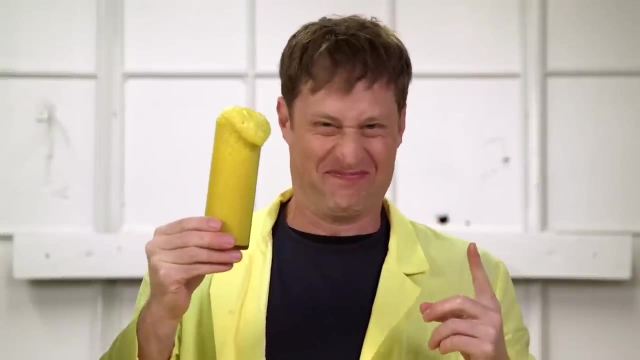 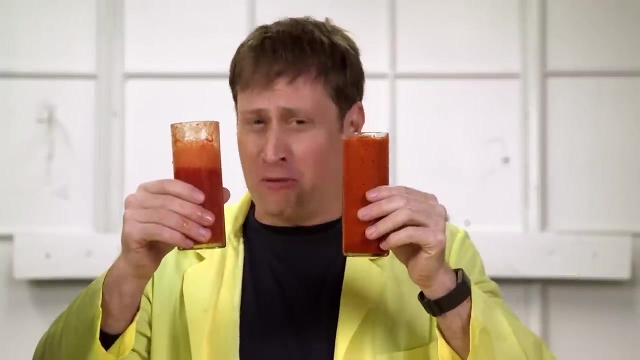 It's like milk meets water, Kind of very odd Chocolate milk. Oh no, that's way better. Carbonated mustard, Carbonated tomato juice, Carbonated hot sauce- No wait, carbonated, that was the hot sauce. 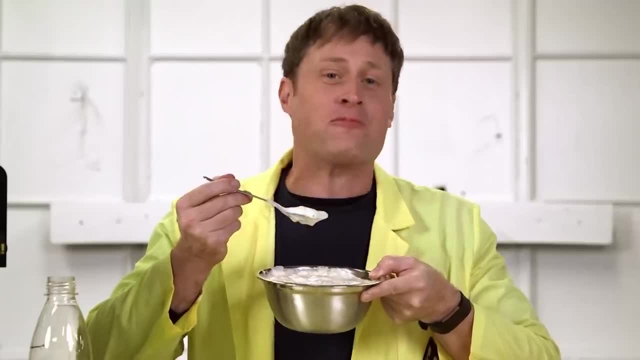 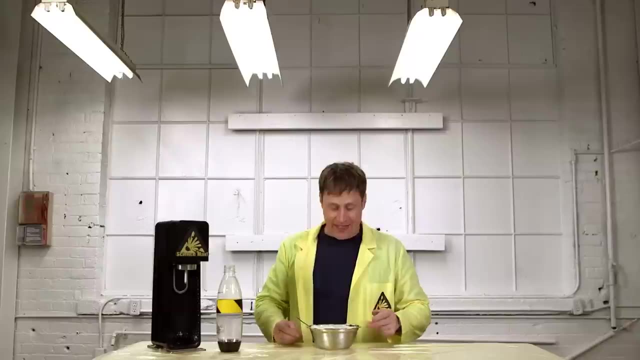 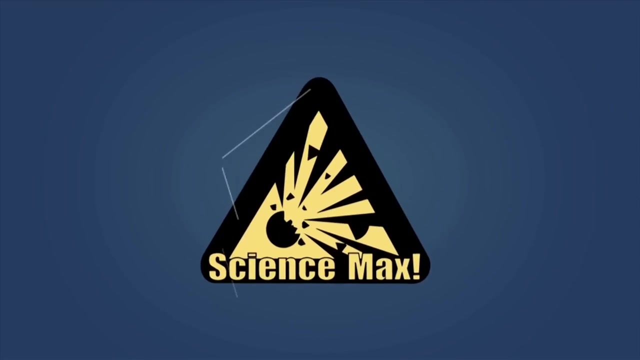 Carbonated clam chowder. Oh, there you go. carbonation, not just for water anymore, And it's definitely not for clam chowder. No, that's just a big bowl of no. never again. CYNTHIA AND I ARE MAXING OUT A NUCLEATION FOUNTAIN. 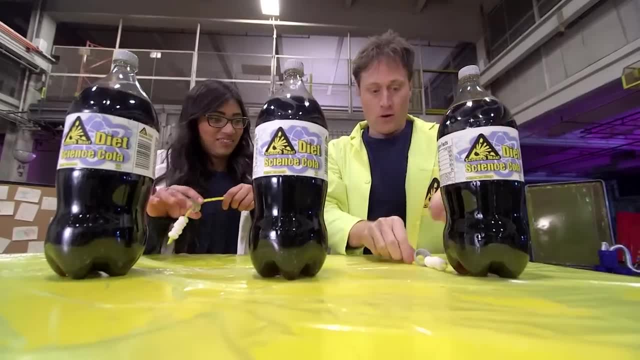 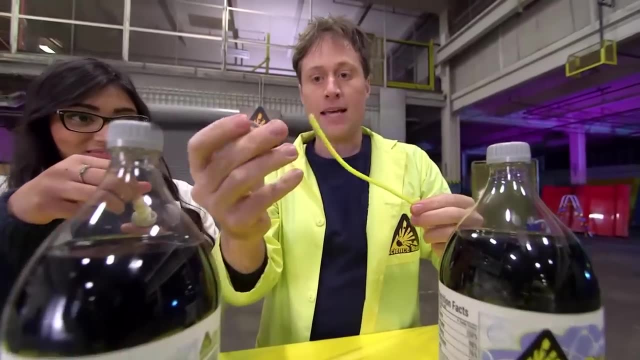 YES, OH YEAH, THAT'S A GOOD FOUNTAIN. WE'RE CHANGING OUR DESIGN A BIT TO SEE IF A SMALLER HOLE IN THE BOTTLE CAP WILL MAKE FOR A HIGHER PRESSURE FOUNTAIN, WHICH WILL MAKE IT MORE MAXED OUT. 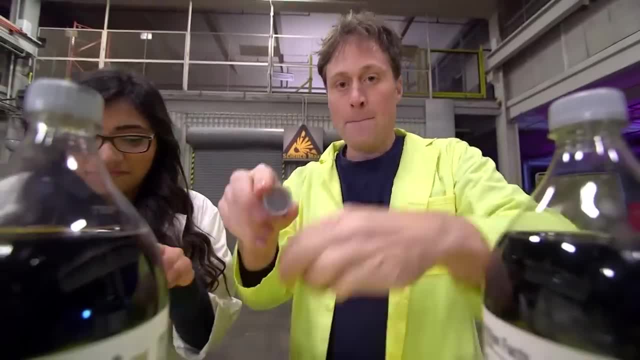 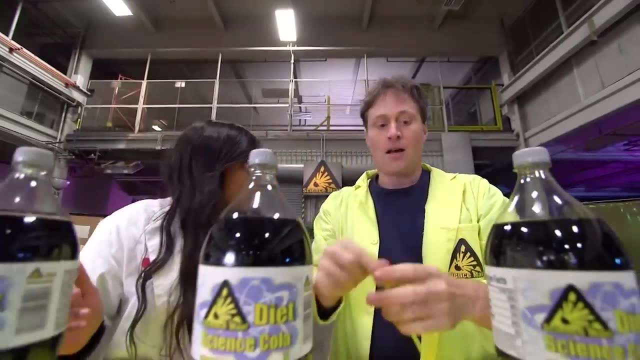 WE HAVE THIS LARGE HOLE. WE'VE GOT A MEDIUM-SIZED HOLE. WE HAVE A VERY SMALL HOLE, SO WE'RE GOING TO SEE LARGE, MEDIUM OR SMALL. WHICH ONE IS THE BEST TO MAX OUT OUR FOUNTAIN? 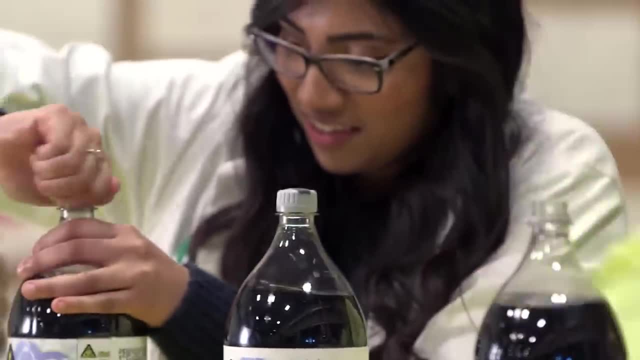 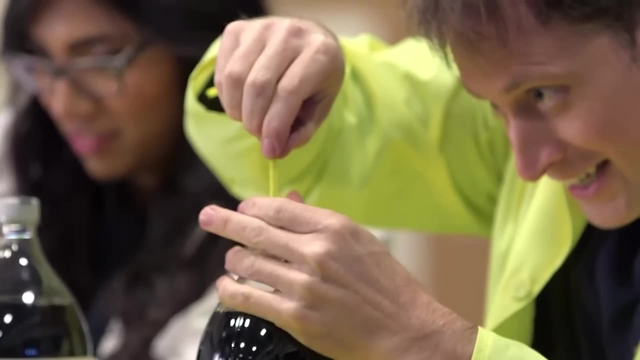 EXACTLY BUT THE PROBLEM IS THAT OUR OLD DELIVERY MECHANISM WON'T WORK IF WE KEEP THE CAP ON, SO WE NEEDED TO COME UP WITH A NEW DELIVERY SYSTEM, SO WE DRILLED HOLES IN THE MINTS AND PUT THEM UNDERNEATH. 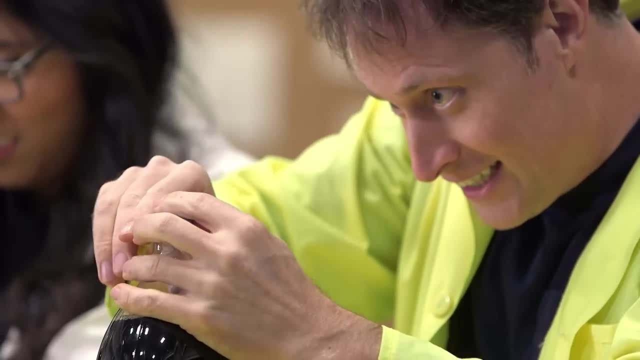 THE CAP ON A PIPE CLEANER. THEY HANG AT THE TOP OF THE BOTTLE UNTIL WE PULL THE PIPE CLEANER AND THEN THEY FALL IN ALL RIGHT. ARE YOU READY? OH, I'M SO EXCITED. 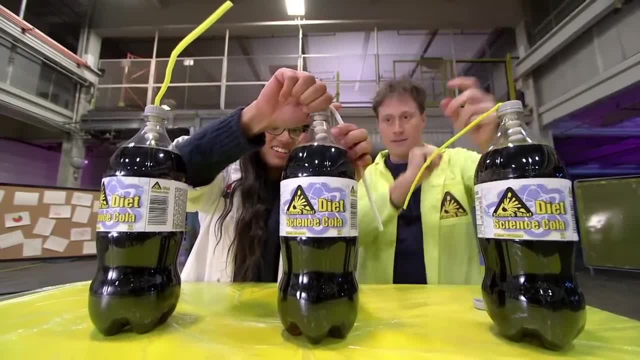 WHICH ONE DO YOU PREDICT WILL BE THE BEST? THIS WILL HAVE A LARGER GEISER. I THINK THIS WILL LOOK COOLER BECAUSE IT'LL BE BIG. BUT THIS ONE- THE SMALLEST HOLE, I THINK WILL GO THE HIGHEST. 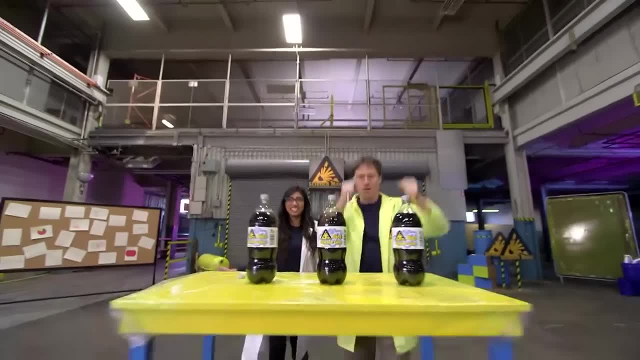 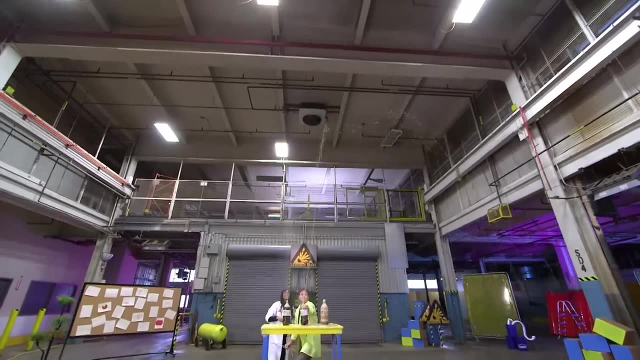 YEAH, READY, THREE, TWO ONE, WHOA, DEFINITELY THE BIGGEST. WHOA, WHOA, THERE, WHOA, CAREFUL, CAREFUL, CAREFUL, WHOA. THIS, ONE IS ALMOST LIKE A SPRAY. 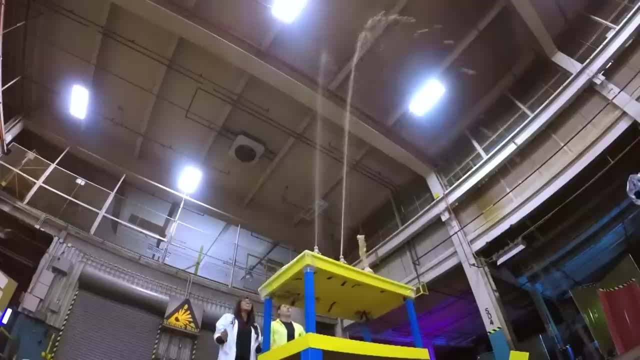 IT'S NOT LIKE A MIST, YEAH A MIST. IT'S A MIST OF COLA. THEY ALL KIND OF WORK A LITTLE DIFFERENTLY. THE INTERESTING THING IS THIS ONE. THIS ONE LASTS THE LONGEST. 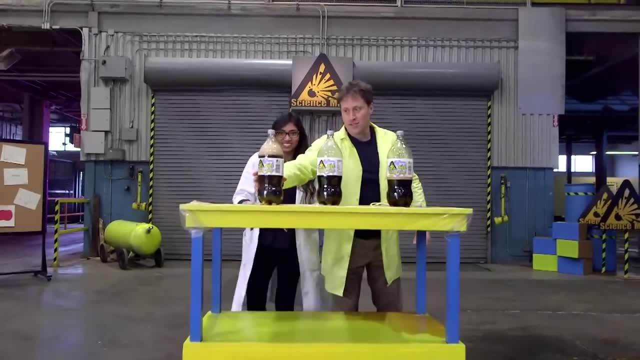 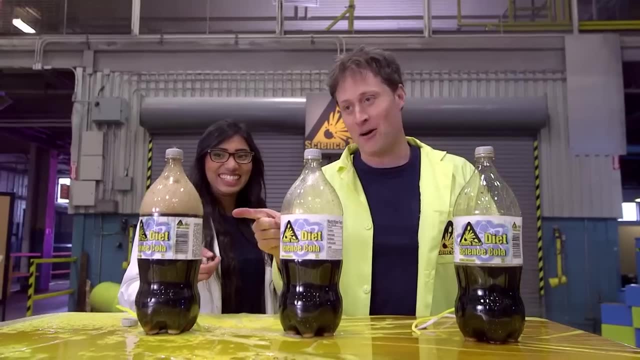 OH, OH, OH, OH, OH, THERE WE GO. SO THIS WAS COOL, BUT NOT THE BEST. THIS ONE'S STILL GOING, IT'S STILL GOING, IT'S NOT OVER. YET, YOU GOT TO GIVE IT POINTS FOR STILL GOING. 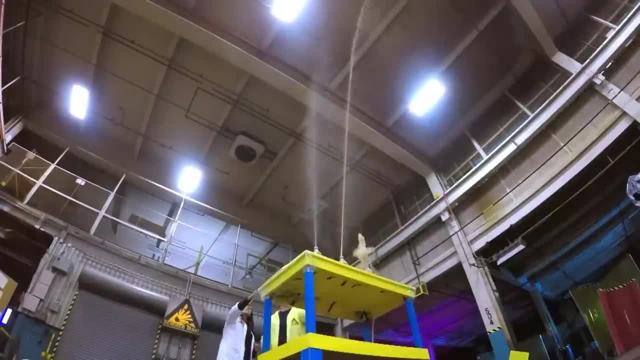 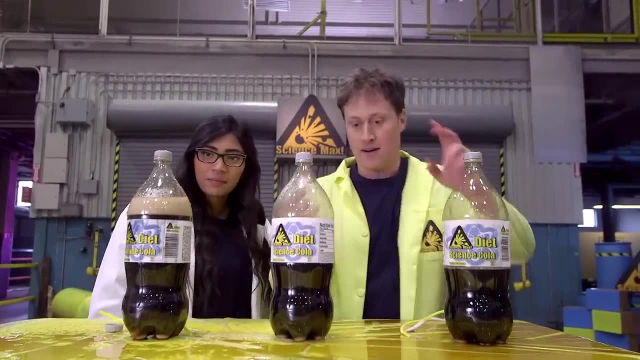 I THINK THIS FOUNTAIN LOOKED THE BEST THOUGH. THIS ONE WAS PRETTY GOOD. SO A SMALL APERTURE- BUT MAYBE NOT THE SMALLEST APERTURE- WOULD BE THE BEST. SO, BECAUSE OF THE FORCE COMING OUT OF HERE, I THINK THAT WE COULD PROBABLY DO SOMETHING LIKE PUTTING IT ON WHEELS. 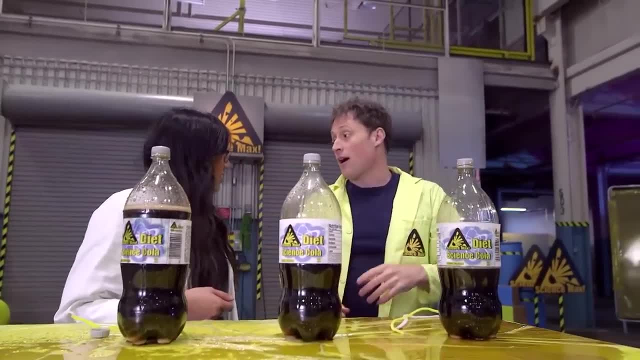 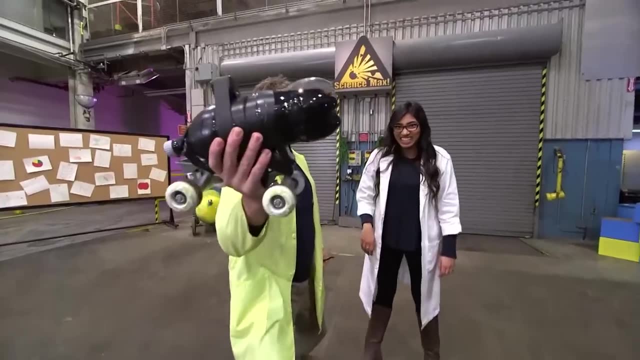 AND SHOOTING IT. LIKE A ROCKET- YEAH, LET'S SEE ON WHEELS. OR LIKE A CAR, OH, YEAH. OR LIKE A NUCLEATION FOUNTAIN CAR: THE NUCLEATION ONE BOOM. 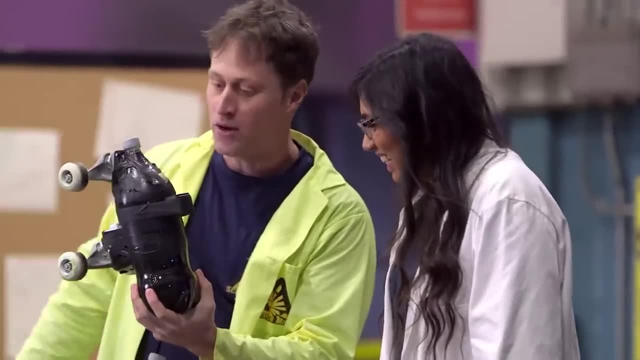 IT'S OUR RACE CAR. IT'S OUR RACE CAR. IT'S GOT FANCY WHEELS. THAT SPIN REALLY WELL, AND WE DECIDED TO GO WITH THE MEDIUM APERTURE, SO IT'S FAIRLY BIG, BUT NOT TOO SMALL. 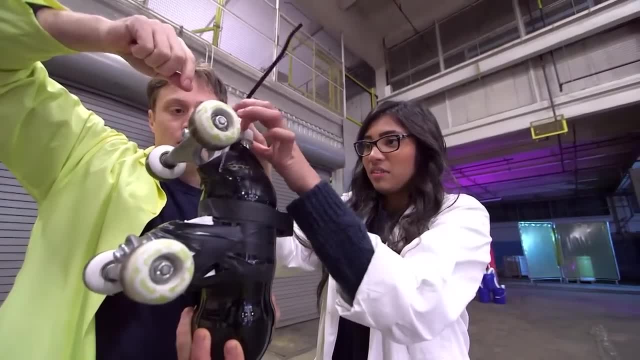 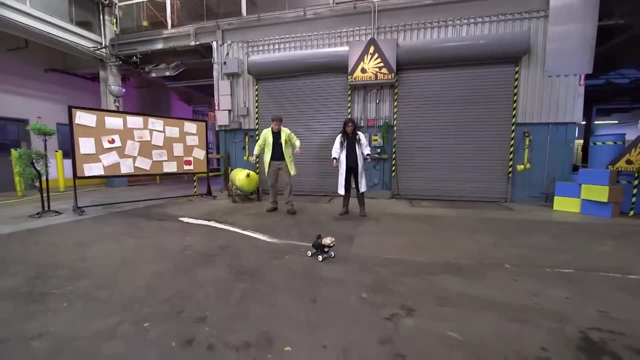 YEAH, ALL WE NEED TO DO IS UNSCREW THAT, PUT THAT IN THERE AND THEN PULL IT OUT. THREE, TWO, ONE. OH, GOOD, GOOD, GOOD, LET IT GO. OH, THAT'S NOT SO BAD. 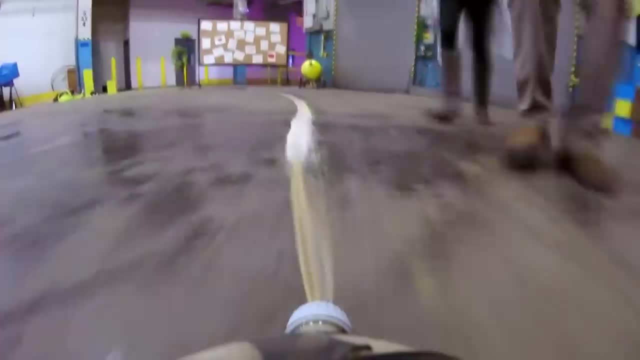 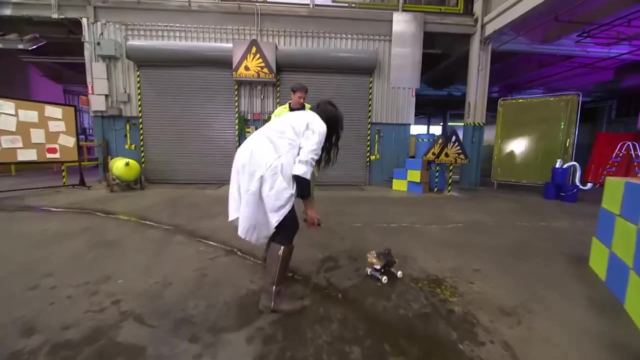 OH, YEAH, OH, YOU MISSED THE FINISH LINE. PASS THE THING, TURN IT AROUND, TURN IT AROUND. DO YOU THINK WE CAN MAKE IT? GET TO THE FINISH LINE? IT'S FINISHED, NO. 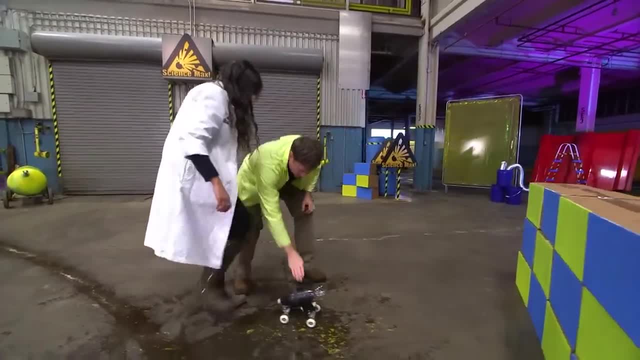 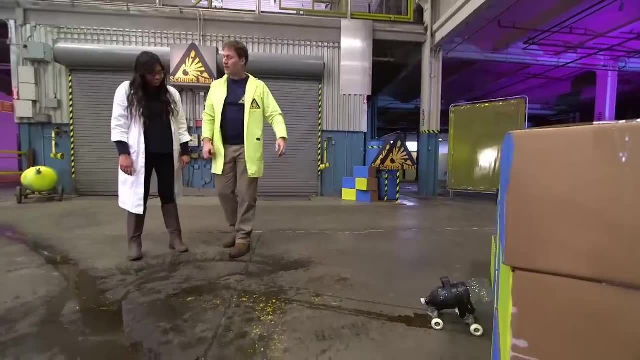 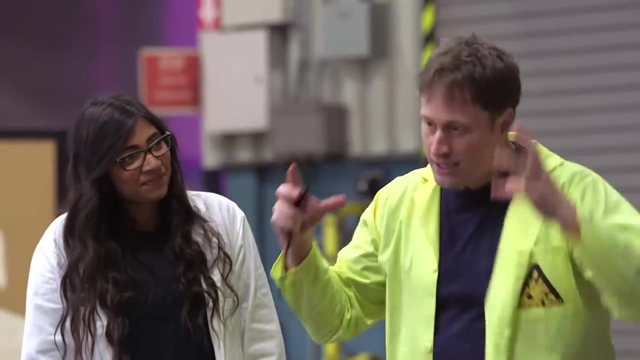 IT'S SPINNING OUT. OH WOW, GO, GO, YAY. IT WORKED PRETTY WELL BUT THERE'S ALWAYS MORE WAYS TO MAX IT OUT. WHAT IF WE JUST GOT LIKE A GIANT CONTAINER BECAUSE WE'RE USING SMALL CONTAINERS? RIGHT. 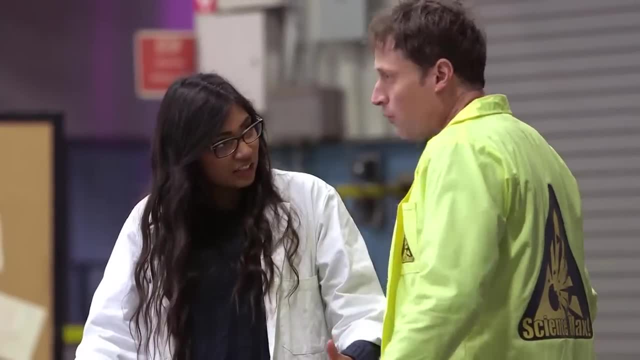 WHAT IF WE JUST GOT A REALLY LARGE CONTAINER? SO YOU WANT TO CARBONATE A VERY LARGE CONTAINER? WE HAVE TO FIGURE OUT SOME WAY TO WELL, COME ON, LET'S GO FIGURE IT OUT. OKAY, LET'S DO IT. 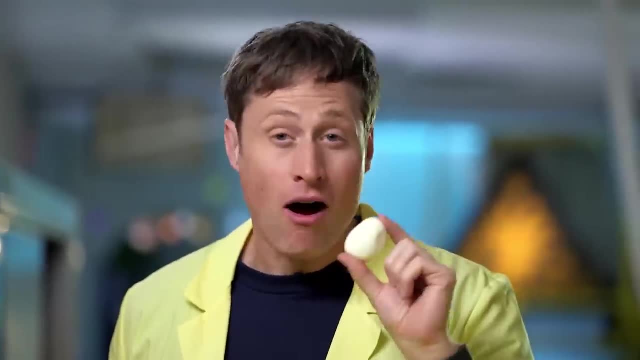 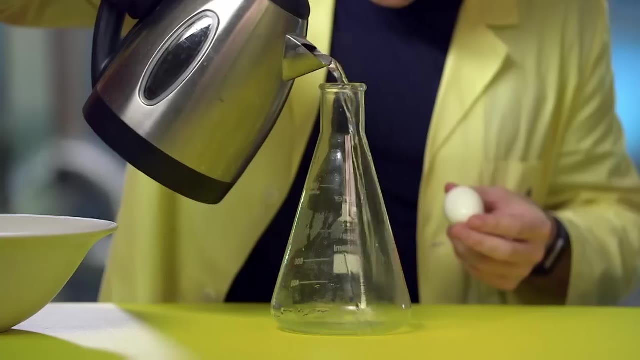 MINIMAX. THIS IS AN EGG. IT'S BEEN HARD-BOILED AND PEELED, SO THERE'S NO SHELL ON IT. THIS IS A FLASK AND THIS IS HOT WATER. I POUR THE HOT WATER INTO THE FLASK. 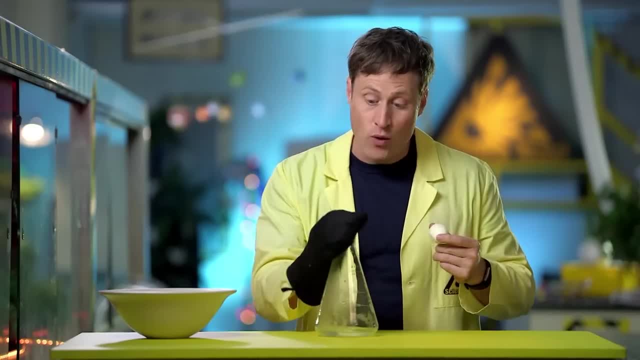 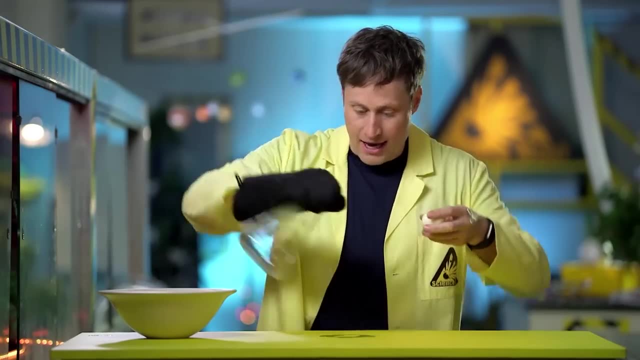 WHICH MEANS THE AIR INSIDE THE FLASK STARTS TO HEAT UP, AND WHEN IT HEATS UP, IT EXPANDS AND SOME ESCAPES THROUGH THE TOP OF THE BOTTLE. I POUR THE WATER OUT AND THEN I CAP THE FLASK WITH THE EGG. 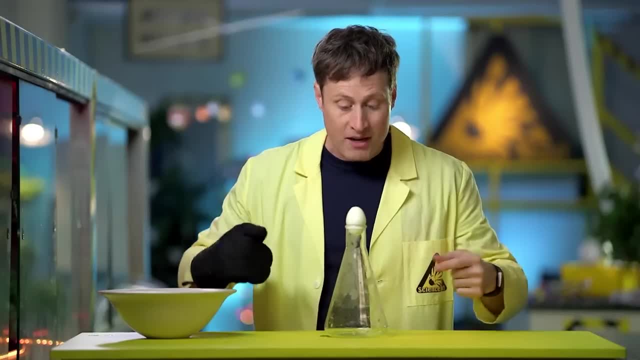 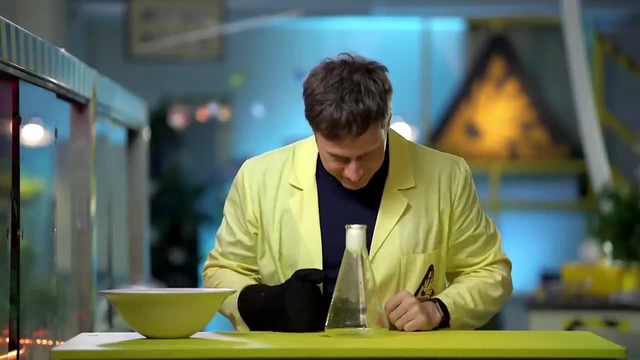 NOW THIS EXPANDED AIR IS STARTING TO COOL AGAIN, WHICH MEANS IT'S LOWER PRESSURE, WHICH MEANS THE HIGHER PRESSURE ON THE OUTSIDE OF THE FLASK PUSHES THE EGG IN HA-HA FUN. 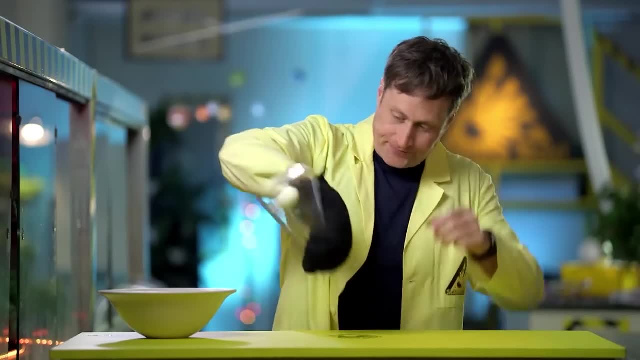 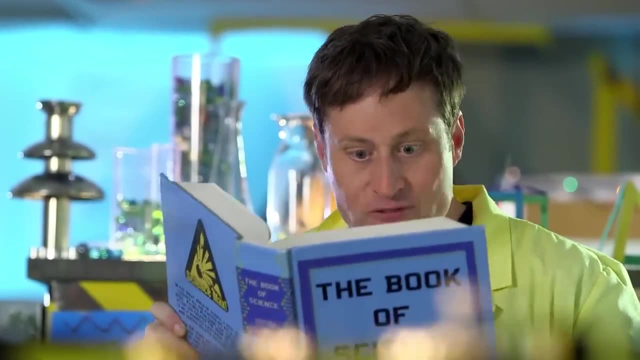 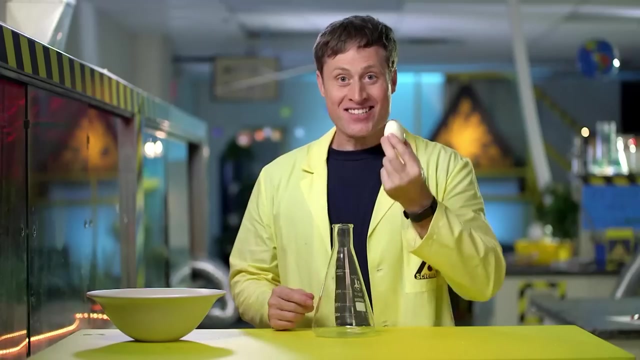 AND THEN TO GET THE EGG OUT. AH, I CAN REVERSE IT. IF I BLOW INTO THE FLASK, I CAN INCREASE THE PRESSURE INSIDE. AH, HA-HA-HA, SCIENCE. AND NOW LET'S MAX IT OUT. 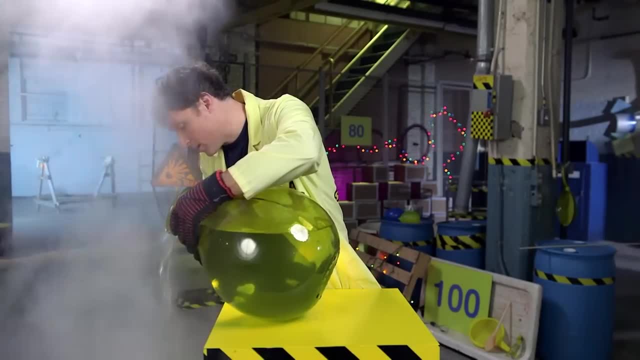 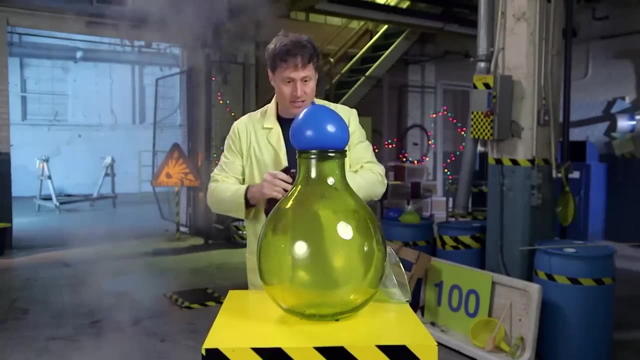 MAX OUT CONTAINER. OK, POUR OUT THE WATER. OH, CAREFUL, CAREFUL. AND NOW I PUT THIS WATER BALLOON ON THE TOP AND WE'LL JUST SEE WHAT HAPPENS THE HOT EXPANDED AIR INSIDE THE CONTAINER. 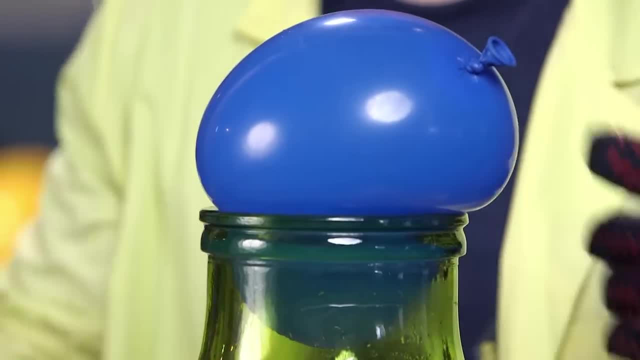 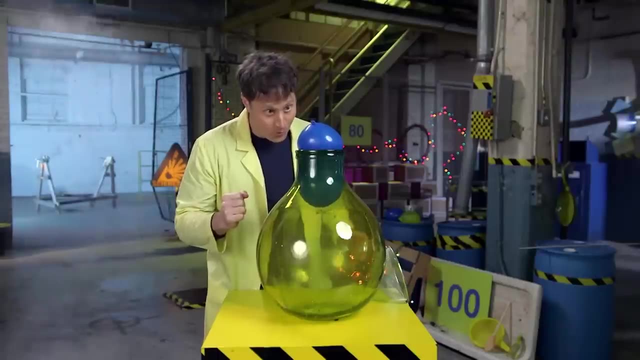 IS COOLING AND REDUCING IN PRESSURE, WHICH MEANS THE HIGHER PRESSURE OUTSIDE THE CONTAINER. IT'S HAPPENING PUSHES THE BALLOON IN IT'S HAPPENING SUCCESS. 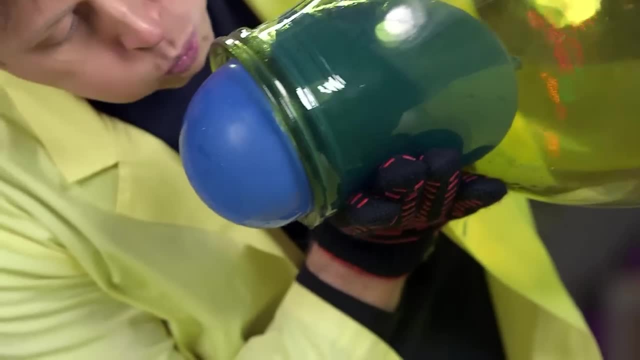 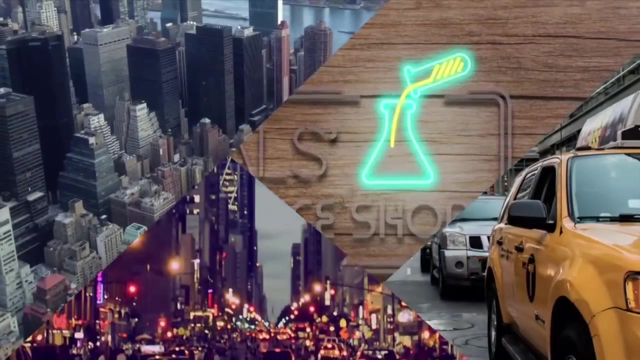 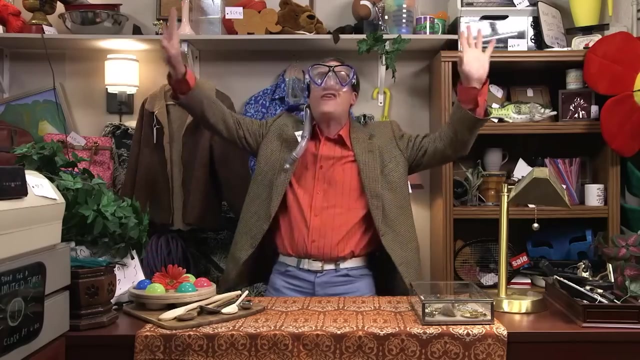 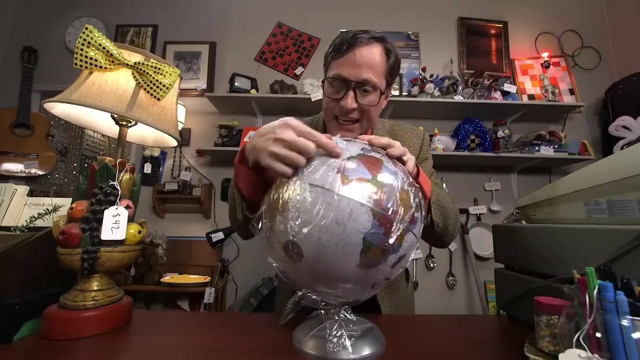 MAXED OUT. HMM. DID YOU KNOW THAT WE LIVE ON THE BOTTOM OF AN OCEAN OF AIR? YEAH, IT'S CALLED THE ATMOSPHERE AND COMPARED TO THE EARTH, IT'S REALLY THIN. 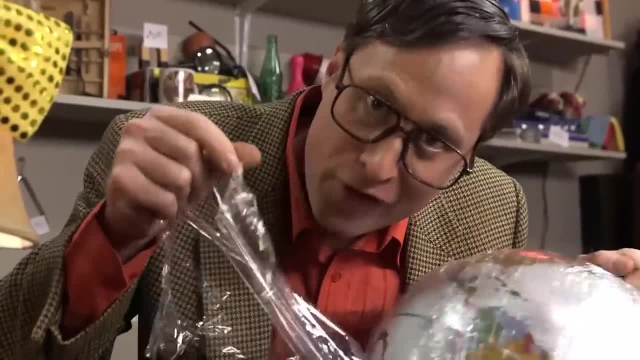 I MEAN IT'S ABOUT AS THIN AS THIS. HUH, HUH, LOOK AT THAT. NOT VERY THICK AT ALL, BUT IT'S A GOOD THING. THE ATMOSPHERE IS AROUND, AND NOT JUST FOR BREATHING. 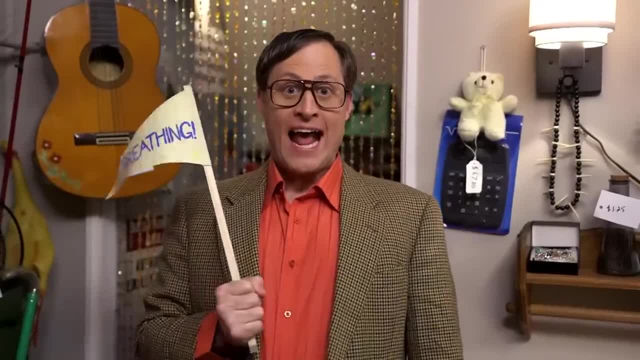 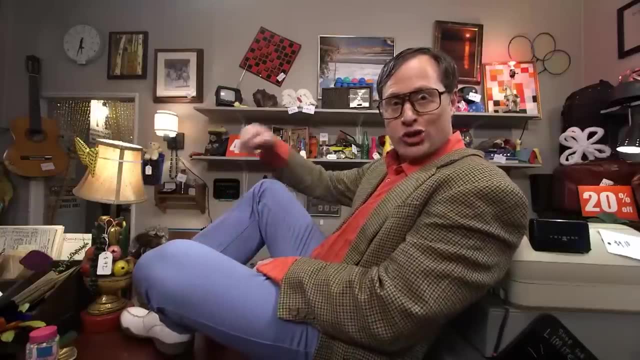 SO I AM A FAN OF BREATHING. WHAT DO WE WANT BREATHING? WHEN DO WE WANT IT? ALL THE TIME, BUT DID YOU KNOW? THE ATMOSPHERE HAS DIFFERENT LAYERS. IT'S TRUE. I WILL WALK YOU THROUGH THEM. 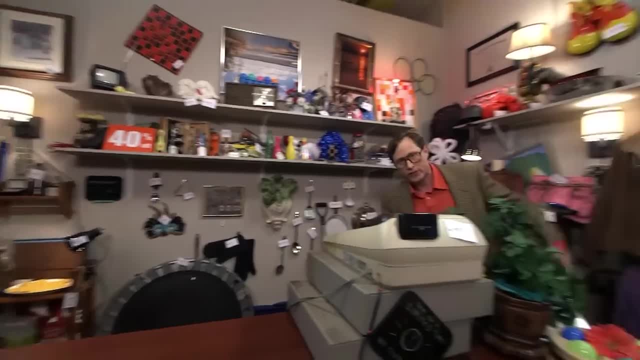 NO, I MEAN, COME ON, YOU GOT TO COME WITH ME. I'M WALKING OVER TO WALK YOU THROUGH THEM. OKAY, THE TROPOSPHERE. THIS IS THE LAYER WHERE WE ARE ALL EXISTING RIGHT NOW. 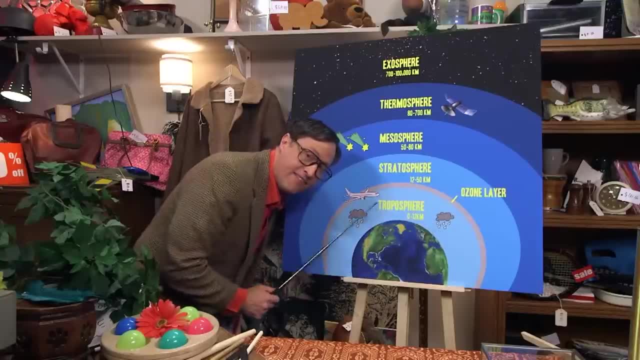 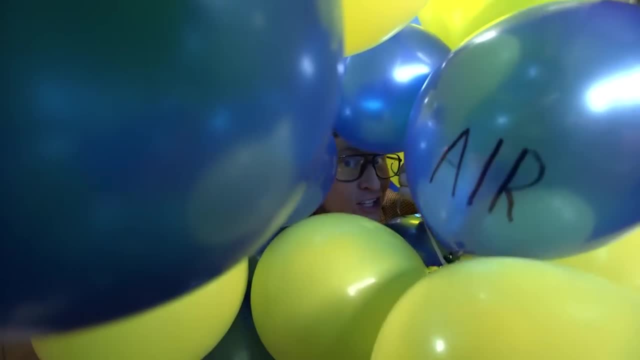 WHERE ALL OF OUR WEATHER HAPPENS. THERE'S A LOT OF AIR MOLECULES IN THIS LAYER. THINK OF THESE BALLOONS AS AIR MOLECULES. THERE'S A LOT OF AIR IN THIS LAYER. YAY AIR. 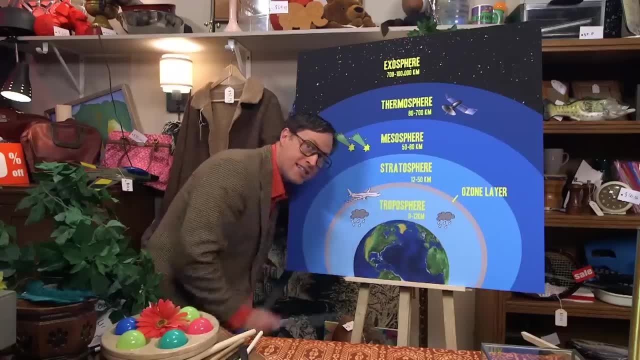 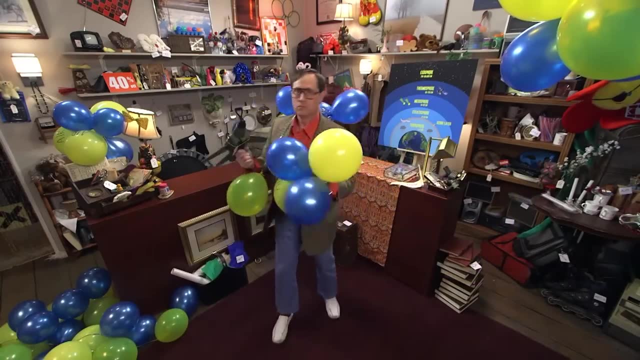 NEXT LAYER: THE STRATOSPHERE. THERE'S LESS AIR MOLECULES IN THIS LAYER AND IT'S WHERE TROPOSPHERE IS JETS FLIGHT. NEXT LAYER: THE MESOSPHERE. THERE'S EVEN FEWER AIR MOLECULES IN HERE. 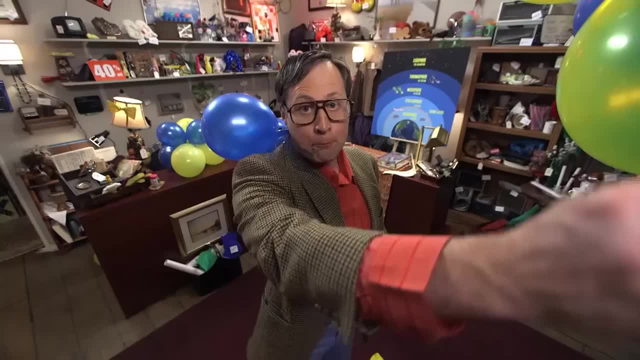 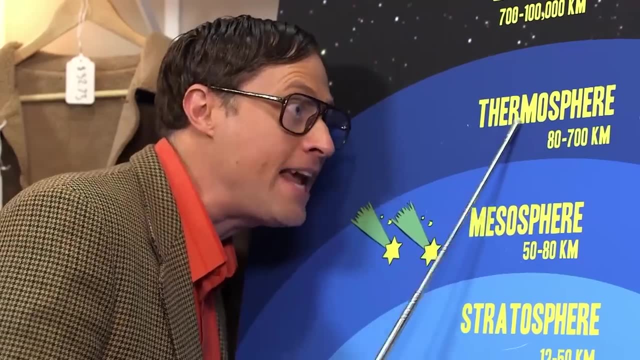 AND IT'S WHERE MEDIAS BURN UP AND TURN INTO SHOOTING STARS. FIRE, FIRE, FIRE, FIRE THE THERMOSPHERE, NOT MANY AIR MOLECULES LEFT UP HERE, AND THIS IS WHERE THE NORTHERN LIGHTS. 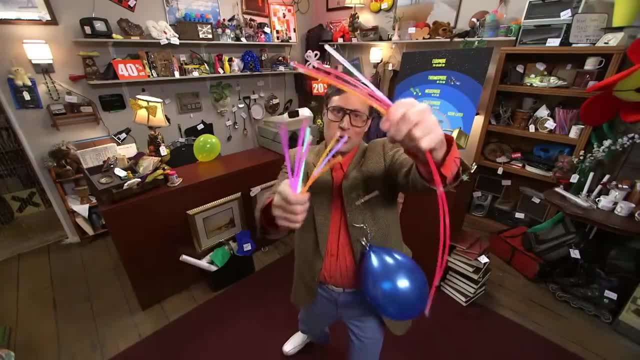 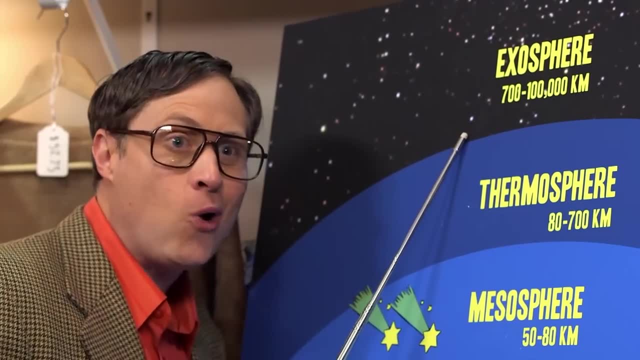 THE AURORAS, HAPPEN WHOO, NORTHERN LIGHTS AND FINALLY, THE AEROSPHERE. THIS IS AS HIGH AS THE ATMOSPHERE GOES. THIS IS WHERE SATELLITES ORBIT. 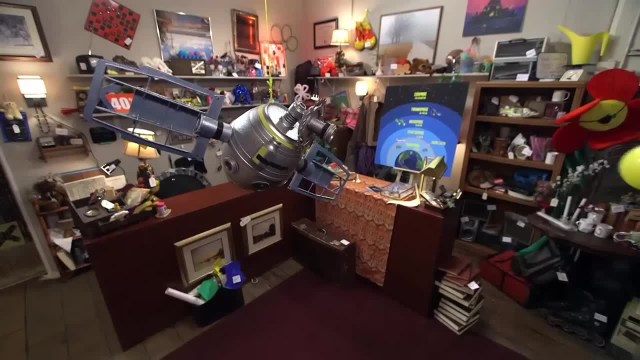 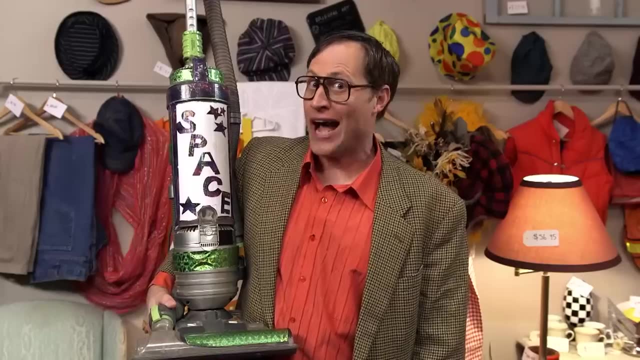 AND IF YOU SEE ANY AIR MOLECULES UP HERE, THEY'RE JUST PASSING THROUGH, HELLO, AND AFTER THAT, NOTHING BUT THE VACUUM OF SPACE, OOH, THE VACUUM OF SPACE OF COURSE. YOU KNOW, IT'S NOT THAT KIND OF VACUUM, RIGHT. 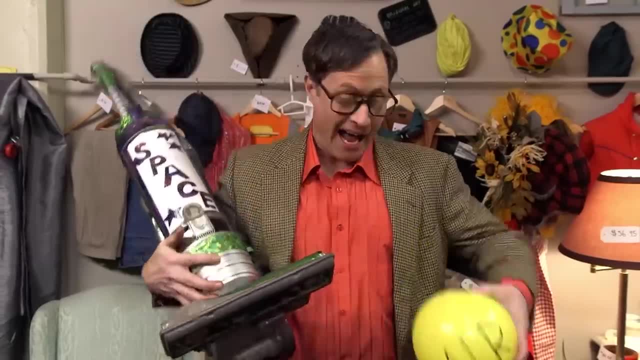 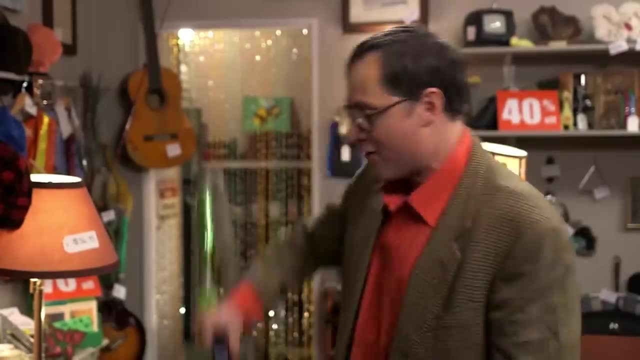 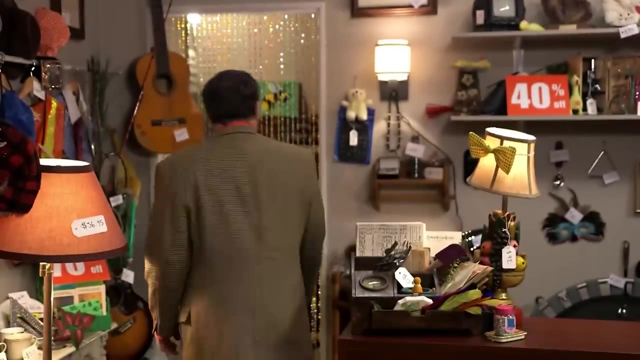 RIGHT VACUUM JUST MEANS NO AIR. THERE YOU GO: THE ATMOSPHERE, THE ONLY THING SEPARATING US FROM THE VACUUM OF SPACE. HA HA, ROBERTA, YOUR SPACE VACUUM GOT BROKEN. 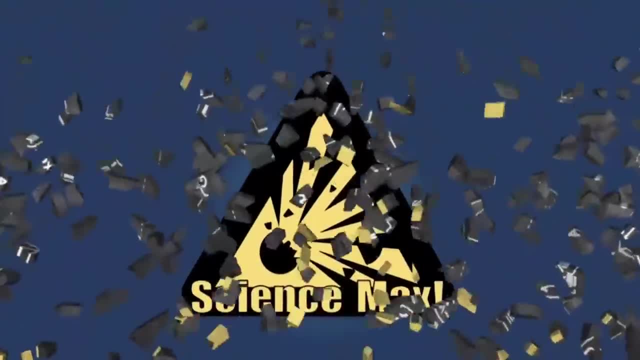 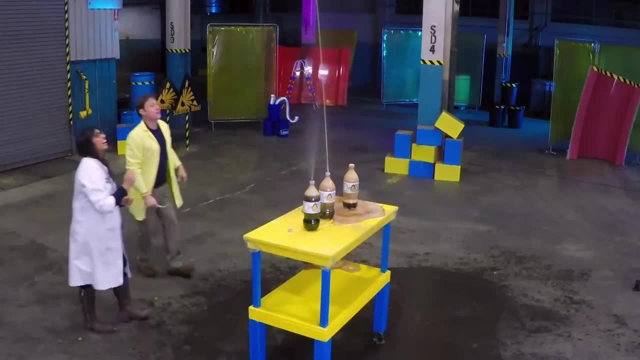 I DON'T KNOW HOW. WHOA CYNTHIA AND I ARE MAXING OUT THE NUCLEATION FOUNTAIN. WHOA, THIS ONE IS ALMOST LIKE A SPRAY. IT'S NOT LIKE A MIST. YEAH, A MIST. 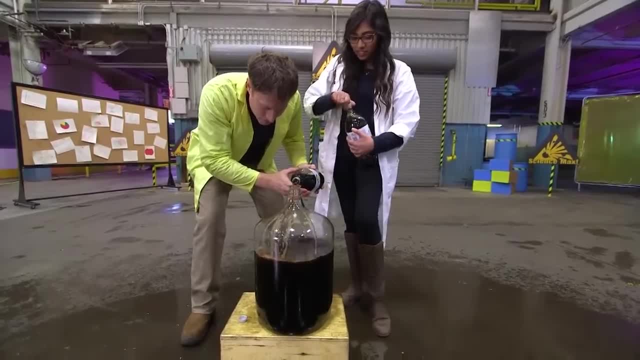 IT'S A MIST OF COLA. JUST TO EXPERIMENT, WE TRIED USING A GIANT BOTTLE AND POURING THE DIET COLA IN. I'M A LITTLE CONCERNED ABOUT THE SCIENCE, BUT IT DIDN'T WORK. 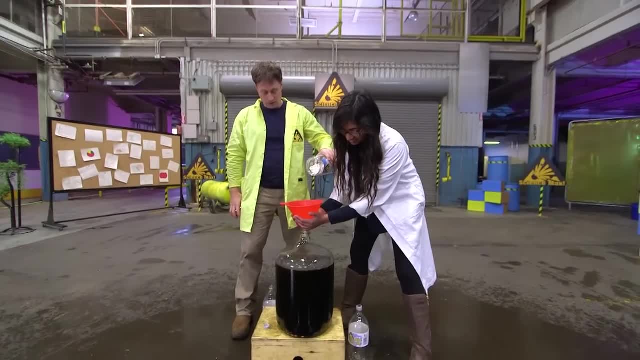 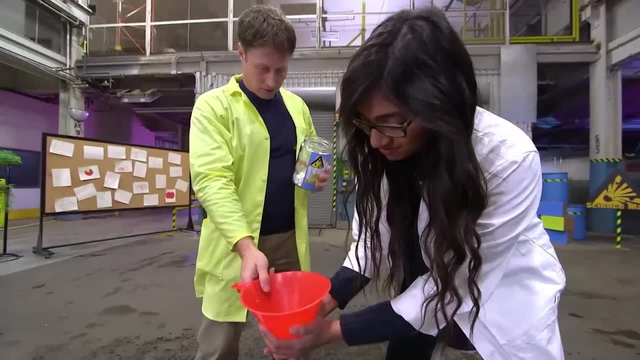 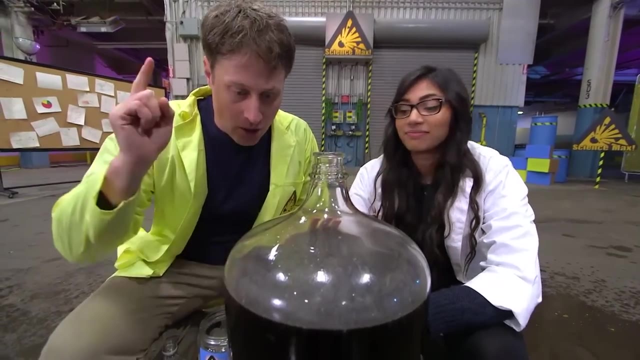 WELL, THAT'S NOT VERY EXCITING. OKAY, SO THAT DIDN'T WORK AT ALL. NO, THIS IS NOT A CHEMICAL REACTION. IT'S A PHYSICAL CHANGE, SO IT'S THE CARBONATION THAT MATTERS. 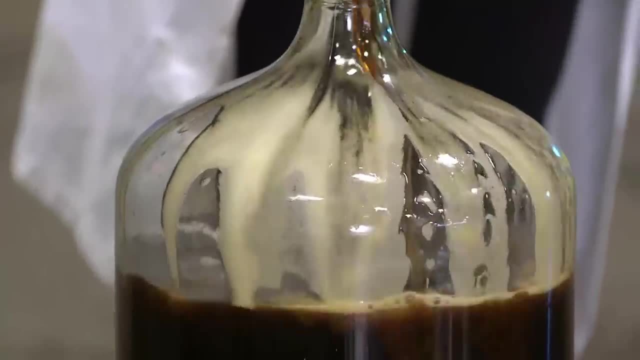 EXACTLY WHEN WE POURED THE COLA INTO THE BOTTLE, WE LOST ALMOST ALL OF IT. WE LOST ALMOST ALL THE CARBONATION. HOW ARE WE GOING TO MAX IT OUT? THAT'S THE QUESTION. 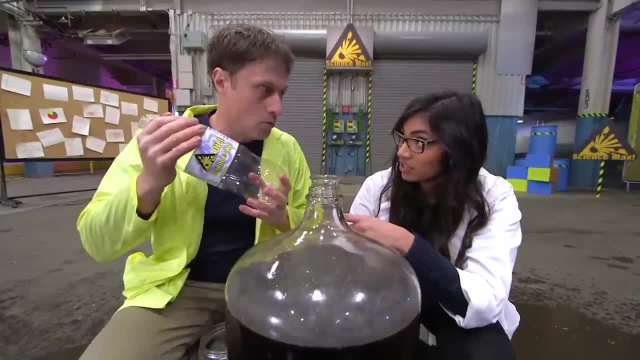 SO IF WE CAN'T MAKE A LARGER CONTAINER, MORE BOTTLES. WE JUST HAVE MORE BOTTLES, SO WE'LL JUST GET A LOT OF THEM AND WE'LL SET THEM OFF IN A SEQUENCE OR SOMETHING. 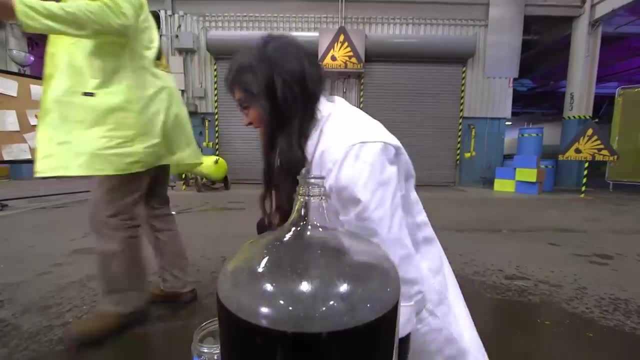 OKAY, LET'S DO A PATTERN OR SOMETHING. WE'LL MAX OUT THE FOUNTAIN. I KNOW WHAT WE SHOULD DO YOU KNOW? WE SHOULD BE SORT OF LIKE A CASCADE, AND WE'LL GET A LAZY SUSAN, OR 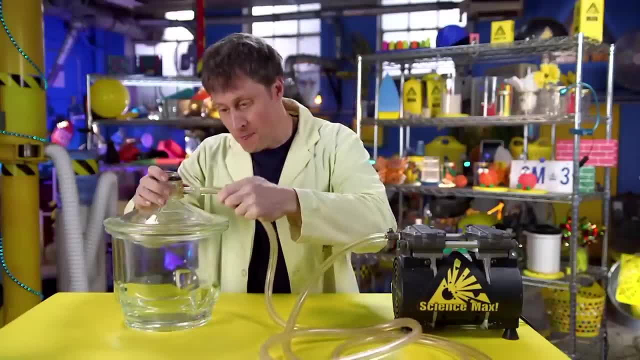 THIS IS A VACUUM CHAMBER. IT'S AN AIR-TIGHT CONTAINER AND I PUT A HOSE ON IT AND THE HOSE IS ATTACHED TO A PUMP. NOW THE PUMP TAKES THE AIR OUT OF THE CHAMBER. 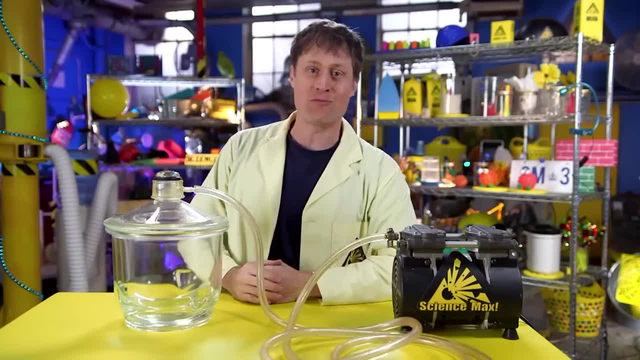 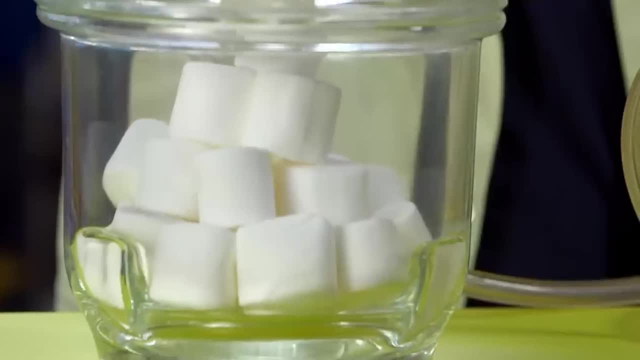 CREATING A VACUUM, SO LET'S HAVE SOME FUN PUTTING THINGS IN A VACUUM. CHAMBER- MARSHMALLOWS IN A VACUUM CHAMBER- THE MARSHMALLOWS GROW LARGER. 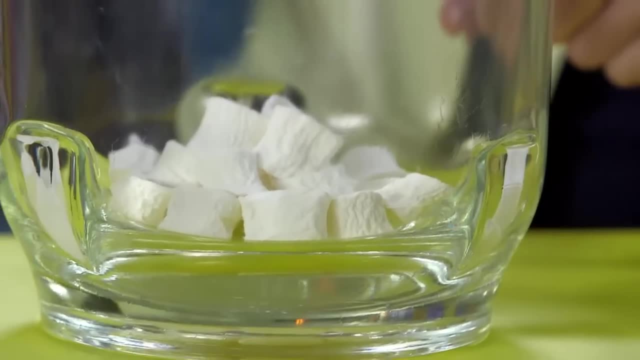 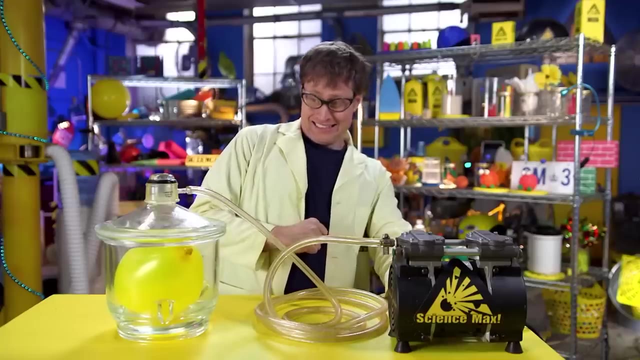 THEN SHRINK MUCH SMALLER. WHEN RETURNED TO NORMAL PRESSURE, WHY? WELL? TAKE A LOOK AT WHAT HAPPENS WITH THIS BALLOON: THE VACUUM TAKES THE AIR AND THE PRESSURE OUT OF THE CONTAINER. 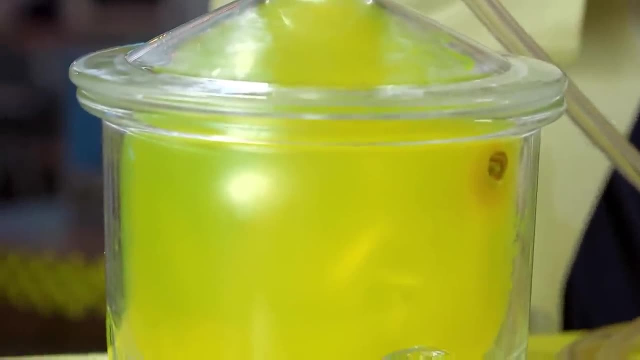 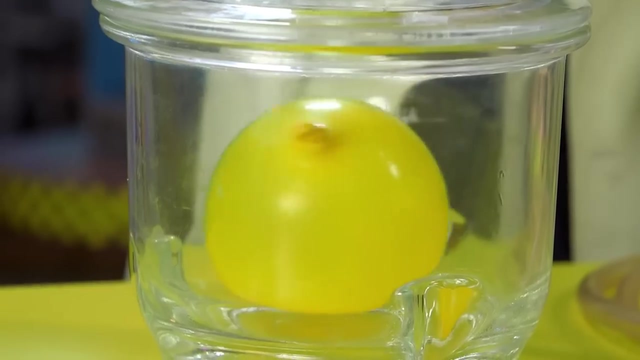 WHICH WAS PUSHING AGAINST THE SIDES OF THE BALLOON. WITHOUT THAT OUTSIDE PRESSURE, THE AIR MOLECULES INSIDE THE BALLOON CAN EXPAND, SO LET'S MAX IT OUT WITH MAXED-OUT MARSHMALLOW. 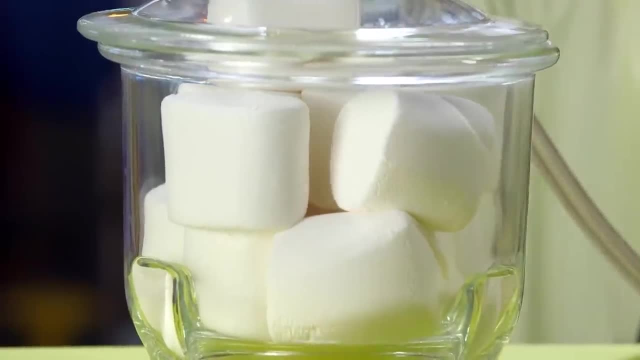 JUST LIKE THE BALLOON, THE MARSHMALLOWS EXPAND, BUT UNLIKE THE BALLOON, THE AIR IN THE MARSHMALLOWS ESCAPES, SO THEY SHRINK WHEN THE PRESSURE IS ADDED BACK IN. 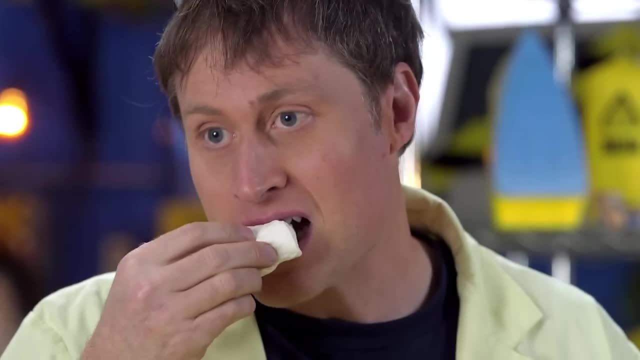 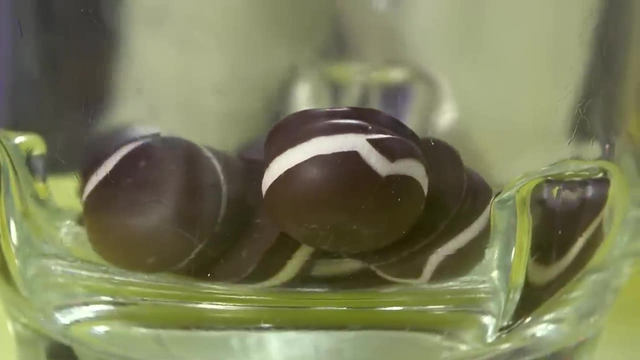 THEY'RE ALMOST THE SIZE OF REGULAR MARSHMALLOWS. IT'S THE AIR INSIDE A MARSHMALLOW. THAT MAKES IT FLUFFY. IT'S NOT VERY FLUFFY. THE SAME EXPANDING PROCESS HAPPENS WITH MARSHMALLOW COOKIES. 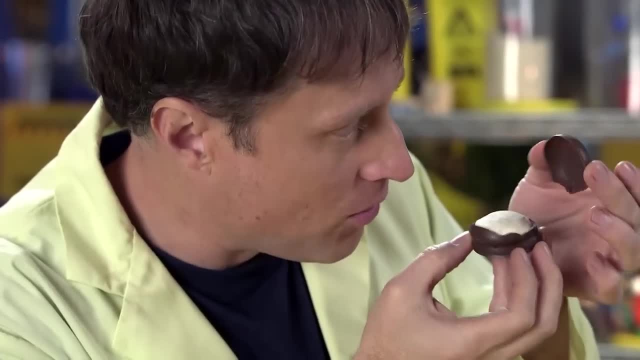 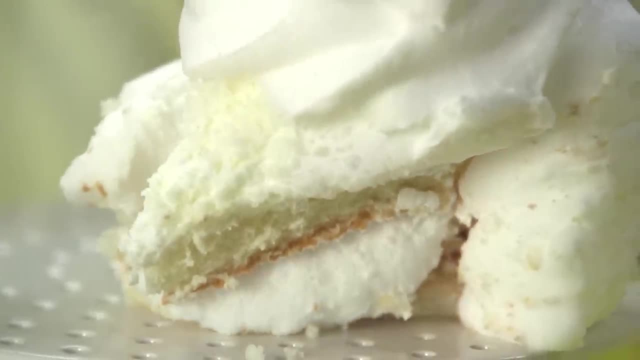 THE MARSHMALLOW HAS COMPLETELY DEFLATED, AND IT'S ALL KIND OF HOLLOW INSIDE THE FROSTING ON A CAKE, MORE CAKE, NO, NO, OOOH, HMM. LOOK AT THIS GIANT BIRTHDAY CAKE. 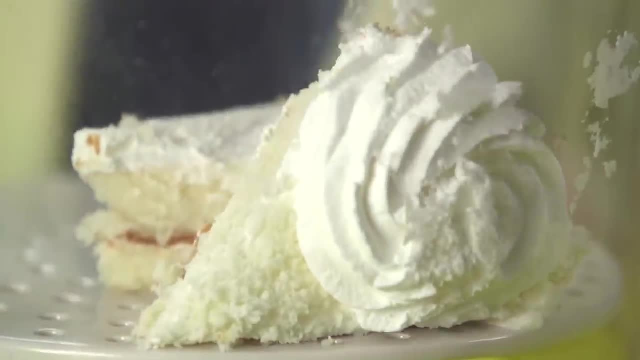 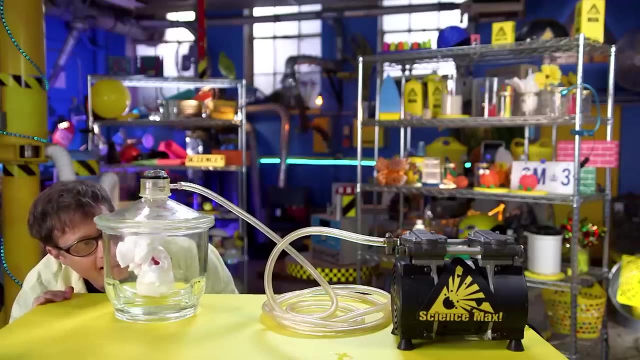 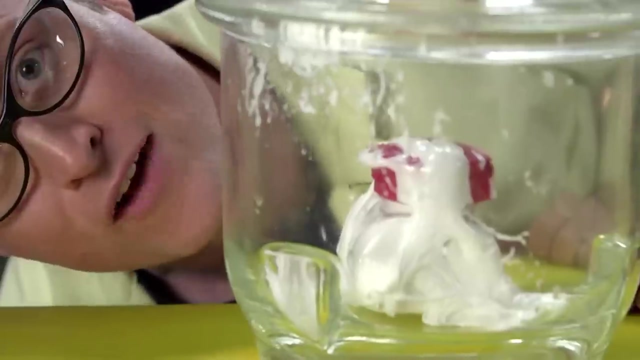 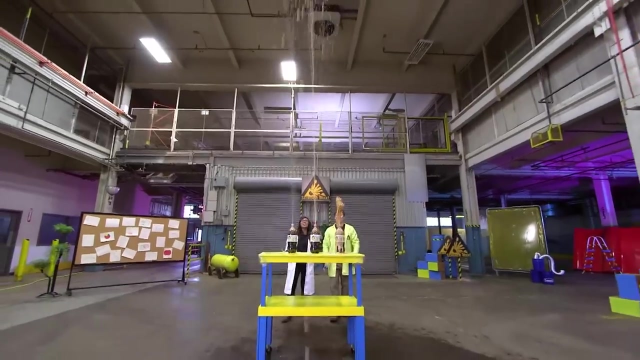 I CAN'T WAIT TO EAT IT. NO, NO, WHY? BIRTHDAY CAKE AND EVEN SHAVING CREAM? NO, SHAVING SLIME CYNTHIA. AND I HAVE DONE A WHOLE BUNCH OF DIFFERENT EXPERIMENTS. 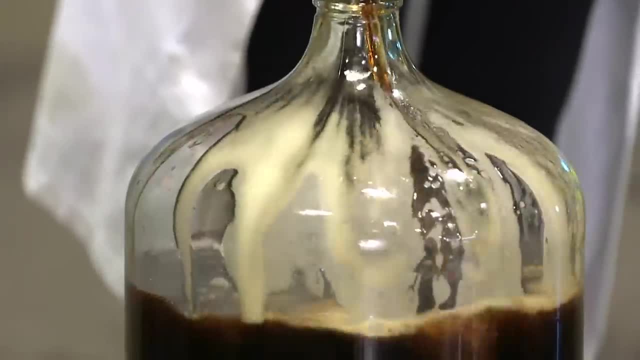 EXPERIMENTS TO FIND OUT HOW TO MAX OUT THE NUCLEATION FOUNTAIN. SO WE'LL JUST GET A LOT OF THEM AND WE'LL SET THEM OFF IN A SEQUENCE OR SOMETHING. OKAY, LET'S DO A PATTERN OR SOMETHING. 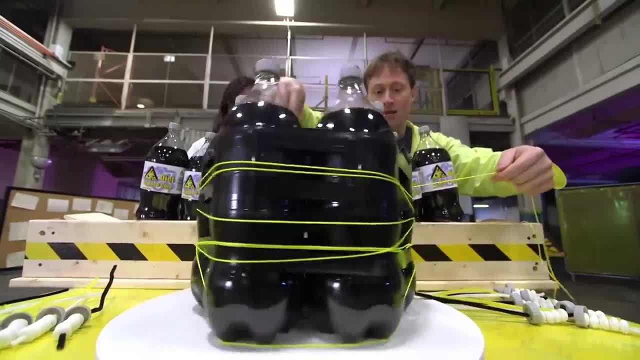 NOW WE HAVE A BUNCH OF BOTTLES AND WE'RE READY TO TRY THE MAXED OUT VERSION. WE'VE GOT OUR RELEASE MECHANISM WITH OUR MEDIUM APERTURE, YUP, AND WE'RE GONNA PUT THE MINTS. 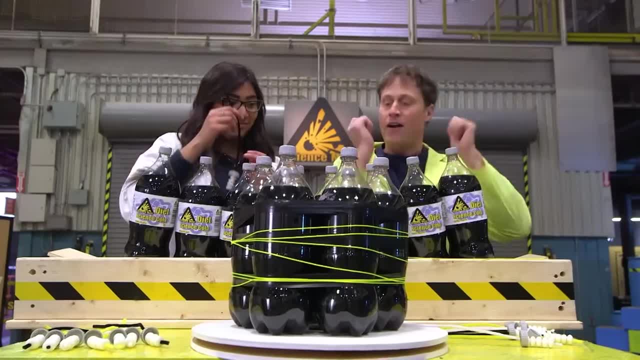 IN ALL OF THE BOTTLES, AND THEN WE'RE GONNA RELEASE THEM IN A VERY COORDINATED PATTERN- REHEARSED, PATTERN, VERY REHEARSED. WE'VE REHEARSED IT A COUPLE TIMES. 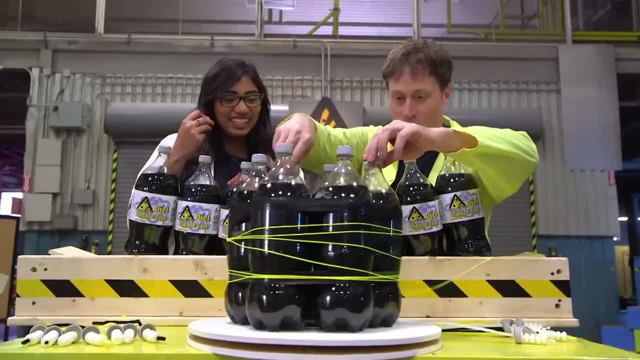 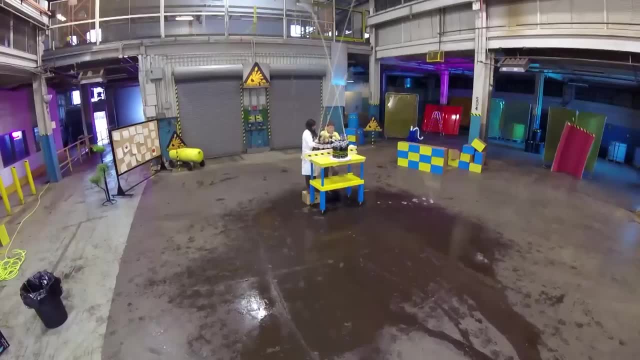 WE'LL SEE HOW IT GOES. AND WE'VE GOT THIS LAZY SUSAN WHICH WILL SPIN AROUND, AND WE'LL SEE HOW IT GOES. AND THREE, TWO, ONE, ONE, TWO, THREE, FOUR, FIVE. 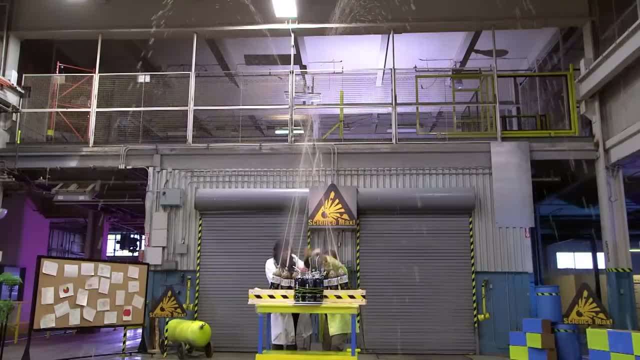 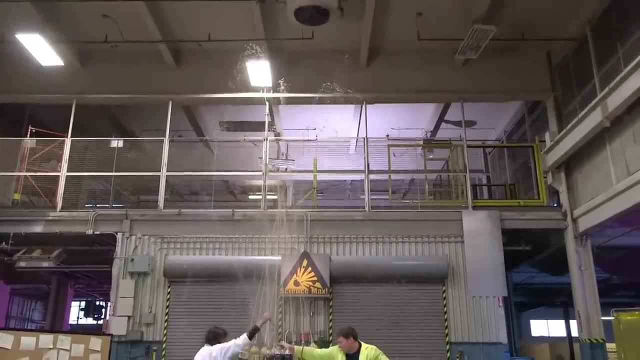 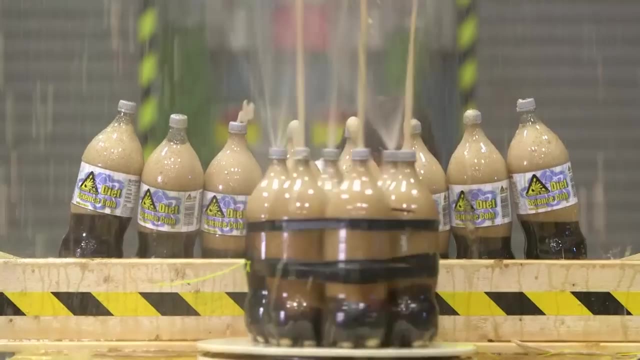 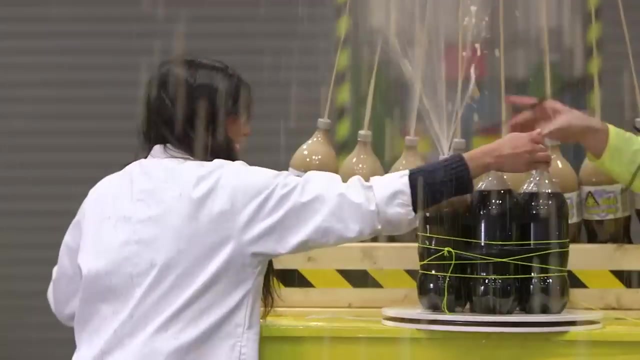 SIX, SEVEN, SURPRISE ONE, TWO, GO, GO, GO, GO. THREE FOUR. WE DID, IT, NOOOOOO, AHH, WHOA, IT'S RAINING DIET. SCIENCE COLA. 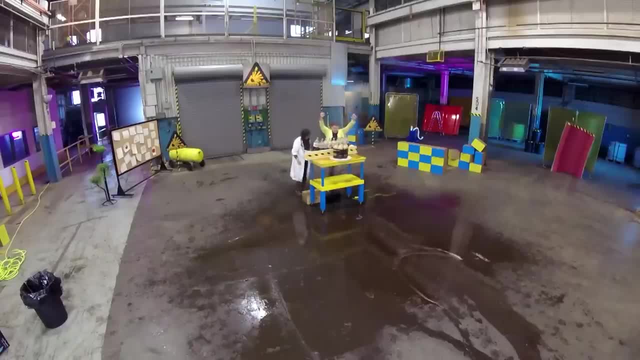 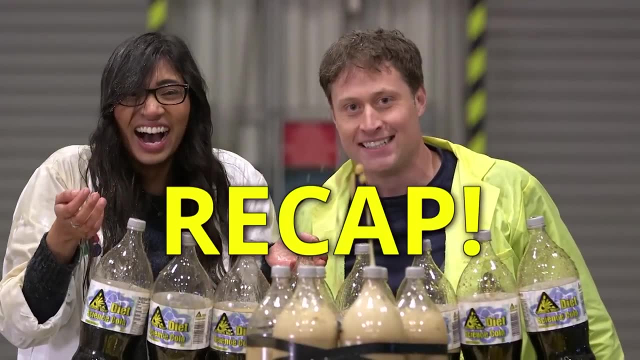 WE MAXED IT OUT. MAXED OUT NUCLEATION FOUNTAIN. THAT IS AS GOOD AS IT'S GONNA GET. SO LET'S RECAP: OUR NUCLEATION FOUNTAIN IS ALL ABOUT RELEASING THE CARBONATION. 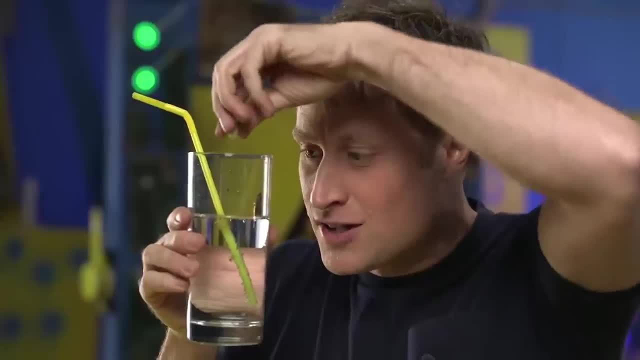 IN OUR DIET COLA FASTER THAN NORMAL. THIS HAPPENS BECAUSE THERE'S LOTS OF TINY BUMPS ON THE MINTS FOR THE CARBON DIOXIDE TO GRAB, ONTO AND MAKE BUBBLES. 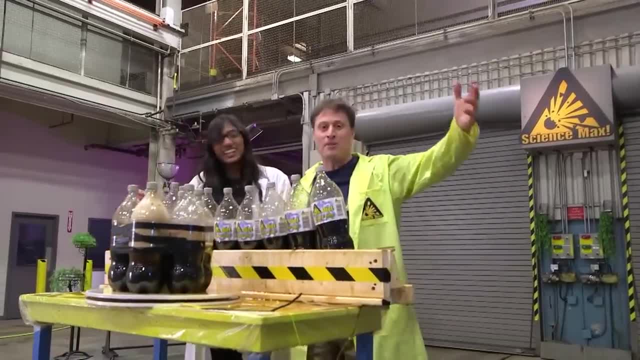 HIGH FIVES. THERE YOU GO. SCIENCE MAX, EXPERIMENTS AT LARGE NUCLEATION FOUNTAIN- EXCELLENT JOB. NOW, ALL WE NEED TO DO IS CLEAN IT UP, CLEAN UP, AND I THINK I NEED A SHOWER WITH WATER. 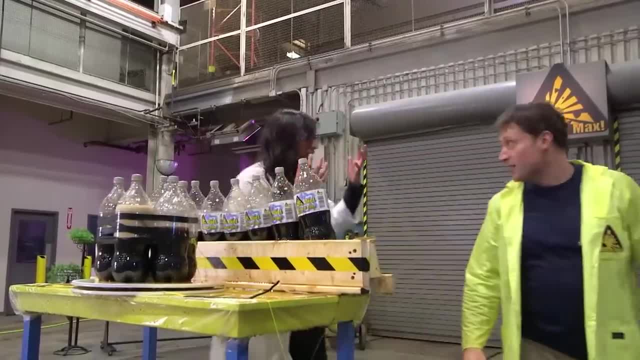 YEAH, I THINK I NEED AT LEAST A TOWEL. YEAH, BUT IT'S SUPPOSED TO VOLUMIZE YOUR HAIR, I HOPE SO. GREETING SCIENCE MAXIMITES. WELCOME TO SCIENCE MAX. 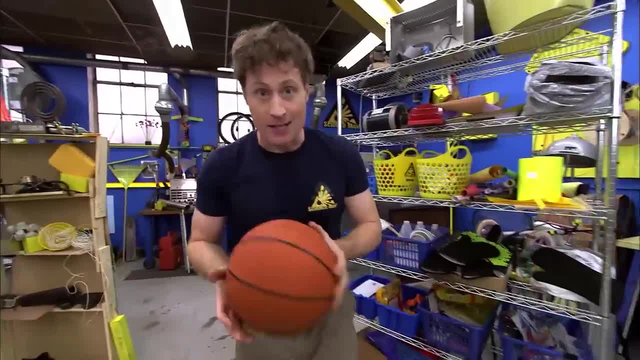 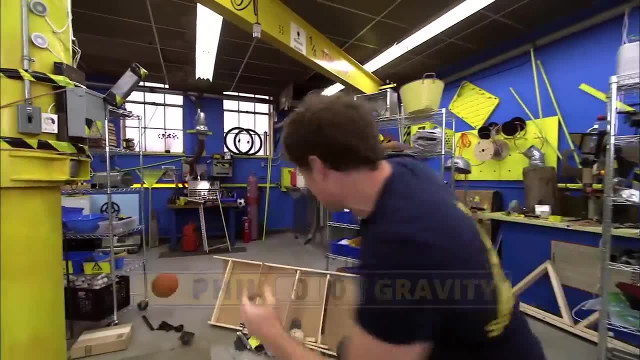 EXPERIMENTS AT LARGE. MY NAME IS PHIL AND TODAY, ON SCIENCE MAX, WE'RE GOING TO BE LOOKING AT GRAVITY. WHAT GOES UP MUST COME DOWN TODAY. GRAVITY IS THE FORCE THAT MAKES THINGS FALL. 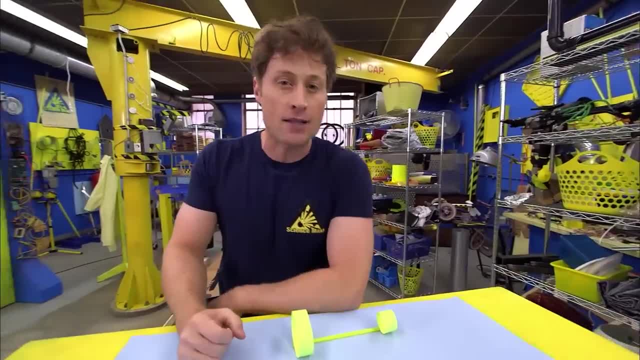 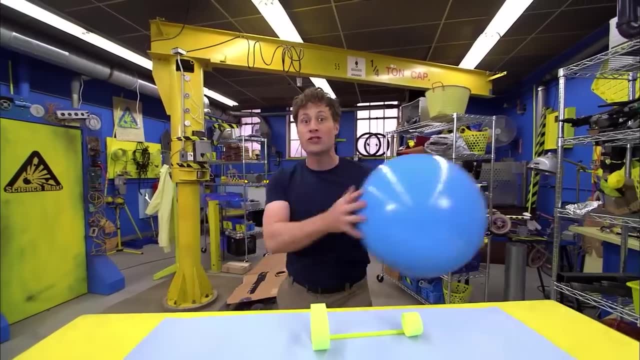 TOWARDS THE GROUND. BUT JUST BECAUSE IT'S A FORCE OF NATURE DOESN'T MEAN THAT WE HAVE TO LISTEN TO IT. NO TODAY ON SCIENCE MAX: EXPERIMENTS AT LARGE. WE'RE GOING TO USE EVERYTHING IN THE POWER. 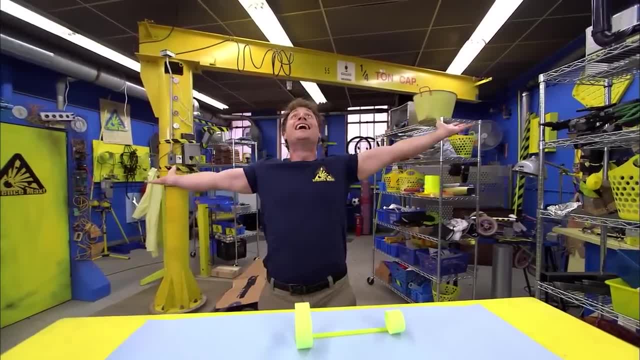 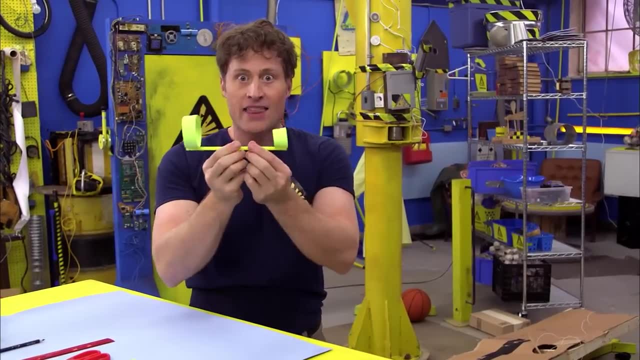 OF SCIENCE TO DEFY GRAVITY. HA HA, WE ARE GOING TO BE MAKING A HOOP GLIDER NOW. HOOP GLIDERS MAY NOT LOOK LIKE MUCH, BUT THEY FLY JUST LIKE PAPER AIRPLANES- WOOHOO. 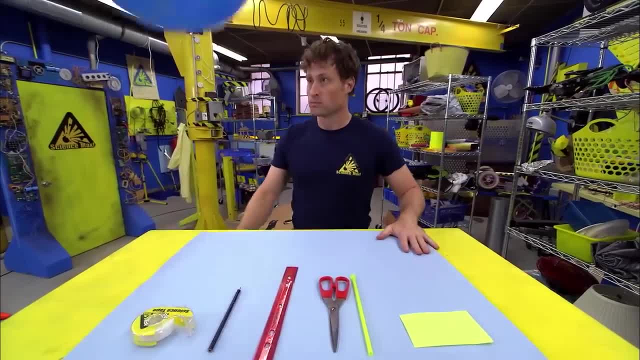 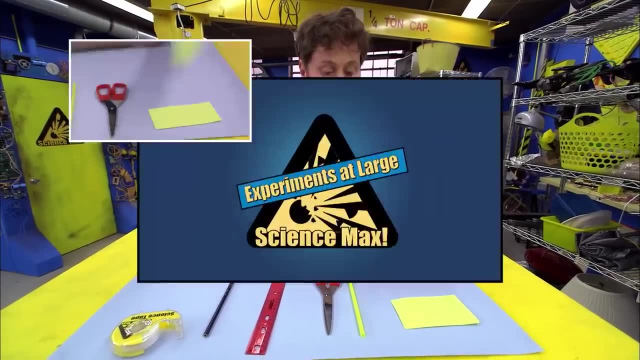 AND HERE'S HOW YOU CAN MAKE A HOOP GLIDER. HERE'S HOW YOU CAN MAKE A HOOP GLIDER ALL YOUR OWN. THIS IS WHAT YOU NEED: INDEX CARDS, SCISSORS, STRAW RULER, PENCIL AND, OF COURSE. 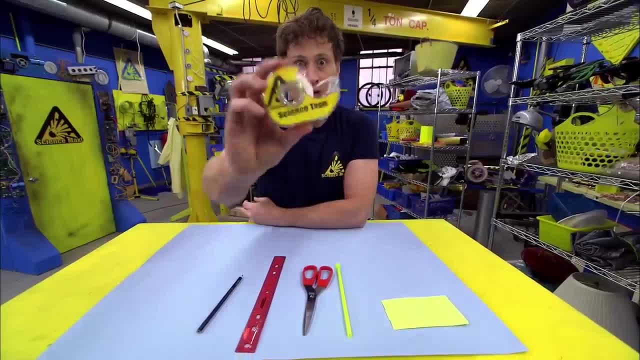 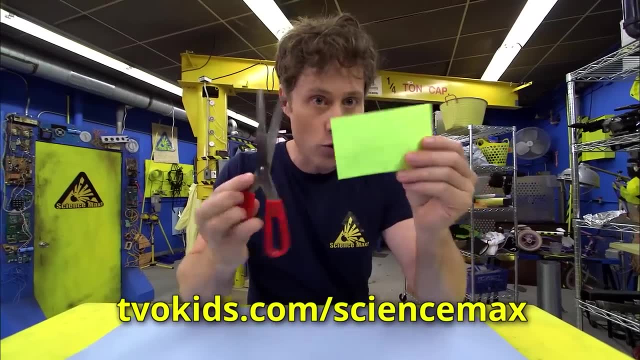 SCIENCE TAPE, WHICH IS JUST LIKE REGULAR TAPE, EXCEPT YOU USE THIS KIND OF TAPE FOR SCIENCE, SO HERE'S HOW YOU DO IT. TAKE YOUR INDEX CARD AND CUT IT INTO THREE EQUAL LENGTHS, TAKE TWO STRIPS AND YOU TAKE. 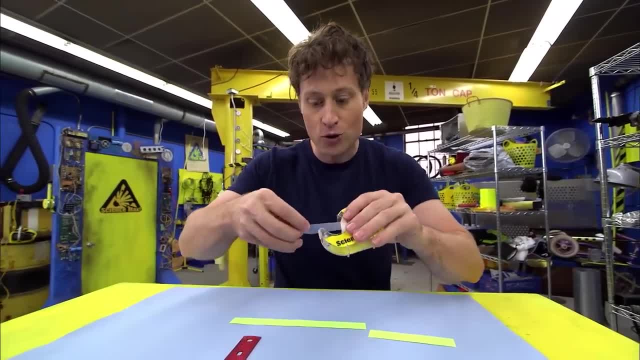 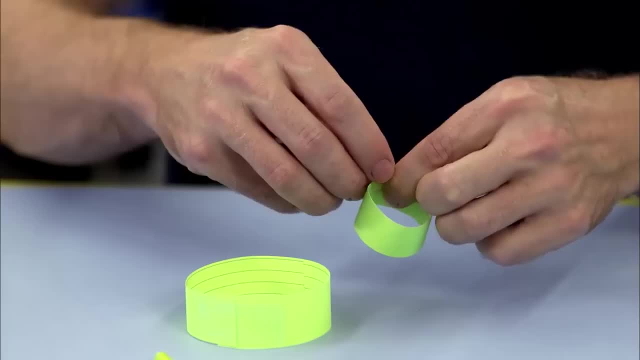 YOUR SCIENCE TAPE AND YOU TAPE THOSE TWO STRIPS AND MAKE A HOOP OUT OF IT. AND WITH A SMALL STRIP, YOU WANT TO MAKE A HOOP GLIDER. YOU WANT TO MAKE ANOTHER HOOP. NOW, WHAT YOU WANT TO DO. 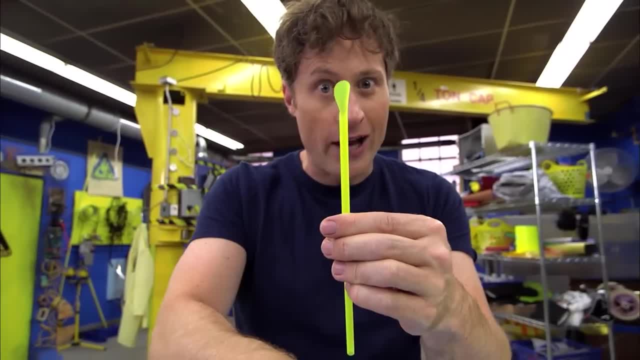 IS: TAKE YOUR STRAW NOW. THIS STRAW HAS A LITTLE SCOOP AT THE END AND THAT'S NOT VERY AERODYNAMIC, SO WE'RE GOING TO GET RID OF THAT. OOH, IT WAS KIND OF AERODYNAMIC. 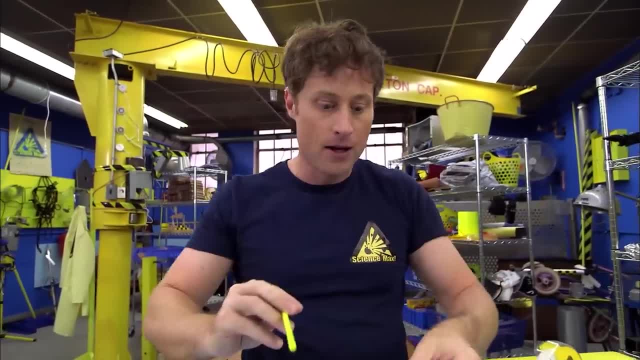 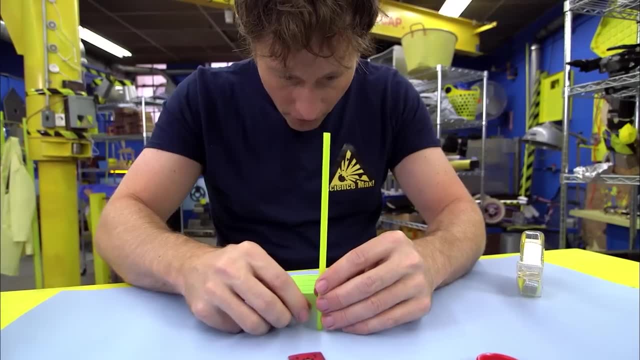 ALL RIGHT. NOW, THAT WE'VE GOT THE STRAW, YOU HAVE TO ALIGN THE HOOP AND THE STRAW TOGETHER. SO HERE'S WHAT I LIKE TO DO: TAKE SOME SCIENCE TAPE AND STICK IT ON THE STRAW, AND THEN ALIGN IT. 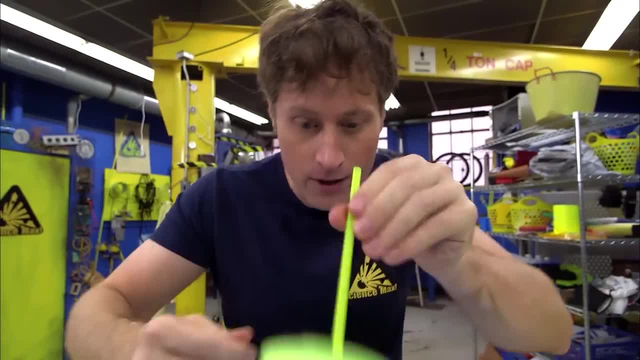 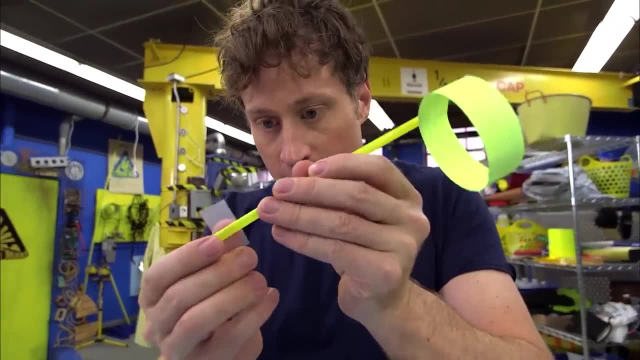 SO THAT IT'S PERFECTLY STRAIGHT. AND THEN STICK IT ON STRAIGHT TO ME ALL RIGHT. THE SMALL HOOP ALSO HAS TO BE PERFECTLY ALIGNED WITH THE FIRST HOOP. SO, AGAIN, PUT THE TAPE. 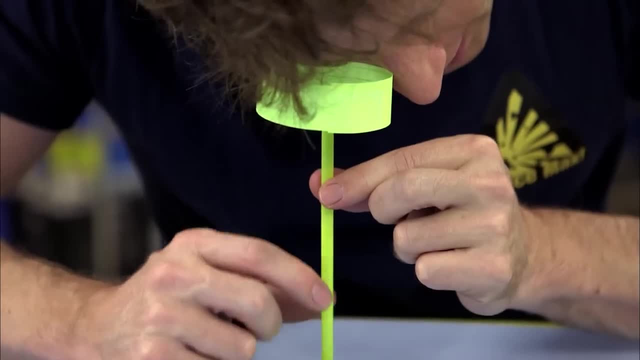 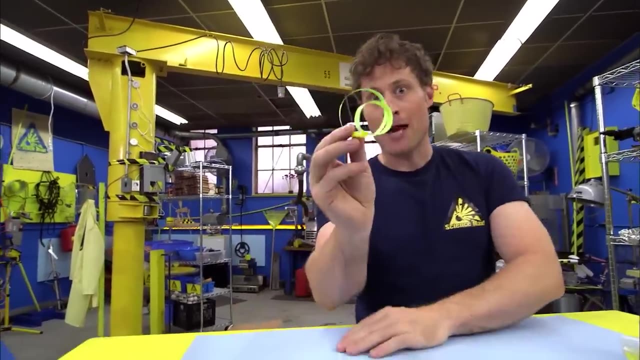 ON THE STRAW FIRST, THEN ALIGN THEM UP AND THEN START LOOKING DOWN THROUGH IT TO MAKE SURE IT'S ALIGNED THERE ONCE. YOU HAVE IT ALL TAPED TOGETHER, YOU'RE DONE YOUR HOOP GLIDER AND IT FLIES. 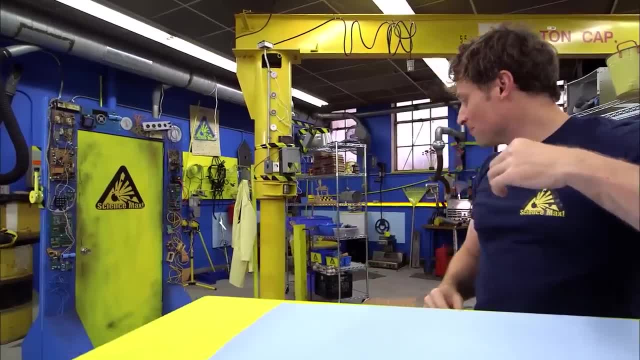 JUST LIKE A PAPER AIRPLANE PEW- AWESOME. SO THAT'S WHAT WE'RE GOING TO DO TODAY. WE'RE GOING TO: OH YEAH, I GOT TO CLEAN THAT UP. WE'RE GOING TO MAX OUT. 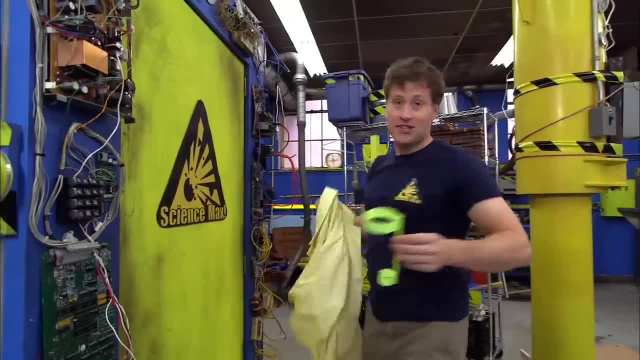 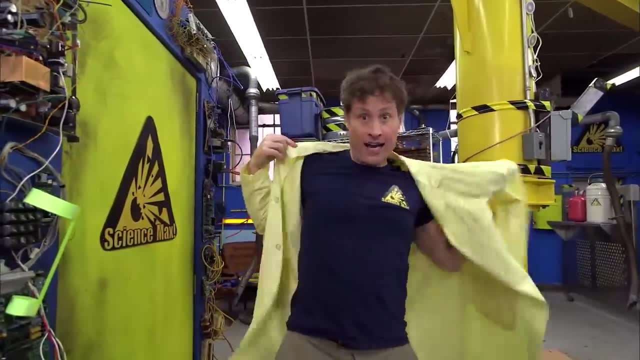 THE HOOP GLIDER. I'M GOING TO GO MEET SONIA AT THE ONTARIO SCIENCE CENTER AND WE ARE GOING TO MAX OUT THE HOOP GLIDER INTO A GIANT VERSION WE'LL PROBABLY HAVE TO CHANGE. 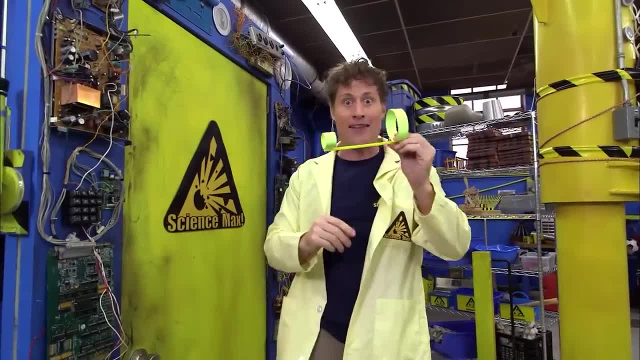 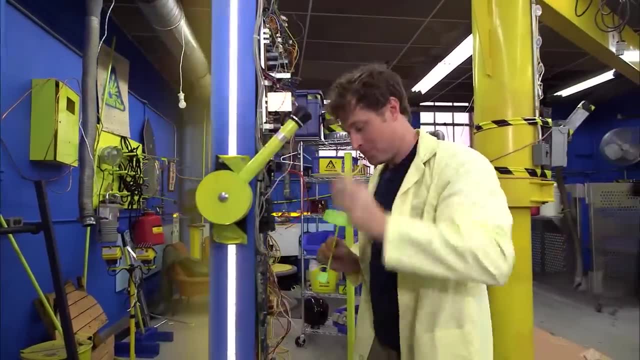 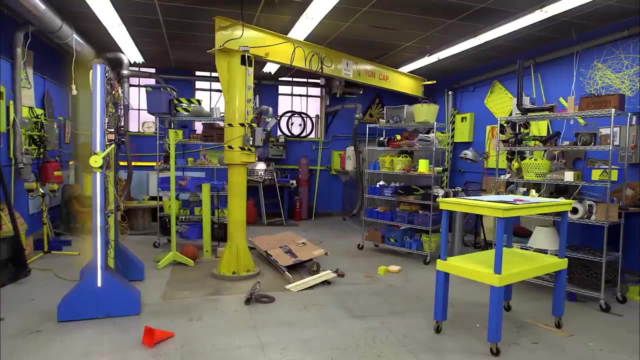 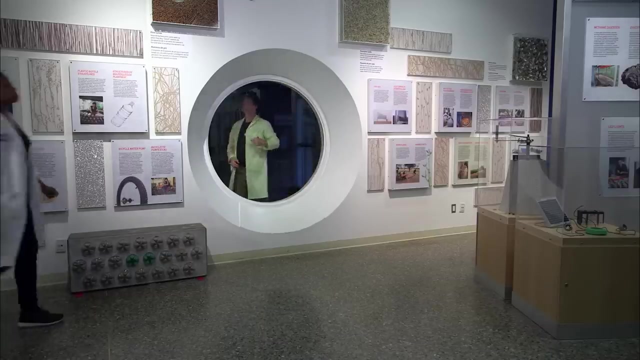 THE MATERIALS WE USE, BECAUSE I DON'T THINK WE CAN GET A STRAW THAT BIG OR A CARDBOARD, BUT STILL, WE CAN FIGURE IT OUT. ALL RIGHT, HERE I GO. HA, HA, LOOK, SONIA, SONIA. 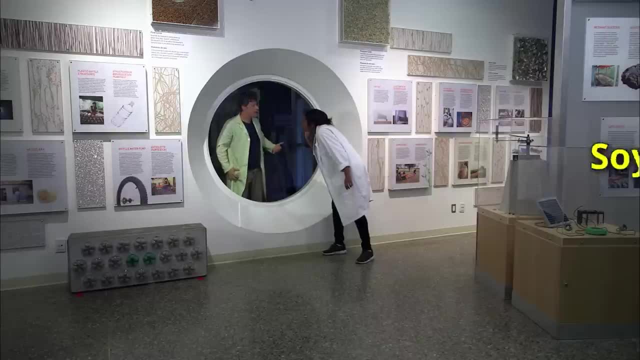 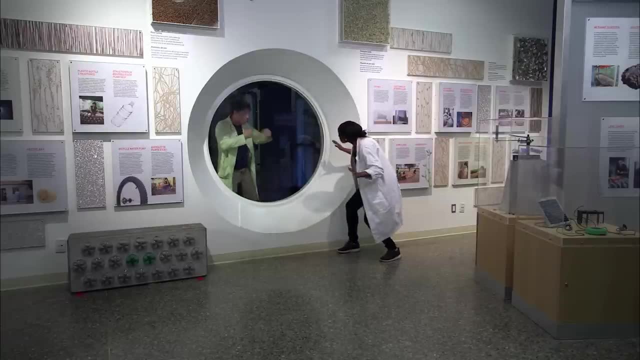 OH, HI, BELL, OH BOY, YEAH, WHAT. I WANT YOU TO HELP ME WITH AN EXPERIMENT PARTY. I WANT YOU TO HELP ME WITH AN EXPERIMENT. YOU WANT ME TO HELP YOU WITH AN EXPERIMENT. 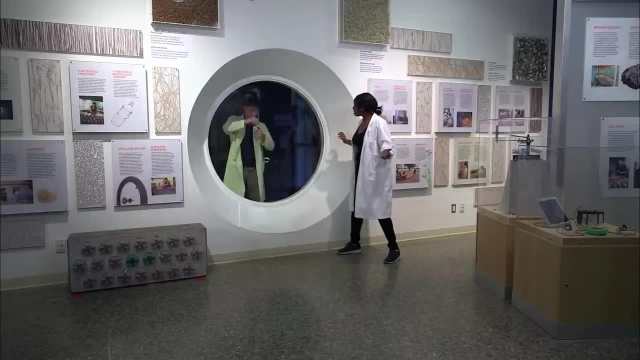 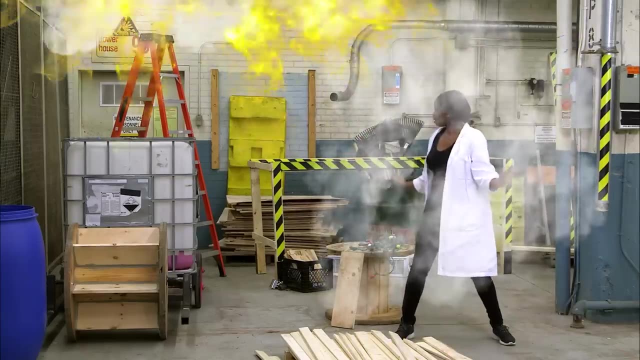 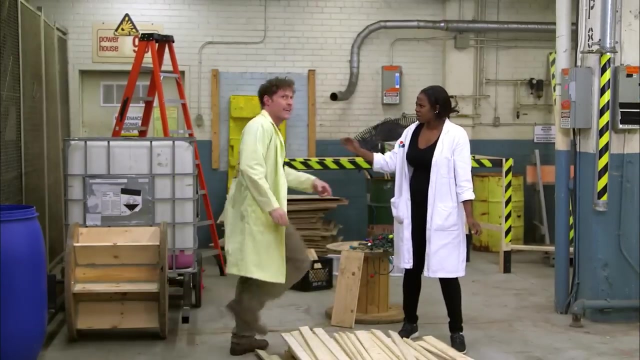 YEAH, OKAY, HOLD ON, HOLD ON, All right, No, Whoa, Oh, Sonya, I came in Phil, are you okay? Are you okay? Yeah, I'm fine, Come on, let me show you. 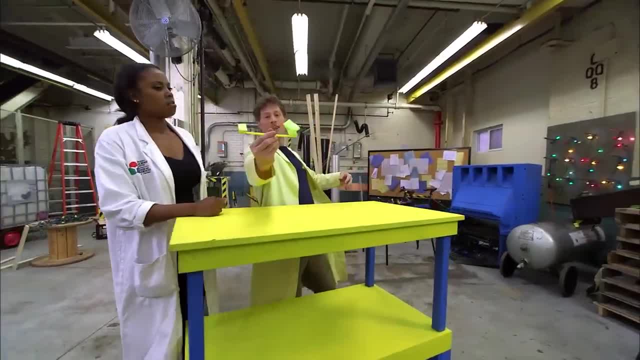 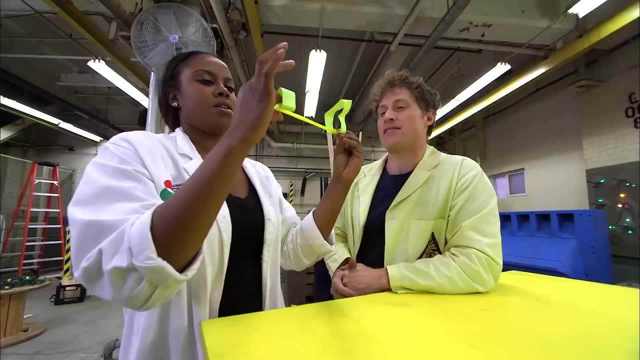 Okay, This is what I would like to max out. It was in my pocket when I fell, so What is that? It's a hoop glider. It was a hoop glider. We maxed this out First. we're gonna need a larger tube. 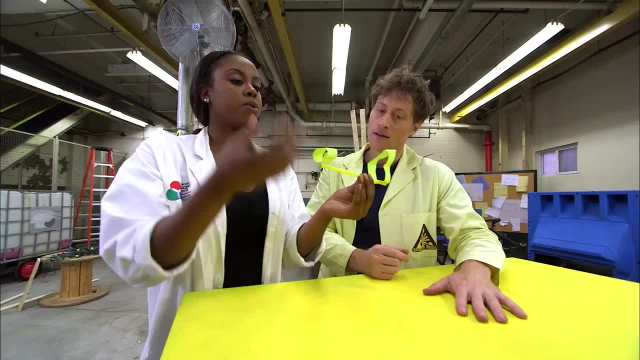 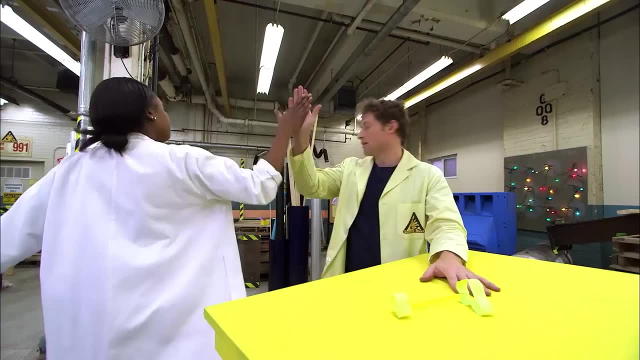 To replace the straw. yeah, Exactly, And we're gonna need two hoops. We need something that's flexible, that will convert into a hoop. Okay, that's great, So why don't we get started? Sounds good, All right, high fives. 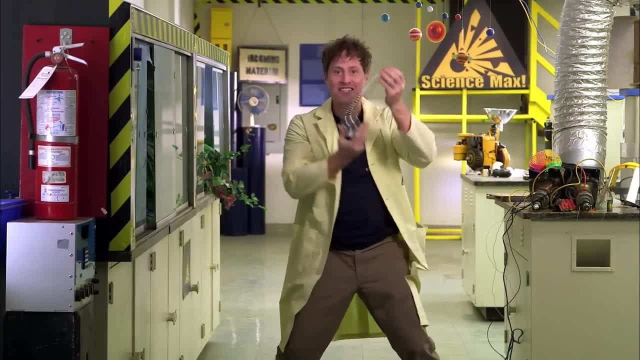 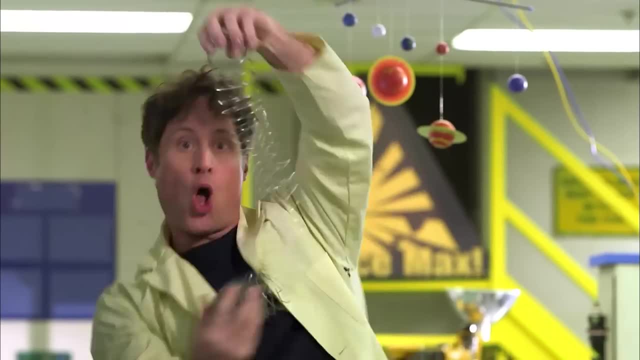 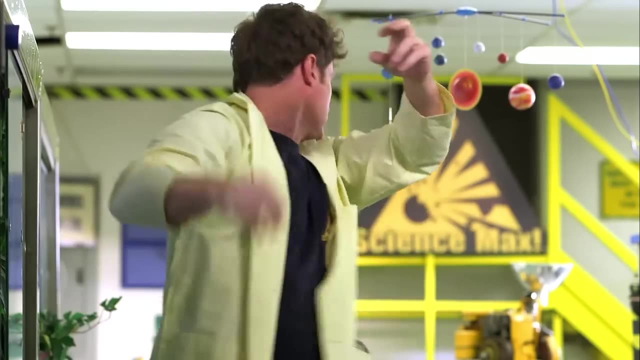 You may recognize this: It is a spring. Yes, good for you. But did you know that springs can defy gravity? Whoa Gravity, defy, Gravity, defy, Gravity, defy. Look at it fly Defying. Okay, not exactly. 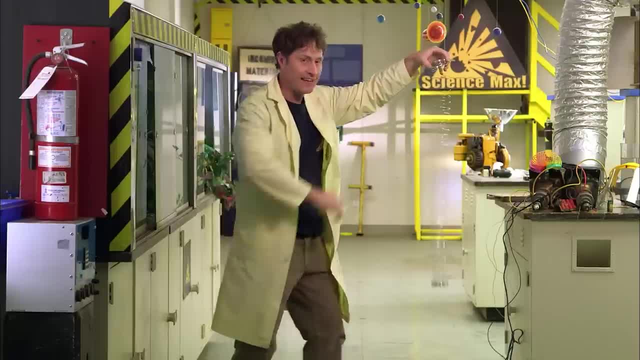 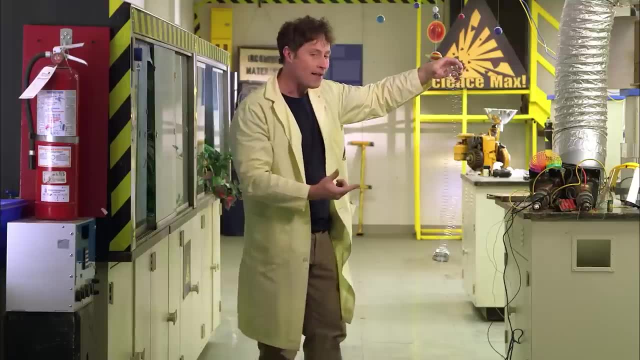 But what if I was to hold the spring like this and let it go? What'll happen? It'll fall. Yes, it'll fall, That is true. But while it's falling, what happens to this end? Does it stay in one place? 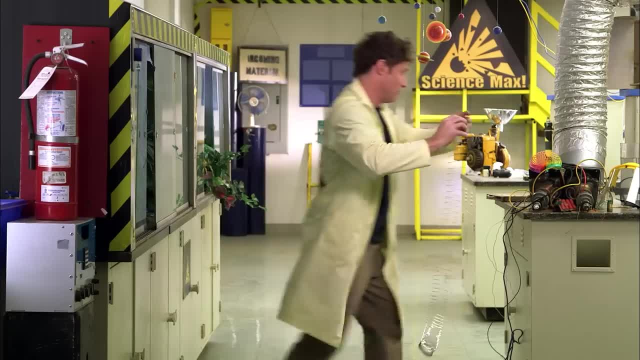 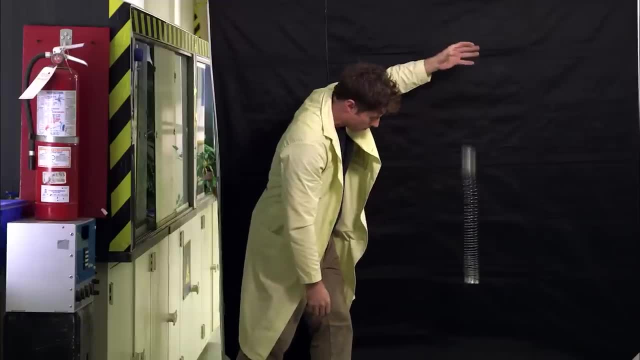 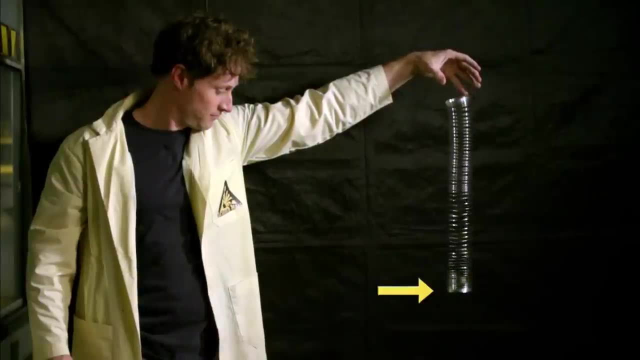 Does it go up Or does it go down? Let's find out. I'll bring this in so you can really see it. Okay, ready, Watch close. Did you see? No, Okay, tell you what. Watch it again, this time in slow motion. 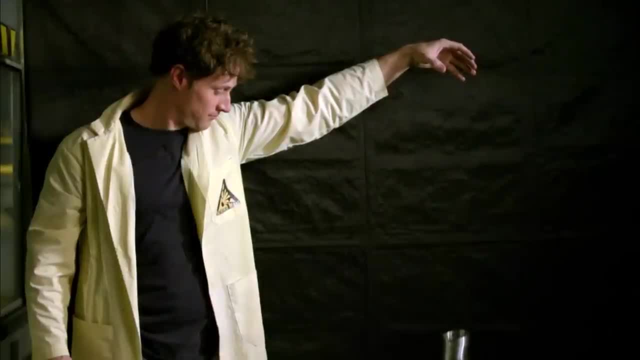 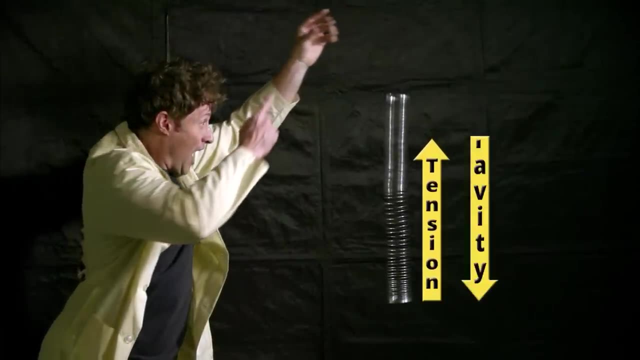 See, The bottom doesn't move, and here's why, When the top of the spring is released, gravity and the tension of the spring are pulling on it. The bottom of the spring is being pulled down by gravity and up by the tension of the spring. 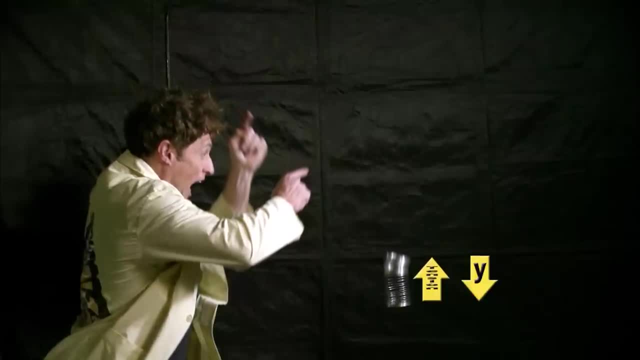 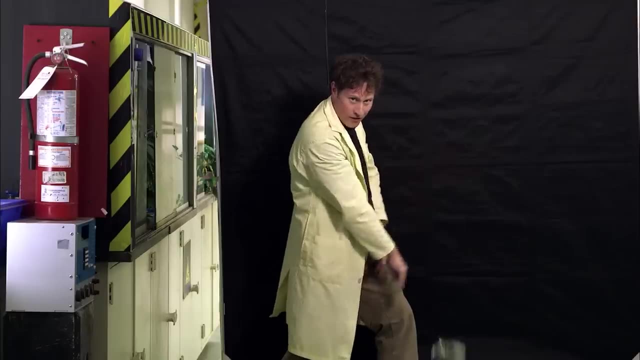 These forces cancel out, stopping the bottom of the spring from falling until the top reaches it, Until there's no more tension, and then the top passes the bottom and the whole thing. That is how it works. But here is the real question. 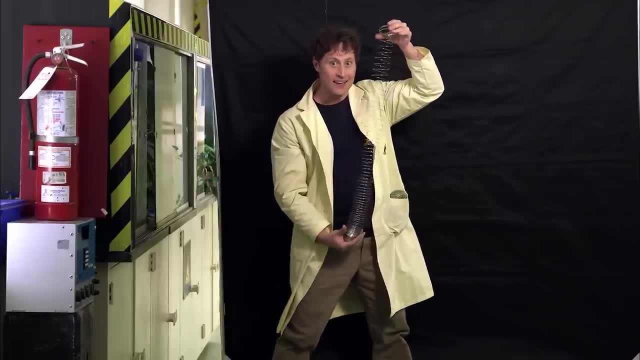 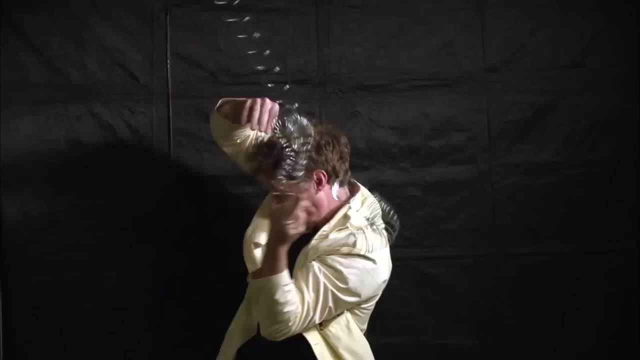 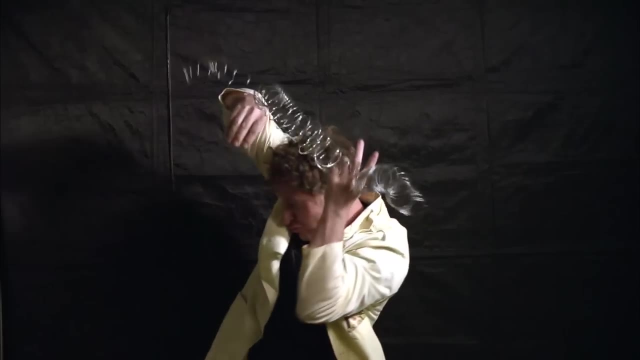 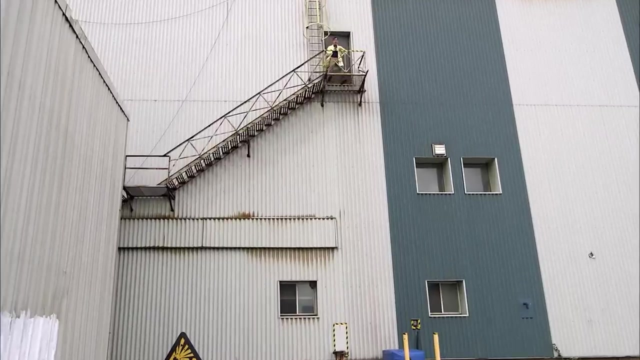 Will it happen differently with a longer spring? Huh, We're going to have a longer spring. Let's max it out, Don't tangle it. So, now that I'm up high on this fire escape, let's test it out. 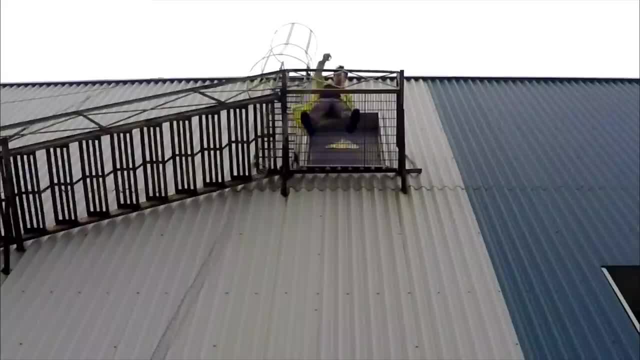 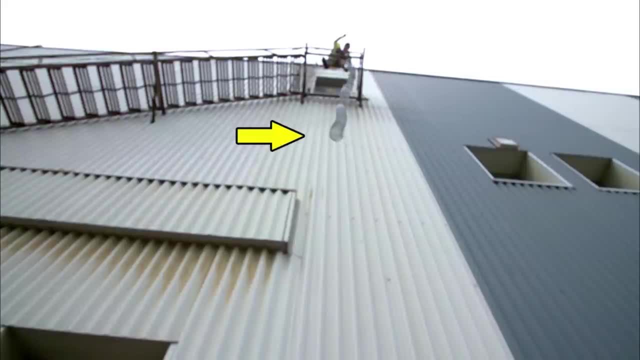 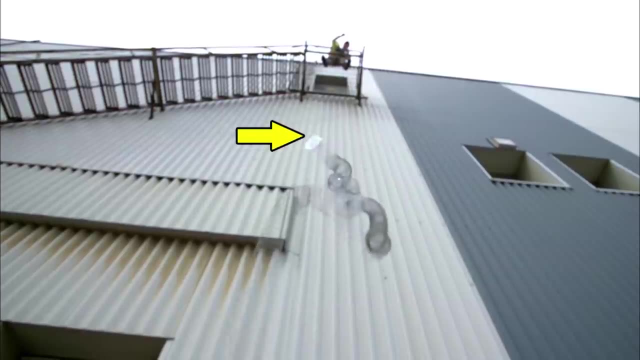 Okay, Three, two, one go A longer. spring still has the same forces working on it: The tension of the spring pulling it up and gravity pulling it down. No matter what size of spring, these forces cancel out for the bottom of the spring until the top. 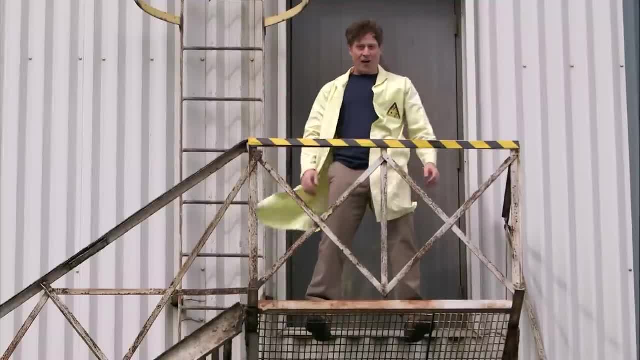 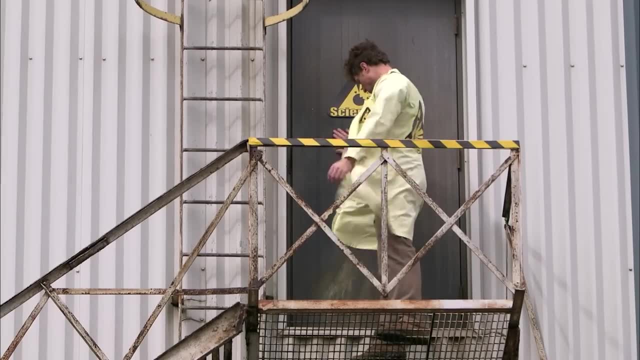 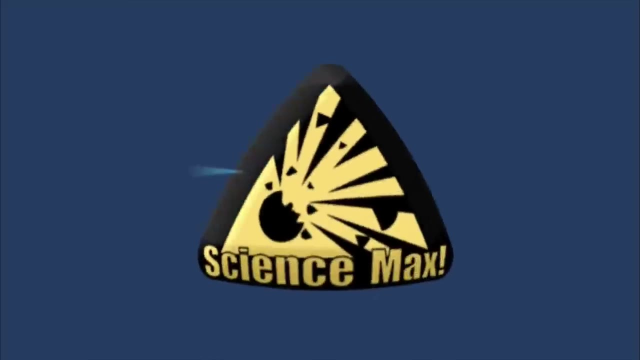 meets up with it. So there you go, An almost gravity-defying spring. Uh hey, There's no door handle on this door. I guess I have to take the stairs. Whoa, Sonya and I are maxing out the hoop glider out of bigger. 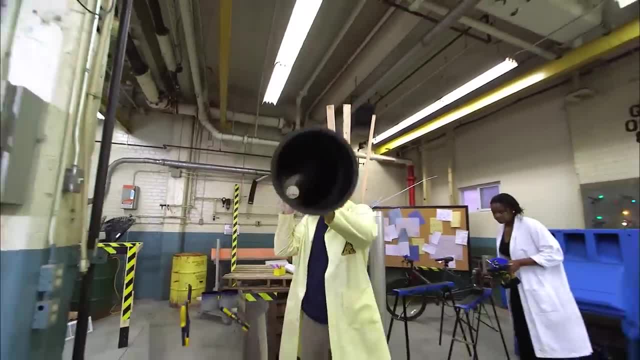 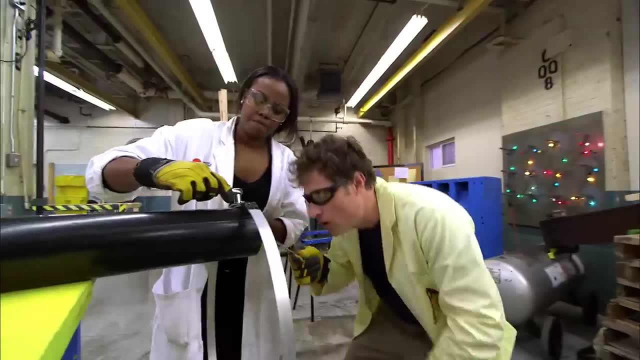 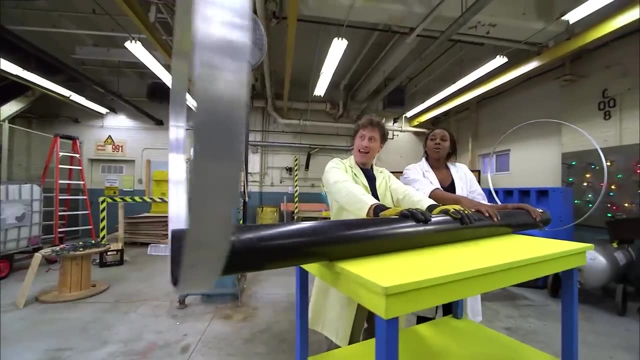 and better materials. This is the largest tube I have Right, A giant ABS pipe and some bendable metal to make into hoops. Then we attach them all together and, Okay, big hoop is done And little hoop is also done- Awesome. 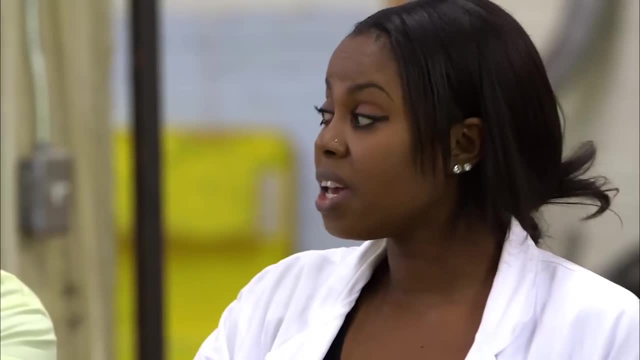 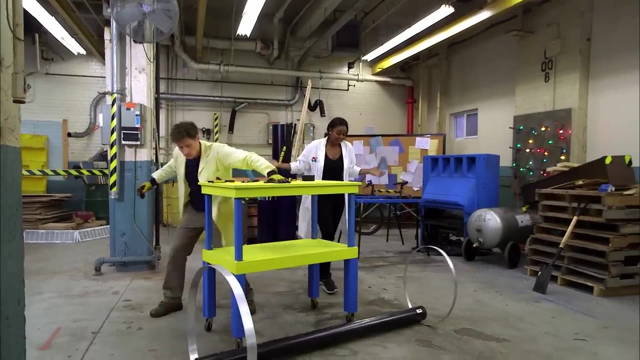 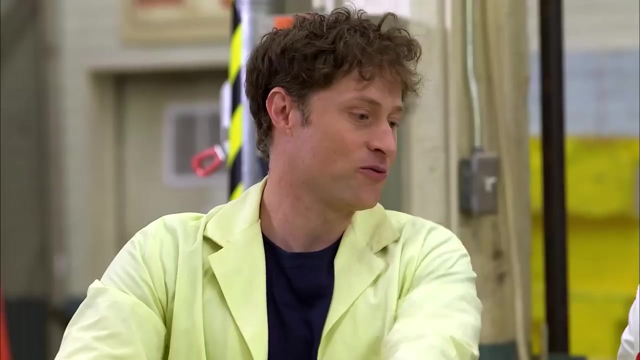 Not bad. Not bad at all. Super solid. So it might not fly as well as we'd like, But something heavy can always be good, right? Oh no, That's what I'm talking about. See how solid it is, No damage whatsoever. 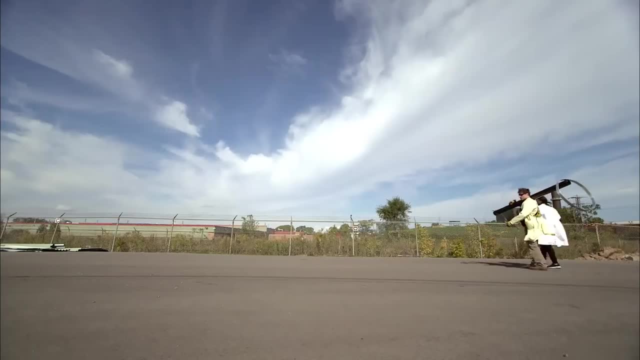 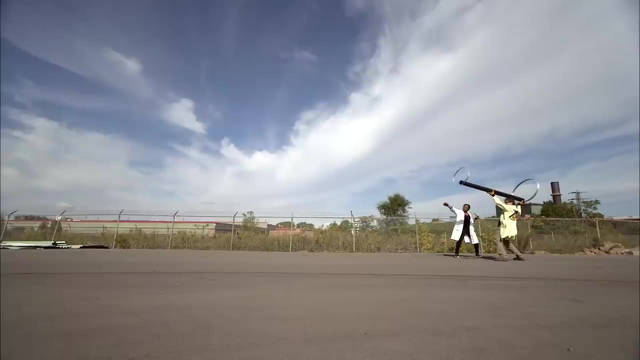 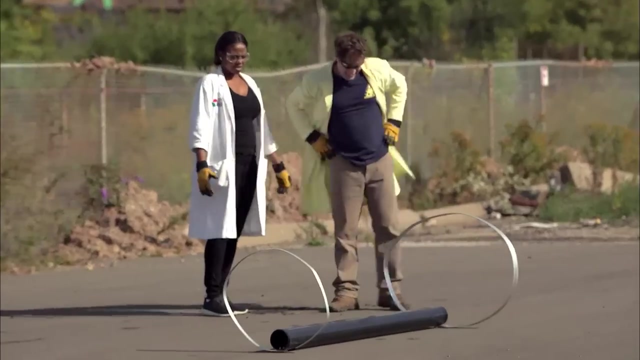 Want to test it? I think we should. Okay, I'm excited. We take our plastic and metal hoop, glider outside to test it and Ready, Ready. One, two, three, Huh. It didn't really fly, did it? 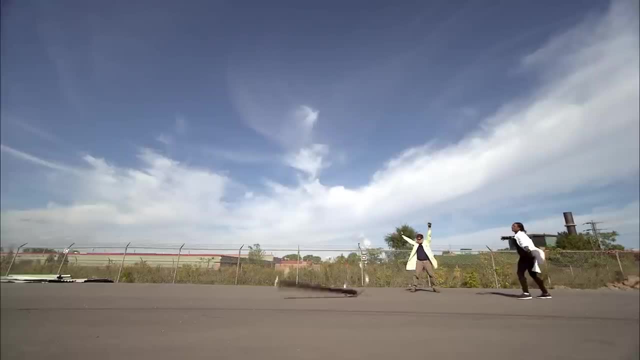 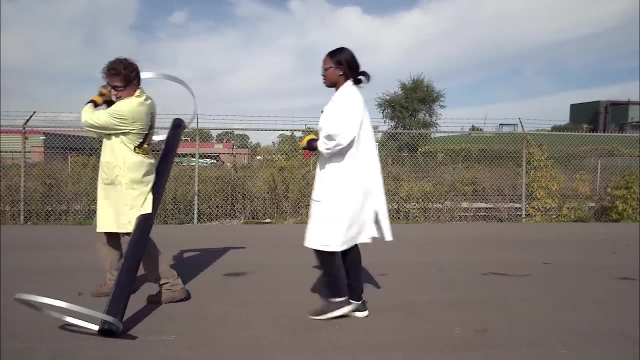 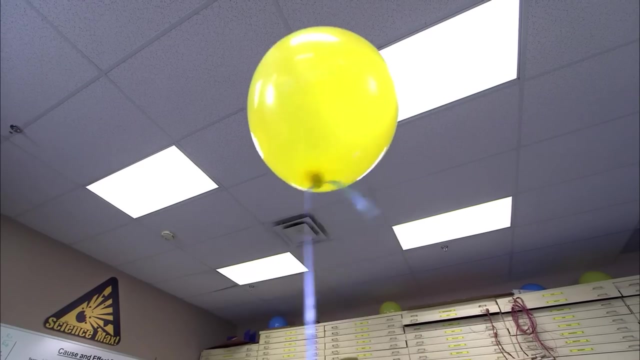 Sonya and I made a very solid design, but the problem with it became pretty obvious. Yeah, It's just too heavy. Well, that's what science is. Back to the drawing board. Mini Max: Here's something fun you can do. 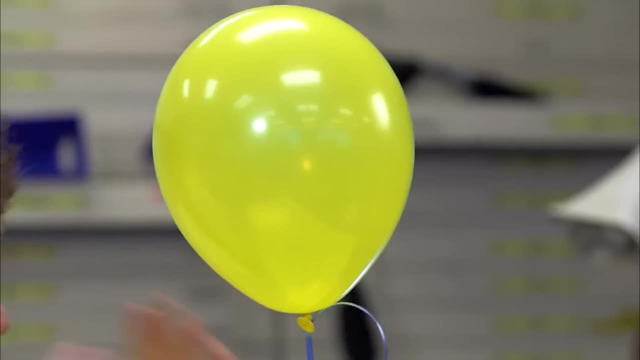 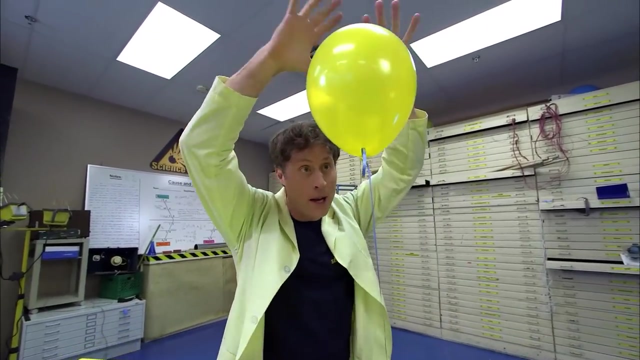 if you ever get your hands on a helium balloon. Now, helium balloons float up not because they defy gravity, but because they're lighter than air. It's because the heavier air on them actually falls past the balloon, and that ends up pushing the balloon up. 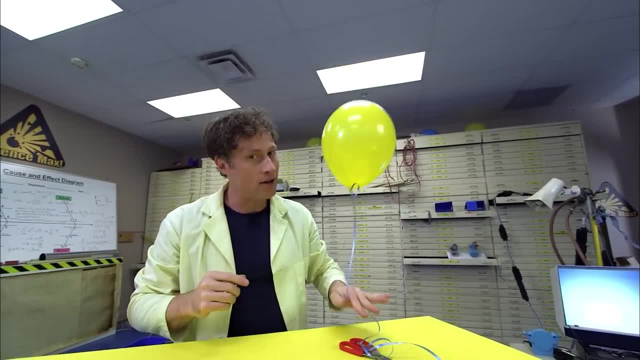 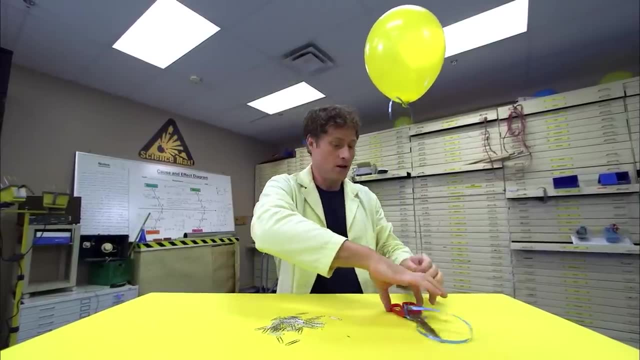 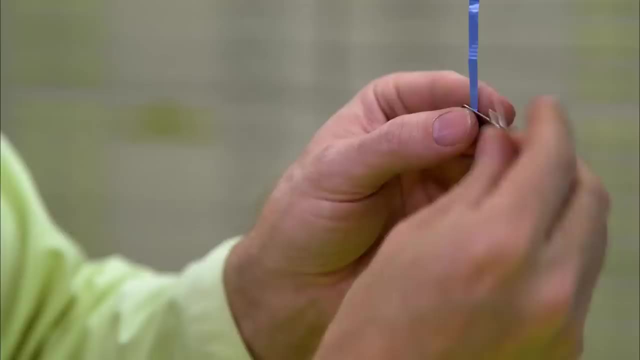 But what if this helium balloon wasn't lighter than air or heavier than air? It was exactly the same. This is what I like to do: Just take a helium balloon with a long ribbon and a bunch of paper clips and adding a little bit of weight every time. 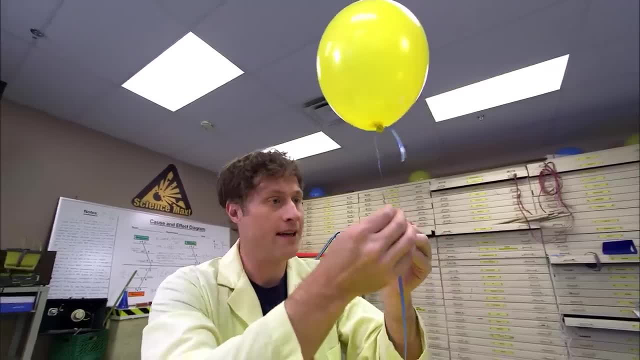 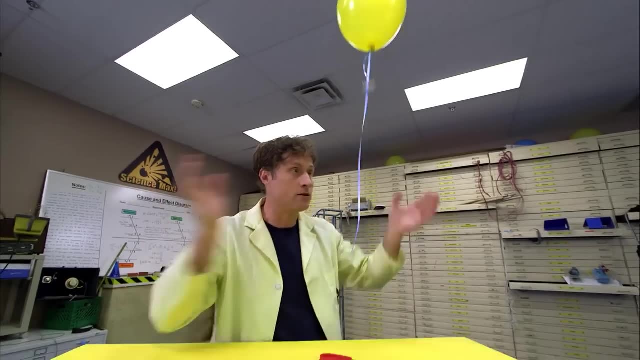 And what we want to do is make this balloon neutrally buoyant. That means it won't go up or down, but it will be neutral. Let's check it every once in a while. Let's see. three paper clips is clearly not enough. 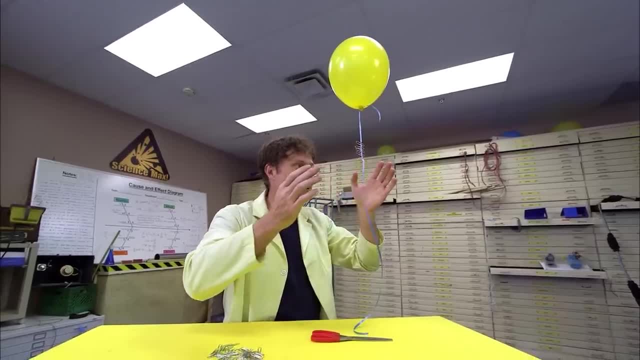 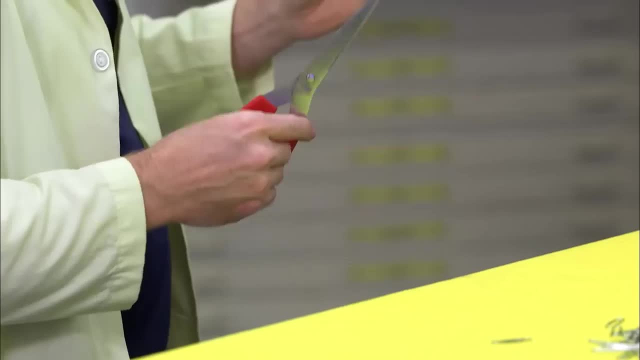 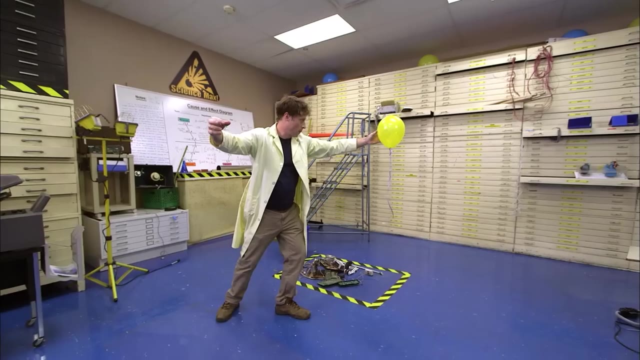 Five paper clips is Ooh. five paper clips is pretty close. It still might float down. so you want to take off just a little bit of weight? maybe about there? Watch this: You just take the balloon and you put it somewhere and it stays. 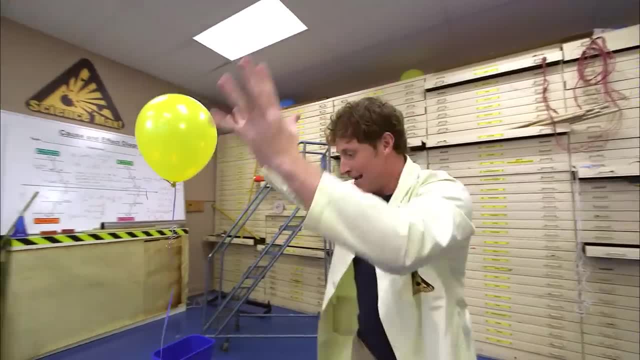 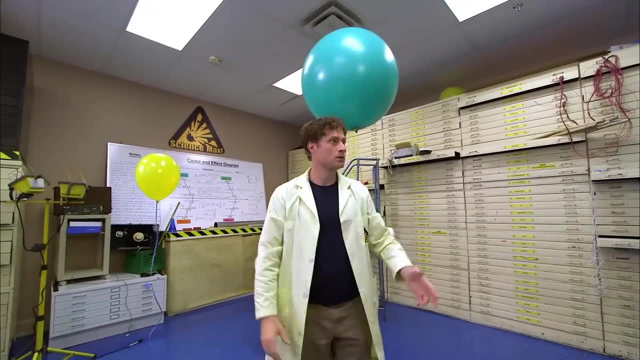 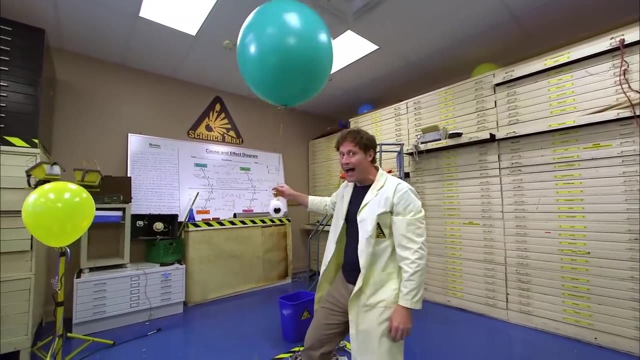 It stays put, It doesn't go down, It's attached to nothing. Now let's max it out. Huh, I had a big balloon and it was a- Oh there, A giant balloon, and look, it's a great paper towel. 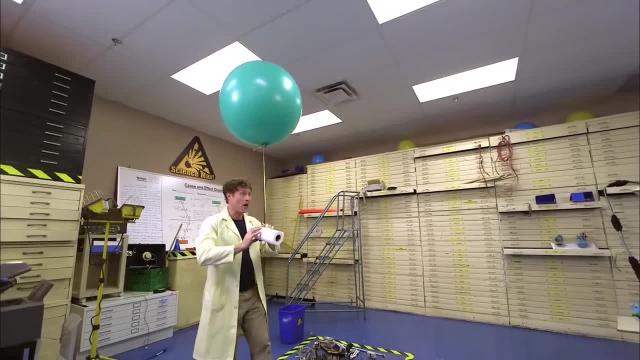 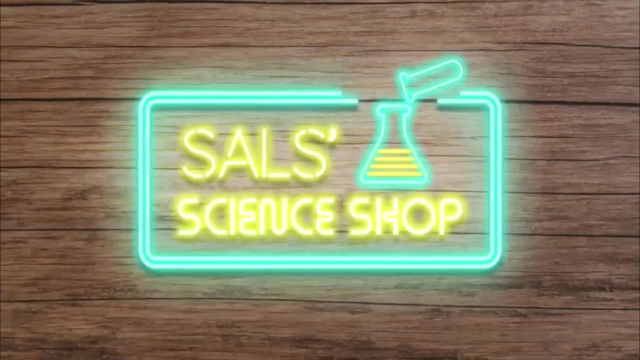 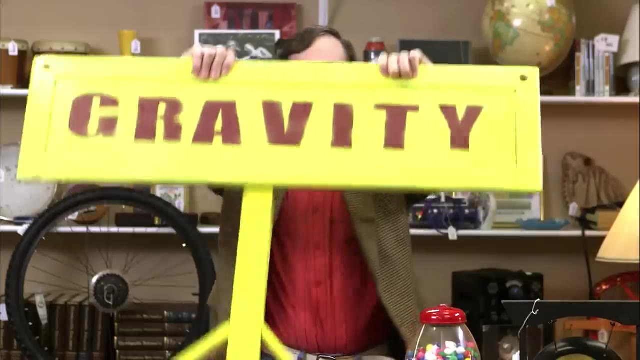 delivery device Say: did you want some paper towel? Here you go. Science. Yeah, don't worry about it, Ramona, Just put them up. high, Yeah, higher, Good, Hey, Gravity, Gravity, huh, Gravity makes things fall. 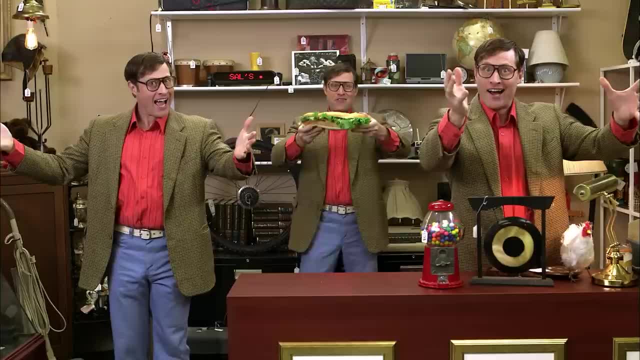 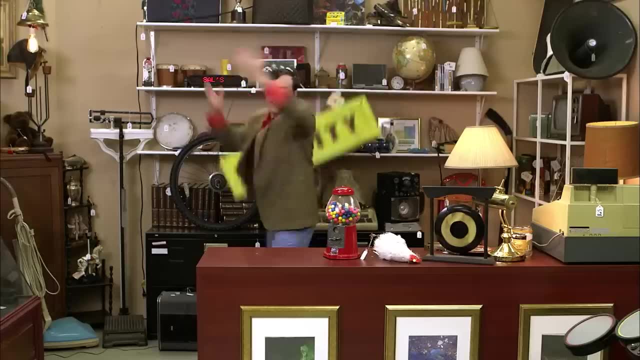 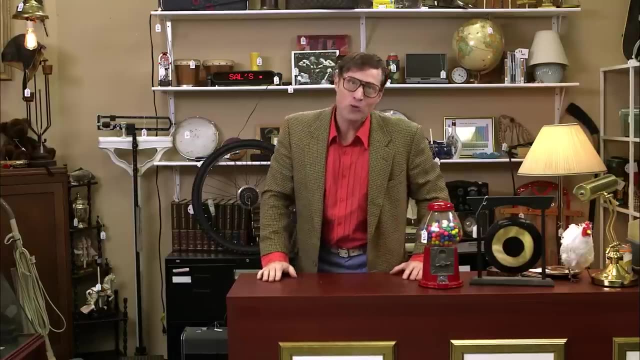 But where do they fall? They fall down, Oh, Towards the center of the Earth. Yeah, Gravity, It fell, didn't it? So the Earth causes gravity, right? Well, yes, Gravity, Oh, come on Everything that has mass. 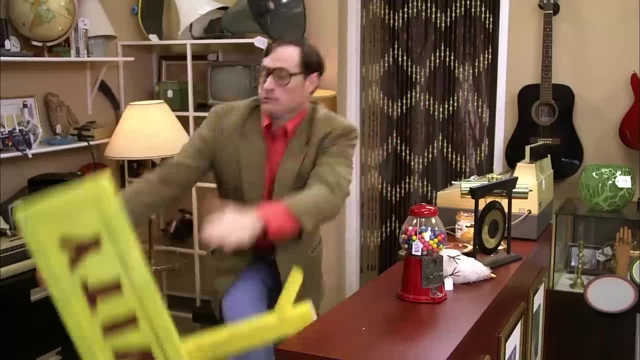 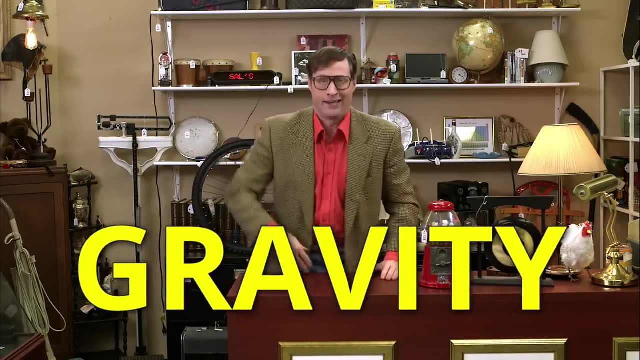 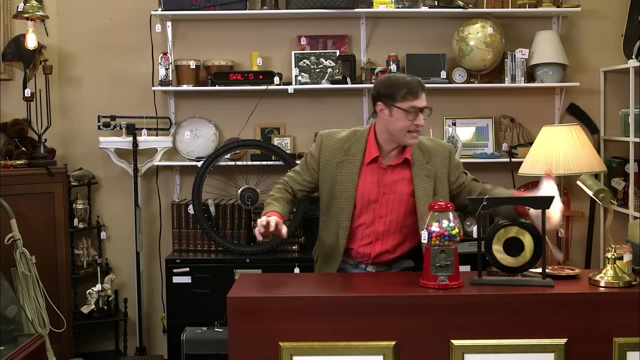 has gravity, Gravity, But the Earth has so much mass that the gravity produced by everything else is like nothing. I mean forget about it, But let's say I was in space with this chicken. I would have gravity and I could exert a gravitational force. 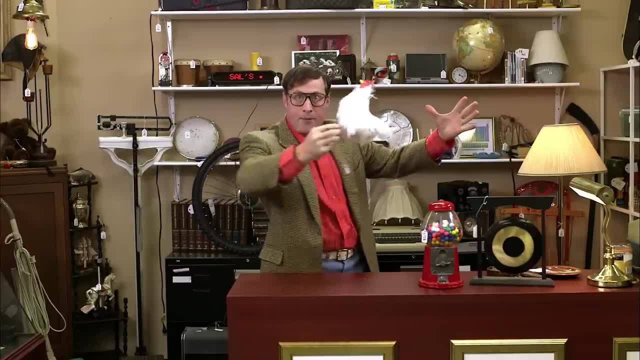 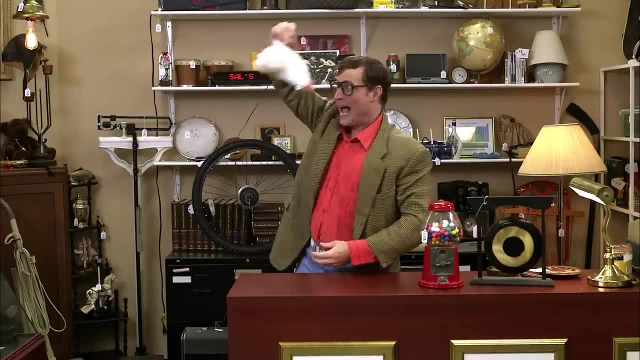 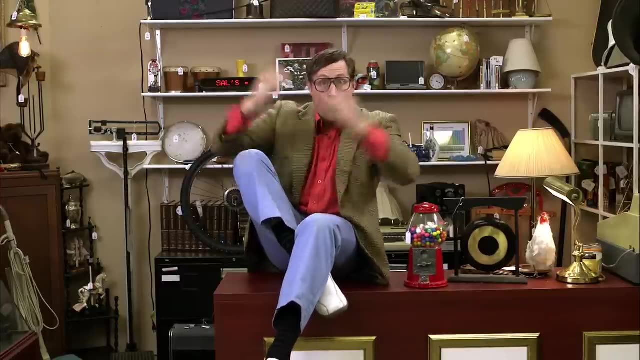 on this chicken And if I get my angles right, I might be able to get the chicken to orbit me like a moon. Behold my chicken moon. Huh, Gravity. But let's get serious. What causes gravity? We don't know. 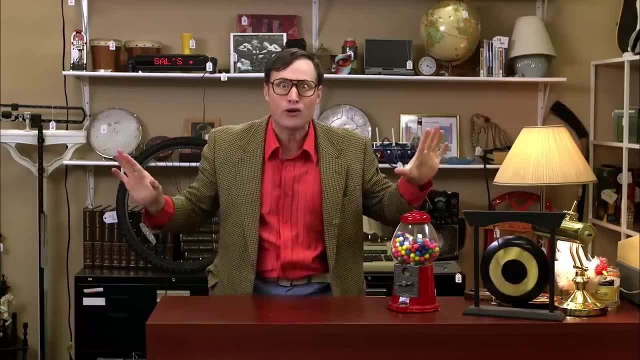 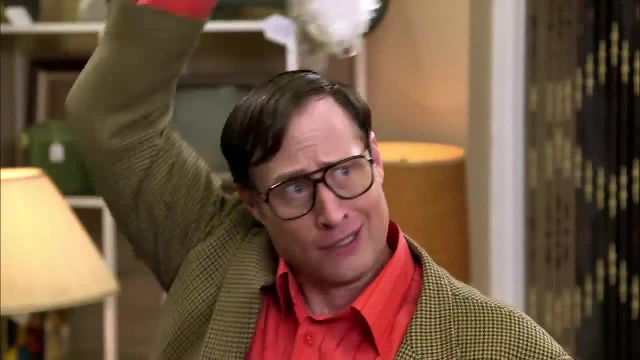 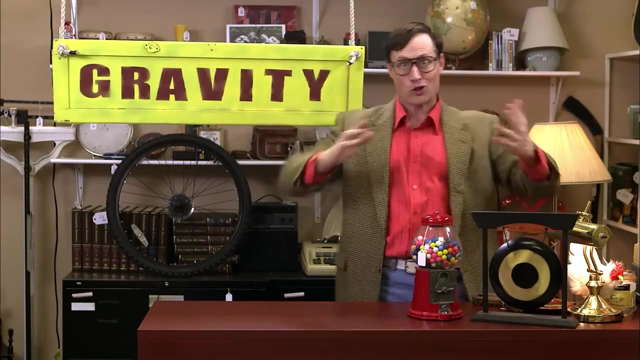 What we do know is that without gravity, there would be no universe as we know it. No you, No me, Chicken moon, I'd miss my chicken moon. Chicken moon, You, what Gravity? Like it or not, the universe wouldn't exist without it. 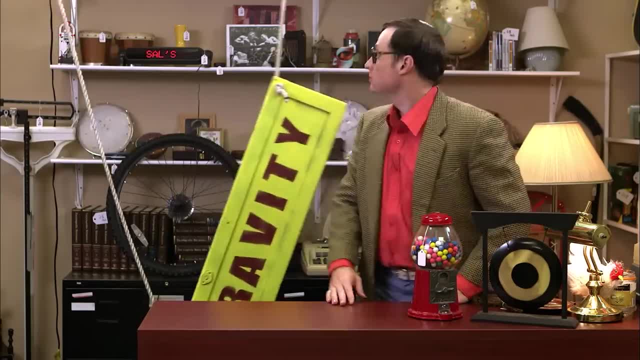 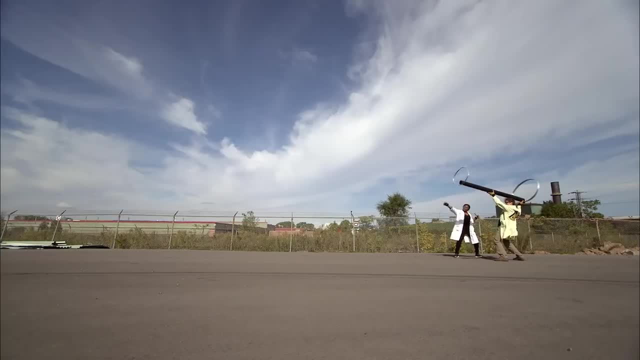 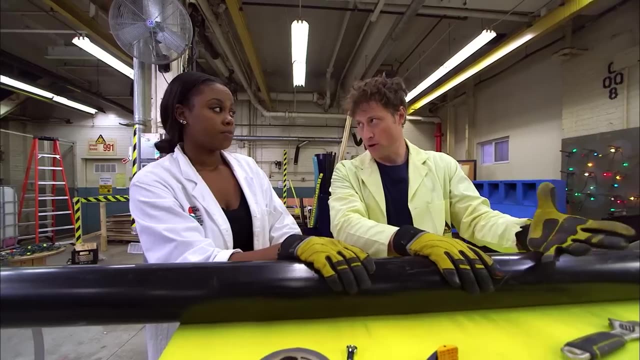 You like the sign, I'll give you a good deal. Half off Back to our hoop glider, which was too heavy. Here's what I don't get. I can still pick it up and throw it. An airplane is way heavier. I could never pick up an airplane, but that can fly. That's because airplanes have engines, so it has a constant source of thrust. When we throw it we just have an initial source of thrust, So we're throwing it eventually loses its energy. 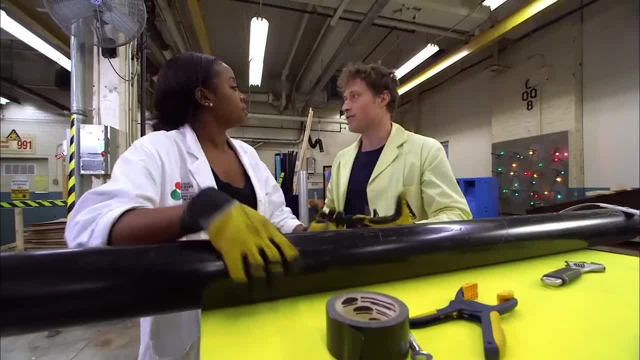 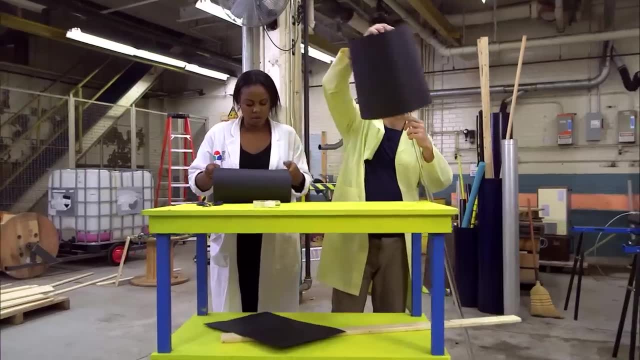 therefore, it falls to the ground. So we need something that's light and something that's strong. Let's see what we can find. It could be paper. We make hoops and attach them with some duct tape and run outside to try it out. 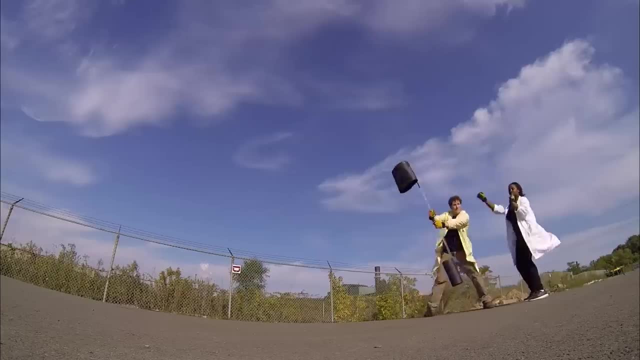 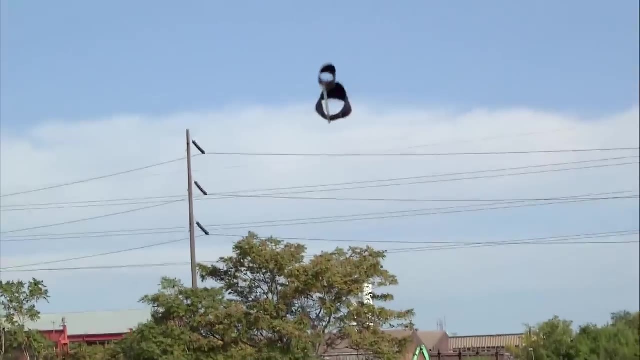 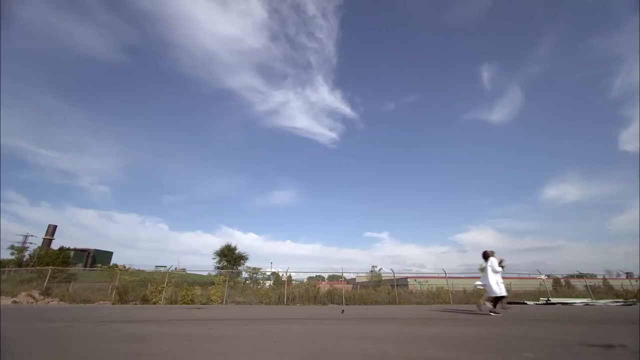 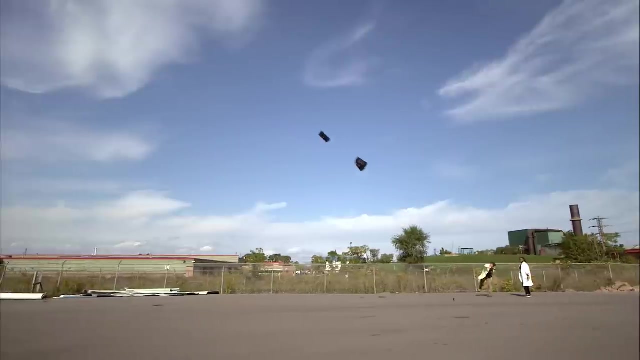 Hoop glider dance. Okay, Three, two, one. That's pretty good. That was amazing. Let's try that again. Here we go. I throw the hoop glider, and also further than I could have just thrown the pipe by itself. That's pretty good. So we've done a good job of making something that flies. Why don't we make a couple different kinds out of different materials and we'll see if we can get one that flies even better than this? I think that's a good idea. 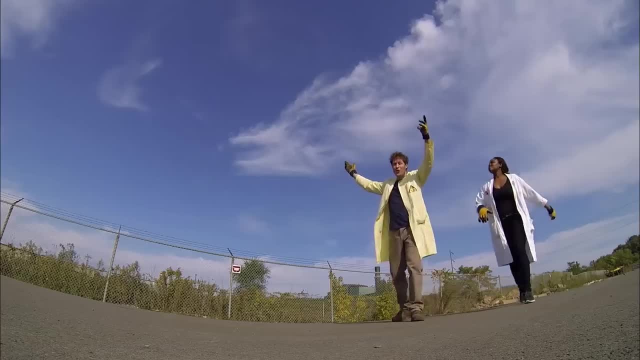 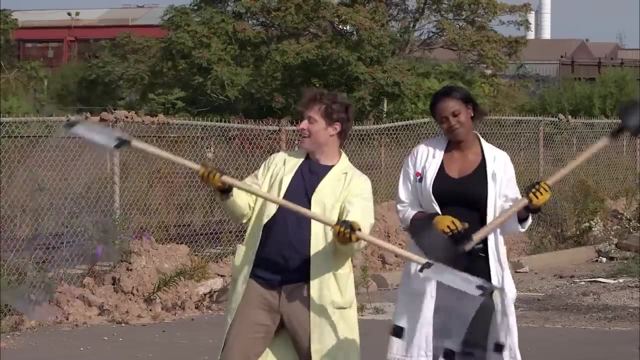 Yeah, okay, let's do it. Sonya and I have created a pretty good maxed out hoop glider, but we wanted to see if different materials would make an even better one, And I I made this, Made a slightly heavier one. 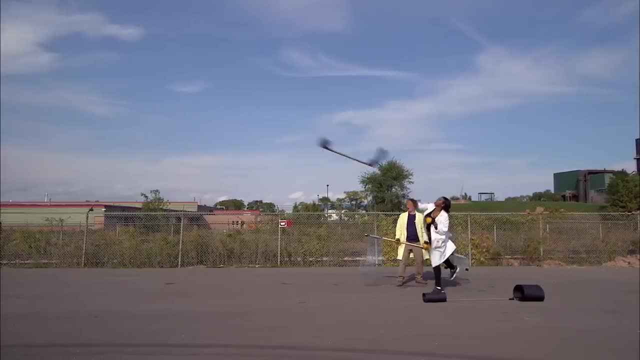 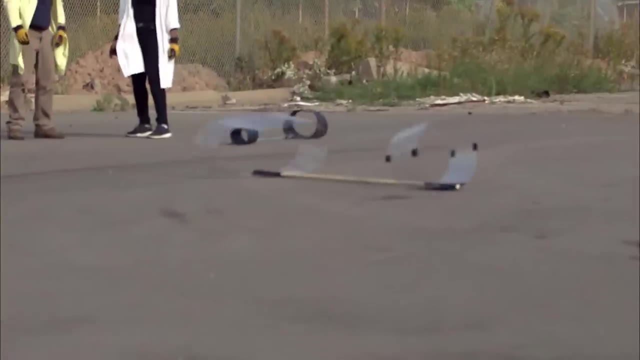 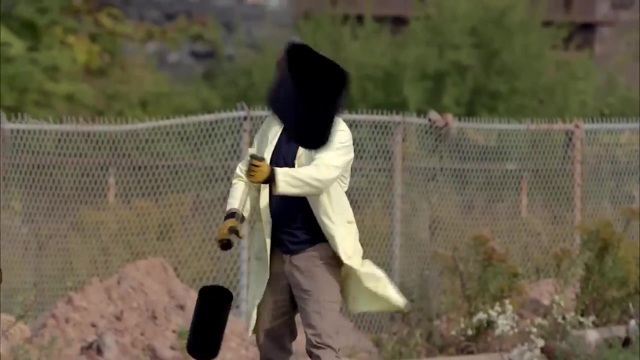 Let's do it Okay. three, two, one go. Not bad, My turn. Here we go. That didn't really go very far at all, did it? No, Okay, so now we can measure it against the one that we threw before. 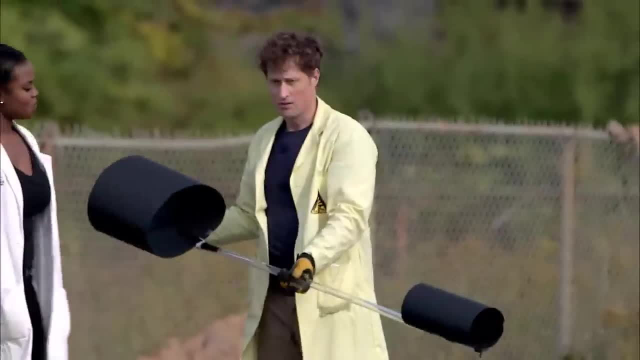 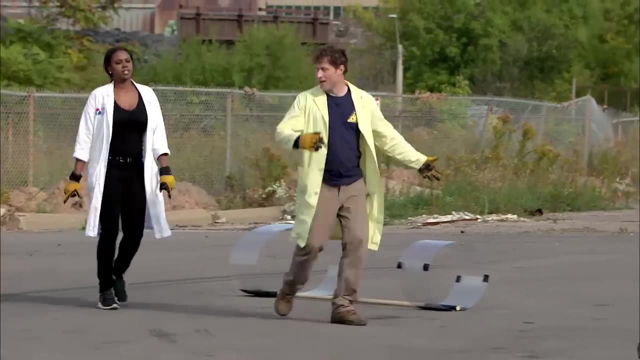 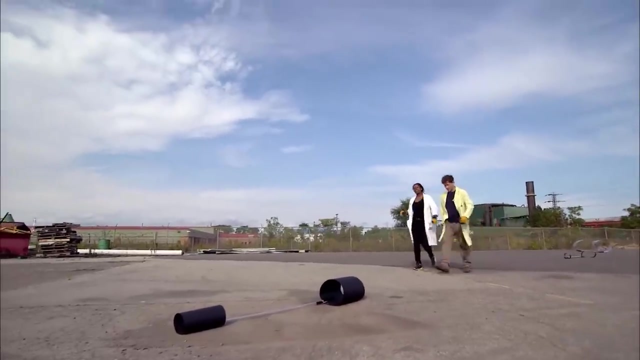 And that went pretty far. This went pretty far to see if we've got a better design here. Here we go. Wow, Awesome, So heavy one no. Light one, no, Interesting, Uh, no, This design seems to be the best one. 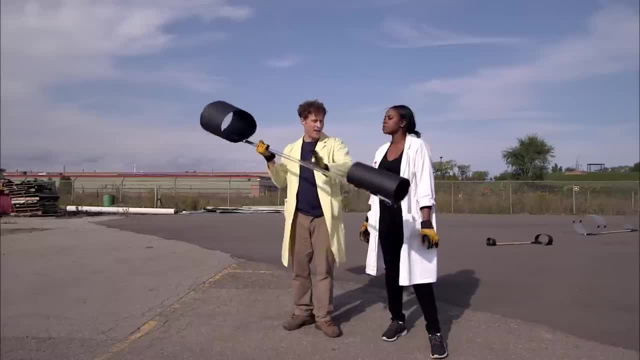 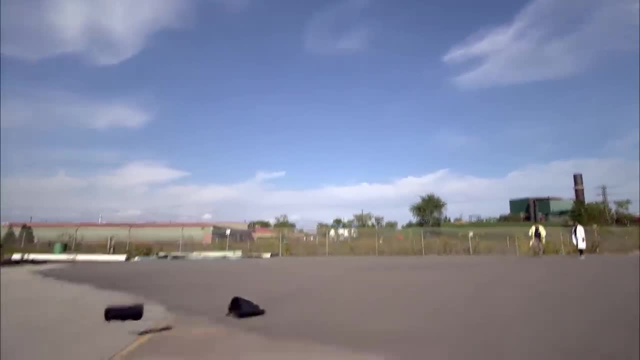 I keep thinking about how you were talking about thrust. Yep, All the thrust that we can put in is just what we can put in with one throw. Yeah, What if we could give it more thrust than that? How can we do that? 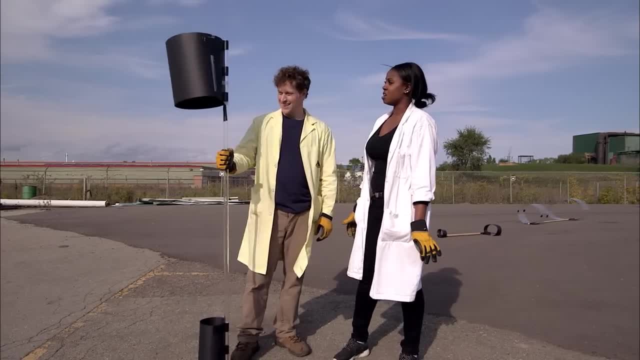 I don't know like some sort of slingshot or something Pretty big slingshot, But I think that sounds great though. Do you think we can make it? I think we can make a big slingshot for this. 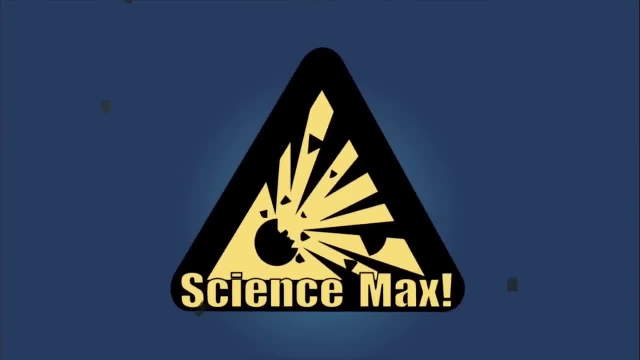 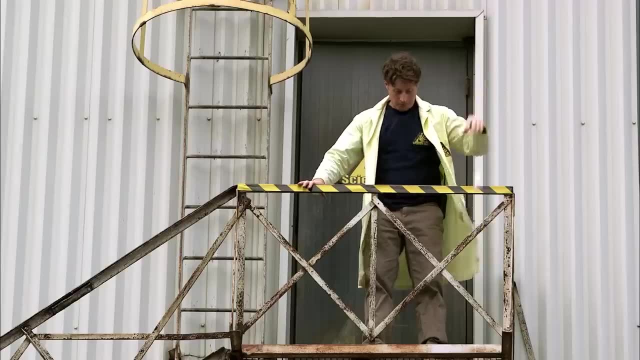 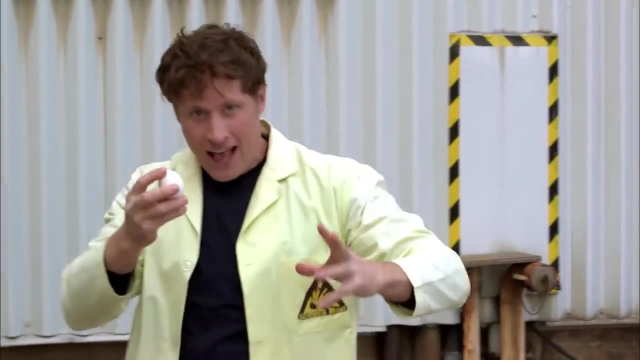 Why not? Okay, high five, Let's do it All. right, This is an egg. Eggs do not like to be dropped. Fortunately, we can use the power of science to design something that'll keep the egg safe as it falls. 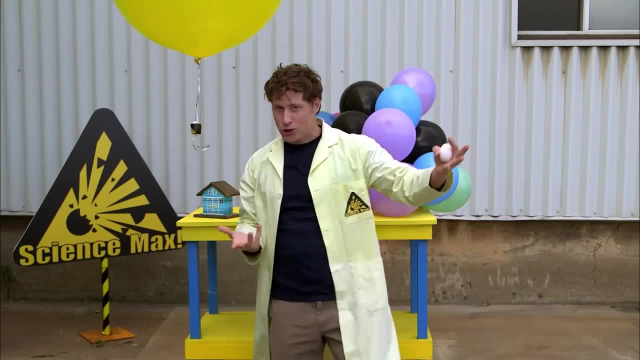 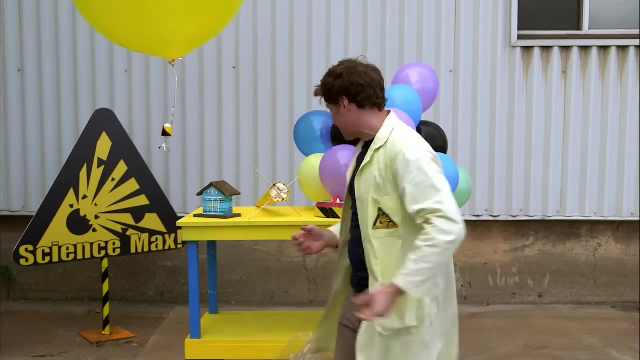 Behold Egg drop contraptions. The thing I really like about this experiment is there's no wrong way to do this. You can come up with any design you want and see if it works. This one here is a bunch of helium balloons. 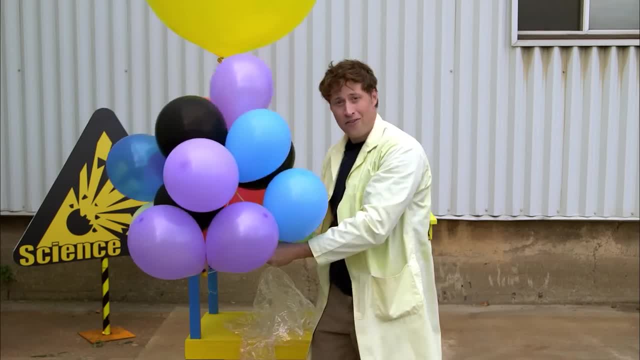 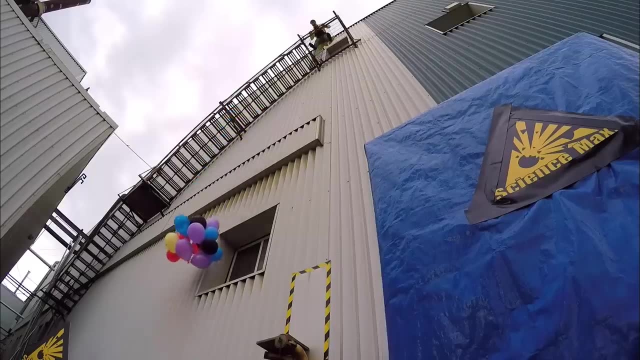 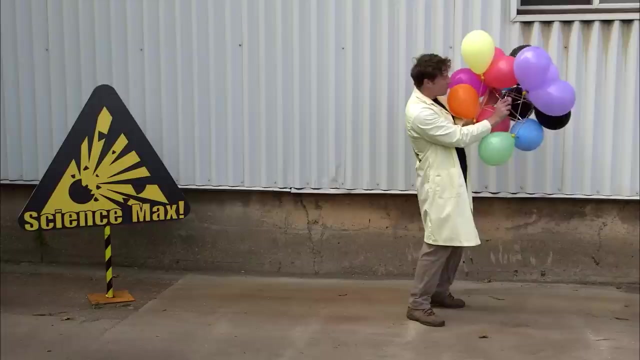 This structure is just to keep the helium balloons on, so the egg can touch down very gently. Here it goes, Whoa, And, And The egg is unharmed. That one worked really well- Success. This is a giant helium balloon. 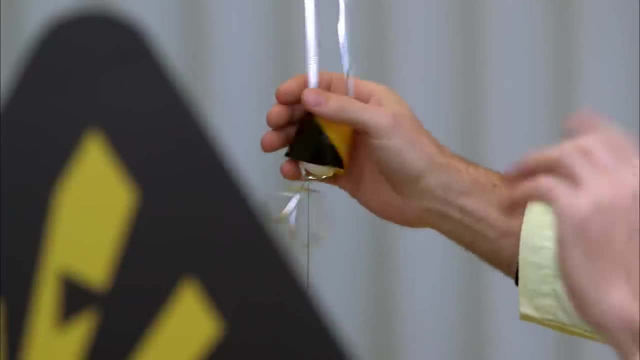 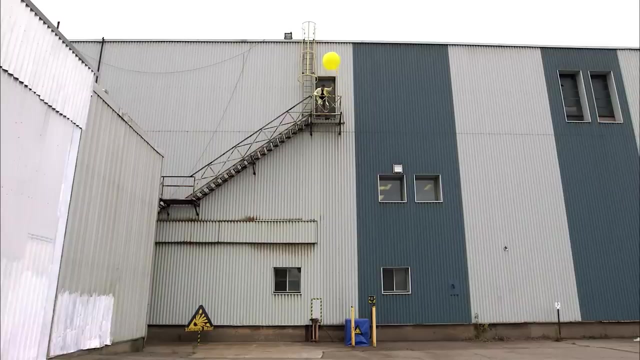 that, I think, will work pretty much the same way, because I think this balloon will drop just slowly enough that the egg can actually just touch and nothing will happen. Um, So that didn't work. And then there's this one, which has no slowing at all. 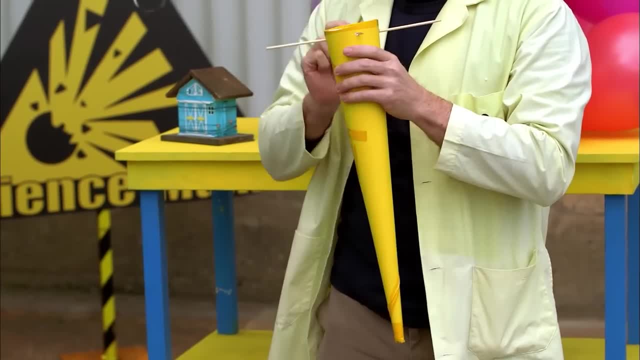 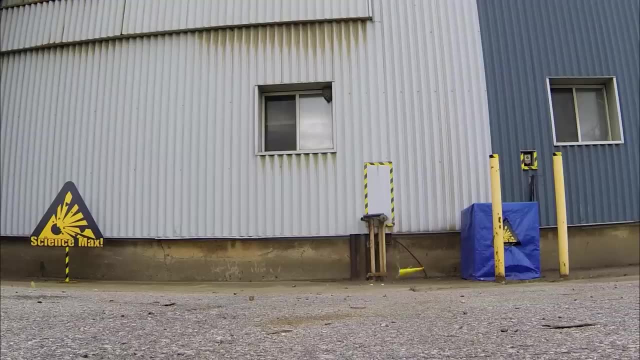 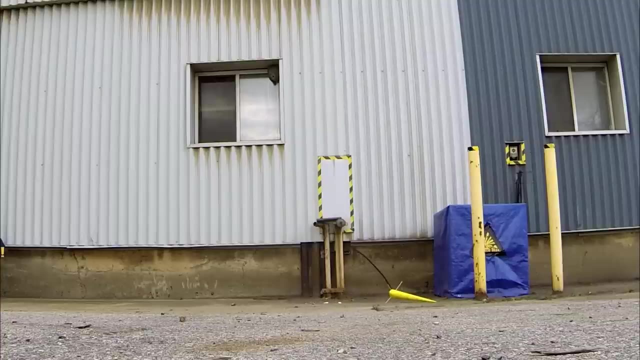 It's all designed to just absorb the impact, And the idea is that the cone will crumple and absorb the force when it hits the bottom. Oh no, Oh no. I think it would have worked if it hadn't turned in the air. 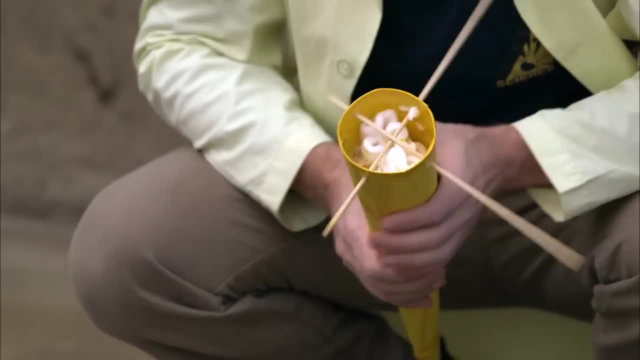 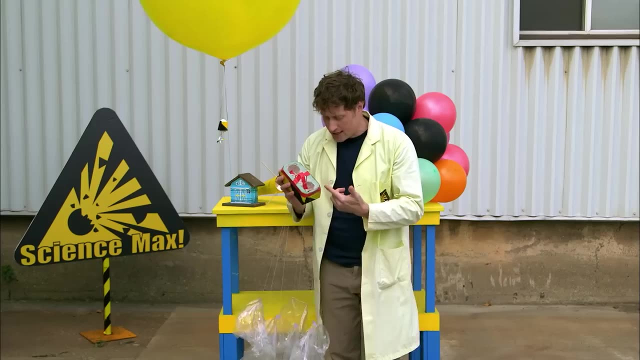 but it did, and well, I guess the egg is completely broken, So I'd call that one a fail. This one is the parachute. You see, the egg has been nestled into this foam container And this is a parachute that will hopefully slow the egg down. 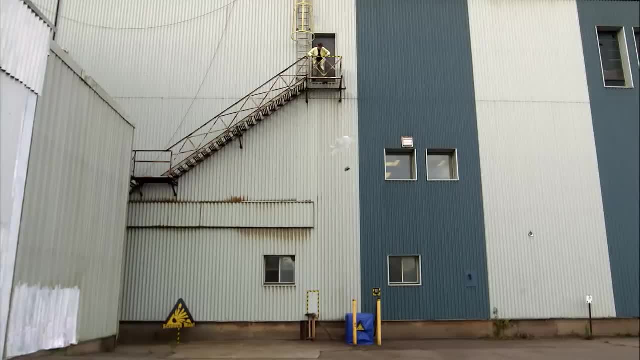 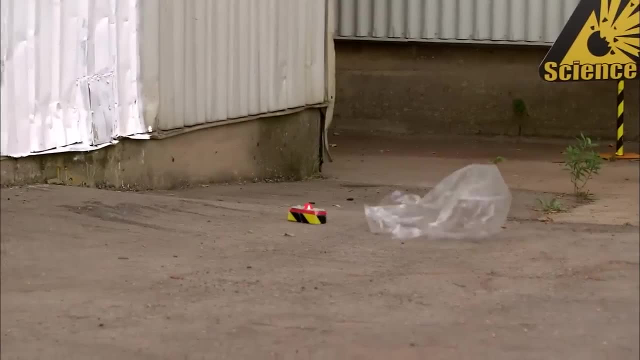 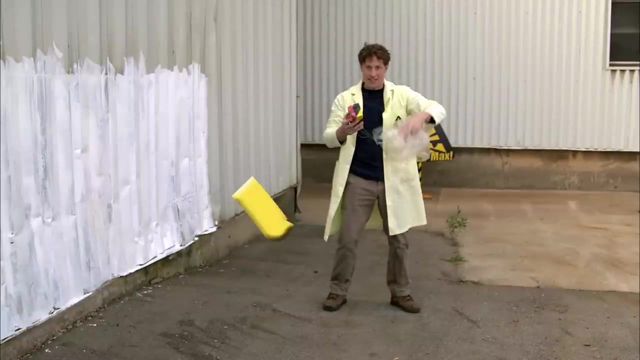 Whoo-hoo, Uh-oh, Whoa, Over Over Good, And That one seemed to work well. Yep, The egg is totally fine. The parachute worked, All right. Egg drop experiment- totally fun experiment to do. 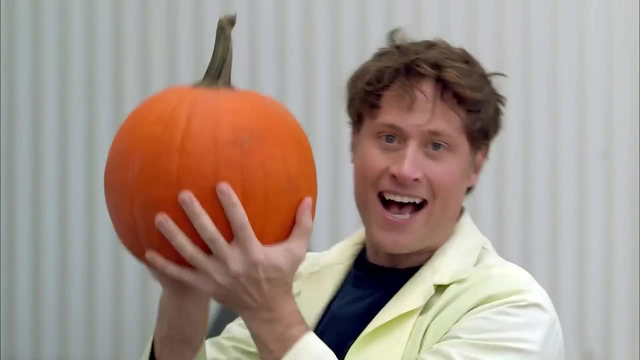 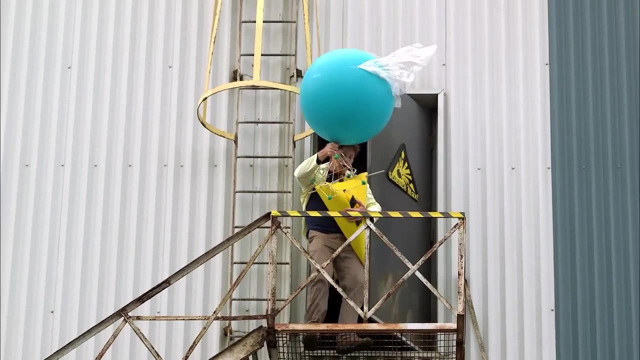 but the question is: how do we max it out? And the answer is: pumpkin drop. Same thing, except with a pumpkin instead of an egg. Come on, Okay, All right, Pumpkin drop with everything attached all at once. Okay, here we go, Ready. 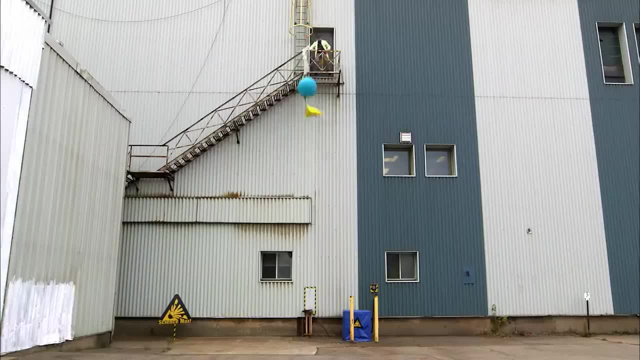 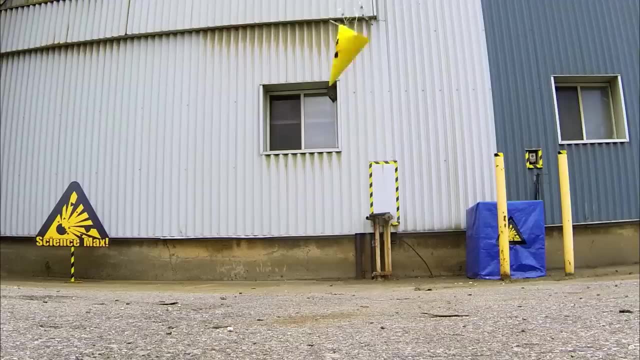 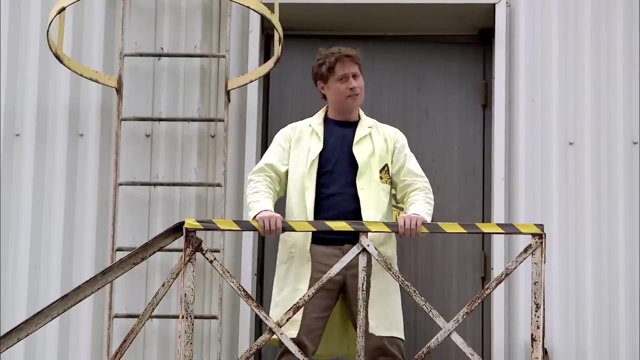 One, two, three. So what we've learned from this is: the heavier something is, the more force is acting on it from gravity, which means the harder it is to slow down when it's falling. Okay, Fair enough, You win this one Gravity. 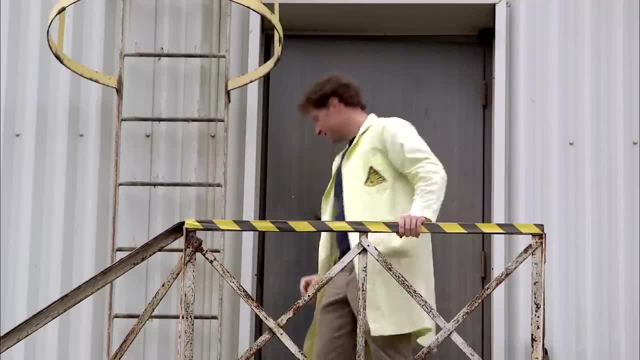 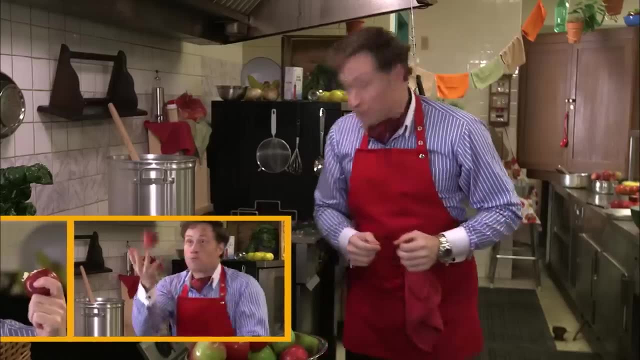 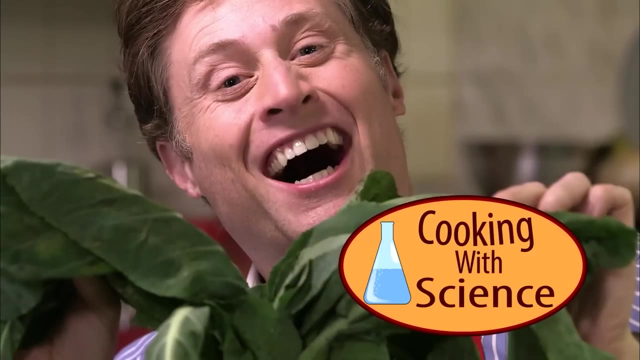 But I'll beat you. next time I'm, I'm gonna get a broom. Being a chef is my absolute passion And cooking up science recipes is my speciality. I'm Buster Beaker and this is Cooking With Science. Oh hello. 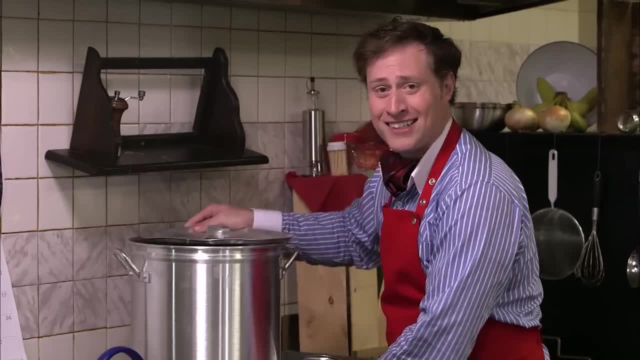 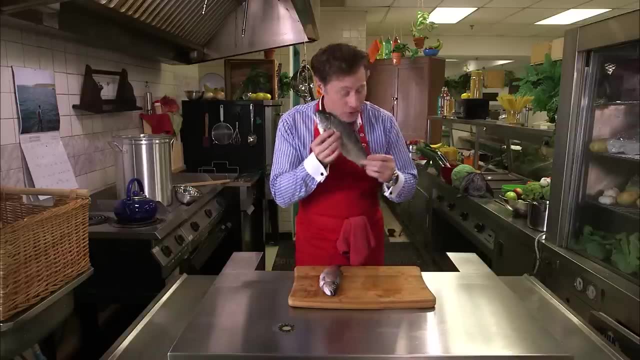 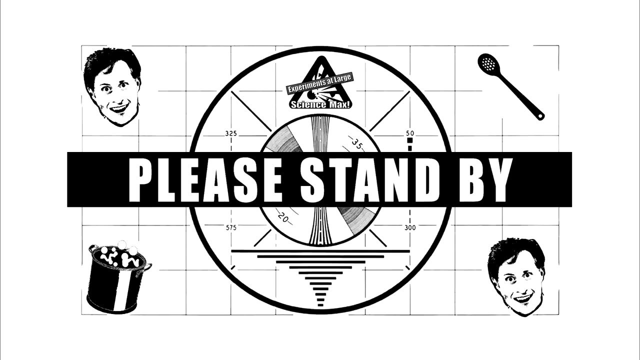 Welcome to Cooking With Science. I'm Buster Beaker Delicious. Nothing is more important to have fresh than your seafood. It's what makes the difference between a fresh fish and one that isn't so fresh If you live by the ocean. 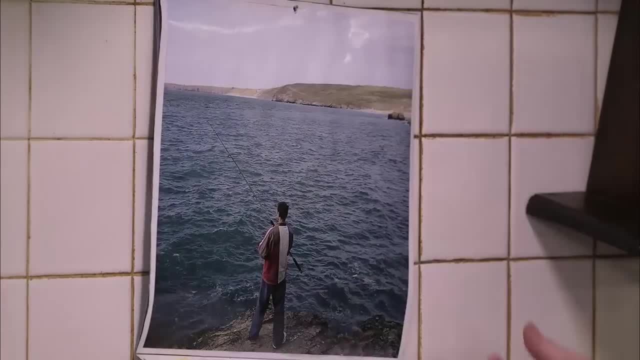 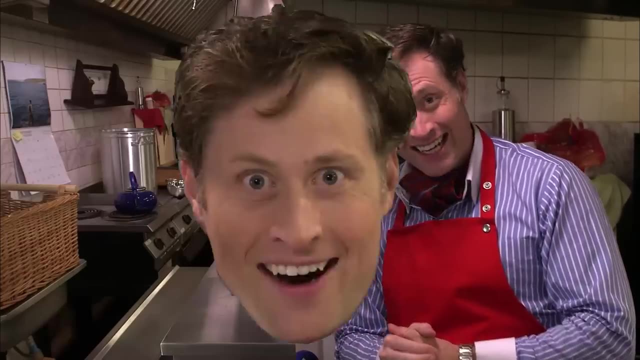 you probably know that the water gets high tide and low tide. Look closely, It's the same location. Amazing. But did you know that this is caused by the gravity of the moon and the sun? See, this cookie is the Earth And this little happy fellow. 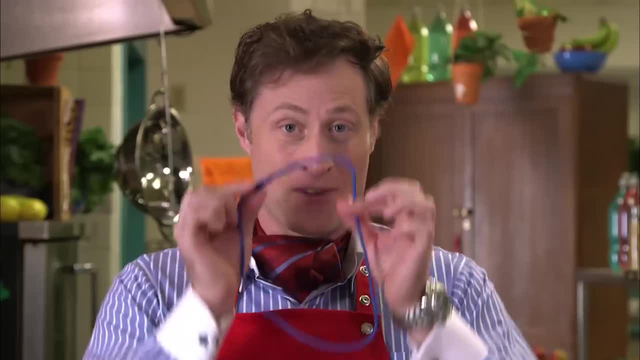 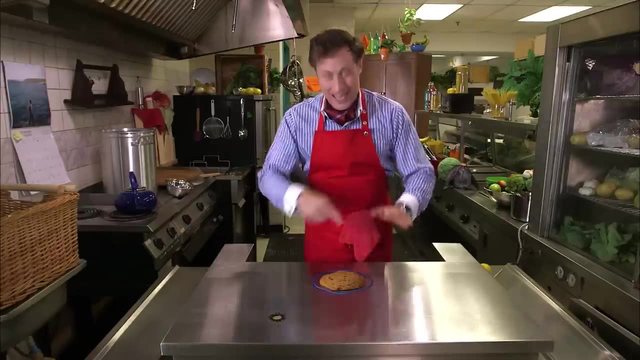 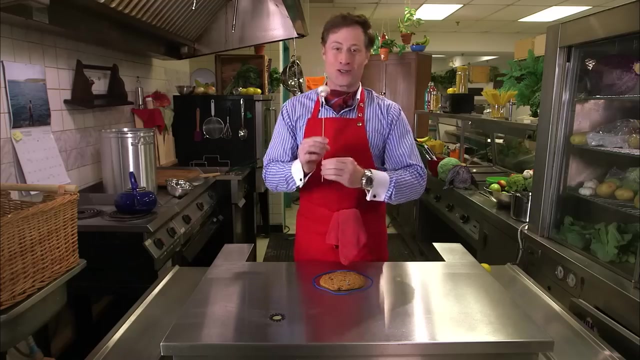 is me, And this string represents the water around the Earth. If we didn't have gravity to worry about, the water would all be equally deep around the Earth. But here comes the moon, this mushroom. Now the moon has gravity and that pulls the oceans. 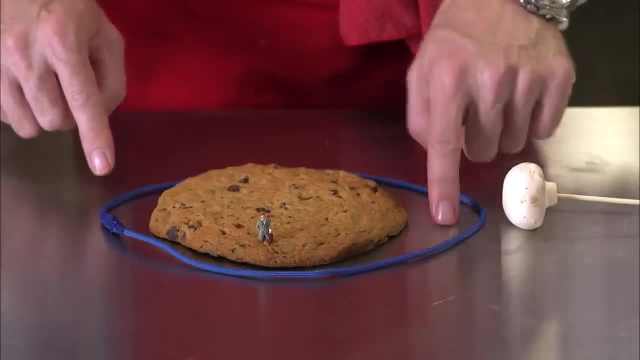 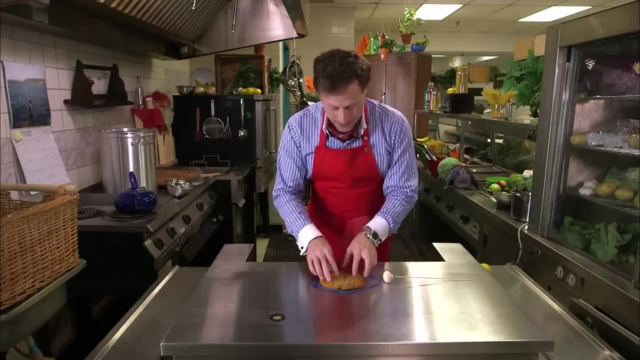 towards it a little bit like this, And that creates high tide there and low tide here and a little bump of high tide on the other side of the Earth. And the reason I'm on it: I experience low tide and high tide. 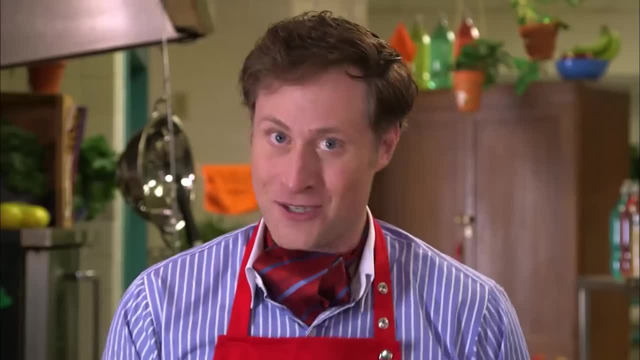 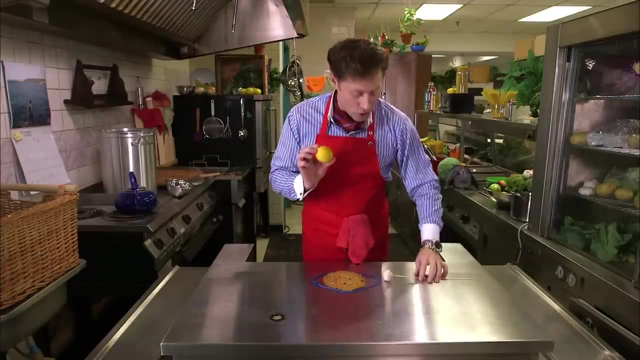 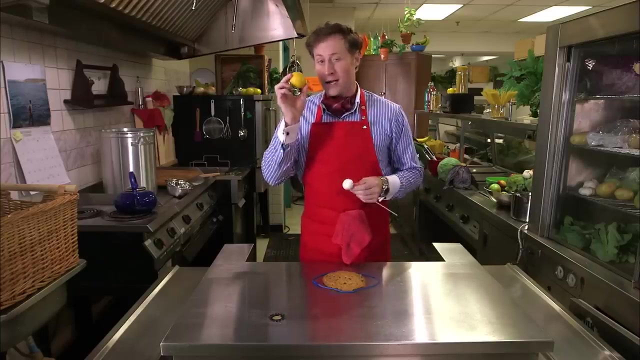 and low tide and high tide. Very interesting. But there's another factor: The sun, or this lemon. Now, the sun also affects the tides, but not as much as the moon. Now, the sun does not affect the tides as much as the moon. 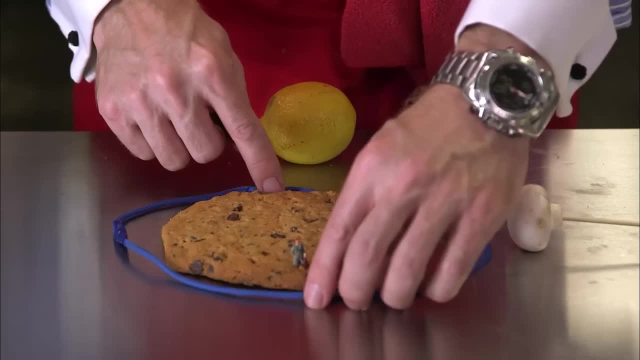 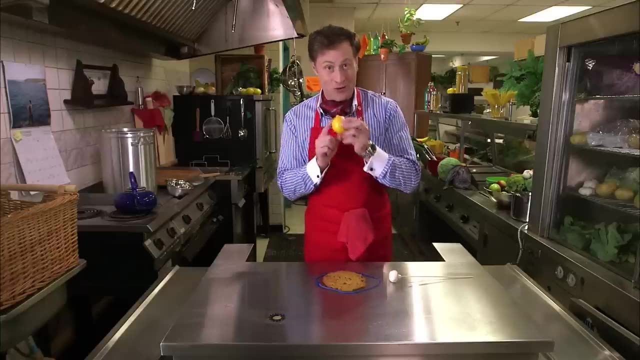 because it's much further away, But it still has an effect. If the sun was here, then the tides would be a little bit like that and the tides would be less severe. But if the moon and the sun line up, 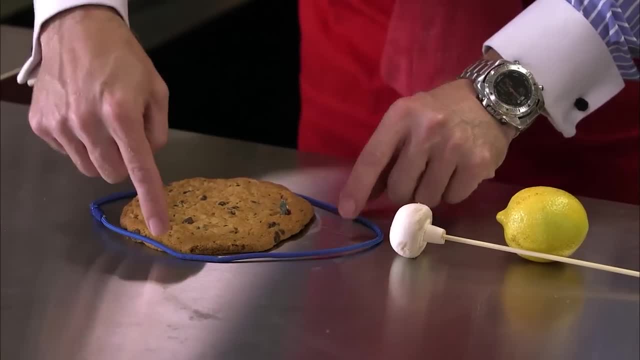 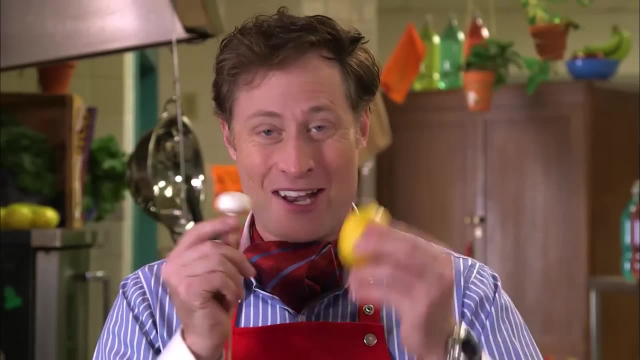 like over here, you'd get a very, very high tide and very, very low tide. So there you are. That's how the tides are affected by the gravity of the moon and the sun. Mmm, delicious. I'm Pastor Beaker, and thank you. 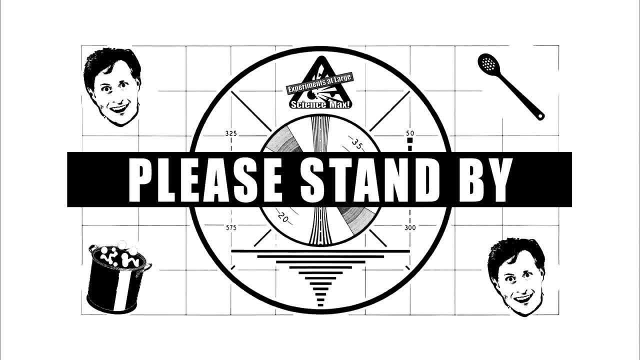 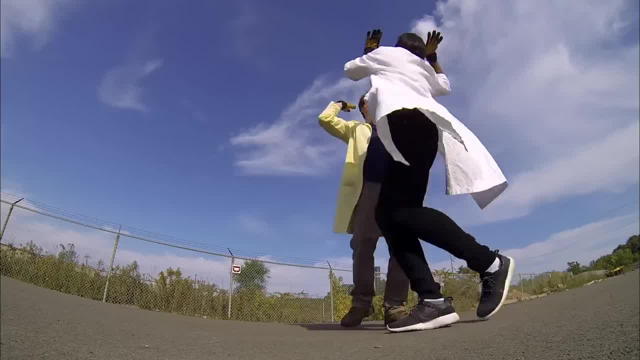 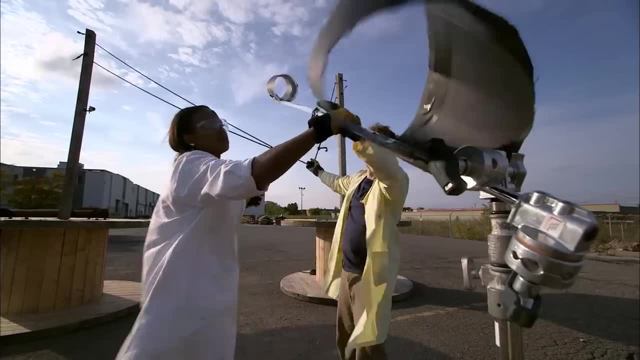 for joining me on Cooking With Science. Oh, This workout hoop glider was working pretty well. That was amazing. But we could only give it so much thrust by throwing it. So we came up with the perfect Science Max solution: Our giant slingshot. 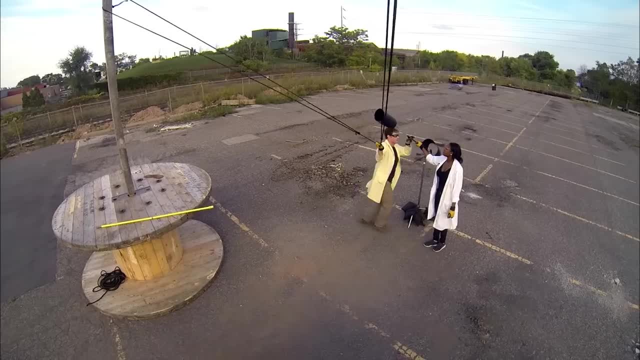 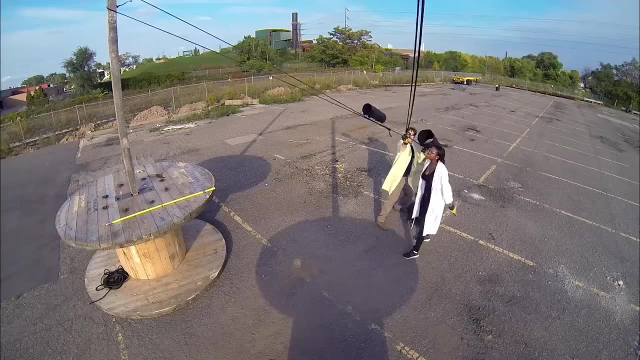 Woo-hoo-hoo-hoo-hoo, We pull the bungee cord back and hook it onto our hoop glider. I am ready to fire. Count me down Three, two, launch it, Woo-hoo-hoo-hoo-hoo. 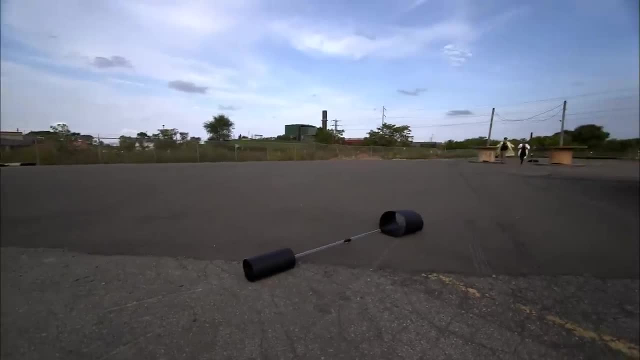 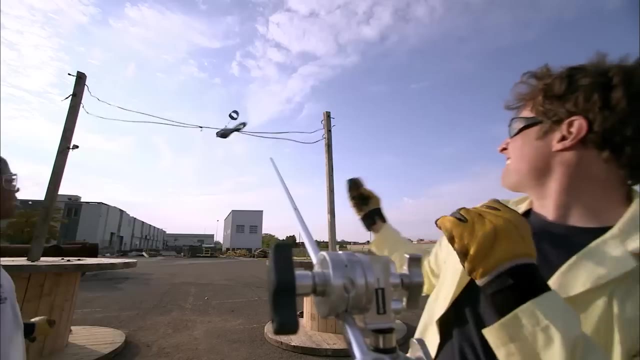 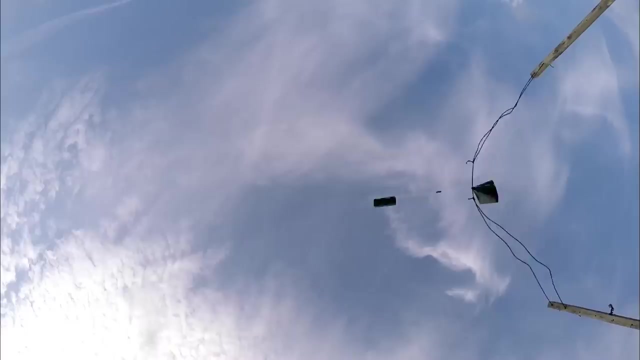 Woo, Very nice. Woo, Our slingshot is amazing. By giving the glider more thrust, that is more energy at the beginning, so it's going faster. when we launch it, the glider soars through the air and flies a long way.